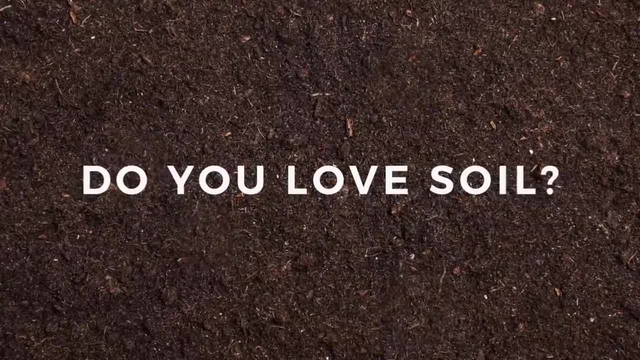 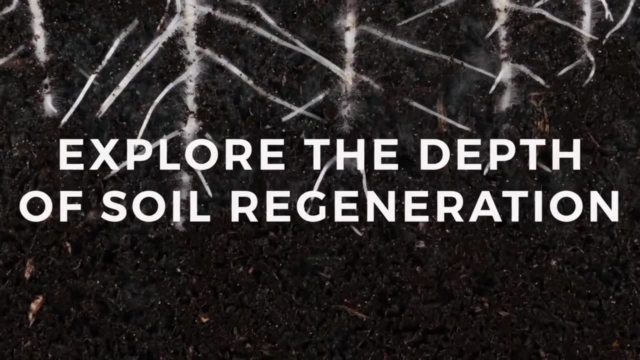 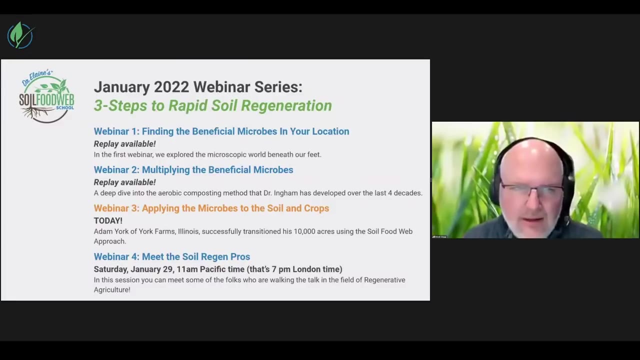 Okay, so we have four webinars in our three steps to rapid soil regeneration webinar series and today is webinar three And we've got a real special guest today. Adam York of York Family Farms is going to be talking about his work that he's done on his farm of transitioning. 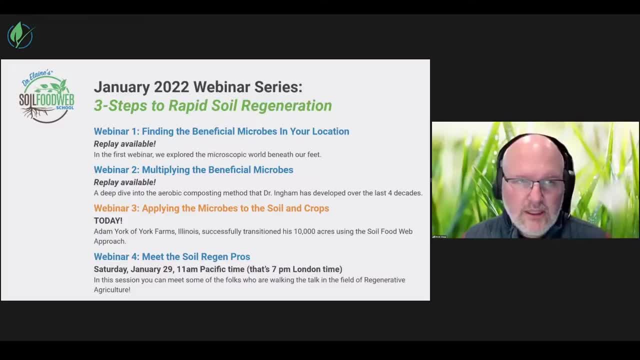 10,000 acres, plus also working on all the neighborhood farms and expanding that business. And then we have a webinar four coming up, which is going to be Meet the Soil Regen Pros, And so that's going to be this Saturday And it's going to be, you know, a number of consultants that 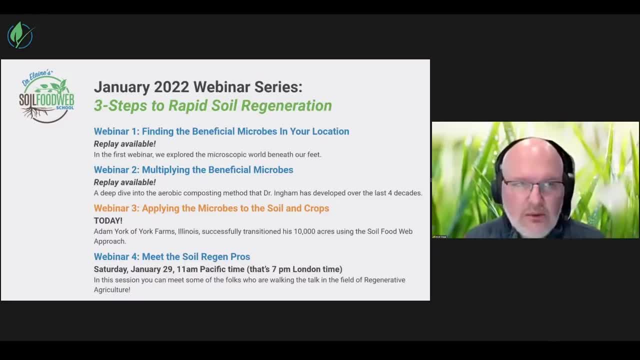 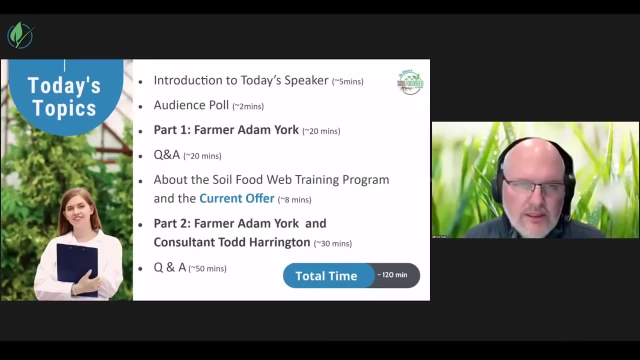 are actually out there doing the work And it's a good opportunity for you to ask questions about what we are actually doing to further the Soil Food Web approach and converting a large scale farming into the Soil Food Web. Okay, let's go ahead and continue on. So the topics for today. 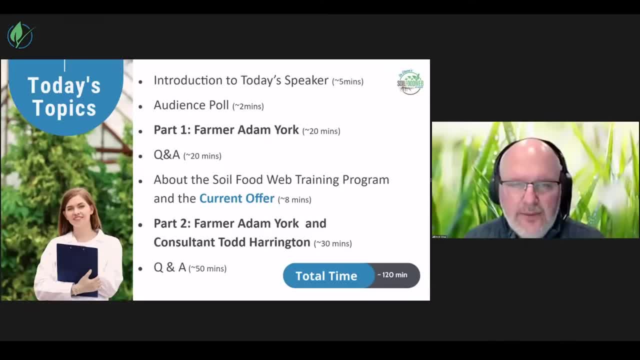 we'll just do a quick introduction with the speakers, the panelists that we have today, And then we're going to do an audience poll. We always like to hear a question for you folks to be able to answer, So we'll take 30 seconds for you to do that, And then part one of our webinar. 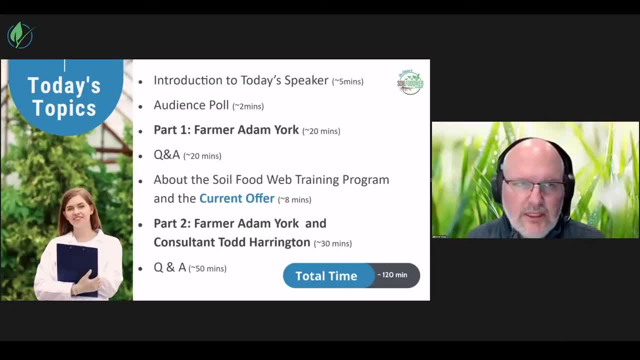 is going to be talking with farmer Adam York and the work that he's been doing And then we'll do a quick Q&A after that. So if you have questions you're going to hit the Q&A button down below And I'll have a screen and kind of describe some of the instructions for that in just a second. 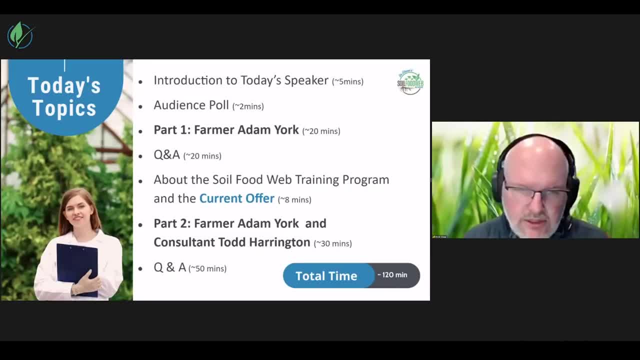 And then we'll get into the promotion that we're going on, which is the About the Soil Food Web training program and the offer that we've got. And then part two is going to be Adam York and also Todd Harrington, who Todd was working with for a while, And then part two is going to be 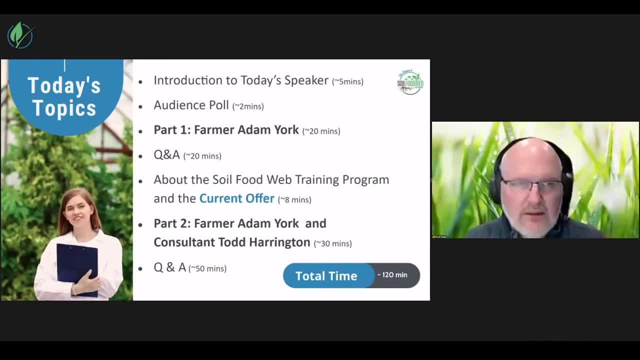 Adam York and also Todd Harrington, who, Todd, was working with Adam to make all this transition work. So they'll talk about some of the good work that they're doing And then we'll finish that with a Q&A session. And so, again, if you've got questions, go to the Q&A section And we expect 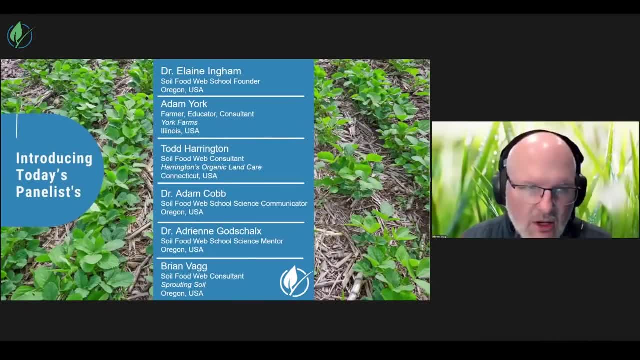 that today's webinar is going to be about 120 minutes or two hours. Okay, for the panelists today we've got Dr Lainingham. of course, Couldn't do this work without her, So this is fantastic to have Aline with us. And then, like I mentioned, Adam York, So he's got York Farms And 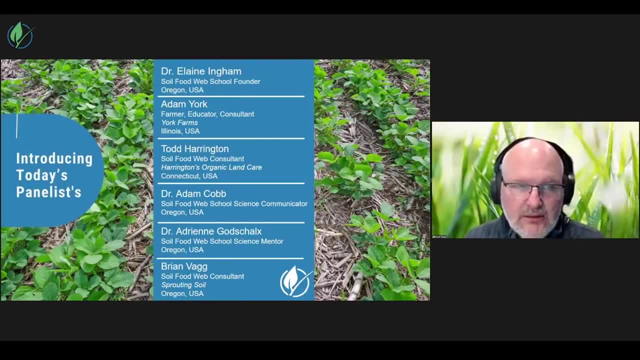 he's farming. He's also now educating other farmers about the Soil Food Web approach and consulting on those large scale farms. We've got Todd Harrington, part of Harrington's Organic Landcare. He's a Soil Food Web consultant. We've got Dr Adam Cobb, which is a Soil Food Web School. 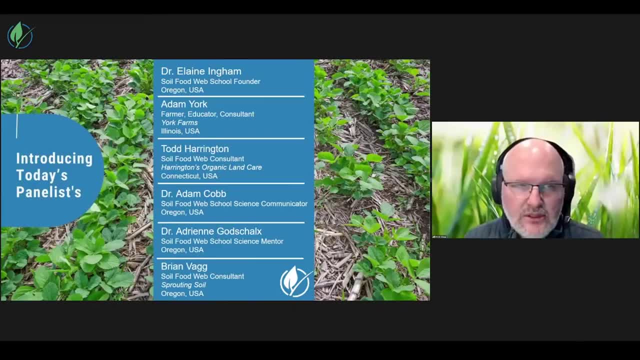 science communicator, So he's helping us do a lot of the outreach. in our Soil Food Web School We've got Dr Adrian Gottschalks, who's a Soil Food Web School science mentor, So helping train the new crop of consultants and lab practitioners that we have out there. 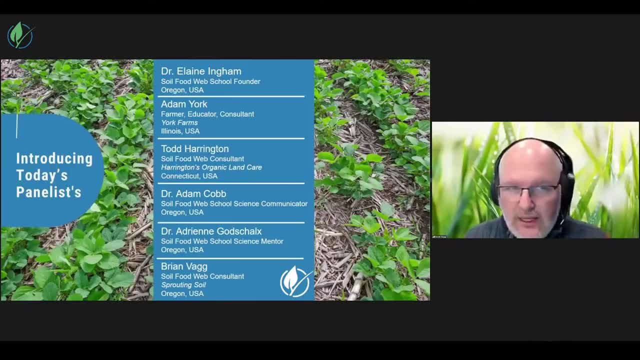 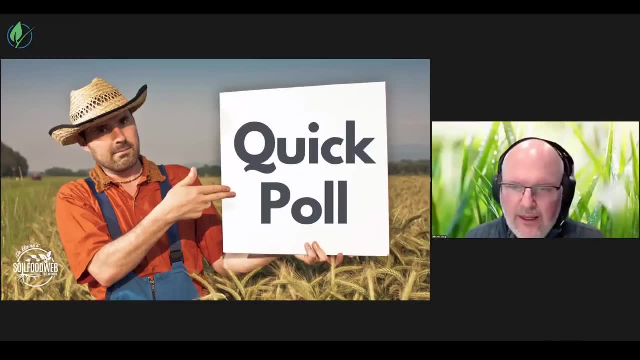 And then myself. I own a company called Surrounding Soil and I'm a Soil Food Web consultant. All right, Next slide, please. So here's a quick poll And again, we'll keep it up for a minute or two And you should see that poll launching into your screens now, All right, And we'll just go. 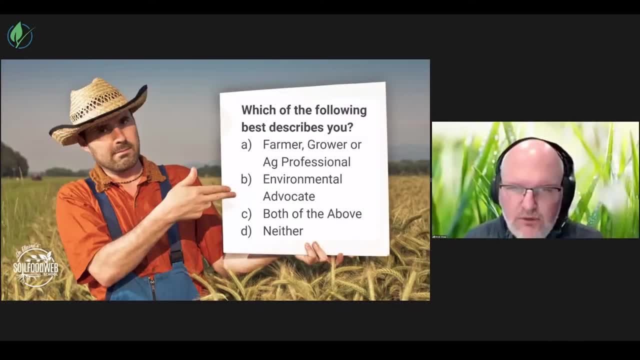 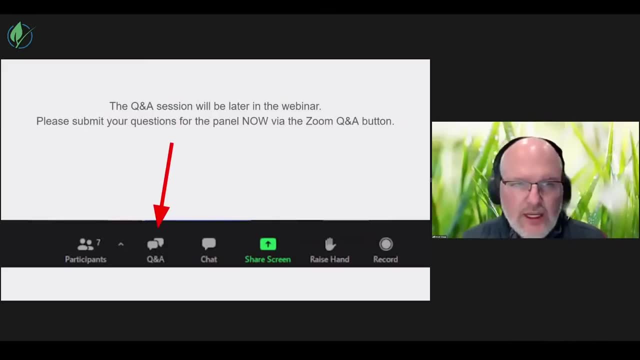 ahead and that poll will be up until you answer it in the background. So, Adrian, we can move on to the next slide, please. Okay, And I talked about Q&A, So it says, you know we like to have this dynamic feedback. We. 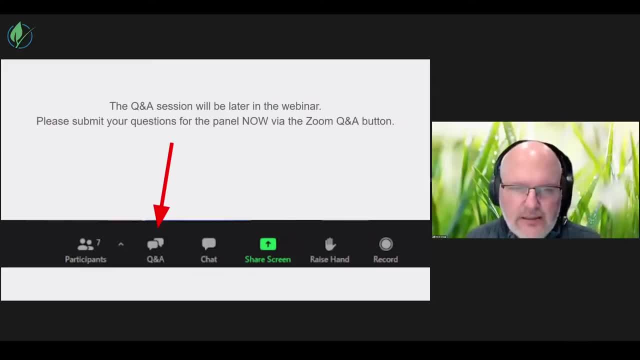 want to hear questions from you, to be able to have a discussion amongst the panelists. So at the bottom of your Zoom screen you're going to see a Q&A and your question will be recorded And then I'll be going through and selecting questions. We won't be able to answer every. 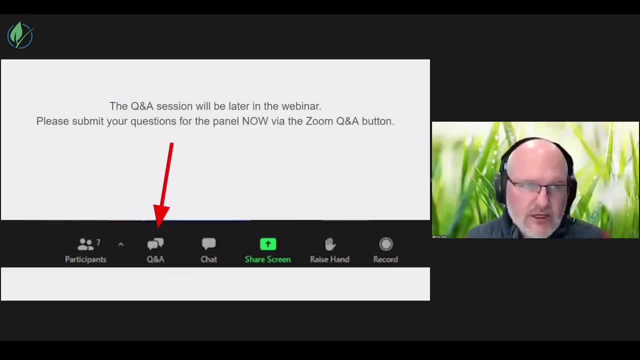 question. that's out there. but if you can, you know we will try to answer ones that are going to kind of fit for the theme for today. And please put your questions in the Q&A. If you put them in chat they may not get caught in actually to our question. So if you do have a question you want, 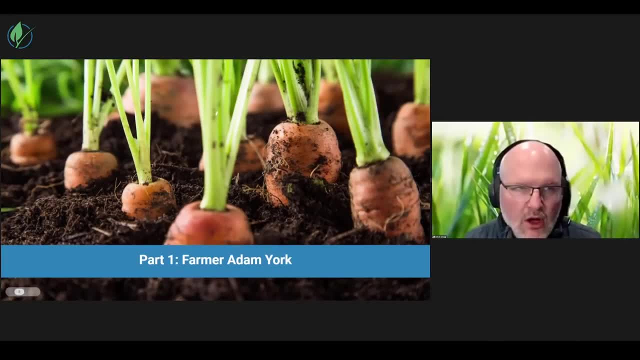 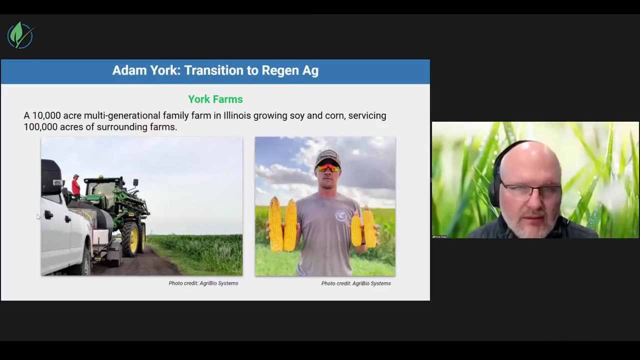 the panelists to ask: the Q&A section is the right area to go. Okay, so part one: we're going to be talking with Adam York, So, Adam, go ahead and take it away. Okay, you hear me. okay, then, Yep. 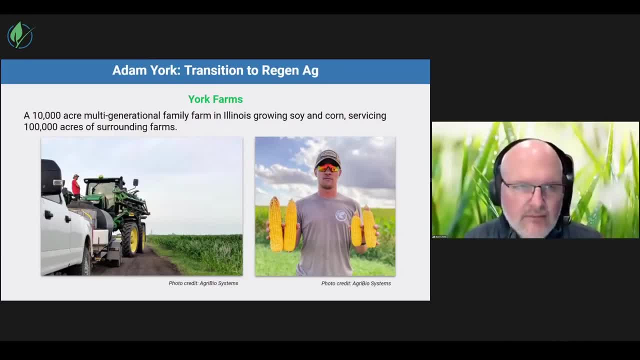 you sound great. Okay, all right. So hello everybody. my name is Adam York. I am multi-generational. we run a multi-generational family farm from Jacksonville, Illinois. I farm alongside my brother, my two cousins which are, and my uncle. 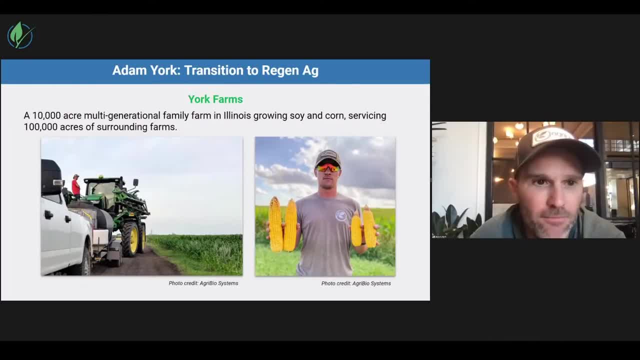 So we grow soybeans, corn and we farm ourselves a little over 10,000 acres of land. So we're a little over 10,000 acres of land. So we're a little over 10,000 acres, probably a little closer to 11,000 now And then we do help some other. 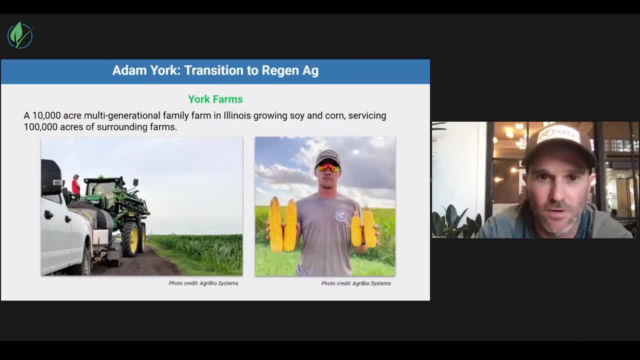 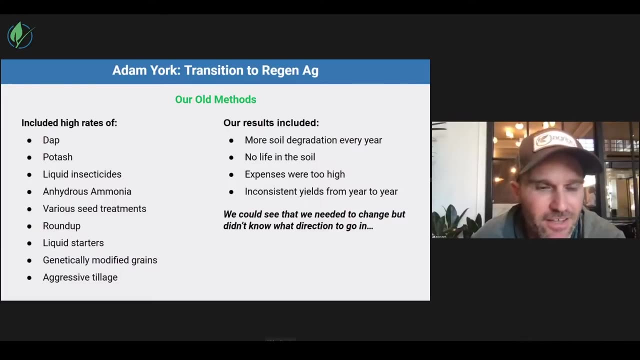 farmers locally in the area service some of their farms as well. Next slide: Okay, so part of our transition. it's been an interesting journey but we have gotten rid of. we don't use any DAP fertilizer, any potash. We do not use any liquid insecticides. 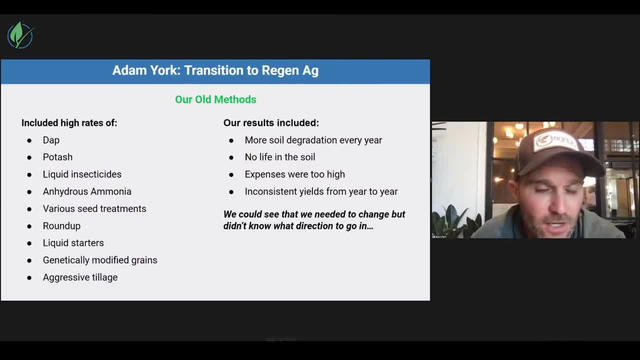 and hydrous ammonia. We don't use seed treatments on our soybeans. Some of the corn around our area is still hard to get some of the seed treatments, not without them. We do not use Roundup anymore. We use some different chemicals, more of a non-GMO type chemicals. We've gotten away from liquid. 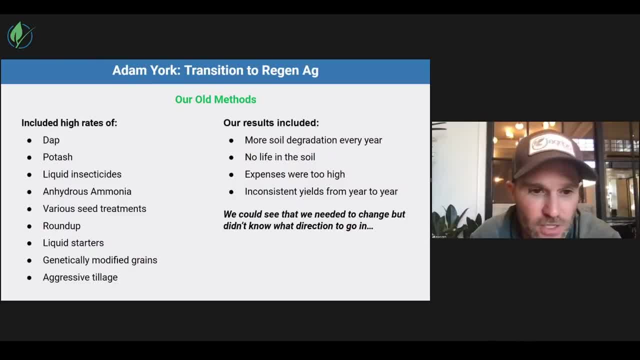 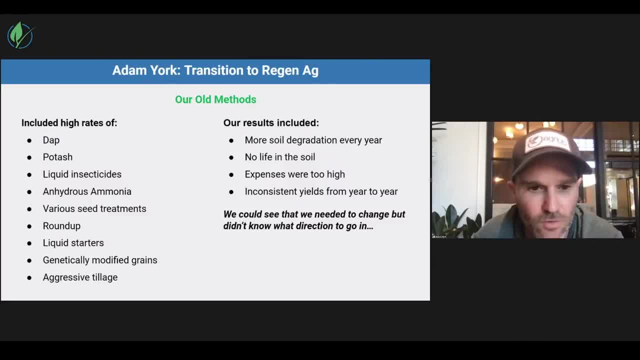 probably about 95% over to non-GMO. I would switch it all. The problem is with some of the dicamba around. some of our fields are bordering some of our neighbors too closely and they do seem to smoke some of our stuff. 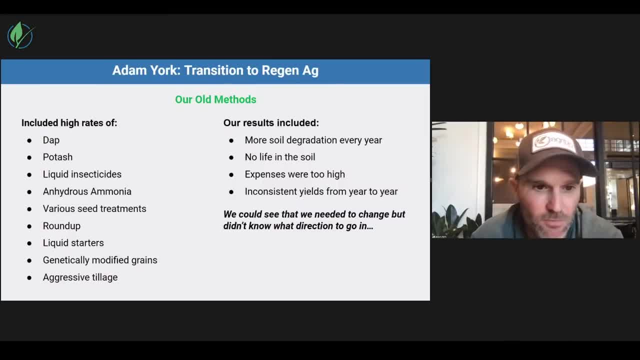 And we've gotten away from aggressive tillage. I do believe tillage is important if you do need it. If you don't, you know that's one thing that you know depends on the soil, but we have went to more of a vertical tillage type tillage system to plant cover crops And if you do need. 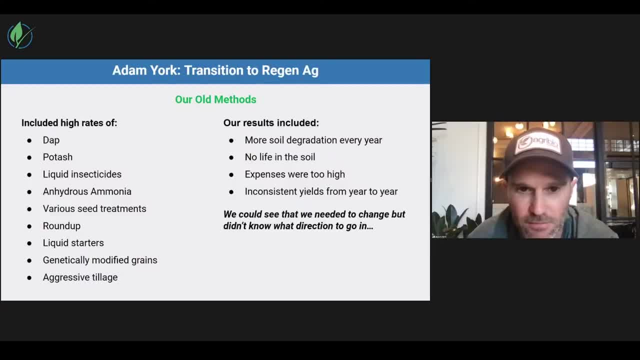 some sort of tillage, we went more towards a inline ripper. But here in the last couple of years we have not really done any tillage whatsoever other than a little bit of vertical tillage. So a lot of our results. we have noticed that when we first started this journey. 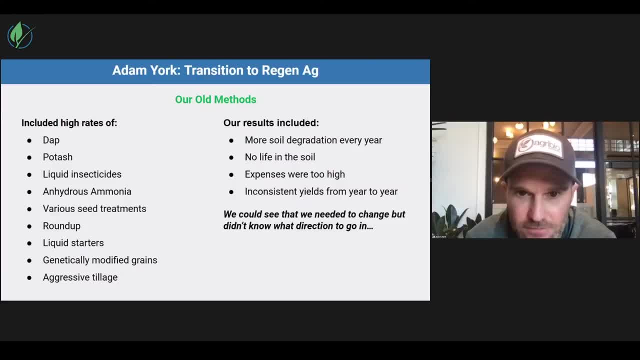 our soils were very degraded. It more or less. it's pretty easy to see. So we're seeing a lot of improvement there. You know I couldn't find a earthworm to save our lives. We were spending way too much money on. 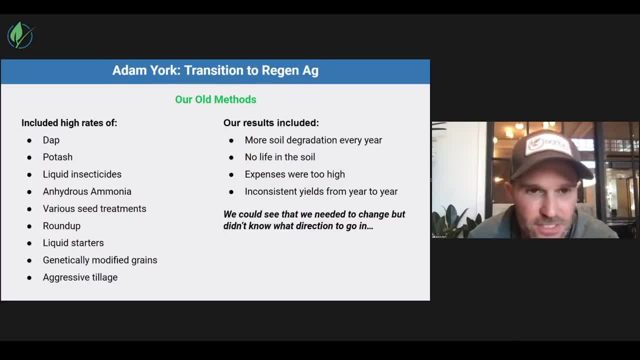 fertilizer And just the inconsistency was was um from year to year was just not there for us and, like i said, we could, we knew we needed to change, but didn't know what direction to go in. and this is kind of how the how the journey started. 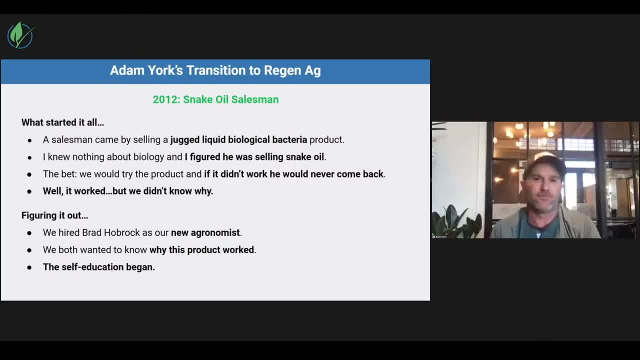 great, uh, next slide, yep, okay. so this is kind of where it gets kind of fun. but, uh and so in 2012 i had a good friend of mine. he actually used to be a- uh, a seed salesman and i've known him for a long time and and he was kind of going down a little different route- um, i never did buy seed. 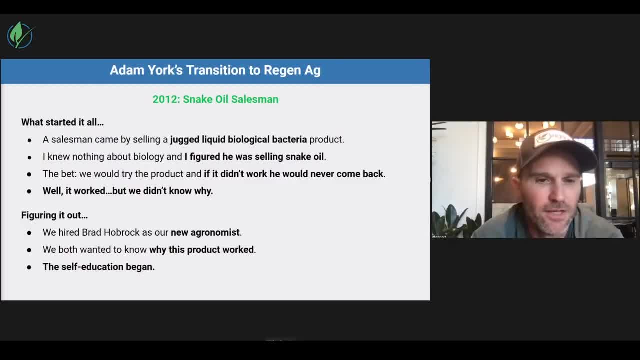 from him before, but i knew who he was and uh, anyways, he came by the farm and and was trying to sell a uh got a jug liquid biological product and, you know, i didn't know, i didn't know a thing about biology at this point in time, and, uh, you know, i think a lot of farmers are trying to sell. 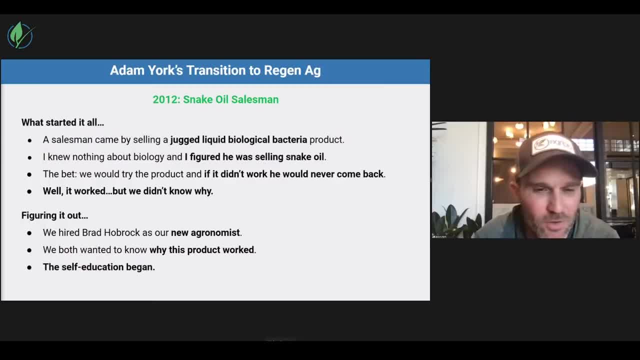 uh, you know a lot of farmers out there know you know what a lot of these salesmen- especially they come out of the woodwork, especially when, when prices are high or whatever, trying to sell, sell you anything and everything under the sun and uh, pretty much said, yeah, you're, you're selling snake. 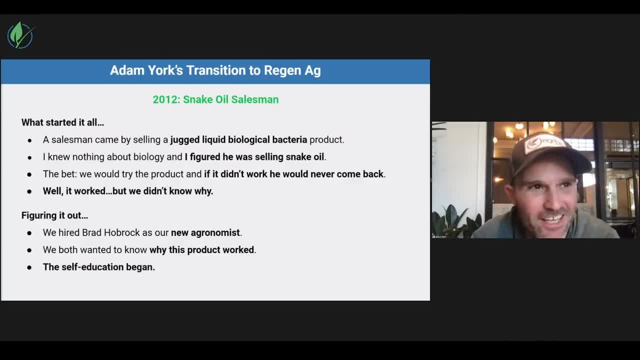 oil and um. we took a bet and um, and more or less he's like: all right guys, if it doesn't work, i'm never, ever going to come back to your farm. it's like deal, one less salesman. we got to deal with um, so we tried it, you know, tried on some small stuff. that was actually a drought year for us. 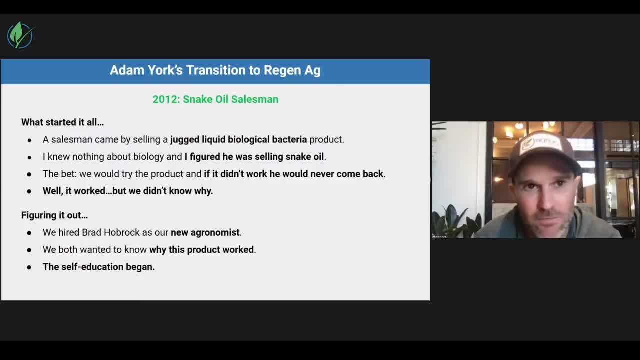 but uh, we do have some irrigation and uh, even where it was drought prone versus under irrigation, um, these trials paid um. you know we had cut the fertilizer there um and did some with no fertilizer, or, you know, cut rates of fertilizer and um, these, these trials paid um. but, like i said, we 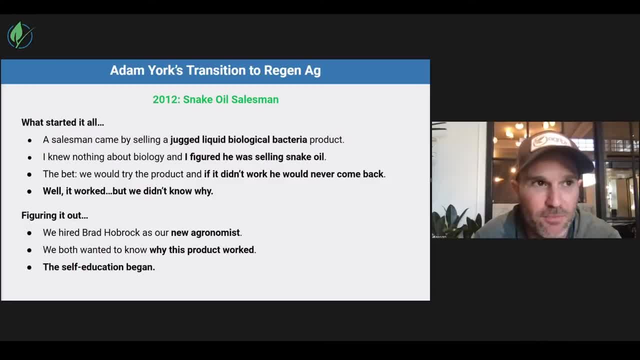 didn't know why, and that is pretty much you know. it boggled mine, my mind and um, i just had to figure it out. so, so at that point in time we were working with agronomists, um, and we were doing i mean, uh, i don't even know, 300 pounds of dap, in some places, up to 400 pounds of pot, i mean. 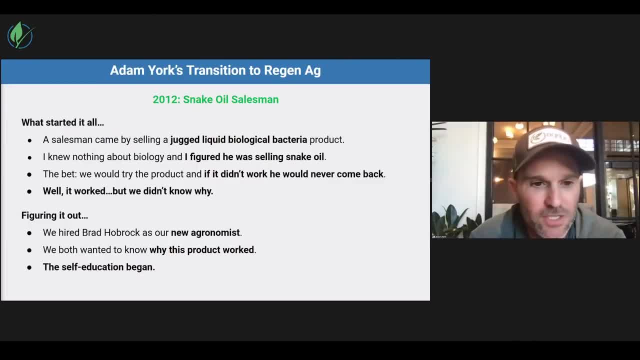 it was. we were, we were throwing a lot of money away. so i hired brad holbrock, which um was agronomist. he worked for a seed company. i've known him for a long time, um, probably since like 2001. i have known him um and he kind of had the same goals as what, well, what i had. so, uh, we. 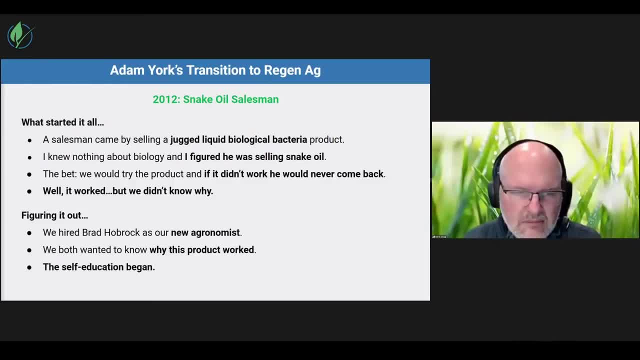 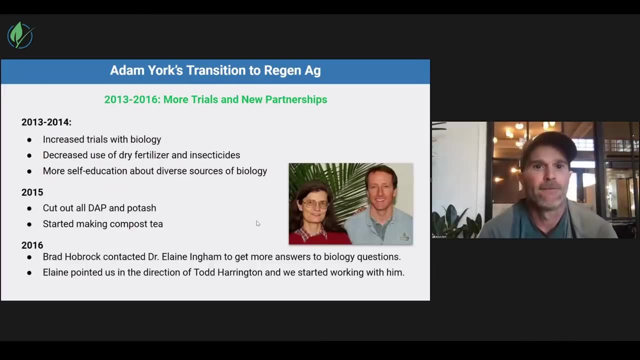 started working together. i think he actually went on his own when i we hired him as an agronomist in 2000, in 2012.. but, um, we wanted to know why, and this is pretty much where our self-education began, so let's see here. so fast forward a little bit, or 2013-14, we did more trials. okay, we were still. 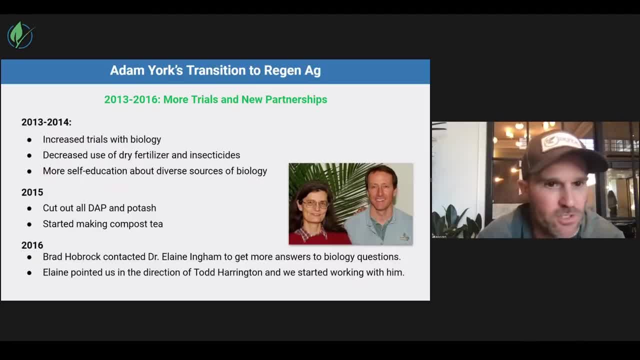 working with this same company. um, we were doing food sources with the biology. um, we continued to decrease the use of dry fertilizers. that was one of the main things. when brad came on. we, we were variable rating, we were, we were doing a few things, but we were not throwing the type of money that we 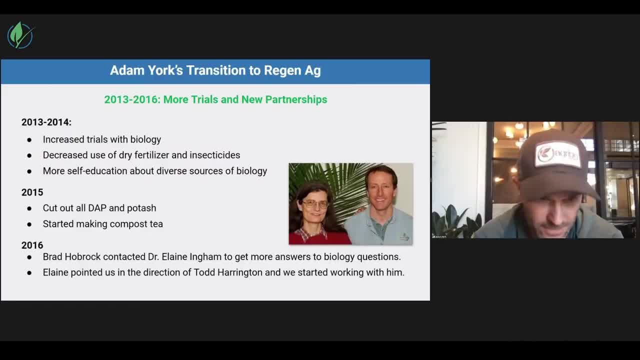 were in 2012.. um, and, like i said, we started educating ourselves, and that's the thing about. i think to this day, it's still very, very important to do that- surround yourself with good people. but, um, and in 2015, we cut out all fertilizer, daft potash. um, and then we started making compost tea. 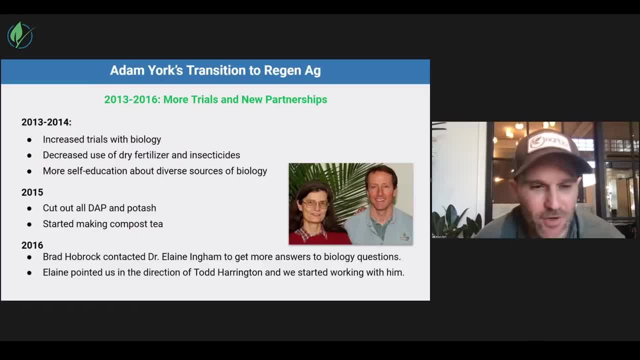 we- uh, todd says we weren't making very good compost tea then, but it still was working, that's. i think that just tells you how degraded our soils were. that even the stuff that we were making- even though todd says it wasn't very good, it still was showing some benefit. um, and then 2016: my partner in agrobio systems. now. 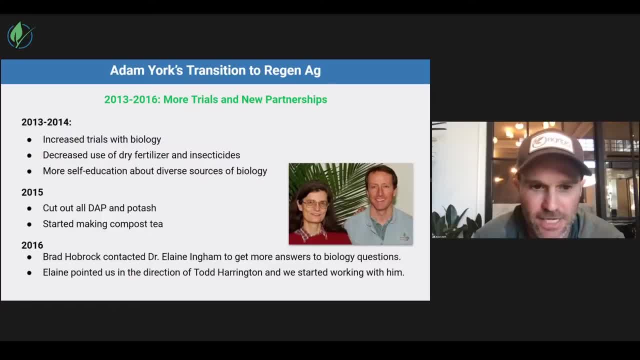 um in my grounds. at the time, brad contacted dr elaine ingham because we just had some answers that we um needed answered and we didn't know who else to call except for um miss elaine. so she pointed us in the direction of todd harrington, and that is about the time that we all started. 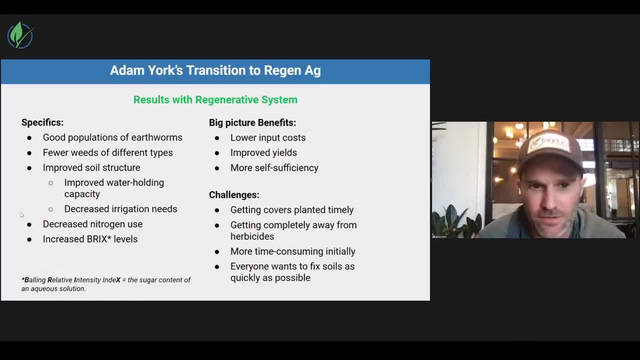 working together with todd todd, started helping us with, you know, improving our extracts, teas, making our own vermicompost and yadda yadda, yadda. so, um, okay, so so part of our transition to region add so what we've actually been seeing um on our farm today versus back when, before we started this. 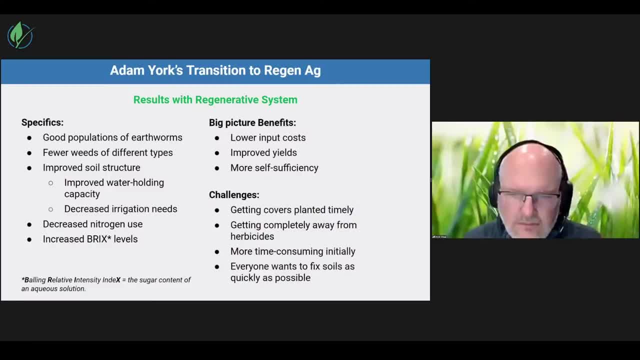 we are getting a very healthy population of earthworms in our soil. More aggregate structure: You know, when we first started this, we had no aggregate structure or any earthworms whatsoever. We were fighting waterhemp- a lot of other horrible weeds around our area that farmers 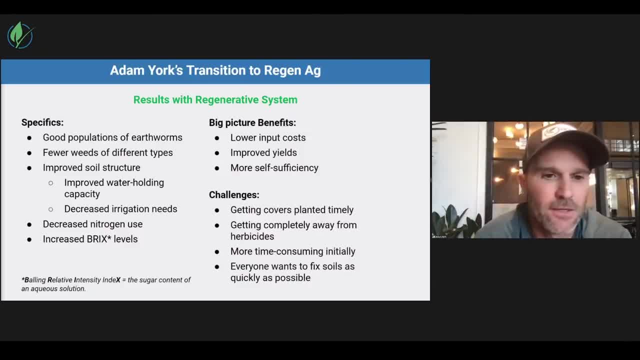 still around this area that are still in the conventional methods are still fighting. We've improved our soil structure. We've gotten rid of some- we've had some some soil compaction layers due to high magnesium levels- that we have improved those switches and in turn proved our water holding capacity. 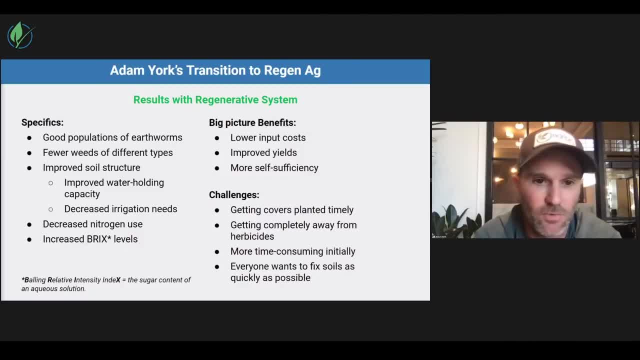 We do farm in the Illinois river bottoms, where we do have some irrigation, where we have some sands, some gumbos, a lot of different types of soil. We have decreased a lot of our irrigation needs, which is Very time consuming sometimes. 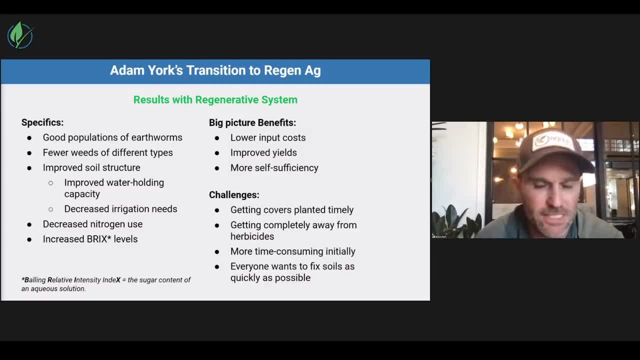 And we've also backed off our nitrogen use by probably about 60 to a hundred pounds, depending on the soil, depending on the situation, And then also we have increased our BRF levels in our plants. So, like I said here, big picture benefits is lower input costs, which is you know. 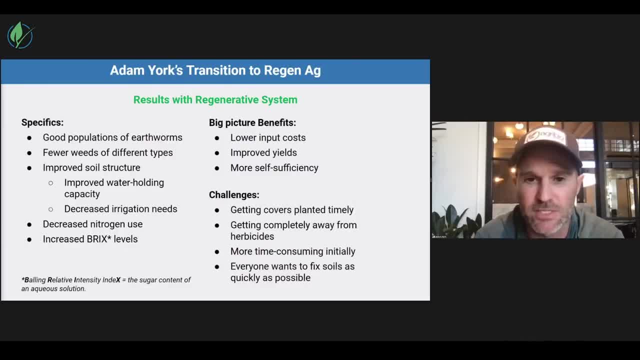 especially in today's world, guys, where fertilizer is really, really expensive. It's a big deal. Even when we all thought that they were somewhat affordable, it was still a big deal. Yields have improved and we are more so self-sufficient as a farm compared to a lot of other farms. 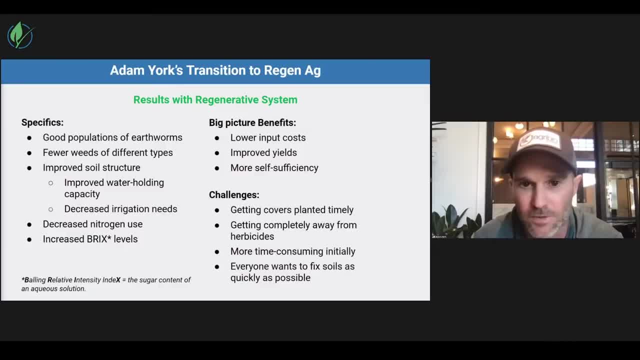 that are very dependent on you. know what, what the next guy's going to try to sell them. So challenges, this is this is always fun, So you know, no matter when you any type of change that you're planning on making. 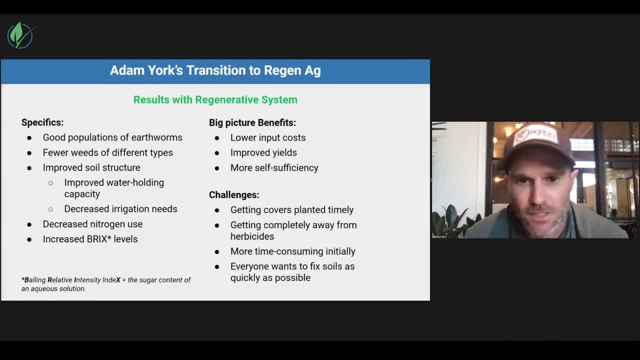 you are going to occur some challenges. Um, we have a hard time sometimes, depending on how harvest goes, depending on what rainfall is, getting some covers, uh, planted timely- We've had some, uh, where we planted some, some corn and some covers- we've had some. 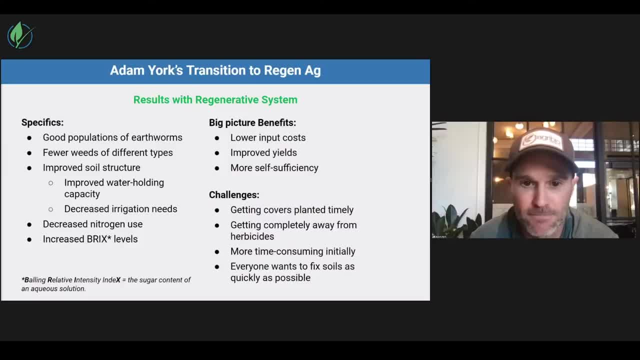 some tough uh learning curves there. Um, we've cut back on herbicides. You know, one of the main things is we've gotten away from a Roundup, but we have- uh, we have not still completely gotten away from it. 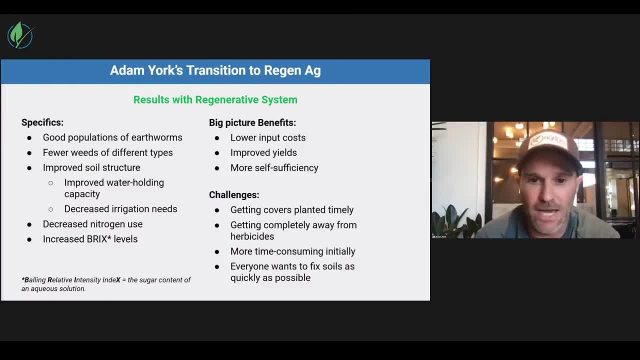 I would love to, But we are working on cutting- Okay, Cutting them back um, and we have been doing so um, and probably I think you know at first, you know it's not. you know, maybe going to this method for us was not pushing. 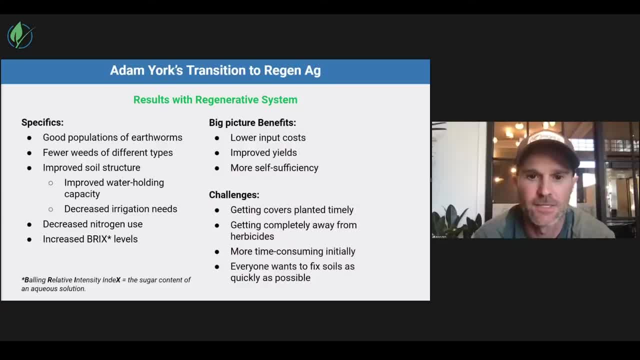 the easy button. um, like some, conventional farming is um, so maybe initially it's a little more time consuming, but I think, over, over time, I think it's going to be um, I think you're actually going to have more time. 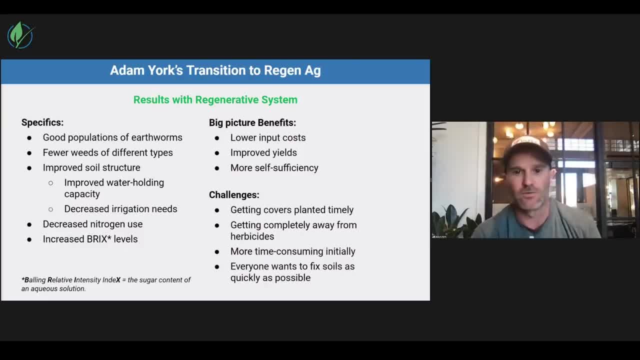 Um, and another challenge is everybody wants to fix it. They want to make soils, you know, obviously as quickly as possible and that, depending on everybody's situation, is a little bit different, and that is is challenging. Uh, we have a saying that pretty much we say we didn't screw these soils up in one year. 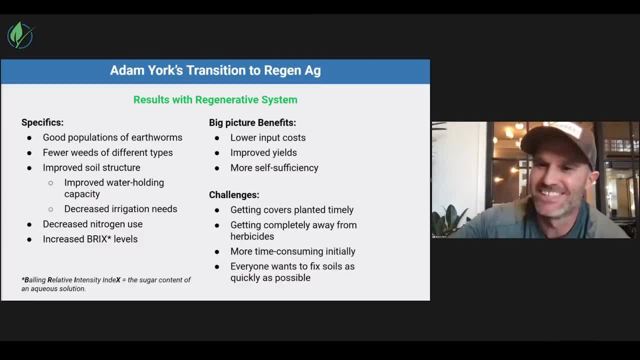 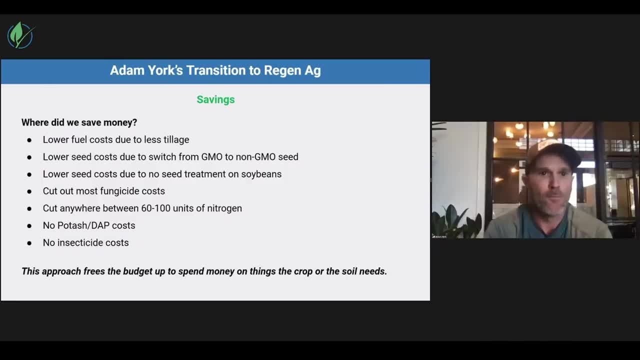 We're not going to fix them in one year, So it's going to take a little bit of time, but you're on the right path. Okay, All right. Where did we save money? So when we first started this, you know it was. 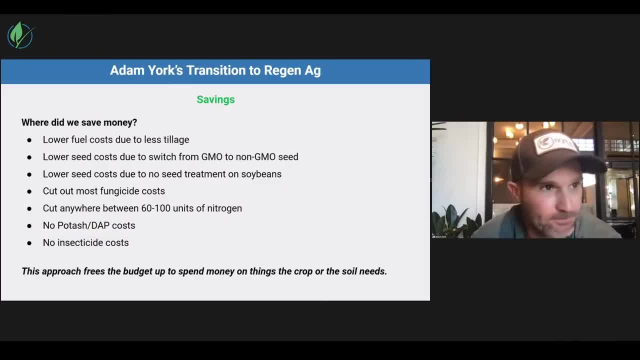 So we talk about budget cuts. it depends on what you do with that money, Right? Um? so we were probably saving right at the gate, probably anywhere between a hundred to $150 per acre. Some of that cost is obviously less tillage, um, lower on your fuel costs. 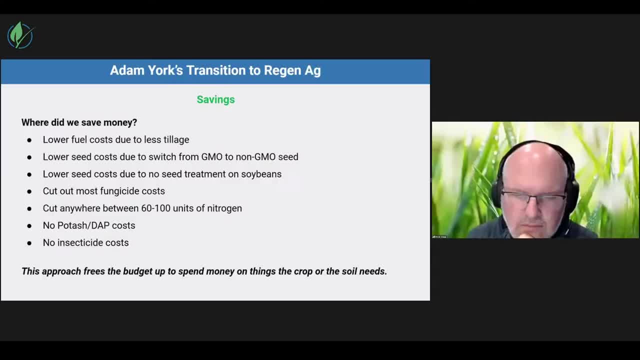 Um, a big one, a real big one, And a lot of guys know is going from a GMO to non GMO seed. Uh, GMO seed. Um, I know a bag of corn for us. if you want to, you know, get it all at. uh, you know. 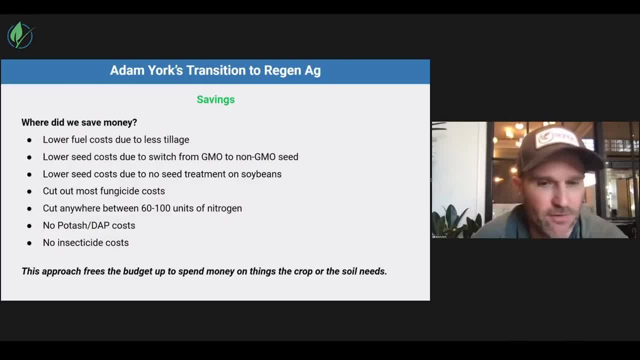 the big GMO seeds. it's going to be 320, $350 a bag where you can get a non GMO bag of corn for, you know, 150 to 170, depending on your area. you know that's a that's a big difference. 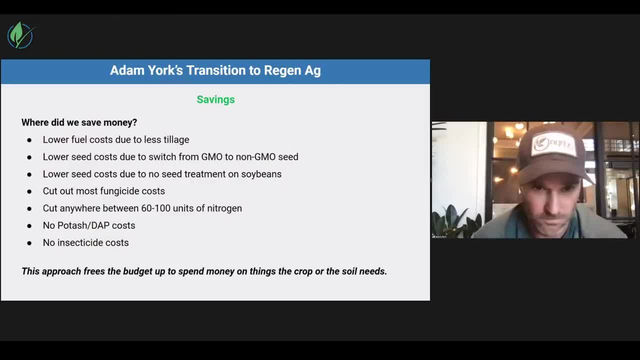 Um so, and we also, we've cut out all seed treatment. There's a lot of- uh, people that are making a lot of money and and spend a lot of money- Yeah, A lot of money- on seed treatments. 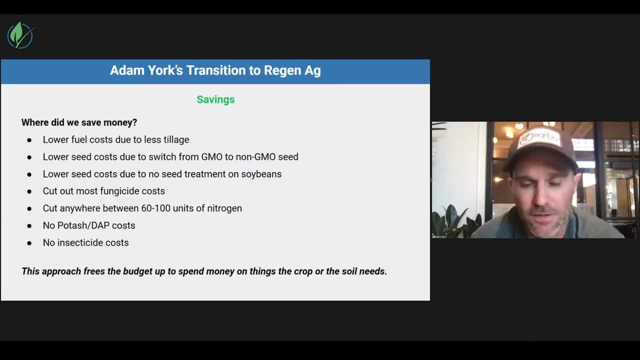 There's some people that are spending all the way up to 30 to $40 on a bag of beans, where normally a bag of beans costs you 30 to $40,. you know um, we've cut out majority of our fungicide costs. 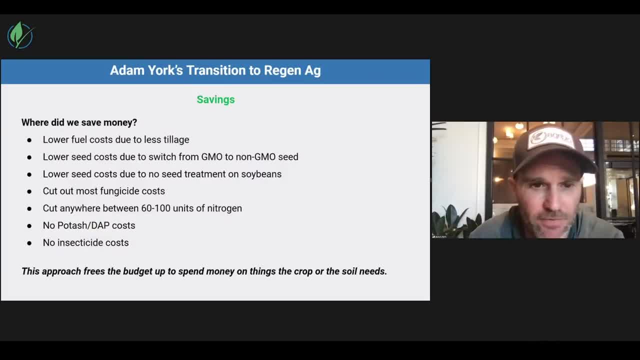 You know, I think, uh, as long as you're keeping your bricks levels up and you're doing some of the right things and mother nature's cooperating with you, she hasn't for us for the last couple of years. it's been a little tough on that side, but, um, that is another cost that you 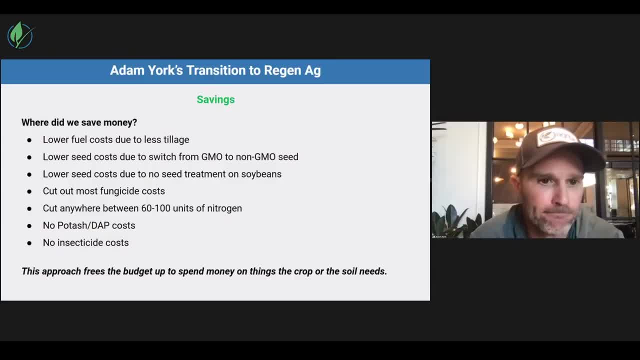 can cut out, if you can, Um, And you can also, like I talked earlier, you can cut out between six, or we cut out between 60 and a hundred units of nitrogen And we're still at that point in time where we're at. 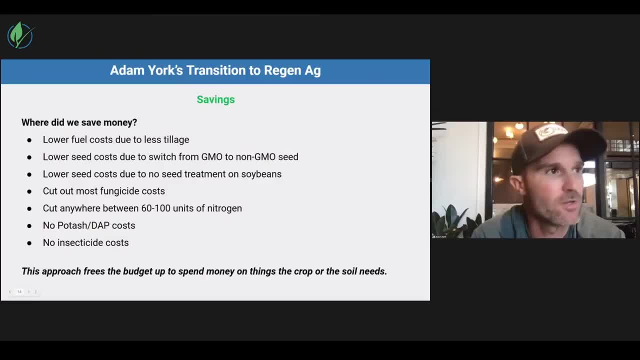 I mean, my goal is still to try to, you know, produce um 250 to 300 bushels of corn And you know, at this point in time we're doing it right now at you know somewhere. 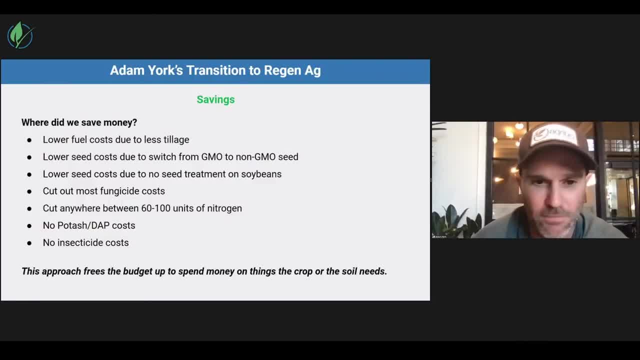 around that, between a hundred and 140 pounds, 150 pounds of nitrogen um, depending on the soil. So we have no potash or DAP costs Um. we do not use any dry fertilizer and then we do not use any insecticide. 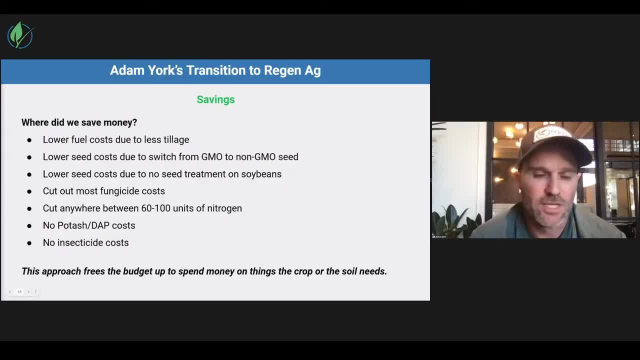 We've cut all those out. So this approach pretty much frees up the budget to spend um money on things that the crop and the soil needs, whether that's biology, you know um, or other fertilizers, you know, maybe like a boron, or or, uh uh, molybdenum, you know certain things like. 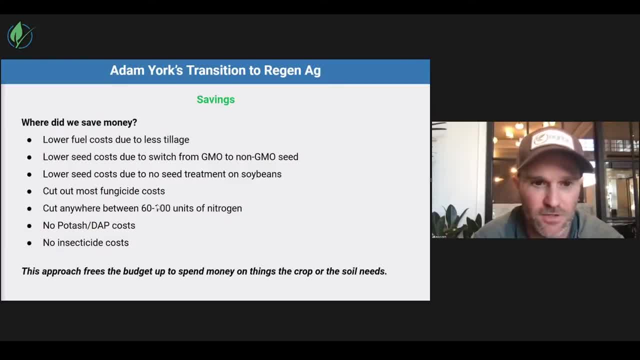 that Um and we, we decide a lot of that versus on um. we do a lot of sap testing, so that's how we kind of come up with um. you know what other nutrients are we missing as well? 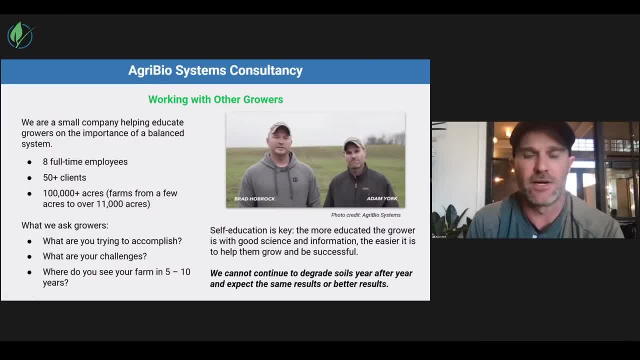 So the the creation of agribiosystems has been kind of an interesting one. So when Brad and I started going down this road, we had really no ambitions to start a company, Um, But the reason why we did start agribiosystems was because we we were doing this on our 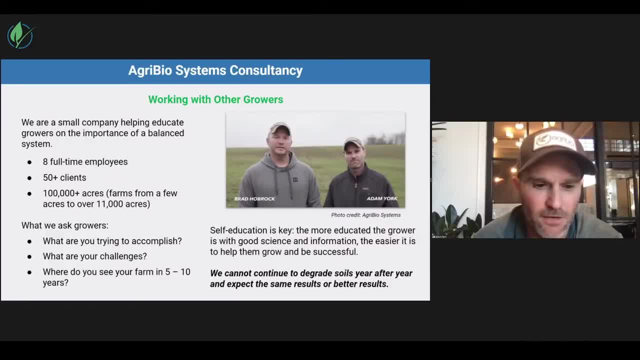 own farms and it kind of sparked the interest of, uh, a few other farmers around our area. Um, they're like, Hey, you know that that sounds like something that we'd be interested in. So so we ended up, uh, going out on a limb and and saying, all right, if, if, if there's. 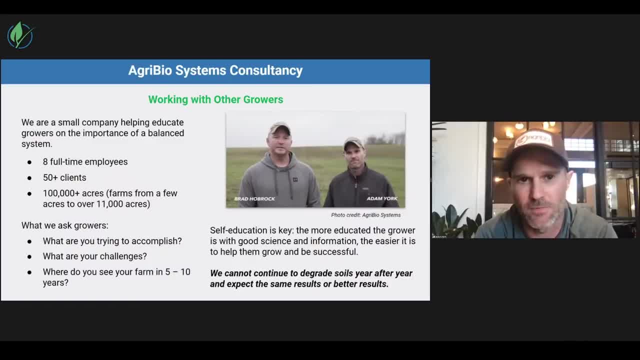 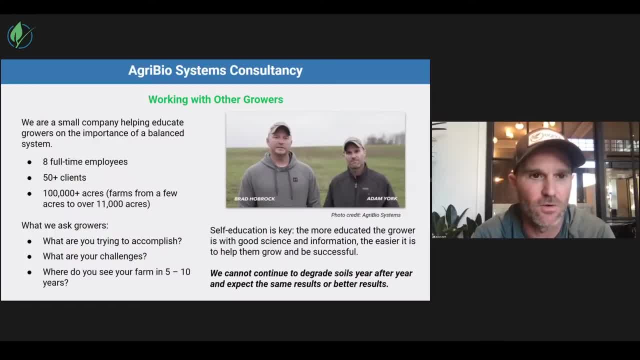 and and kind of learn this deal together. So, um, so at this point in time we do have eight full-time employees, you know 50, some clients, um, probably a little bit more than that. Um, you know, some are more locally summer, summer, scattered across United States. 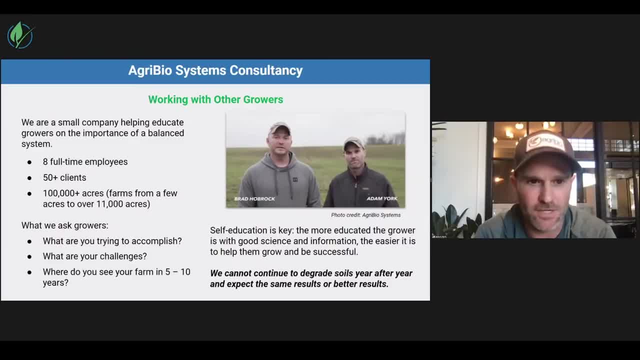 Um, and yeah, we probably work on a hundred thousand acres or so, um, give or take, uh, farms, you know that are all the way up to 11,000 acres, to farms that are 8 000 to 9 000 farms. that are, you know, five to ten, you know. so, um, but one of 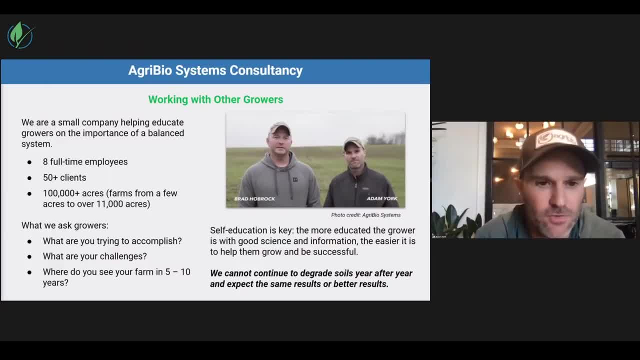 the things that we do at agri-bio systems is we do tell, try to help educate growers um, and the main reason is because, um, we're not trying to tell guys you know what to do or you know, but if we can help educate guys on um why certain things that maybe we promote are important, it. 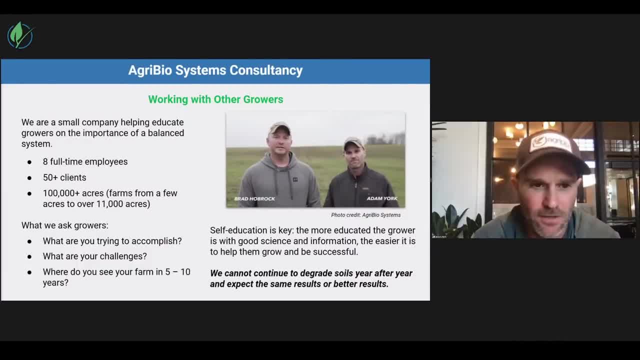 does? it does help make that transition a little bit easier. um, and you know i said a couple of things. we like to ask them is: you know what? what are your goals? what do you? what are you trying to accomplish? um, you know there's a lot of farmers around home. sometimes they're just trying to get. 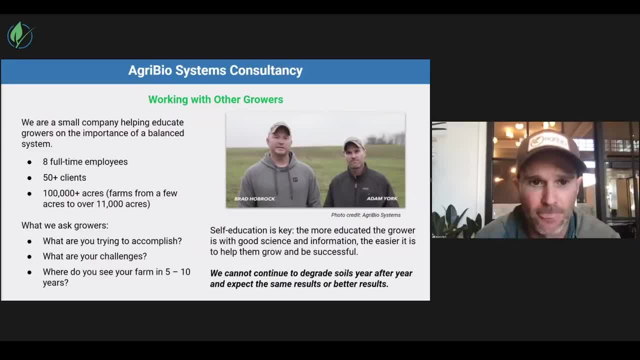 from one year to the next year. you know, um, you know for me, i have, i have three boys. my brother has four boys. um, this is about trying to leave. you know, for me it's about trying to leave this soil when i found it. um, so these guys, so my children, don't have to go through, possibly some of the 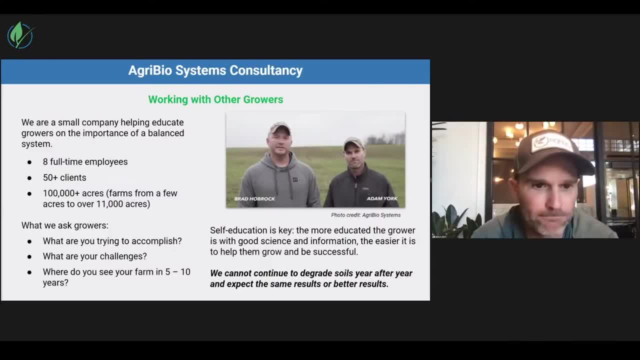 the challenges that that i've had to, um, and we ask growers what are their challenges. you know, um, everybody, everybody in agriculture has has certain things that, um, uh, that are challenges and they're tough, you know, and and uh, you know, i'm a farmer, i understand it. 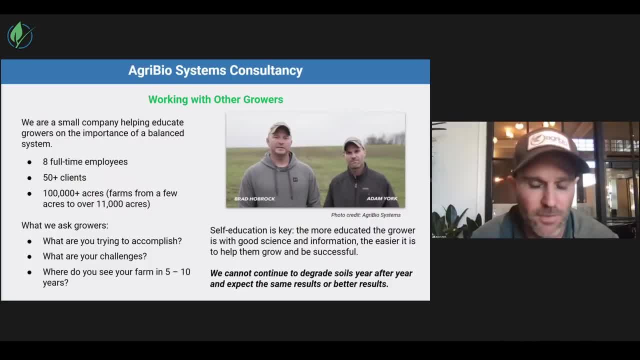 you know. so it's something that we kind of help, you know, kind of help guys try to work on some of their uh challenges. um, another thing: yeah, we're, you know, trying to trying to put a uh vision in front of some of our growers. just uh, where do you want to be in five to ten years? um? 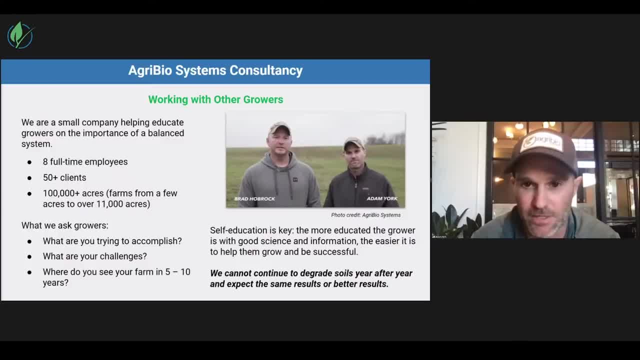 and how you gonna get there, you know, and that's kind of where we come in and try to help help that. so, um, self-education is key. the more educated the grower is, with good science and information, the easier it is to help them grow and be successful. um, we can't continue to grow. 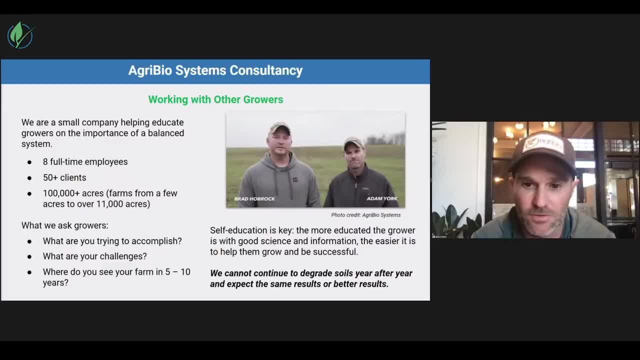 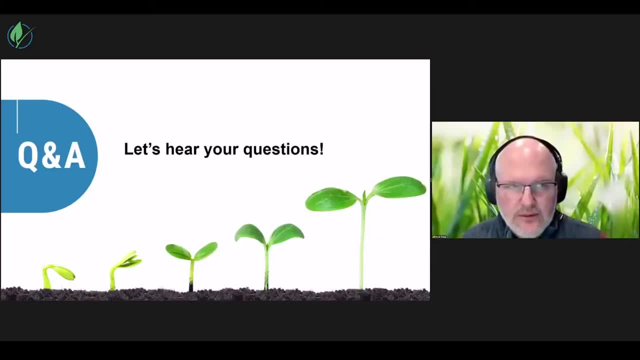 and degrade soils year after year and expect the same results, or better results from year to year. so, adam, this slide really resonates with me, because that's one of the challenges of being a consultant. out in the field is um the education part of it. you know there's a lot of people who 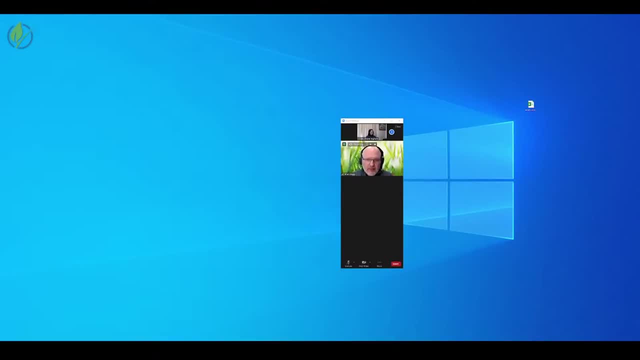 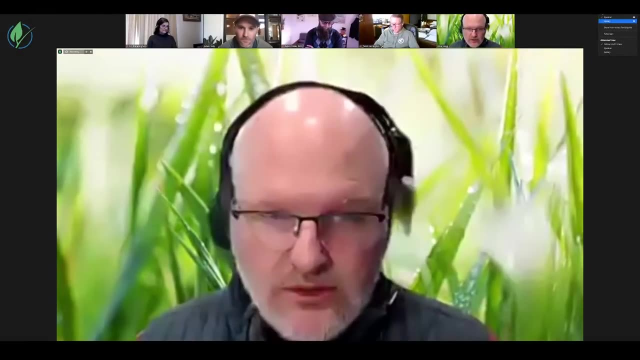 are kind of hearing through the zeitgeist. you know, hey, farming with biology the soulful approach, but and be able to really internalize that and change that to their operation. the educational hurdles- one of the things we first got to tackle, so i'm glad to be able to talk to you about that as well. 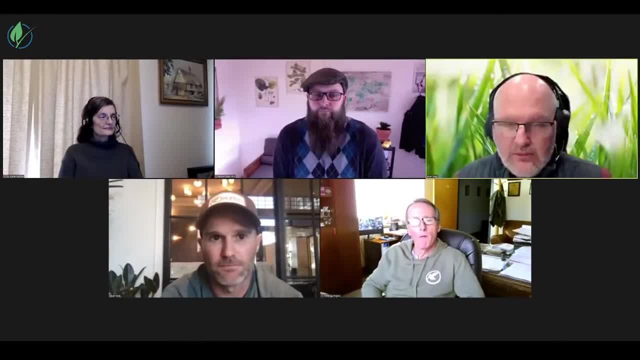 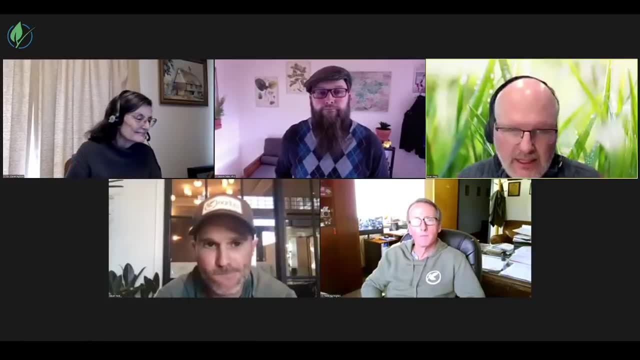 and i'm glad to be able to talk about that as well, and so you know i really appreciate that. yeah, i would just say thank you. it's been a great opportunity to to hear from you, um to see, uh, if there's anything else you want to add to that for our um, to see if we could. 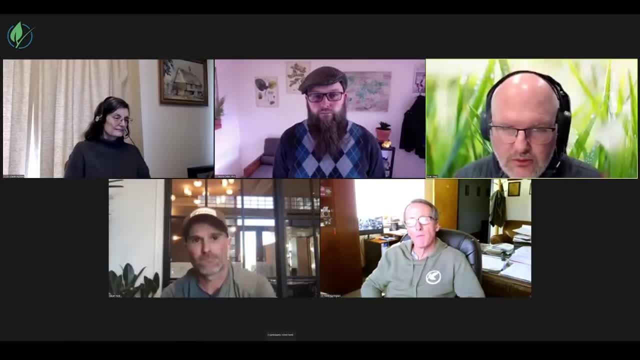 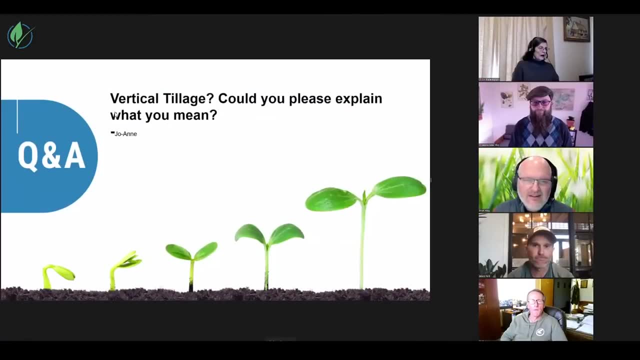 use that to our advantage with that as well, or in your uh questions. i'd love to see more of those um questions and then, uh, you know, uh, terminate that all right, and i'll see you guys next week and see if there's anything else that can be done over the coming weeks as well. okay, thanks. 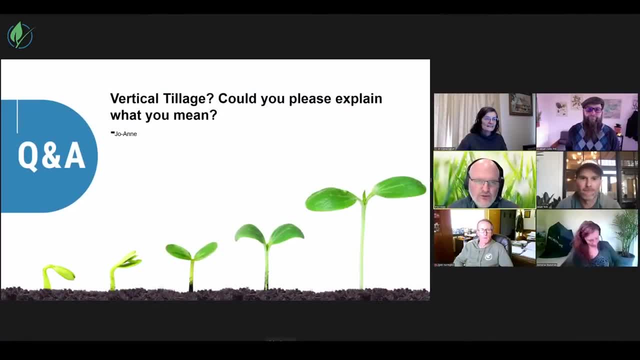 thanks, dr frederick. i's just like. i've seen you guys on youtube and stuff, so your questions are there. you're all over the world with me. so, yeah, i'm day, um, so thank you all for your time and uh, and i'll see you guys next week. we're going to see you guys next week for our next week and then we're going to see. 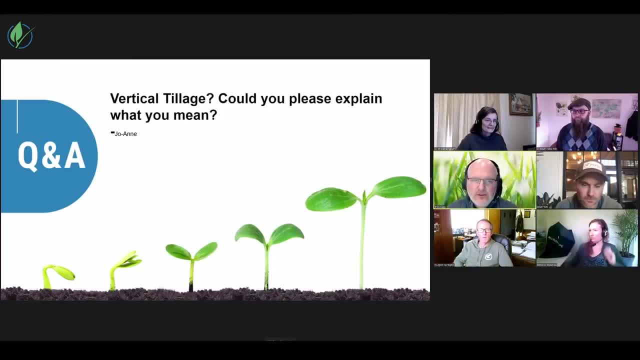 You mentioned vertical tillage. Could you explain what you mean by that? That's a question from Joanne. Yeah, so for us we use a – it's a Krauss Accelerator 8005.. I do believe is the number on it. 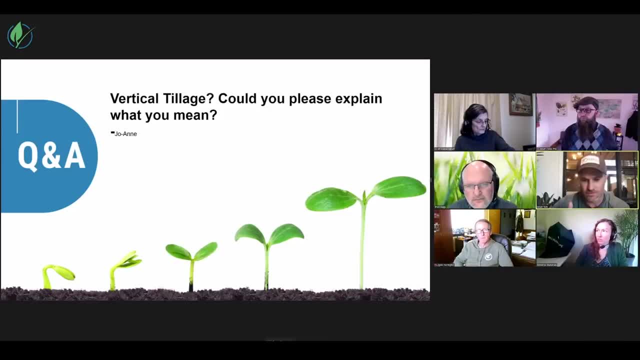 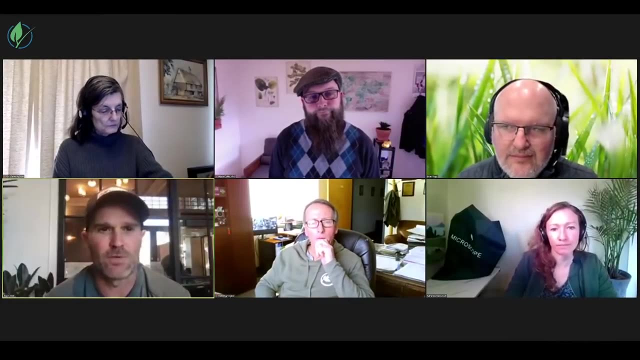 And more or less it's got some notched blades that are going straight. They're not the cup like the old discs, It's a notched curve – not curve, but they're notched straight blades and they just kind of – they're only tilling the soil about an inch and a half, two inches. 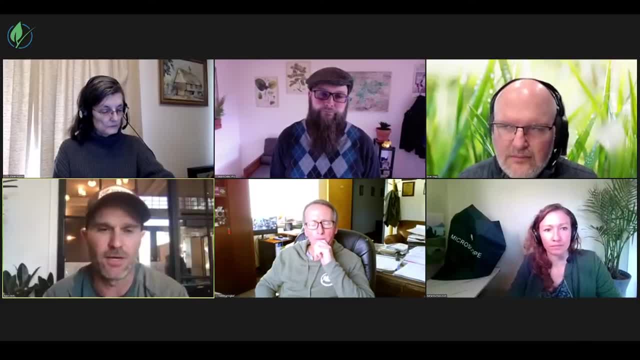 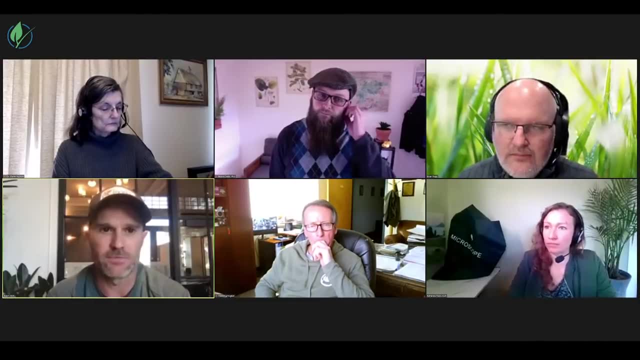 You can set it depending on what you're trying to accomplish. But on our accelerator we have a seeding unit on that as well and that's how we seed our cover crops is with that just to kind of help incorporate them in the top inch to two inches of the soil. 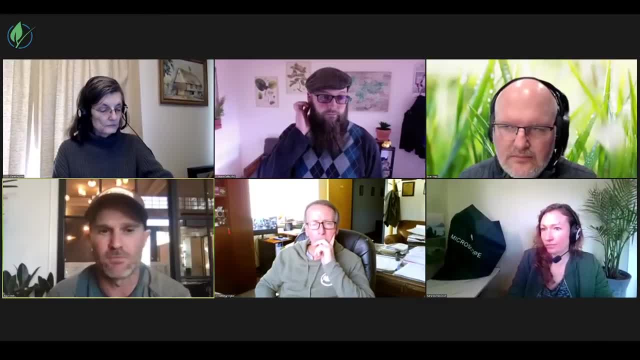 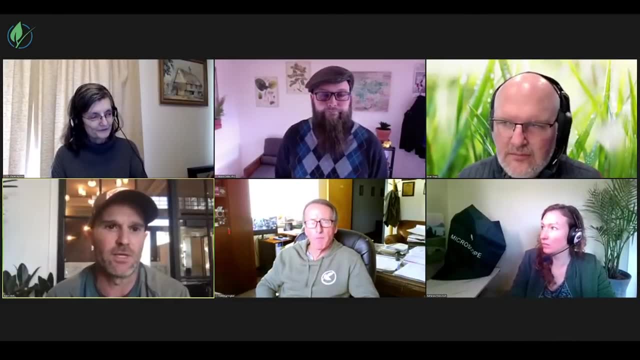 It's what works for us. You know, there's people that do some no-till, and it's been successful with that as well. This is what's worked for us, But that's – That's the piece of equipment that we use currently. 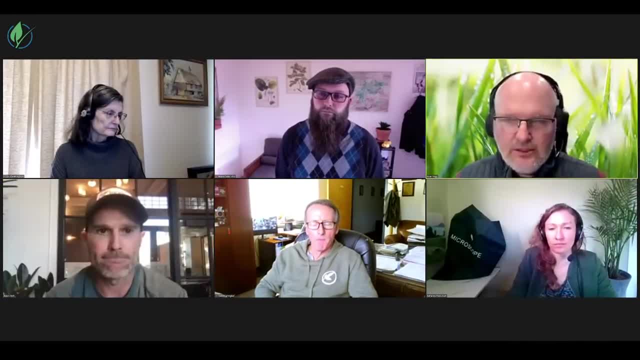 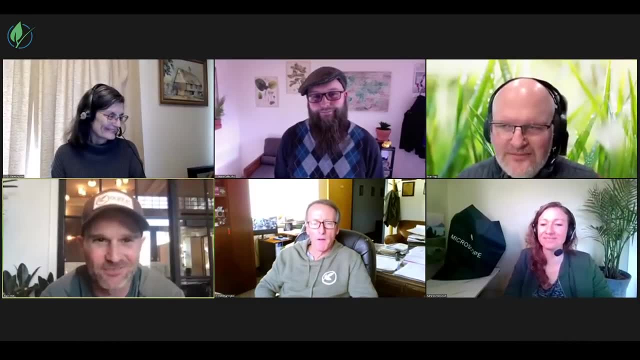 And would you say that it minimizes the amount of disturbance in the soil compared to other tilling techniques that you've used in the past? Correct, A lot less disturbance for sure, Right, Yeah, And that's all we're trying to – you know we're trying to – 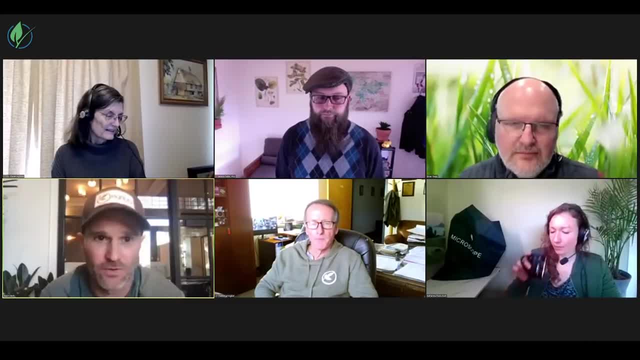 if we're trying to build aggregate structure, we don't want to tear it down. You know, it's kind of like building a house, So we're – I don't want to have to build a house every year, I don't want to tear it down every year. 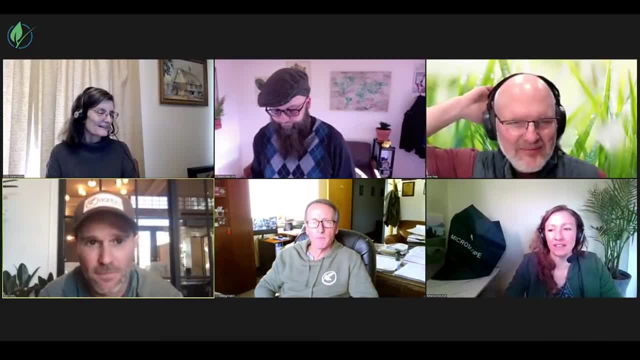 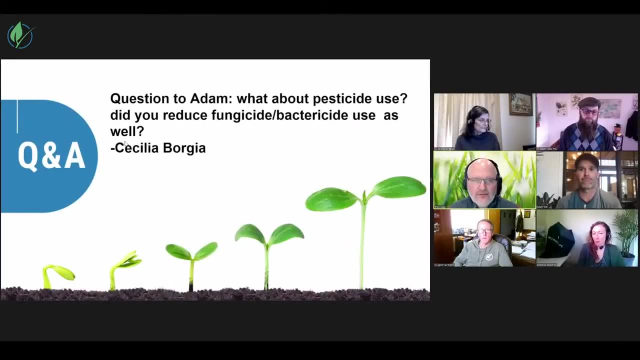 So it's kind of the same concept, Right Yeah, Fantastic Panelists, any other comments you guys want to make to that question about vertical tillage? All right, Let's move on to question number two And this one's from Cecilia. 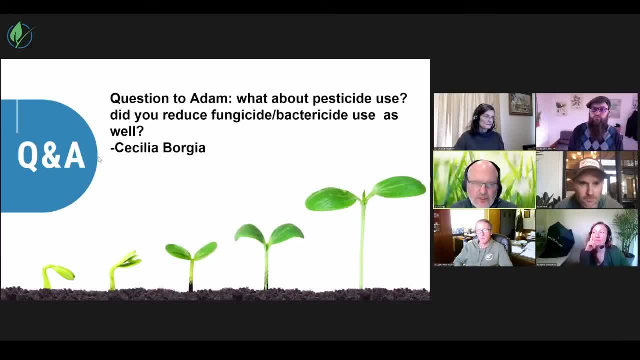 And the question is: what about pesticide use? Did you reduce fungicide, bactericide use as well? And I mean that could go to nematocides, somaticides and all those other kind of sides. I would say you, Adam, about that. 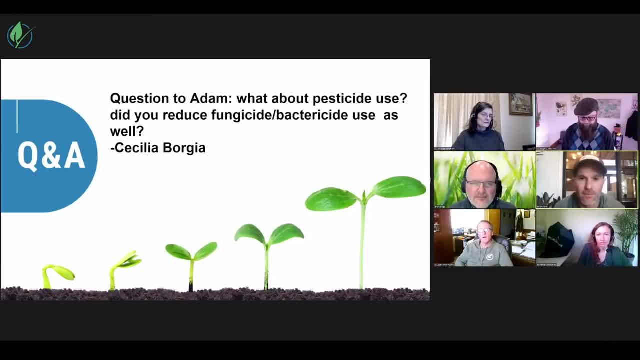 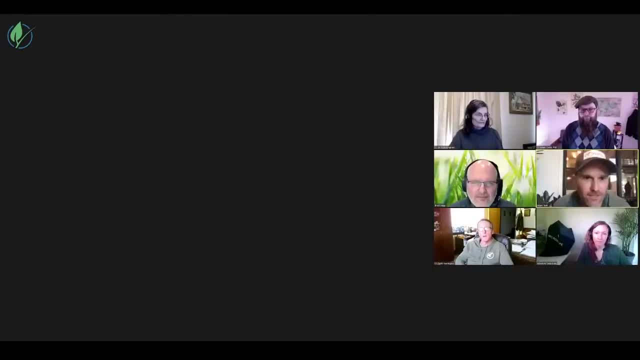 Yeah, So we don't use any sides at all, unless we – which we do. We use a fungicide here and there if we have to, But otherwise we don't use any of the sides. So we do use – well, other than pesticide, I guess. 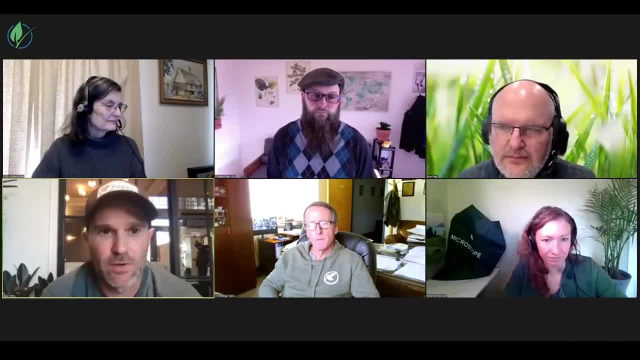 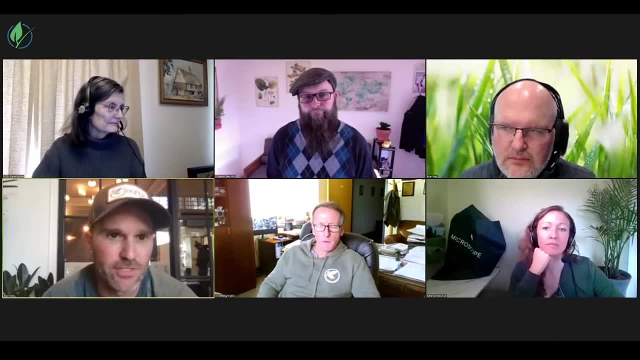 But where we've been with pesticides is when we went to non-GMO. we just went more to a non-GMO chemical program We have incorporated – there's a lot of really good research out there. I still have a little bit of work to do myself. 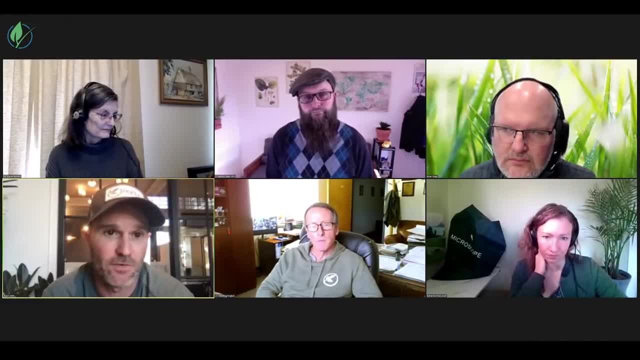 But there is a lot of research out there that guys are using fulvic acid, which we do use fulvic acid Helping to reduce their rates of pesticides. There's a lot of good work out there. That's something that we're still working on. 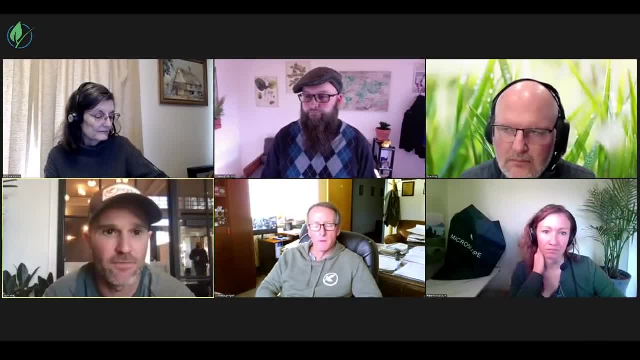 We have cut our pesticide rates. We have not cut them in half, but we have cut them down as much as another 25 percent and had really really good luck with it, And I think this year we're going to hopefully be able to do more than that. 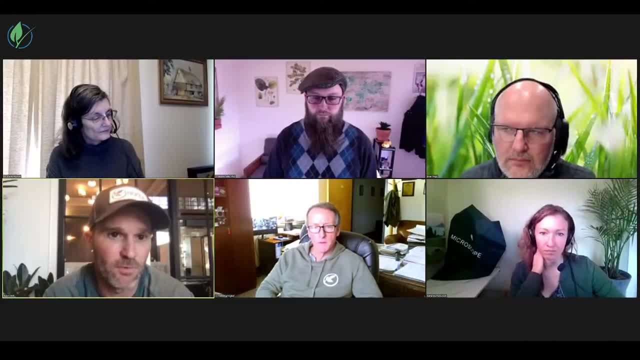 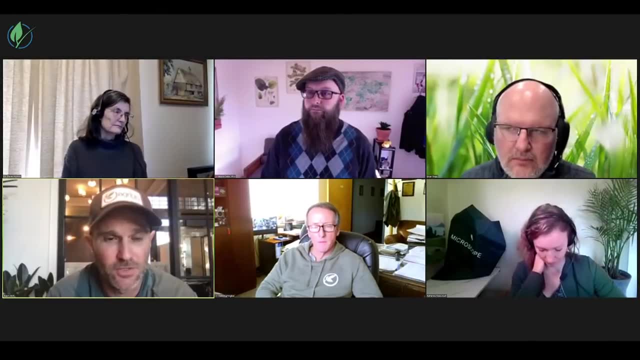 We just got to get to the point where we're feeling you know a lot more comfortable with that And we have to do trials And you just got to figure out where your comfort level and what you can and what you can't do. you know, so you don't fail. 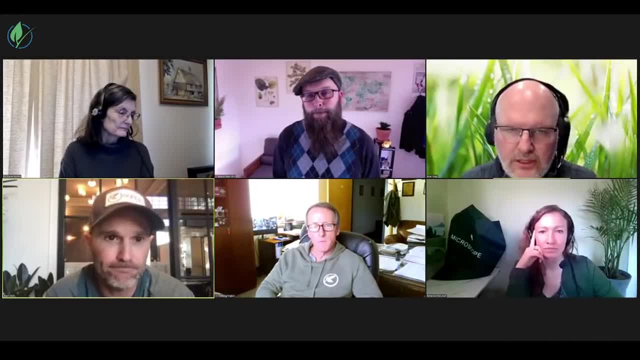 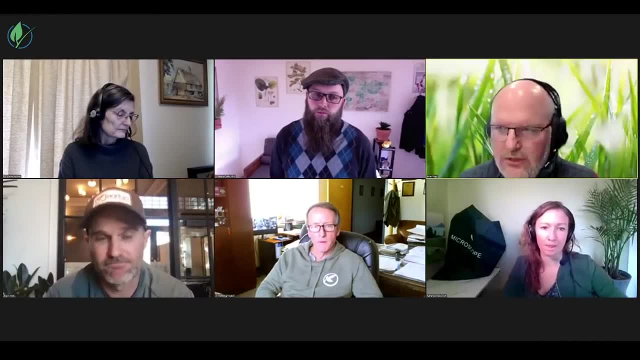 And that's kind of where we're at with it at this point in time, And, would you say, year over year, you think you're just on a sliding scale, reducing the amount of pesticide use. Your pest pressure is just becoming less and less and less. 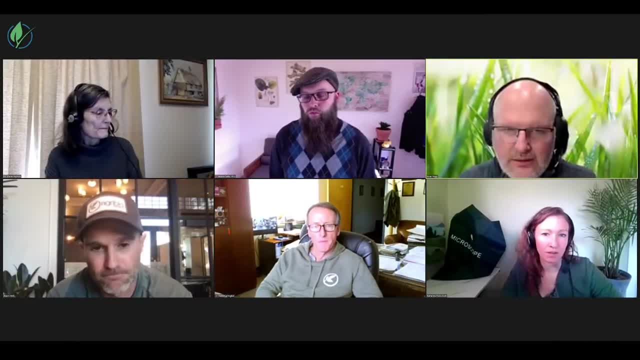 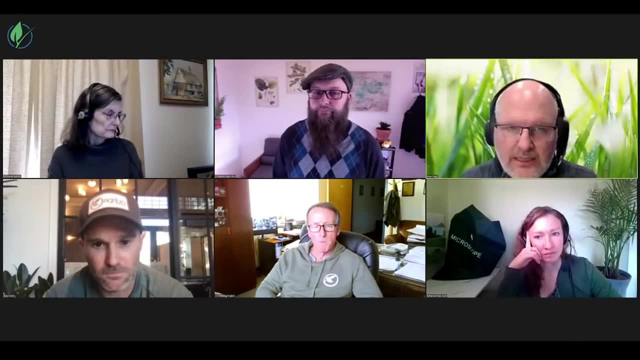 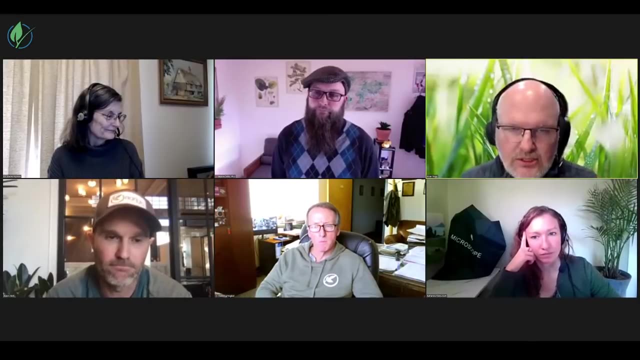 Yeah, Yeah, that is correct And I think you know some of the exciting things about pest control is in the biological side of the house- is we need to get better understanding about the life cycle, The pests we're dealing with and trying to attack those life cycles with biological, you know, applications and things like that. 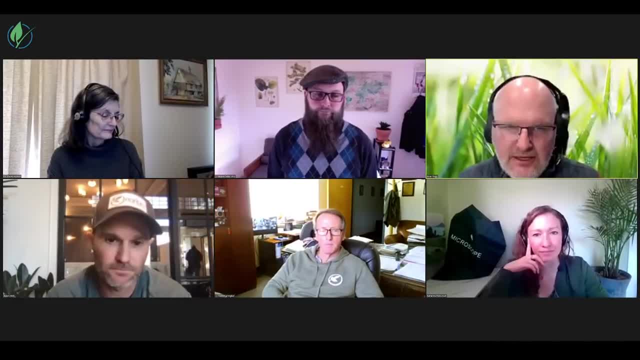 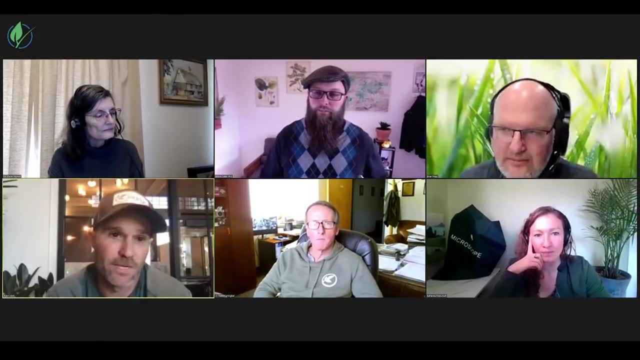 And you know and I know that there's a lot more science that's happening in that realm. But I agree with you. I think pesticide use you can reduce and then eventually just phase out. Yes, And that's the goal. I mean it's hard to just completely transition and just go cold. turkey. 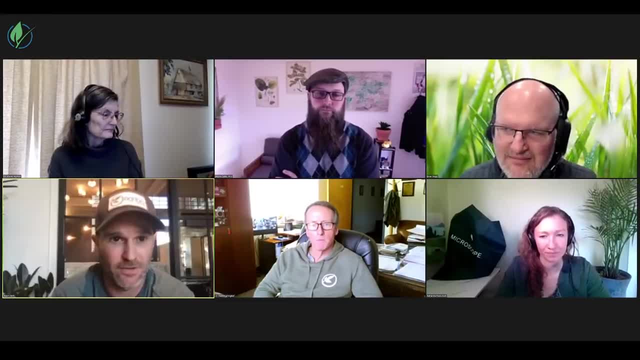 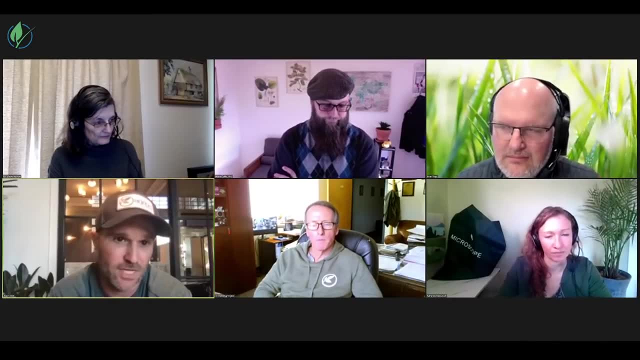 I've heard a lot of people doing that. I think that can be somewhat of a failure. you know, right out the gate. So you just kind of have to, you know, go And kind of cut, you know, but also test it to. you know say, hey, I'm going to go take a strip here and I'm going to do 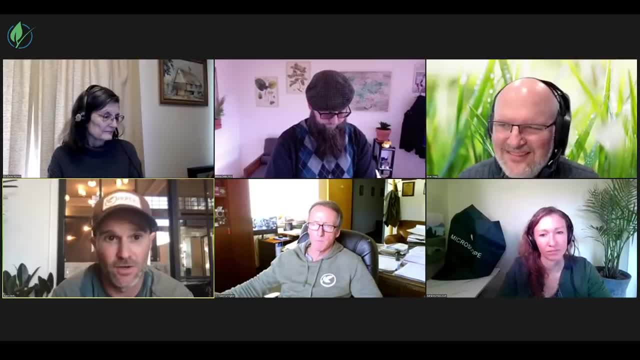 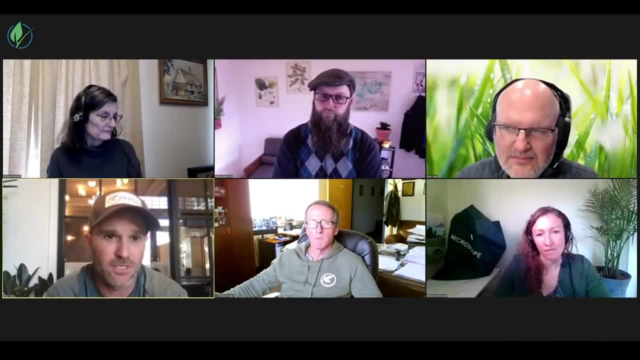 I'm not going to use any pesticide. and see where I'm at, you know, or do half a rate. See where I'm at there, And just you know. you don't have to do it on big scales, but do it on, you know, somewhat of a scale that you can actually prove to yourself. 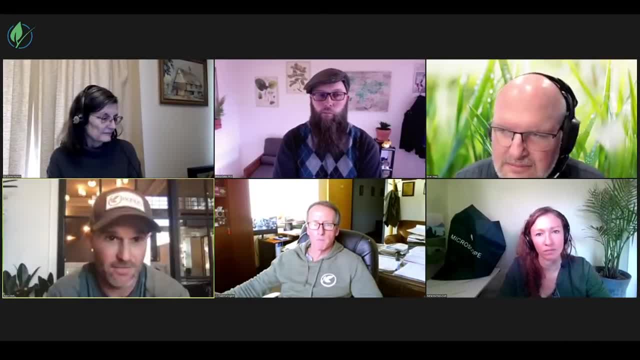 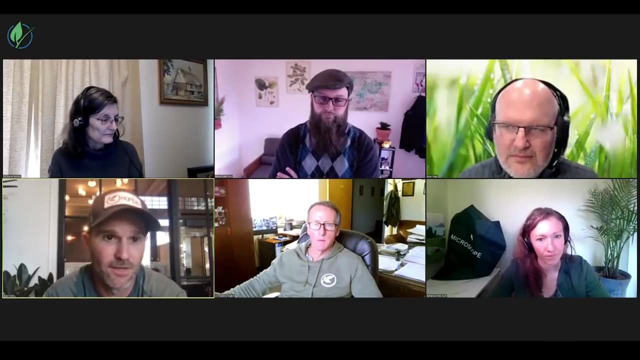 It's no different with nitrogen, You know. prove yourself that. hey, if I I'm scared to cut nitrogen or whatever, we'll just just just take a little bit And Try it, and that's the only way you're going to prove to yourself that you know I can- either I'm ready for this or you know not ready. but play around with different rates, and that helps you learn, in my opinion. 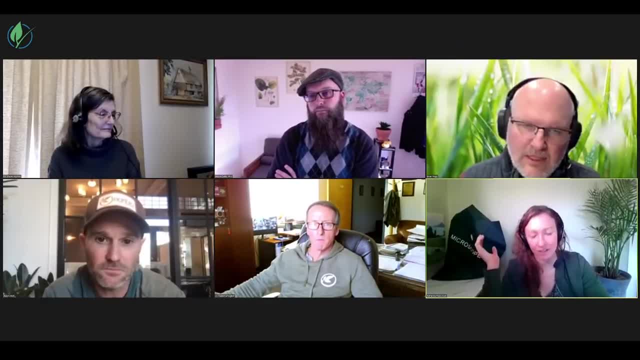 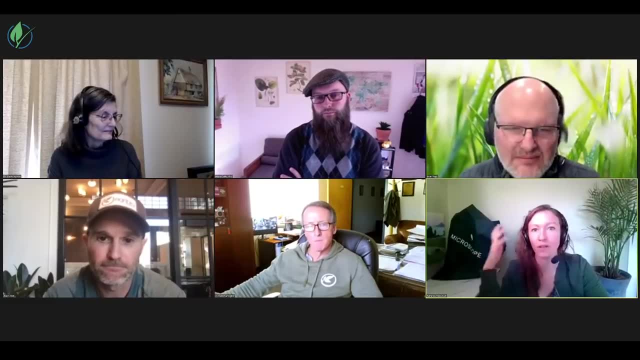 Well, in the tricky balance regarding- Well, I think you mentioned some diagnostic tools. Oh, go ahead, Adrienne. Oh no, that's fine. But the tricky balance there is that you know, once you start to build up this beautiful habitat and your soil and your plant communities, you're drawing in these insect predator communities that, if there's any, 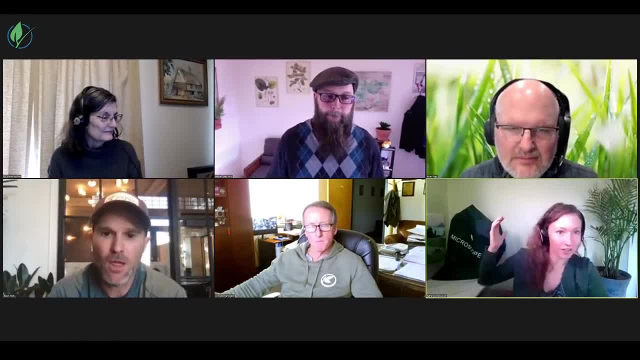 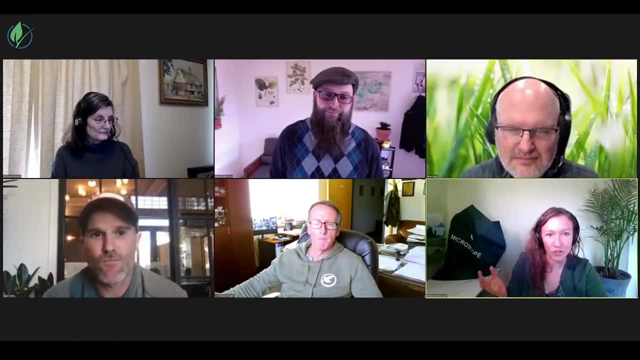 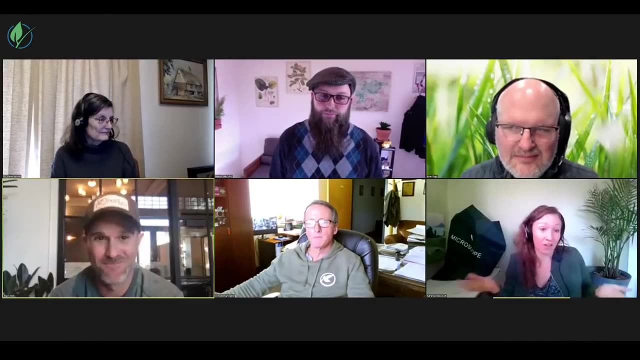 kind of Pesticide residues on that, then you're. you're cutting your legs out from under you when you could be using that workforce and community support to help just solve the rest of the problem. So at a certain point it is like a leap of faith that you lost, or the opposite, right? 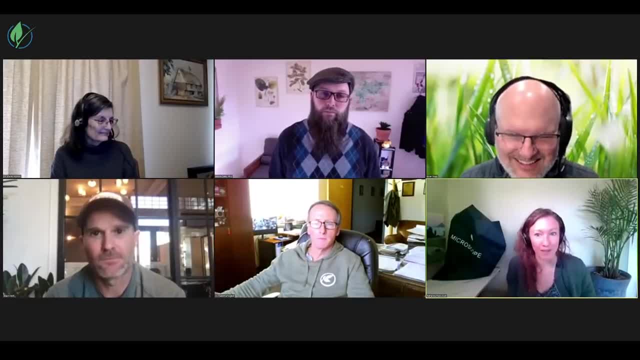 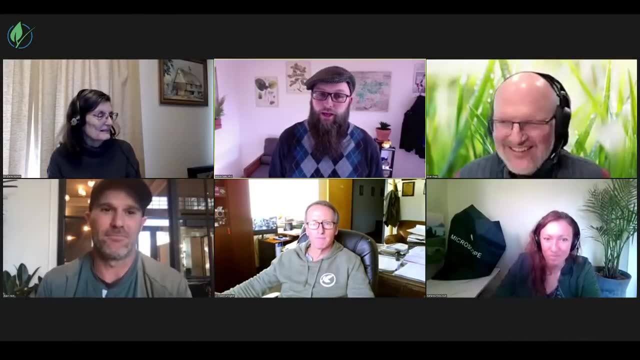 You bring them in and you kill them. Then you're killing the predators in your area with your pesticides that you're afraid to let go of those houses again. Yeah, exactly, Build new houses, right, Yeah? And you know I really like that. 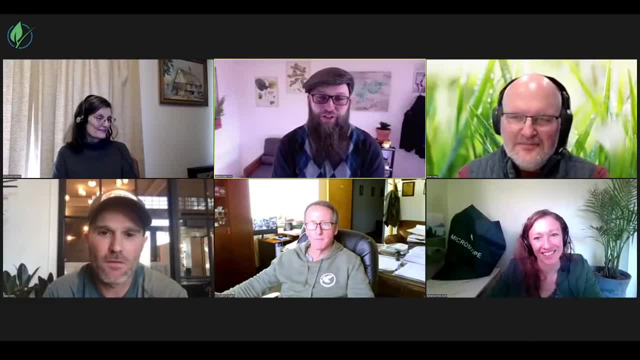 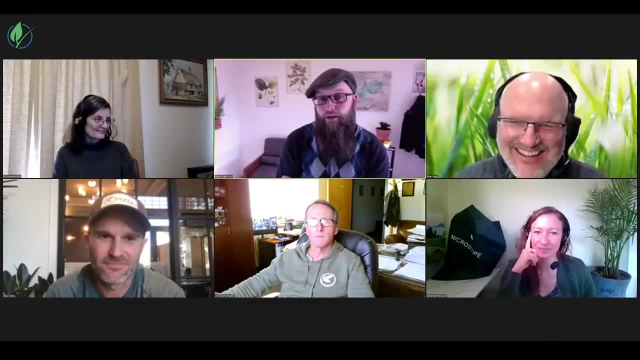 You brought that up, Adrienne. You can tell that we're two ecologists in the room, because I love anything related to this kind of discussion so much. I heard a talk by our local Xerox society that focuses on, you know, especially native pollinators and other beneficial insects. 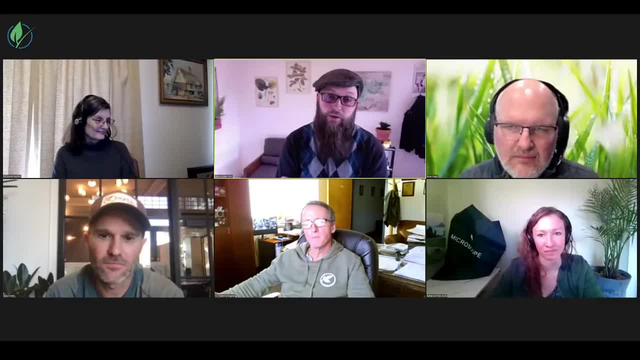 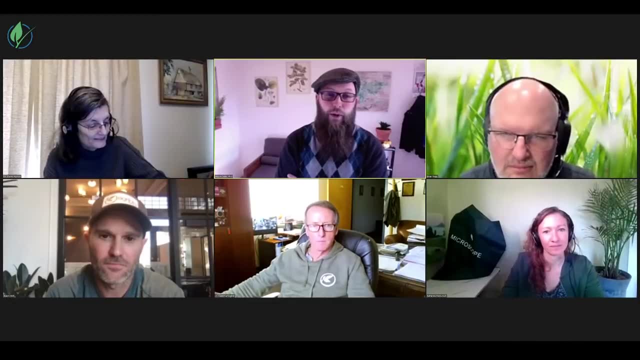 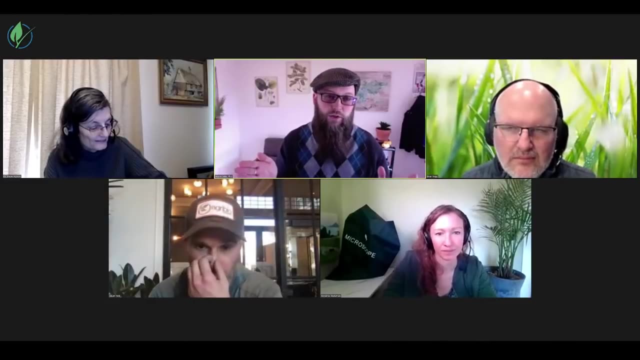 And most states have an active Xerox society. If you're in the US there's probably an equivalent group in most international contexts that can help you determine if you have like most farms. Yeah, absolutely, But you know some of the barns have little areas that are not economic for actually row cropping. And so if you can start to establish the kinds of native plants that draw in the native predator insect populations and give them places to overwinter or floral resources, like nectars, that are specific to them, then you know- I've observed with my own eyes in home gardening that certain flowers will bring in, like parasitic wasps that destroy all the aphids. 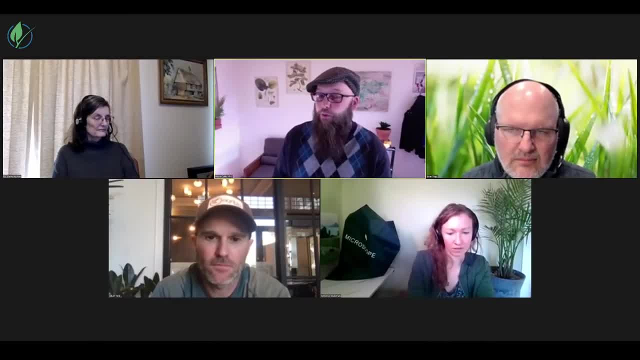 You know happy, you know feeding, You know that's a kind of a thing that a lot of individuals like to do. That's a great way of doing it, And we have to think of this as something that we could do. 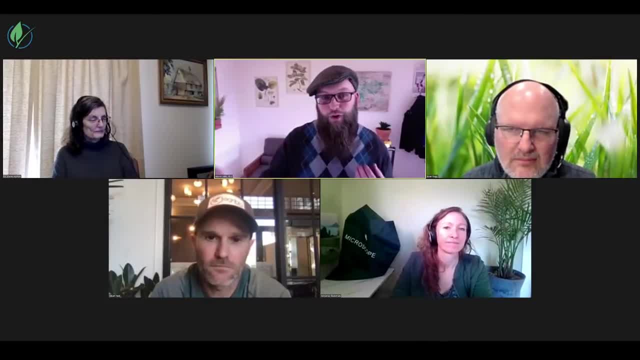 You know we're talking about a powerhouse for a lot of people, Yeah, And we don't want to do it again, Right? You know we're talking about some of these things that get on your cabbage, right, because they're laying eggs inside every aphid and you can just. 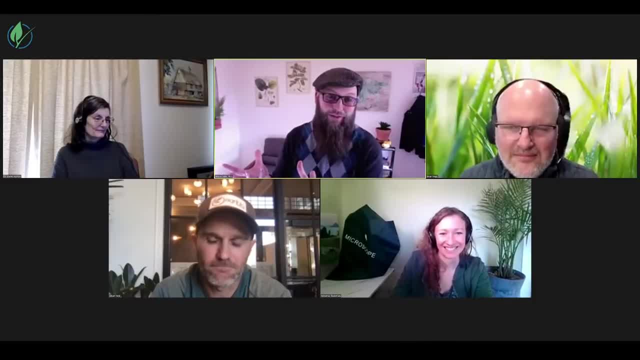 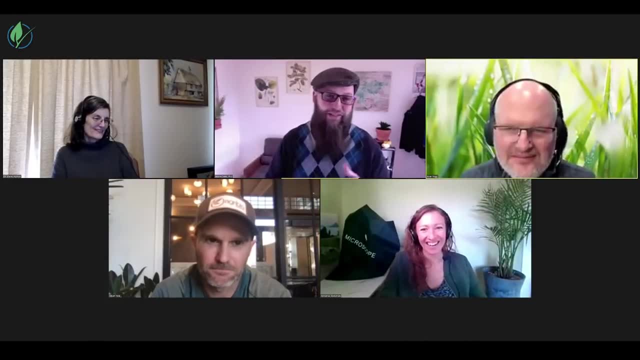 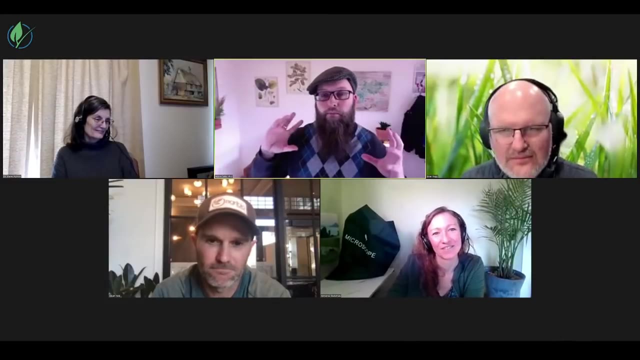 see, they call them mummies, the, the dead aphids after a while. so what i say? they look like little puffed rice rice. yeah, it's, it's really gross, but it's better than them eating your cabbage, right? so, uh, you know what? what i've seen is when, when, when, people make the the mental transition. 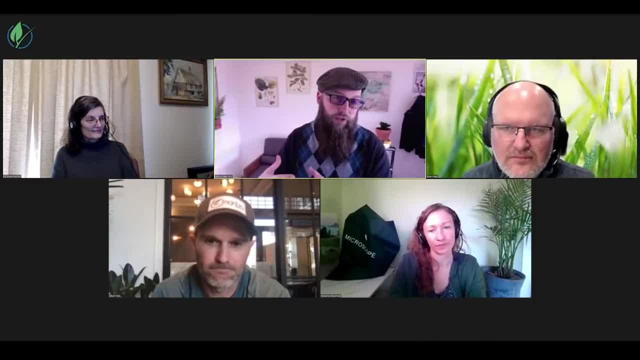 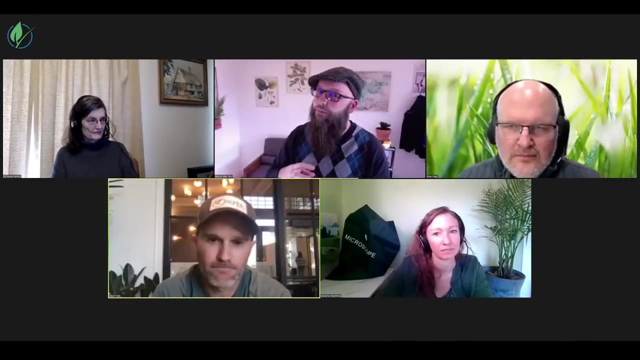 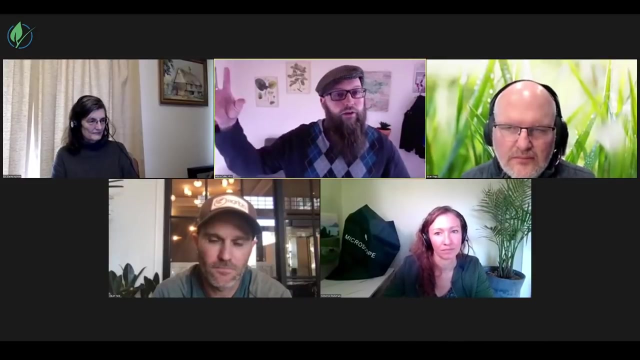 to thinking about optimizing especially the nutrient inputs on their um operations and making that- uh, you know what adam referred to is sort of like an investment strategy rather than a kill it deal with the fire strategy. then it frees up a little bit of time and resource and energy to think: well, i've got that area over there by the creek i can't crop, but maybe i could. 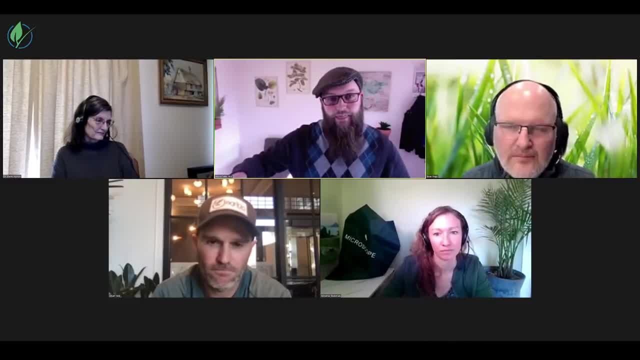 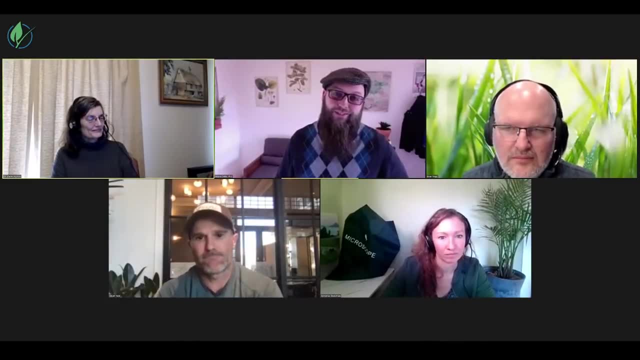 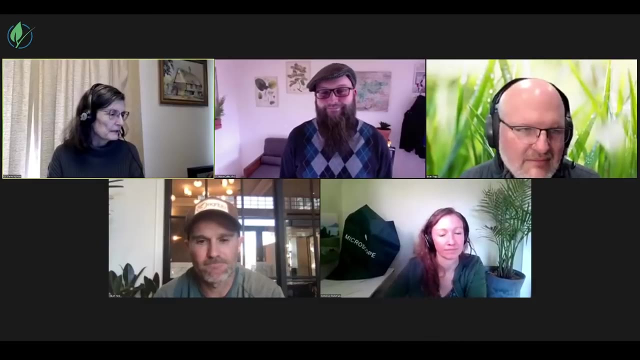 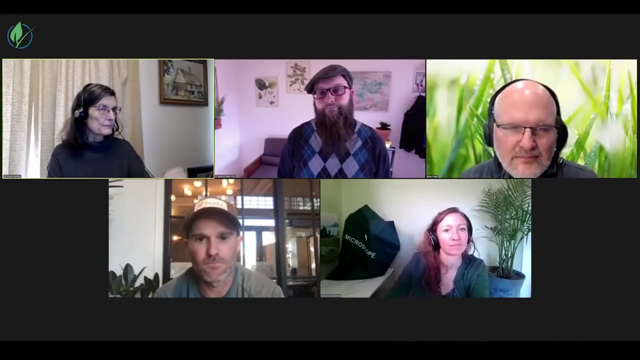 establish some beneficial native plants there and then that just builds over time. you see this like virtuous cycle going on with the ecology of farms. yeah, i also think it's probably really important to be keeping track of what the biology is in your soil. have you gotten the organisms up to the point where they can control where they've? 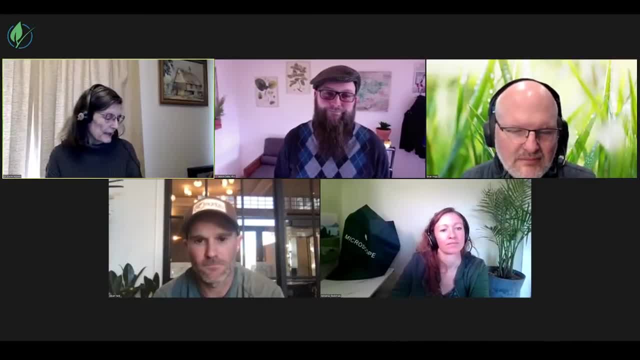 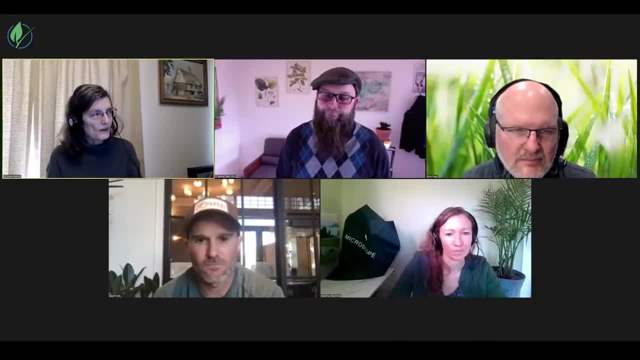 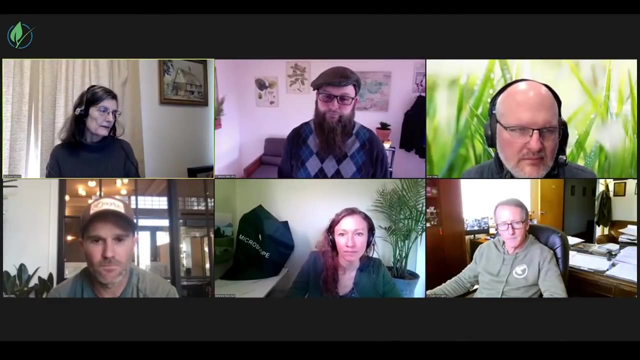 have the workforce to take care of the problems if you've just gotten barely started getting your bacterium, fungi, protozoa, nematodes, micro arthropods up to the right place? if you haven't gotten there yet, you can't be expecting that these organisms are going to take care of all of your problems. right away. if we can get all of that biology back into the soil, we see that we can do this in a year. but if you know, for one, one reason or another, it takes a while to get those microorganisms established, well then, go at it more slowly. go with reducing your nitrogen by x amount by. 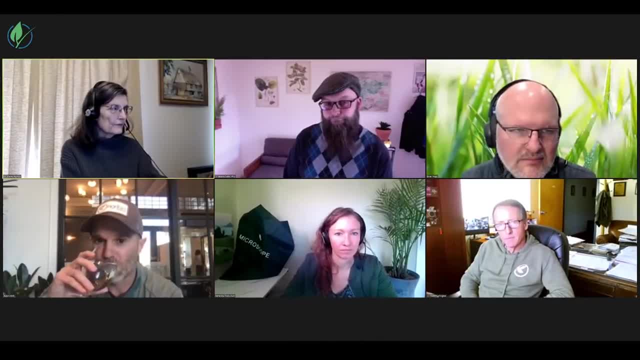 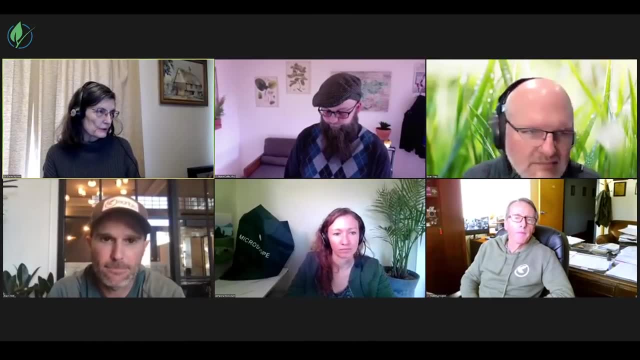 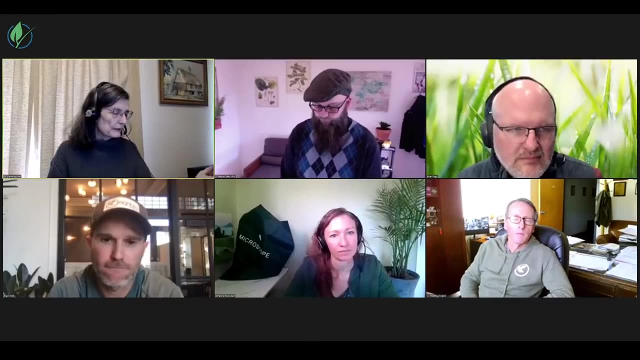 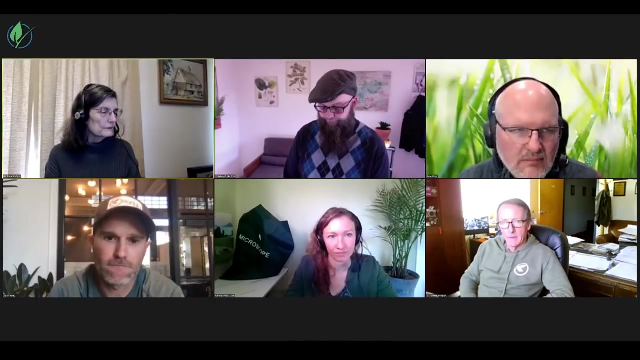 putting on fulvic acid. so you'll have some of the pesticide and fungicide effects of those materials feeding the organisms, getting rid of your problems. little by little it'll increase. so it's kind of up to you as growers, up to us, to encourage our clients to be moving along that sequence as rapidly as possible. 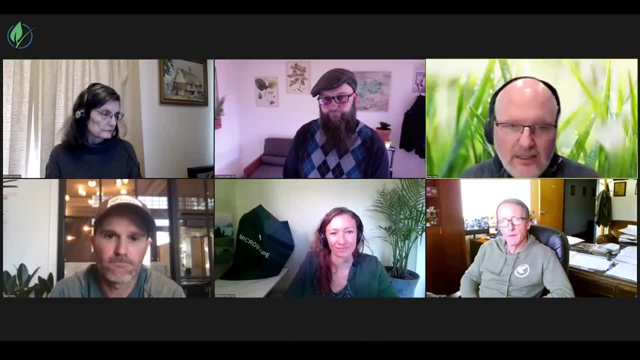 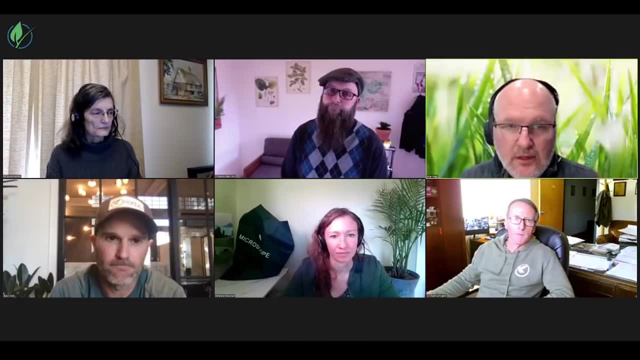 i keyed on something that adam had mentioned too, that you know it's not like we have to make it a guessing game. there's a lot of diagnostic tools to help you make decisions about this: plant sap analysis, tissue analysis, soil chemistry, microbiology assessments- all that data then helps. 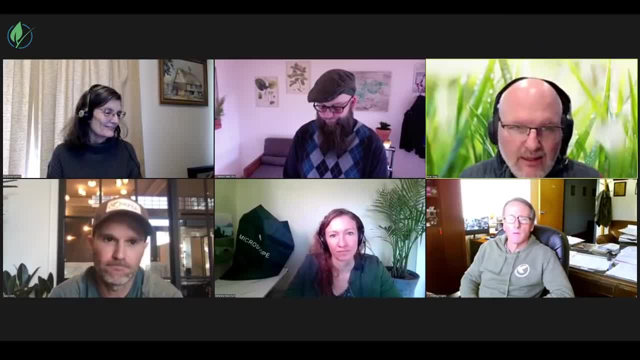 you exactly helps you build this picture of saying, okay, here's what's happening and here's what we need to do, and you know you can be very smart and specific and prescribed about what you're trying to do, versus just a guessing game. all right, our next question is related, so i thought i'd pop this up. 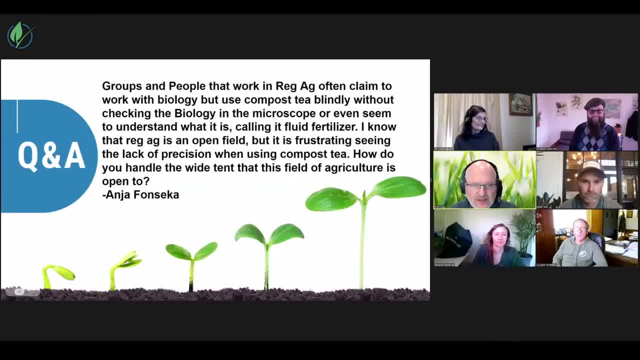 here, perfect, and i i love this question. so, anya, um, i think this is a fantastic question. uh, groups and people that work in regen ag often claim to work with biology but use compost tea blindly, without checking the biology in the microscope or even seem to understand the biology of the compost tea. 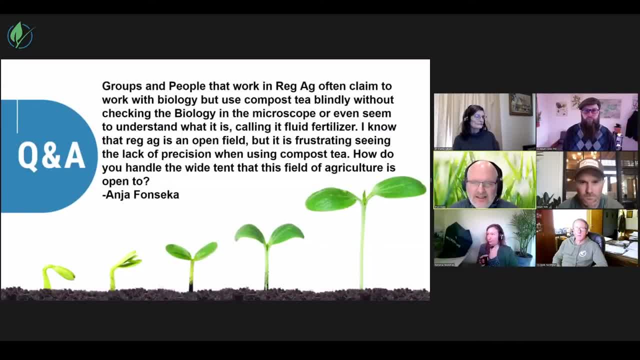 but it used compost tea blindly, without checking the biology in the microscope or even seem to understand what it is, calling it: a fluid fertilizer. i know that regen ag is an open field, but it is frustrating seeing the lack of precision when using compost heat. how do you? 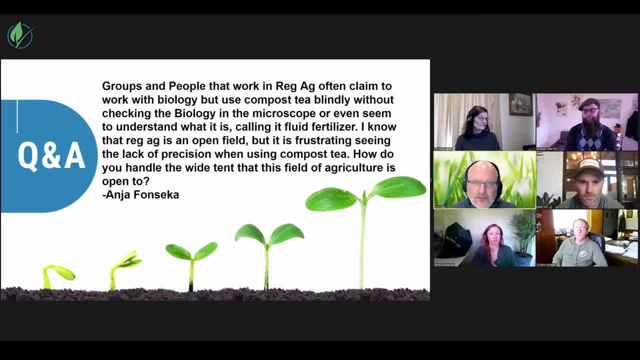 handle the wide tent that this field of agriculture is open to and boiling. i think this question's geared right to you, because your work has been focused really on this question, right, yeah, and where you have to be finding out what those sets of organisms are in your soil. so where are you? 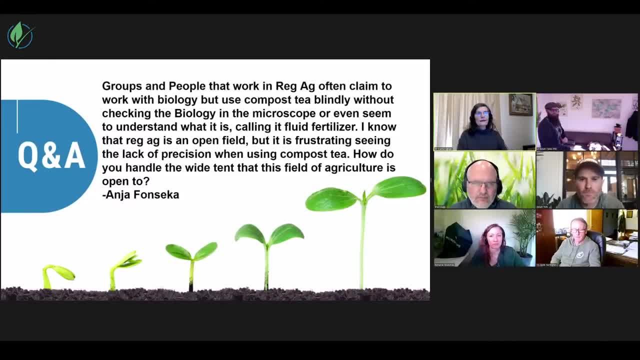 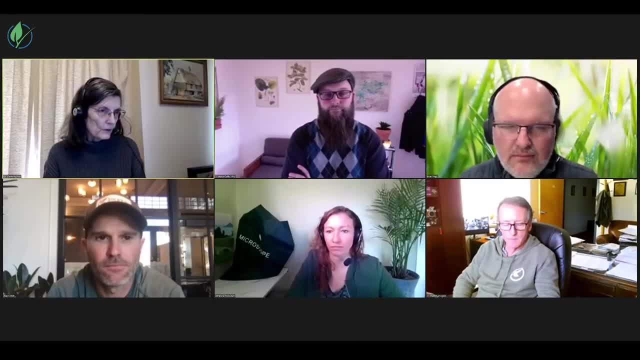 from what's missing. how much of it are you missing? And then how are you going to get those organisms established in your soil? So how rapidly can you convert your dirt back into soil? And I think we've just got to remain steadfast, reminding people that they do have to know what they're. 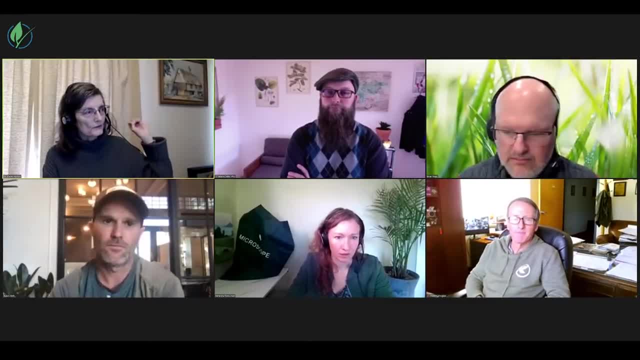 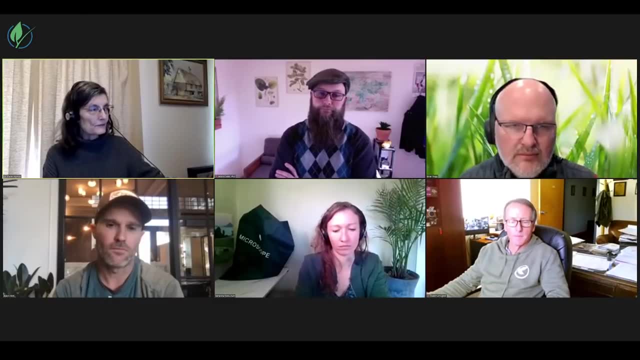 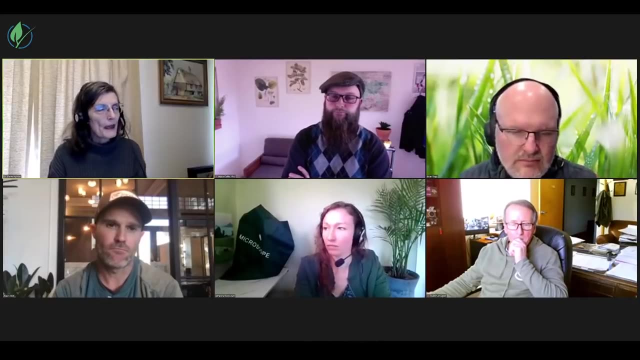 doing. You know you're not going to just throw a firebomb on something and cross your fingers and hope that it's going to come out with the right kinds of microorganisms left in the soil, because most certainly it is not. You need to be measuring It's. you know, how can we manage if we can't? 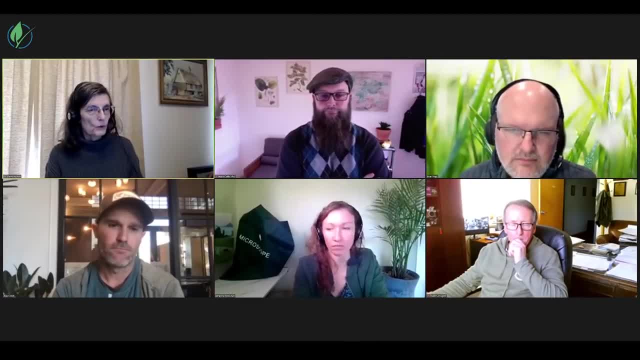 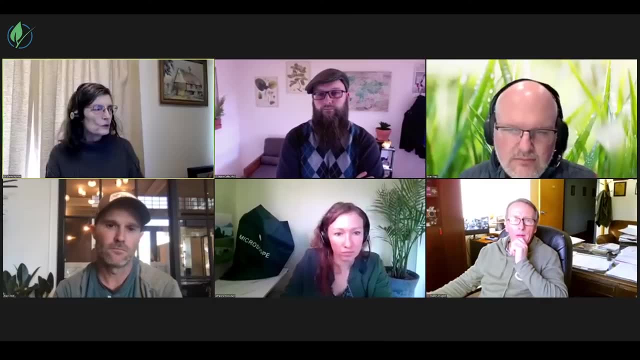 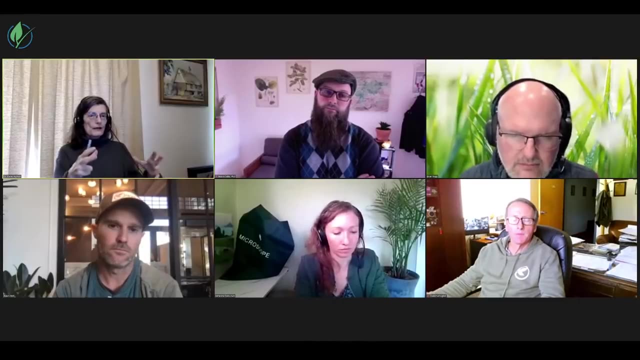 measure, And that's what the biology, the microscope work, the biology in the soil is all about. You need to be measuring the organisms. Do you have what you need? And then remember that it's not just looking at your soil. It's looking at the soil as if it's one way of existing, because soil is constantly trying to. 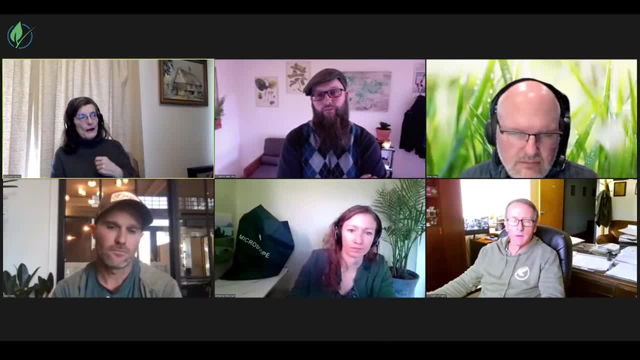 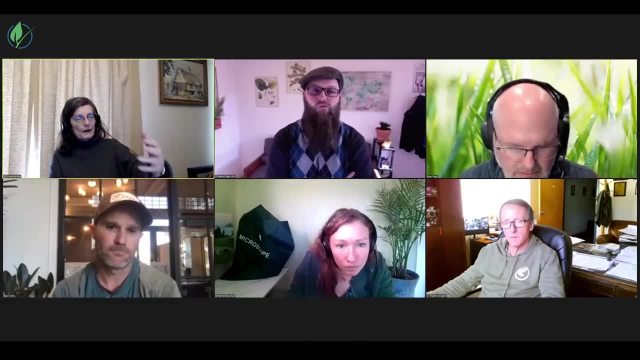 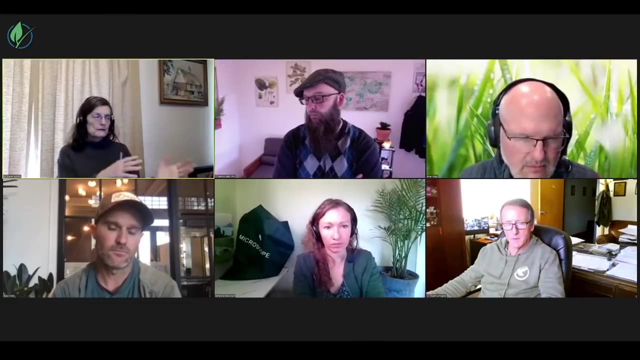 improve itself. A disturbance comes along, you're going to go backwards, And then you get to restart fixing the problem again. And if you disturb before the biology is established, you're going to go backwards. So how many times do you have to do the back and forth game until you understand? 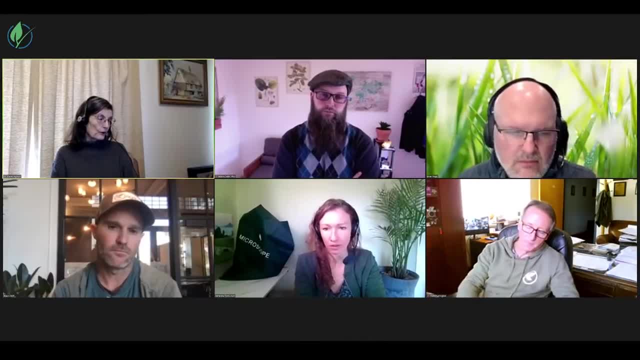 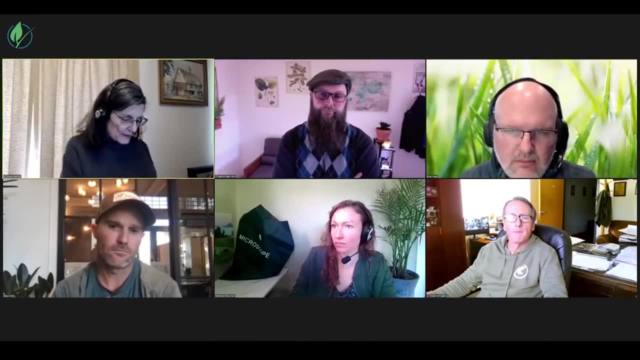 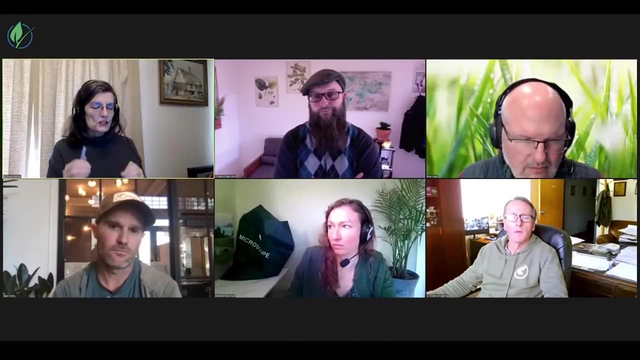 you need to be keeping an eye out on your soil And then you get to restart fixing the problem again. You don't have to be really serious. you know seriously. you know pinpoint in your answer. we don't need three place decimal precision And we can do more of a qualitative test- you yourself. 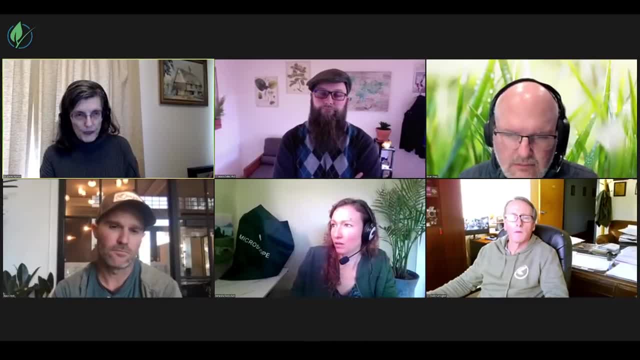 could be looking at your soil once a week And it's going to take you 20 minutes to get an idea of whether this works or not. And then you get to start looking at your soil once a week And it's going to take you 20 minutes to get an idea of whether this works or not. And then you get to start. 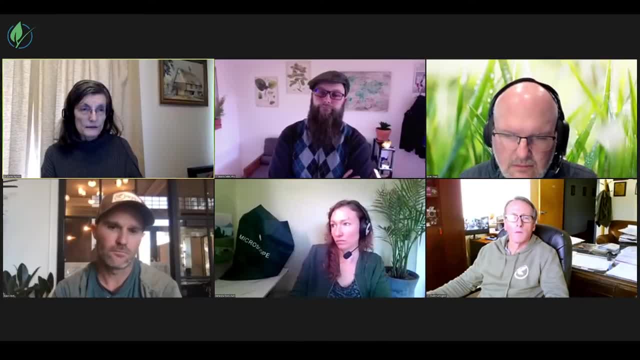 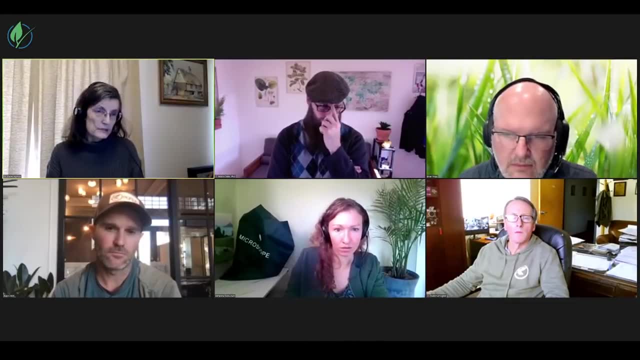 looking at your soil once a week And it's going to take you 20 minutes to get an idea of whether this field has a decent level of organisms or not. So you know the reliance on quantitative analysis is important several times during the growing season, but in between you can be taken really. 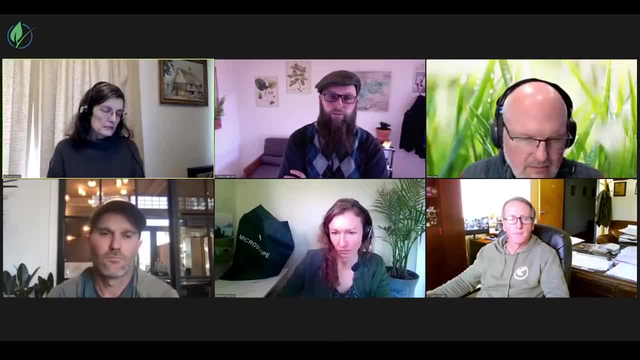 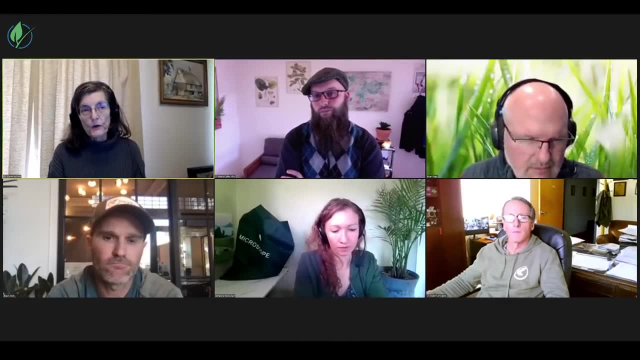 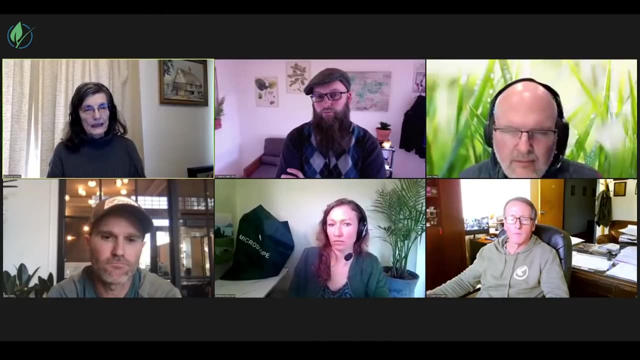 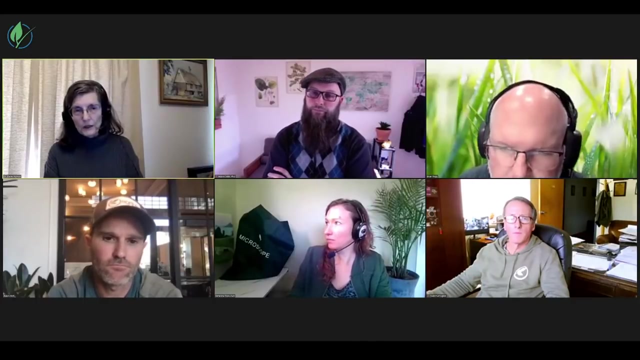 quick and easy to do assessments, just having come and worked with us for going through the foundation courses, for example, the fourth foundation classes teaching you how to use a simple microscope and getting qualitative comparisons of. here's where we started. we've increased it by by a factor of two. we need to increase it by a factor. 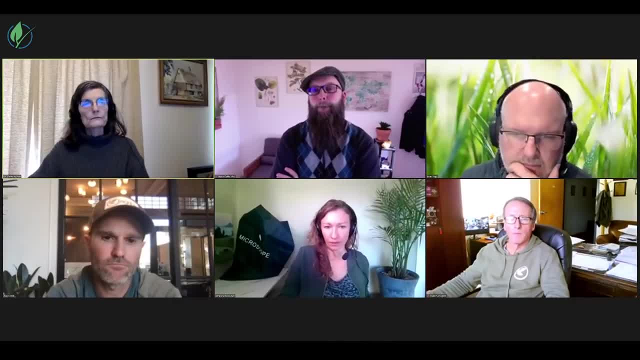 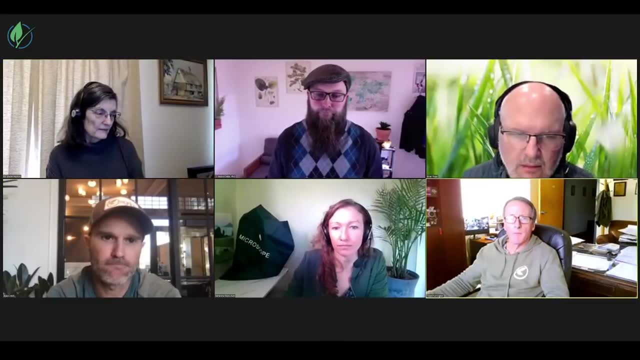 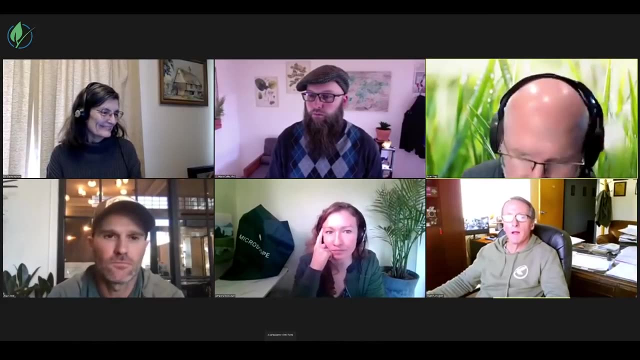 of 10.. And so you just keep working for that goal, knowing that you'll get there as rapidly as possible, hopefully. Hey, Elaine, I have a quick question. Brian, I asked Lane, a quick question for you. Yeah, go for it. Yeah, So a lot of clients are doing this: applying these compost. 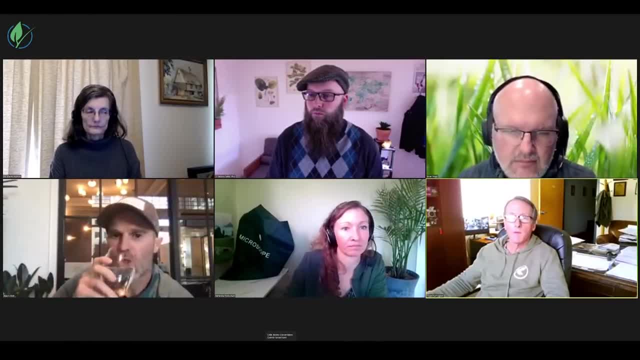 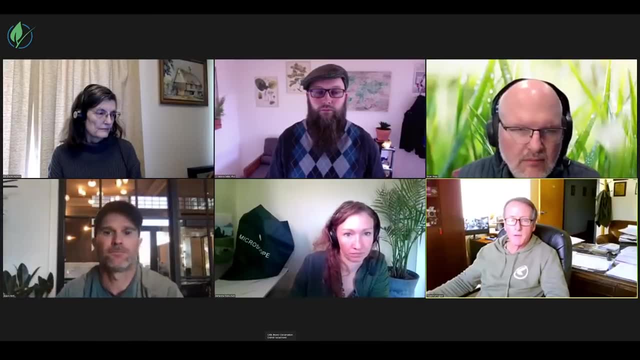 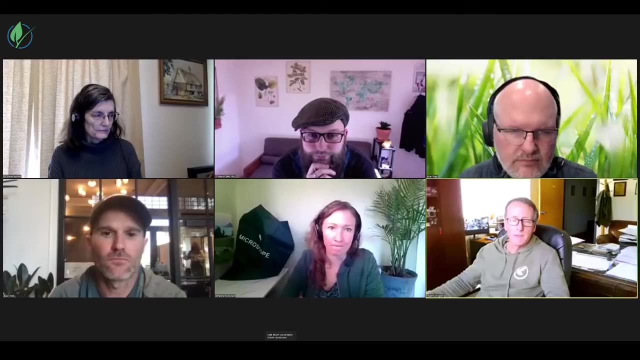 teas kind of randomly, without testing. at least you know direct microscope plate counts And yet they're doing. you know they're having companies come in doing pretty expensive tests, doing the PLFAs and the DNA testing, And so they're getting all the different you know species and 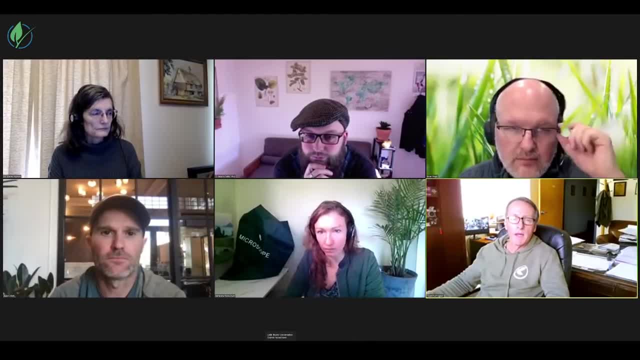 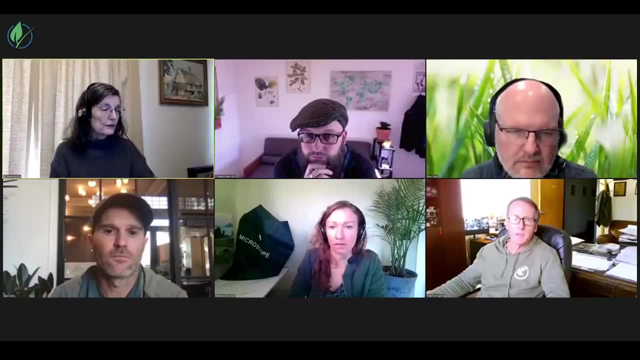 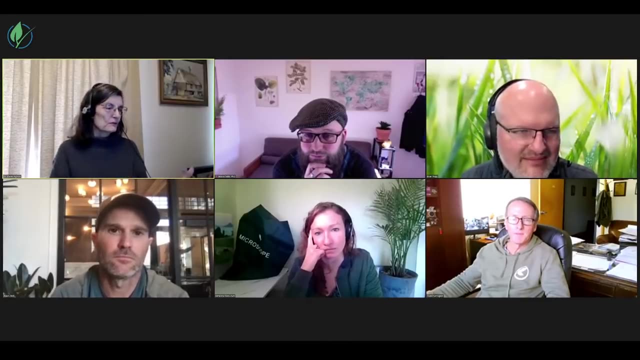 you know doing these expensive tests, but yet they're not doing direct plate counts with their biology, their compost and their extract. Well, you don't, you don't ever, you don't ever want to waste your money on plate counts. That's the most meaningless thing that you can do. 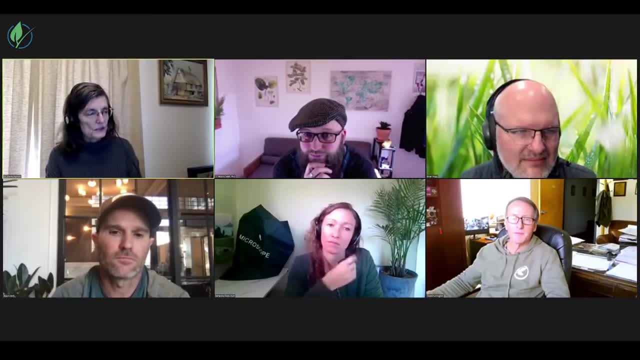 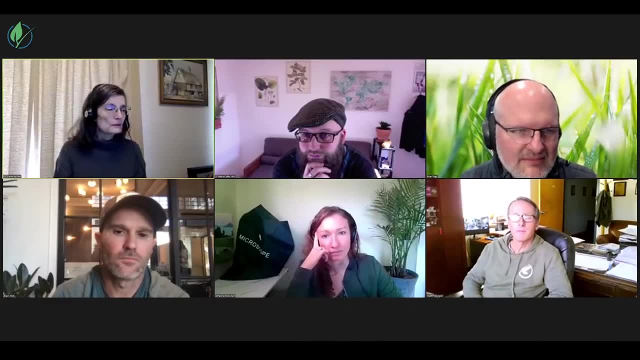 thinking that you're learning something about the organisms in your soil. 99% of the organisms that are in your soil cannot and will not grow on plate cultures in the laboratory. They just sorry. it's a waste of your time and money. 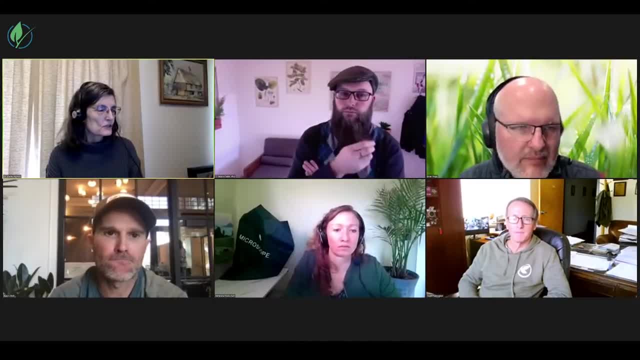 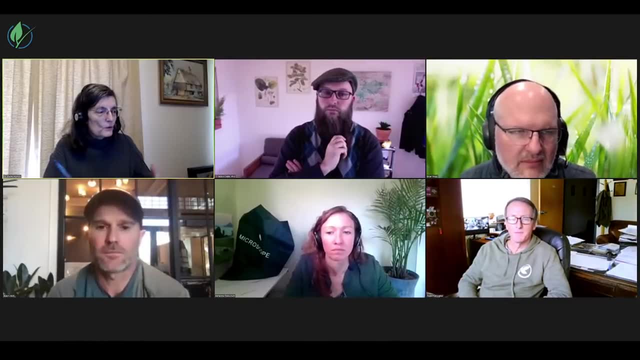 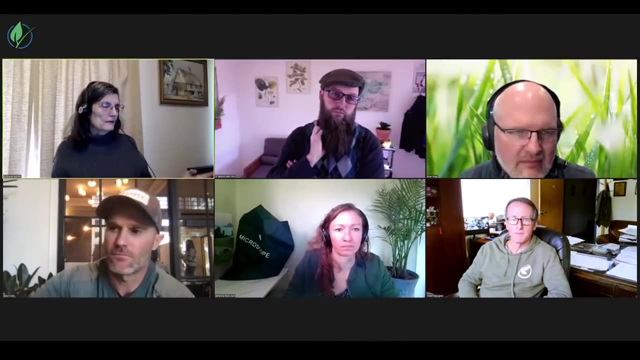 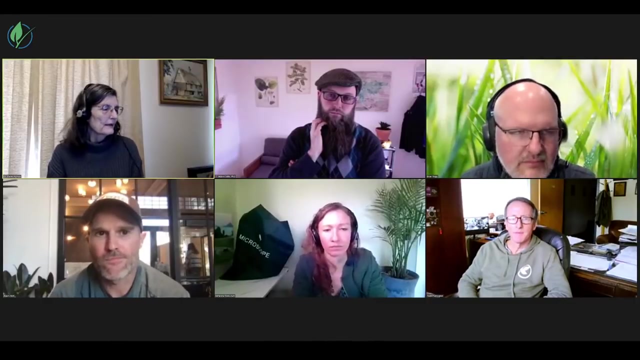 PLFAs. we're showing that that has nothing to do with the biomass of the bacteria and fungi. Most fungi don't make the PLFAs, the phospholipid fatty acids. They just don't make that PL, the simple, easy to determine PFLA. So you're not getting an estimate of that fungal biomass. 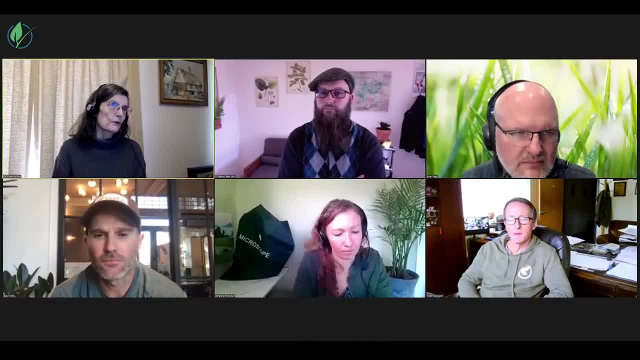 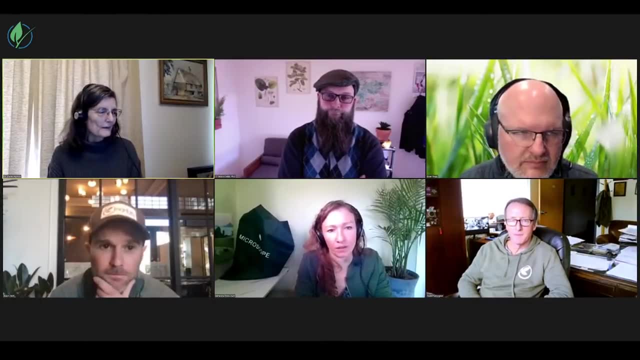 You're not getting an estimate of the protozoa or the nematodes, good or bad. So it's you know. again, that's another waste of your time. Now, microscope work. Yeah, That's what we want to be doing. 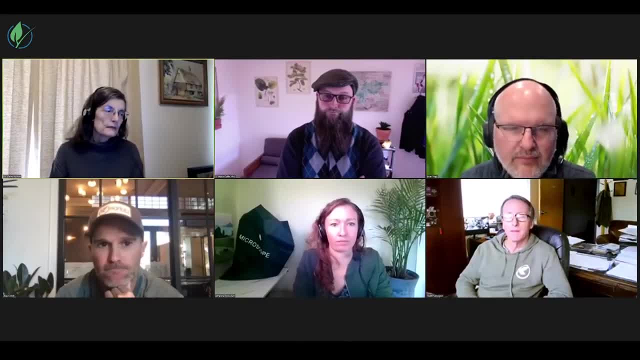 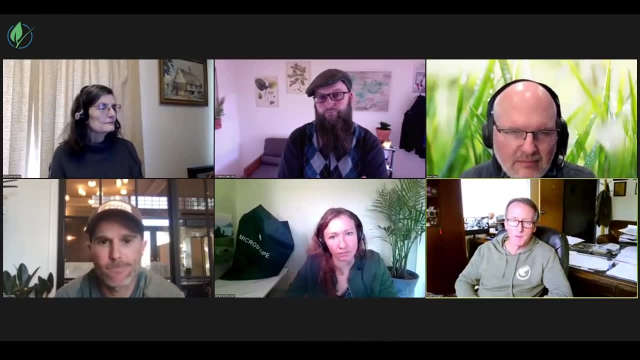 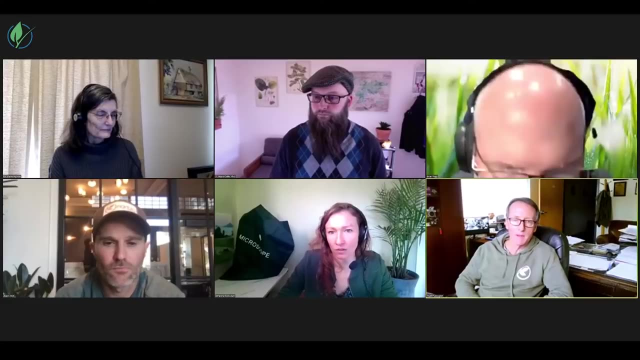 It's easy to you know folks that have gone through the courses, you know they- they being able to do the microscope work is it's really really important when you're doing this, you know, looking at the extracts and the actives, you know, and that's something that 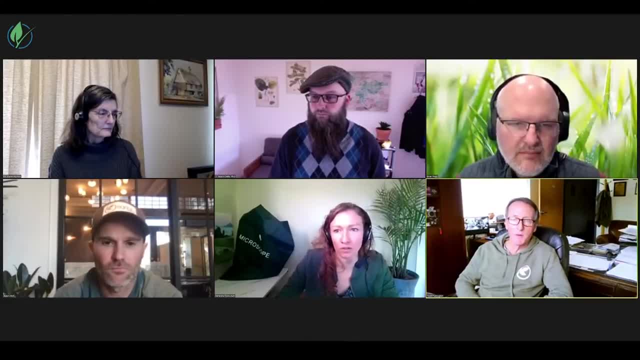 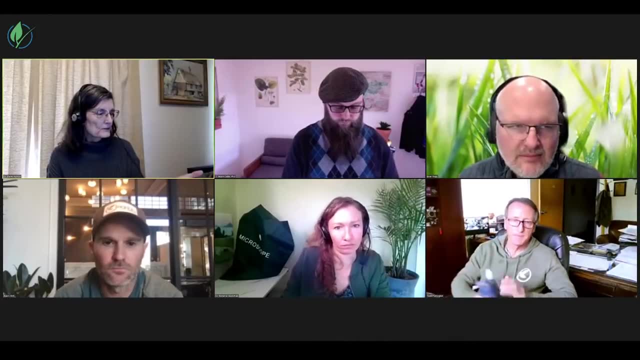 Adam's done a great job with. They have, we've got them, they've got a microscope and they're always looking at their stuff, Always Yep, And that that gives you an idea of whether you're moving things in the right direction. Why keep putting on something that's actually 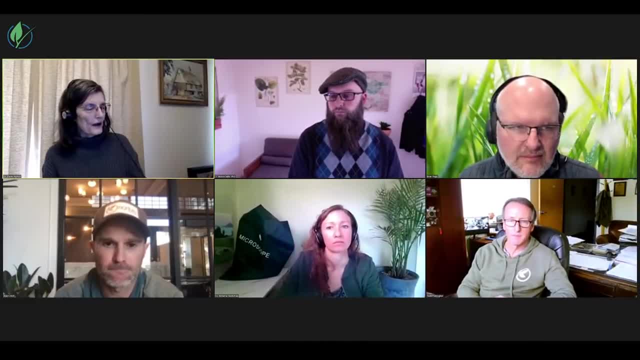 making you go backwards, And if you don't make your your compost tea correctly, you can push the biology backwards into a worse condition where you're going to be promoting diseases and pests. So you want to make certain if you're going to take the time to 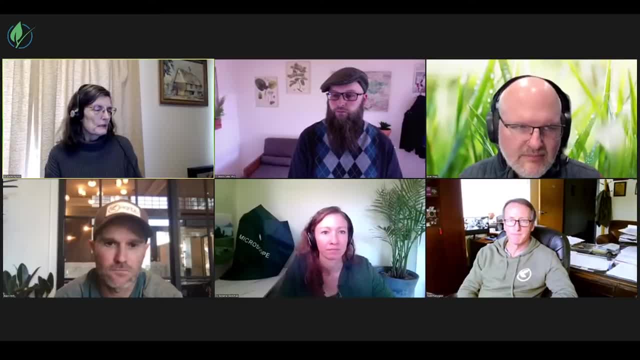 make a compost tea. let's take the 20 minutes to look at what's in there And is it going to improve your soil or not? If the answer is not, go put it someplace else where you still have a problem, Even once we have a good compost tea. sorry, Brian, Go ahead. Adrienne, No, go ahead. 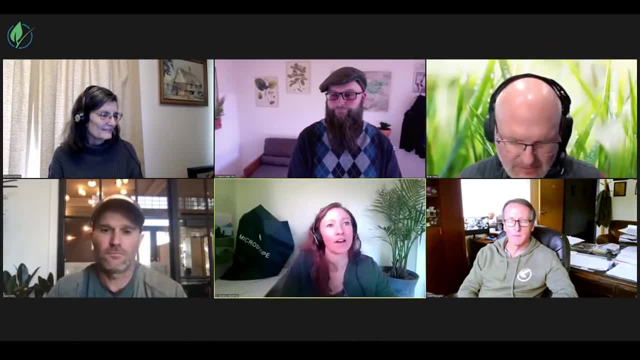 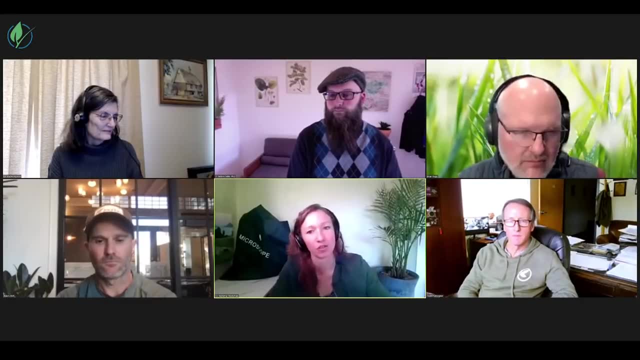 Even once we have a good compost tea. thinking about the things, the other practical elements like you're describing, Adam. thinking about how you navigate your field and work with your practices to make sure to support those. the biology that you get out there you have to reassess and make. 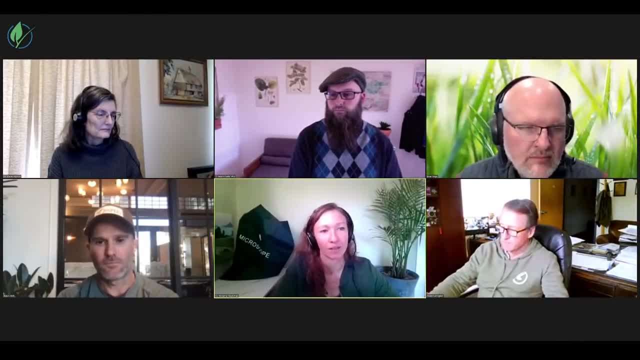 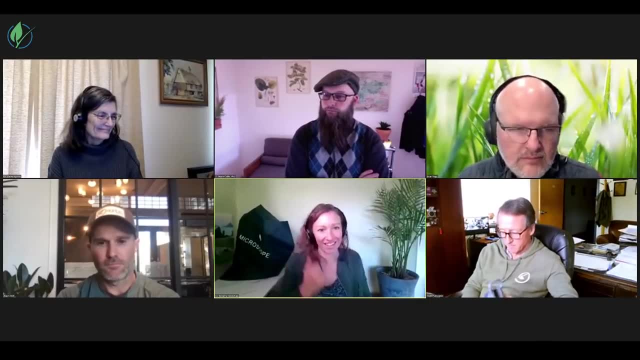 sure they're actually establishing And make sure you know, like you're saying, the asides. you try to keep as many of those asides out of there. I like to say let's leave the asides aside. You know, and that's the truth, And we have a, so we bought a crimper, oh, a couple of years ago. 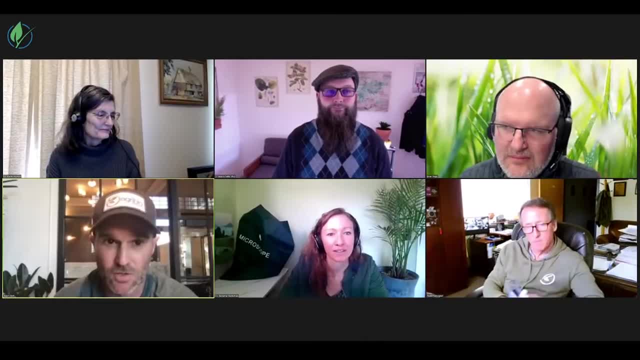 And our plan is, you know, we're going to try to transition a couple of hundred acres all the way up to the top of the mountain And we're going to try to make sure that the asides don't go over. you know, and and roll and cramp. You know there's a lot of there's. 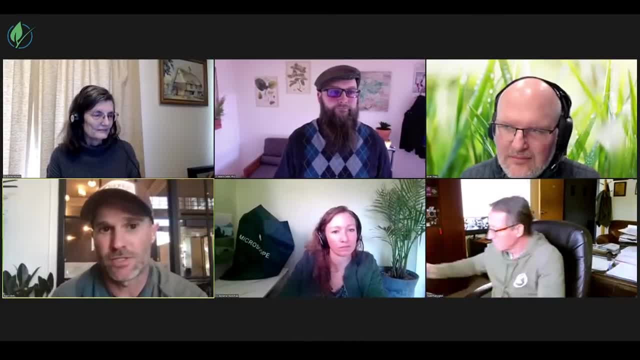 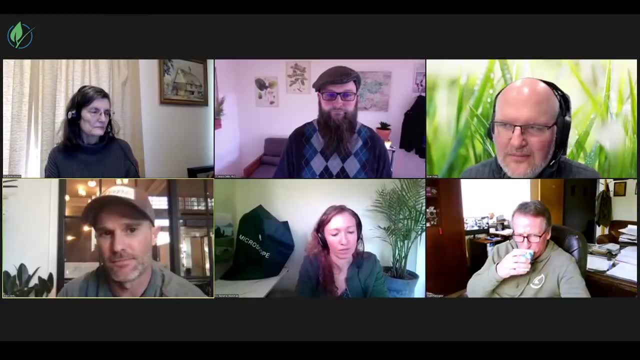 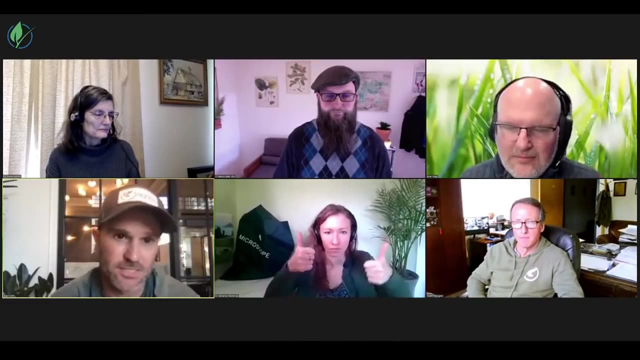 a lot of organic guys that are doing a lot of tillage, you know which, whatever, but we're, we're our. my plan is to maybe do some more cover crops: crimp it, plant a crop into it and kind of go that transition to get away from insecticides or you know pesticides. 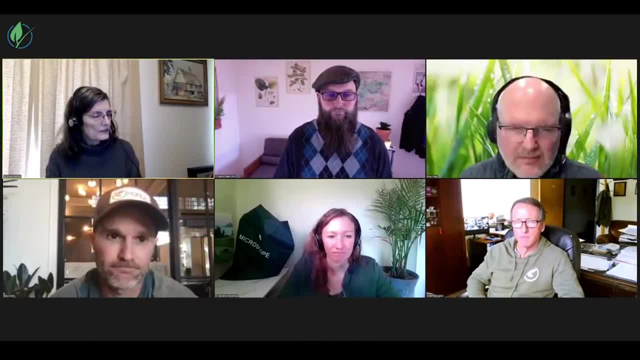 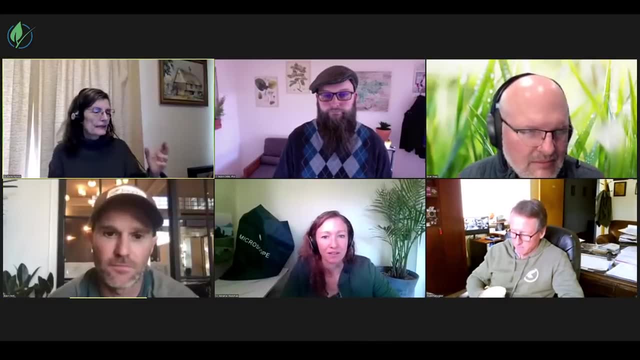 you know at the end of the day. So, And I'd encourage you to look into short, low growing ground covers instead of something that you got to roll and crimp, Because I can never get out there at the right time to roll and crimp and get the result. 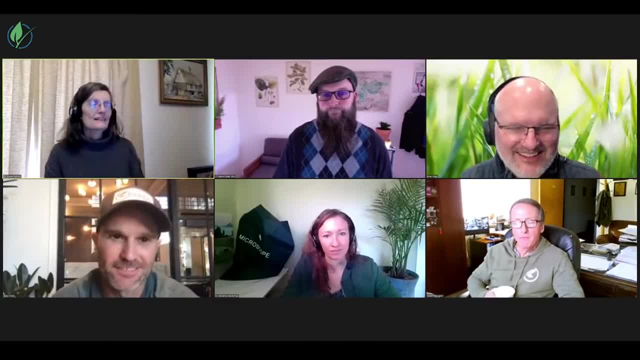 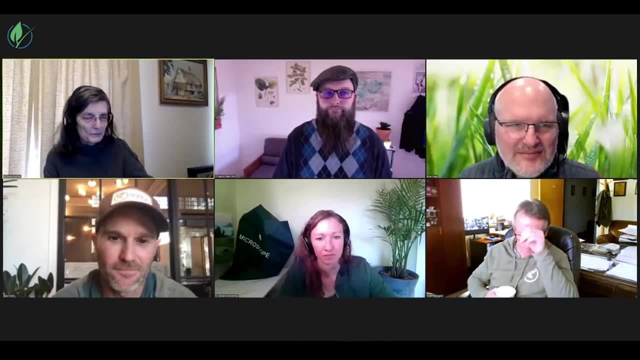 that I want. It's just my life is too complex. I just, you know, it's like you look out the window and you go: darn, I should be out there rolling and crimping and I could take care of the problem, but I'm not going to be back home until next Sunday, So it's ah. 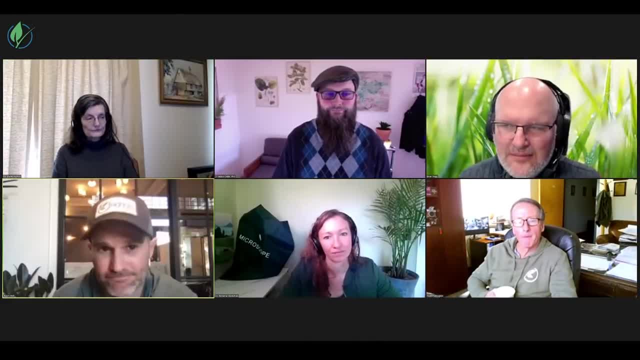 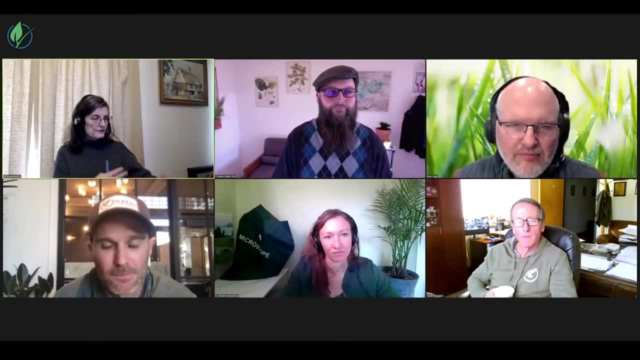 I agree. I think some low lying covers would be Yep. So we have a whole list of things that we've been working with, and people are starting to show which ones are the best for their kind of land- Dichondra repens, which is the 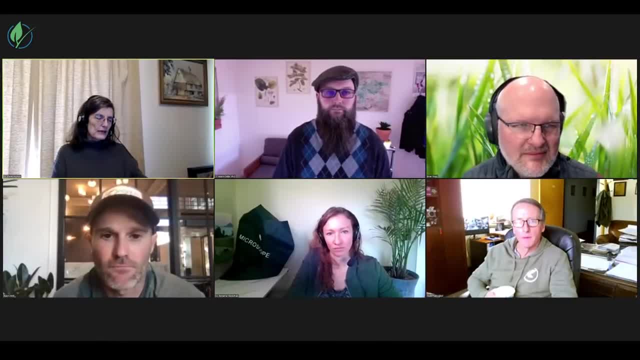 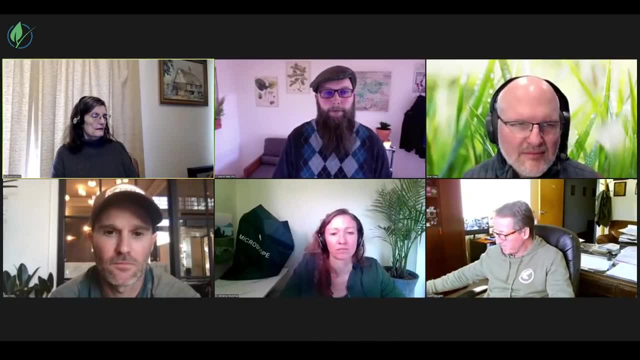 temperate dichondra, not the tropical dichondra That's. that is a weed. You want to make sure you get the right kind of dichondra And because you have wet springs, the dichondra is going to grow. 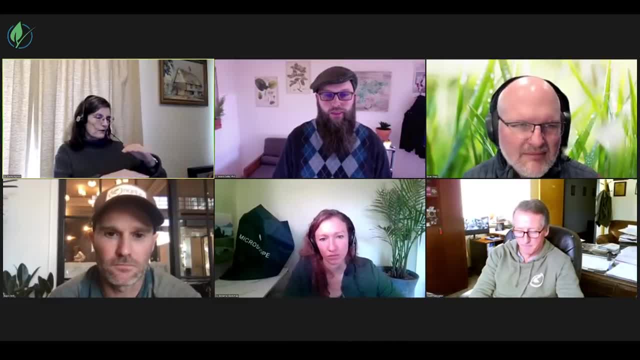 They're going to grow, They're going to be established, take over, but they never grow more than maybe, you know, three to five inches, and that's it. So they're self-seeding. when they make seed, They maintain themselves over the years. Well, you want more diversity than that. So throw about 20 different plant seeds out there and get them established and they'll share the space and they'll give you lots of benefits. So try a small area This growing season, perhaps with a bigger mix of ground covers. 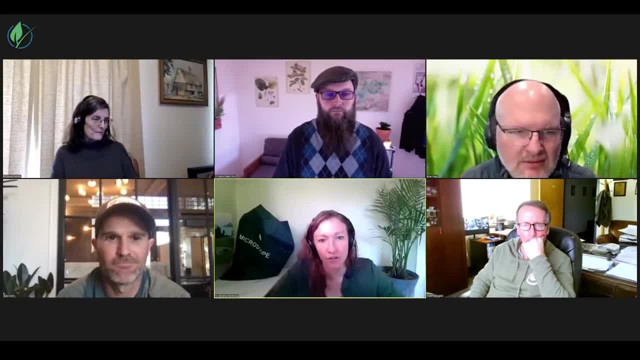 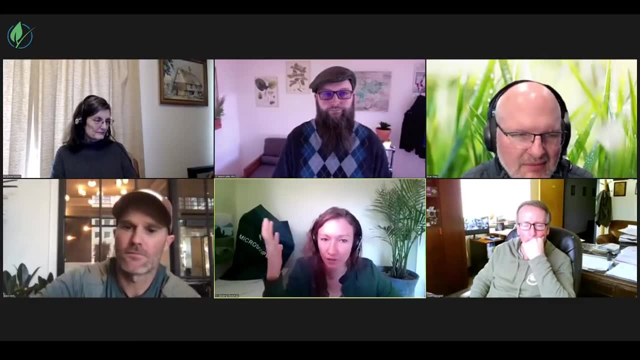 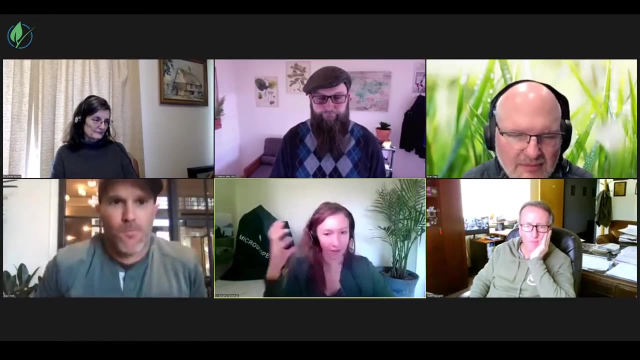 You know this is a really interesting area of ours to discuss and I'd love to also engage Todd and Adam and hear all of your thoughts about. you know, the goal here is just to keep those roots healthy and in the ground right and to keep our crops supplied with. 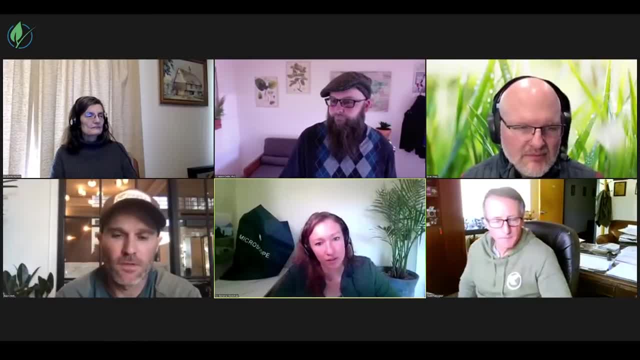 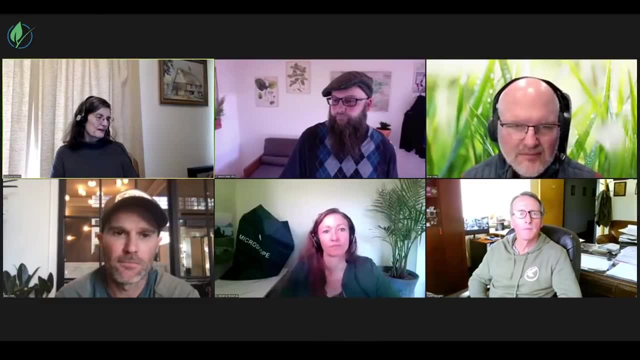 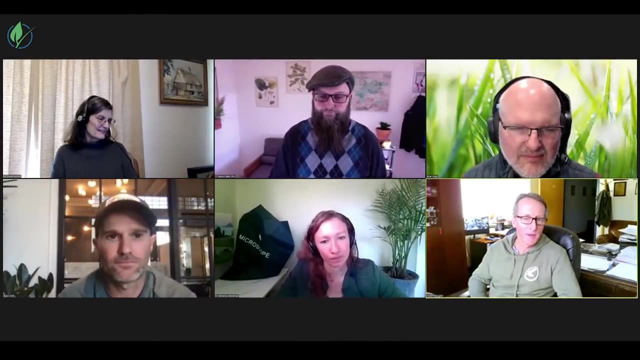 healthy structured soil and protect that soil surface. So I'd love to hear more about, for both of you, how you've been able to do that practically out there- Keep those nutrients coming. Yeah, cover crop technology is really advanced. Looking at you know even the exudates right. 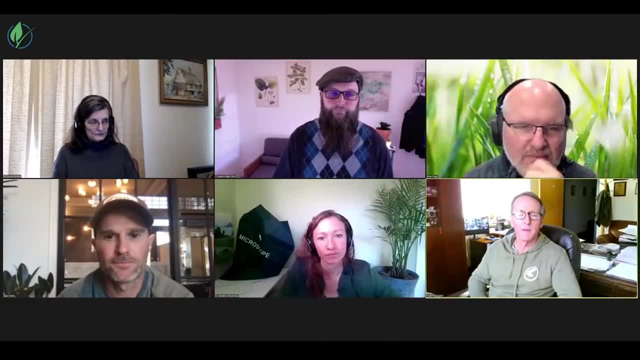 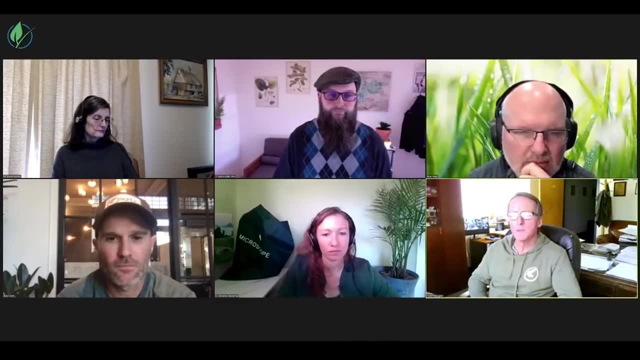 Elaine, the different exudates that are being produced by these different cover crops, how they benefit the biology and also the intended crop. I know, Adam, there was one of your fields that got flooded. You planted a lot of sorghum. 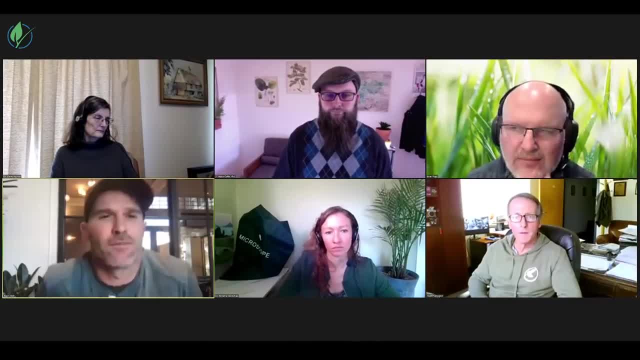 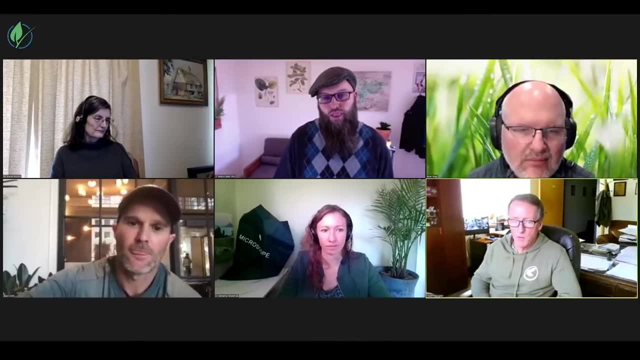 Yeah, that's right. Sudan sorghum: Yeah, yep, And we. I remember looking at the biology and we were lacking something. I don't know if it was protozoa or what, but after a season of putting that in, it really brought. 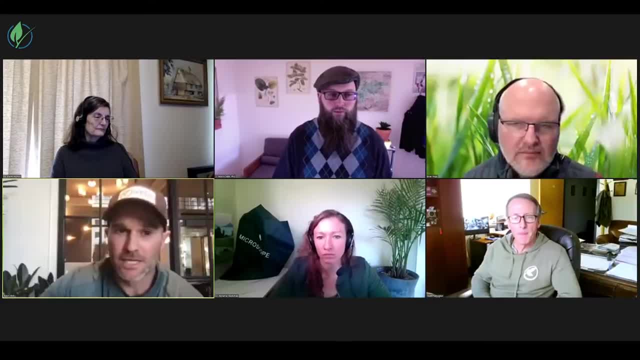 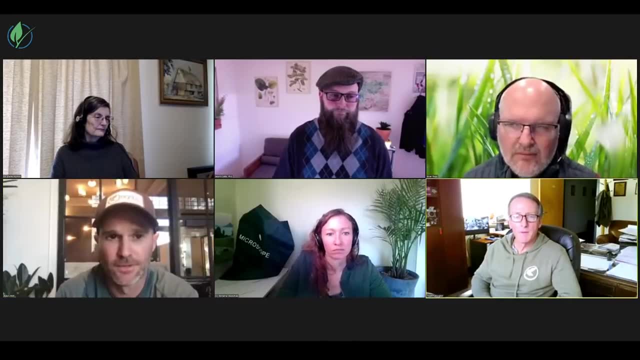 the biology back around. And then the season— We were seeing a lot of beneficial nematodes in it after just that one year, Right With the covers helping with that So— That was a flooded soil. That soil got really flooded. I mean you can grow anything. I. 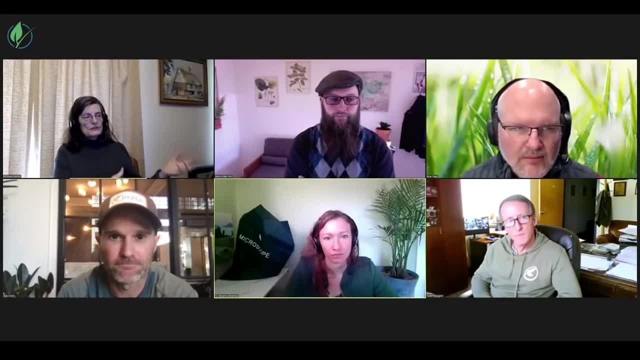 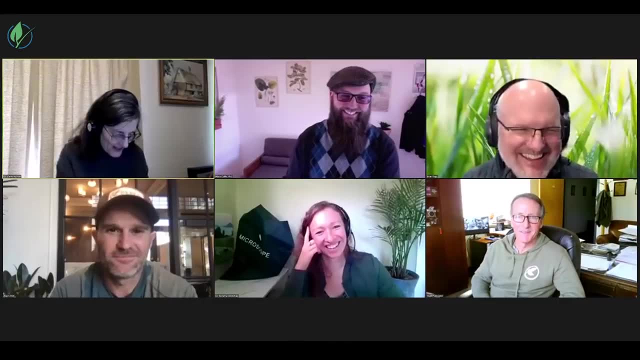 don't think on that. That's amazing, Yeah. And then, Todd, you need to be talking with Adrienne because she's a chemical ecologist, So she knows all of those. you know what are the waste products, What are the secondary. 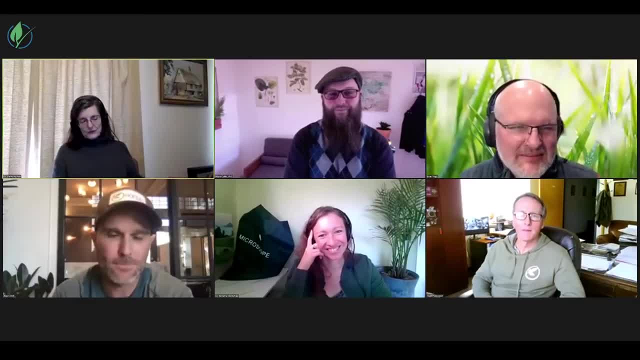 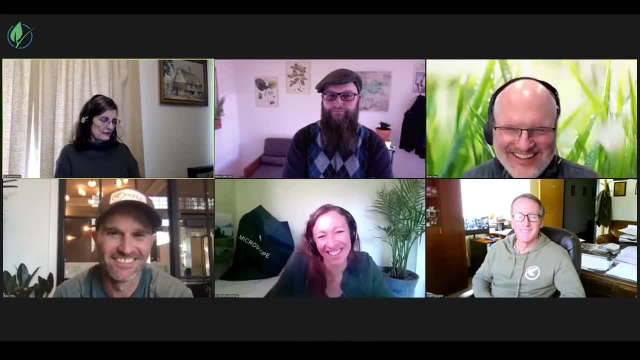 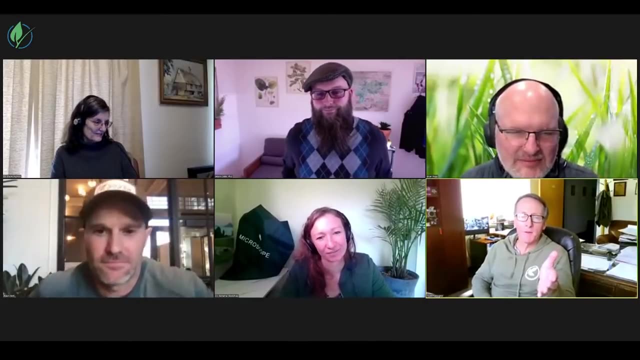 metabolites, What are the tertiary metabolites? And Adrienne gets talking to me about that and I'm kind of like, okay, I've had enough, I need to go digest for the next two weeks. Let's have another conversation. She's grinning and smiling, But hey, you know, it goes back to the original topic, Brian. 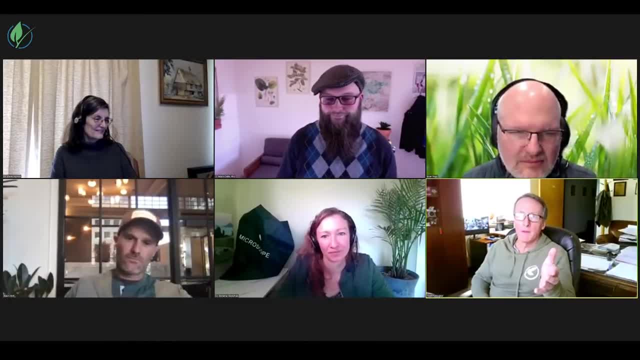 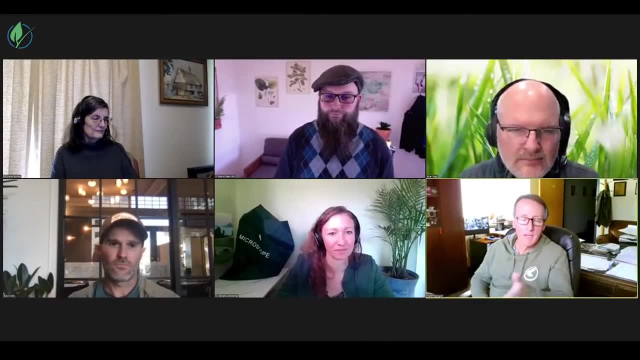 when we were talking about, you know the reason and the need to do the actual microscope work. Yeah, We wouldn't have known this unless we took samples and looked at it. But everything that Adam does, he always throws under the scope, you know, And that's really played. 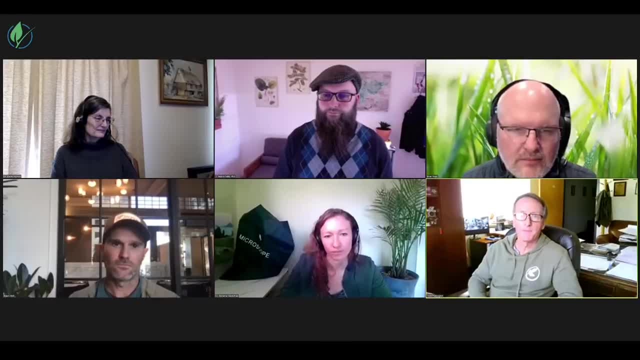 out really well, going forward on making decisions, For sure. You know, and it's interesting when I look at the regenerative ag space, you know this, you know what we're doing. like the soul food approach, it is an emerging 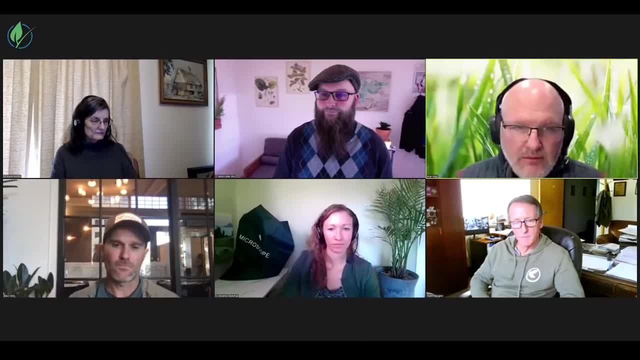 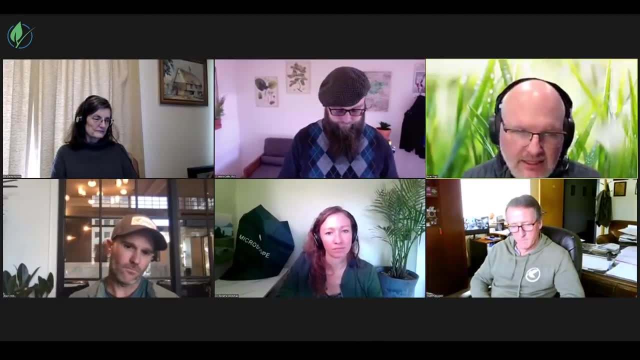 market. You know the science has been around for quite some time but to really start to transition large scale, it is really starting to gain momentum and starting to change And with that I am seeing a tremendous amount of new products coming on the market that are claiming to be 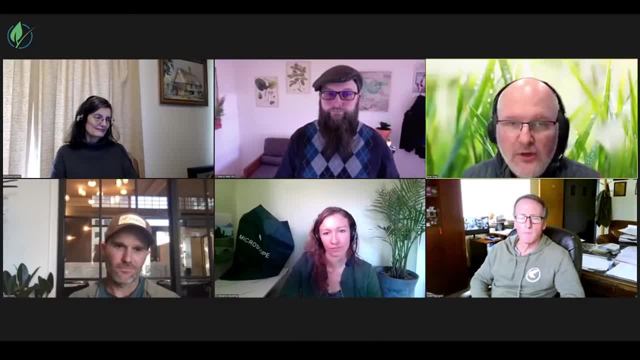 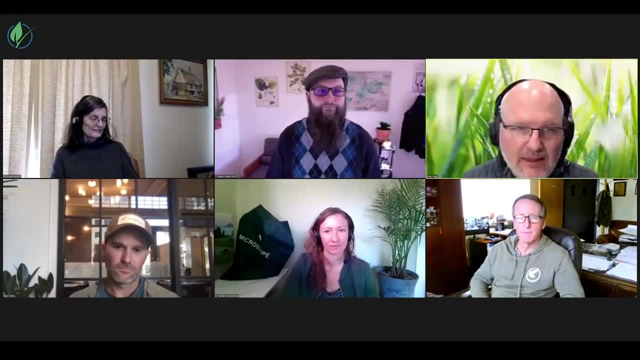 biological, And it's really hard for you know my growers, because I get constantly inundated. well, what about this product? The salesman's trying to sell me this. What about that, What about this? And I have a feeling the market's going to be in that little bit of a potential. 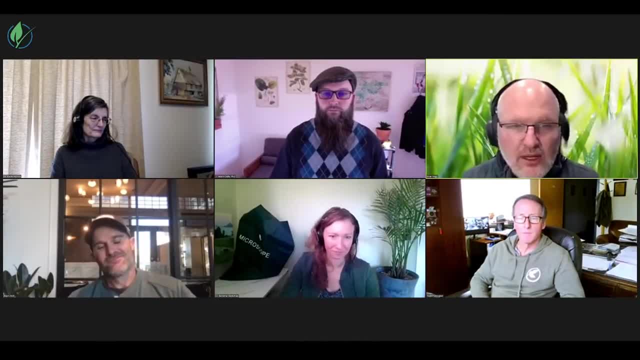 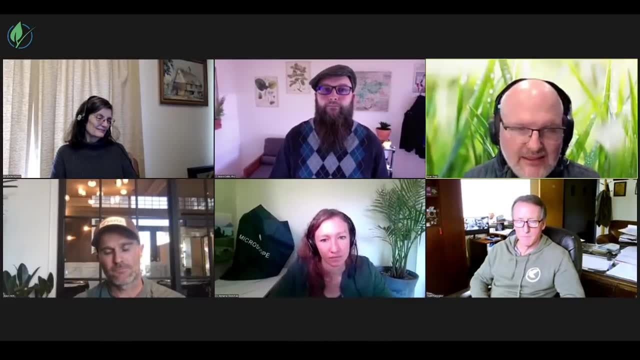 some snake oil salesman kind of stuff out that you have to really pay attention to. What we've been trying to do is really just set some consistency, some, you know, straightforward practices that really can help our growers and education, work with a microscope and getting 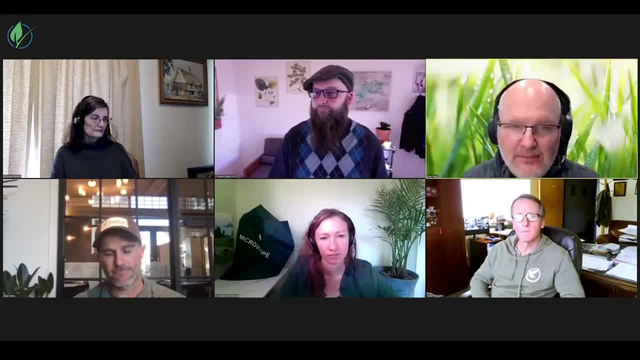 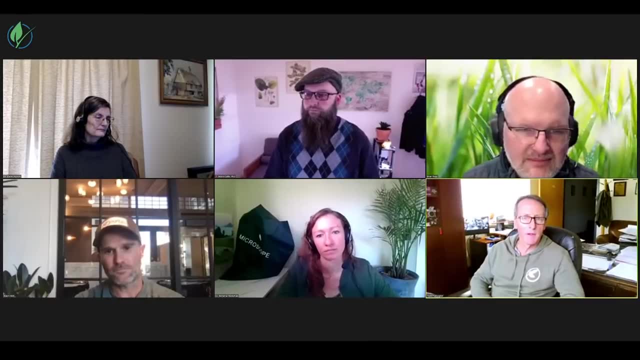 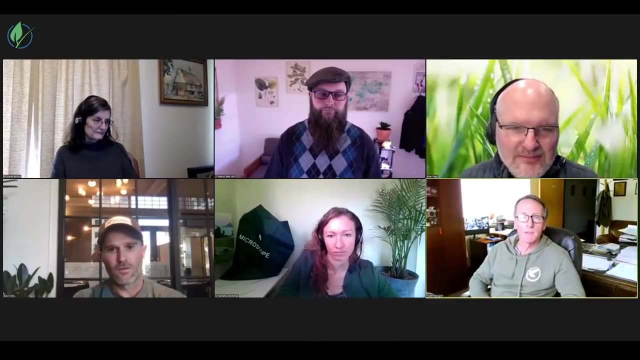 our farming community. educated in that space, I think will help tamp down some of that snake oil salesman activity that's out there. Well, that's interesting because a lot of the reason that Adam and Brad started AgroBio was because they were buying products from other salesmen and they decided to go directly to the 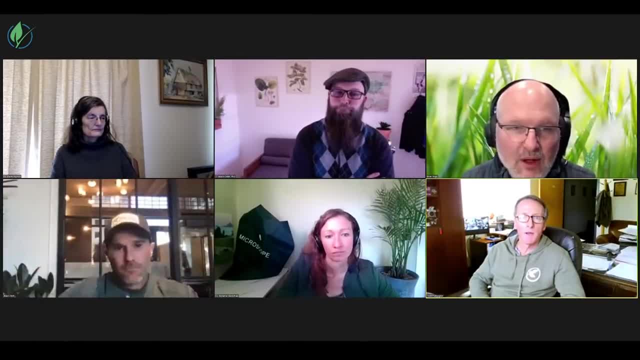 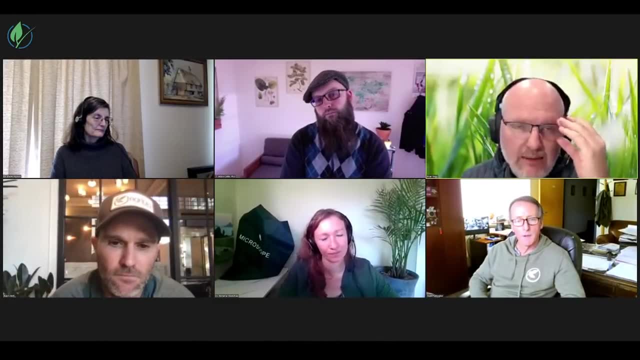 source and get the raw materials. So I'm sure Adam can talk a little bit about that. I'd say probably over half of my clients that I had already gone down the road of biological before I got to them. And then I go look at the products that they're putting on that are supposed. 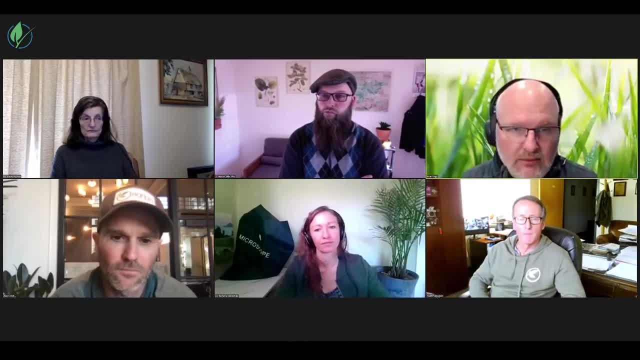 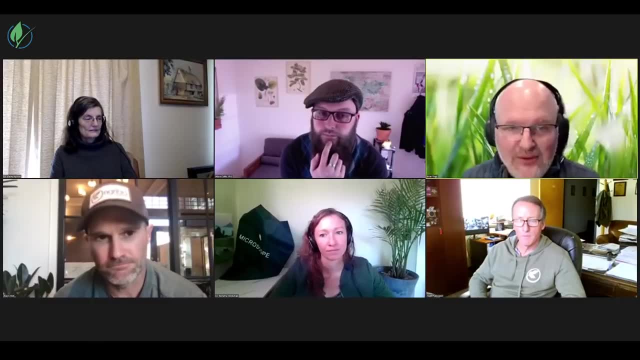 to be biological products. And you look at it and you're like, wow, there's, there's nothing in here, Maybe a lot of bacteria, but there's no fungi, no protozoa, There's nothing to make. constitutes a soil food web. And, like you know, it's kind of funny because Adam was saying: 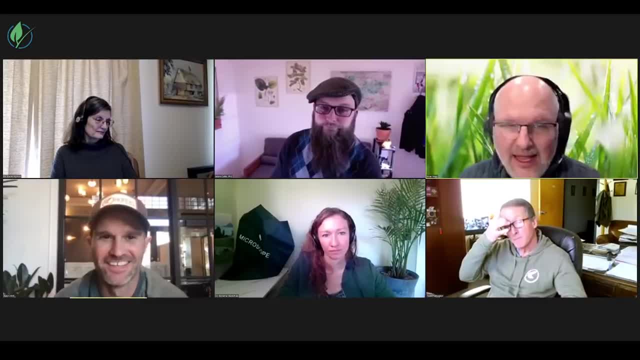 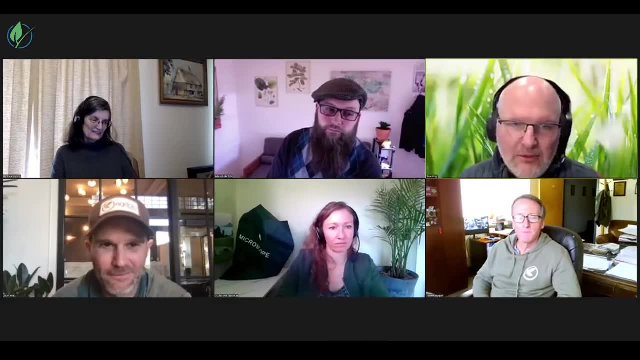 Hey, I bought a product, was probably suboptimal, but I did see a benefit And I see that all the time. where it's like, well, I applied this, I got something, you know, help control a little bit of powdery mildew. I helped do something, but it's like, okay, your potential is so much larger. 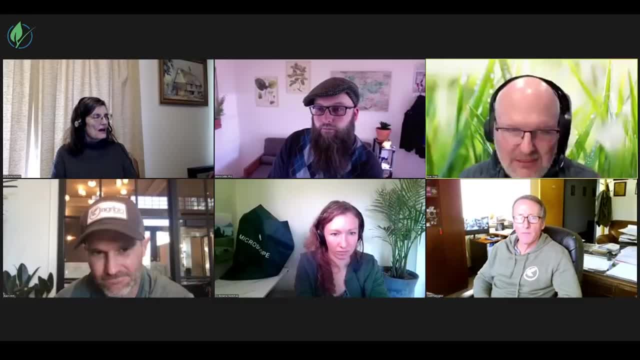 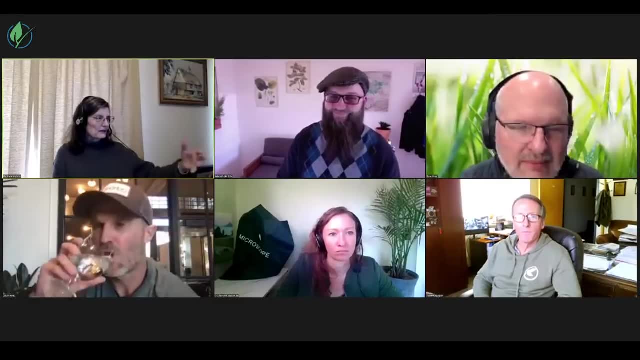 Let's really take a look at. you know how we can optimize. you know the microbiology in that soil And we don't, we really don't want to be bringing alien species that. you know. they isolated it in Pennsylvania And now here you. 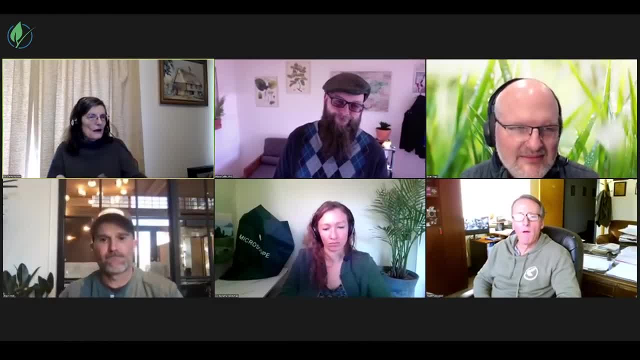 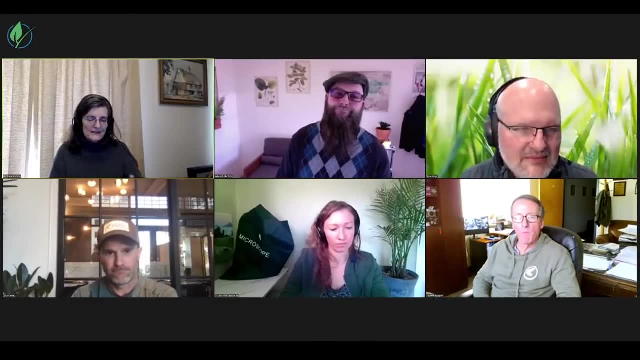 are in Illinois. Those aren't the right sets of organisms to grow in your soils under your conditions, with your crop species, And so you know you've actually when with that mixture you actually only put out a lot of food, perhaps to grow a lot of bacteria, but it got your. 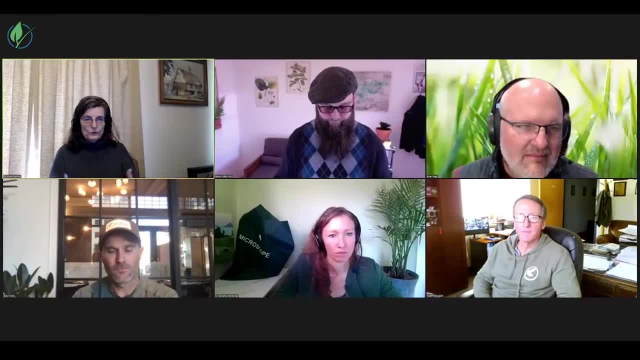 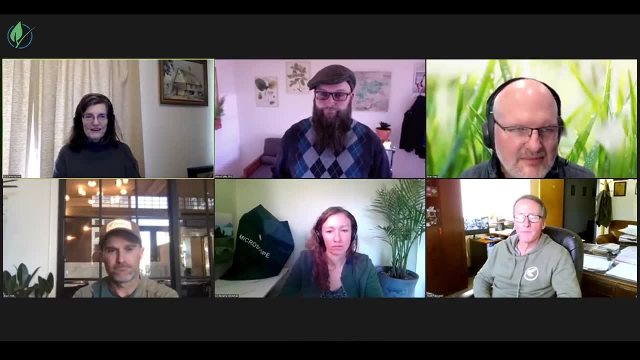 indigenous bacteria going And that was the real reason why it works so well. So, you know, really being absolutely sure about what's causing the benefit. Well, you know, we need to interpret things correctly And I don't think you can do that if you have no idea of what actually happened. 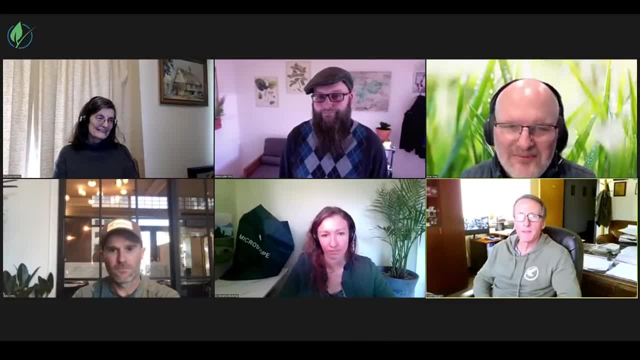 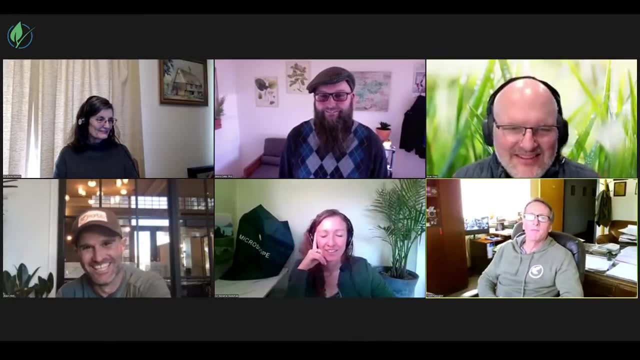 Well I got to tell you Adam's gotten pretty good at micro herding. I got his guys to start going out into the local indigenous environment And we have kind of a funny story, right, Adam? When I way back in the day we were looking for some. 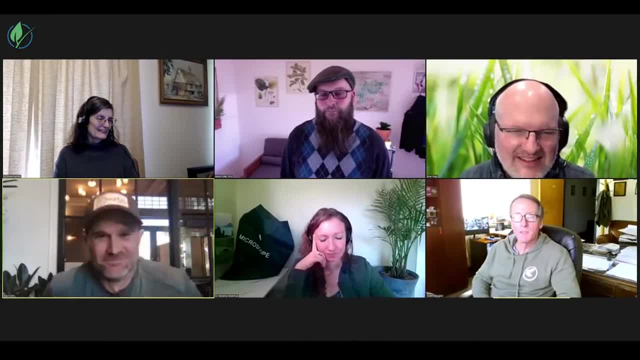 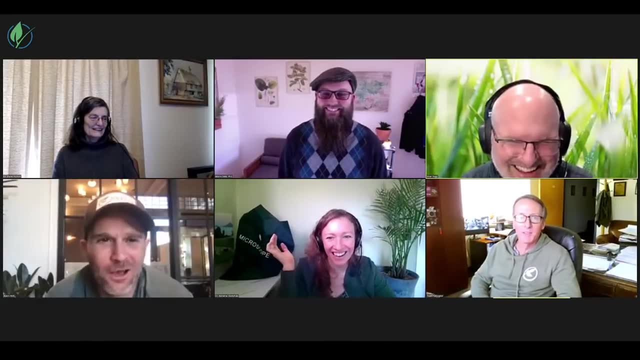 fungal foods. You know, you were like, well, I don't know where we're going to get wood chips. And then, you know, I turn around, look across the street and there's a big goddamn pile of wood chips. I had to walk down there and, sure enough, it's like holy mackerel I started digging into. 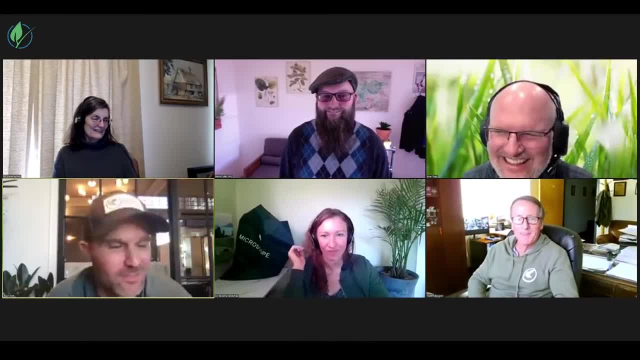 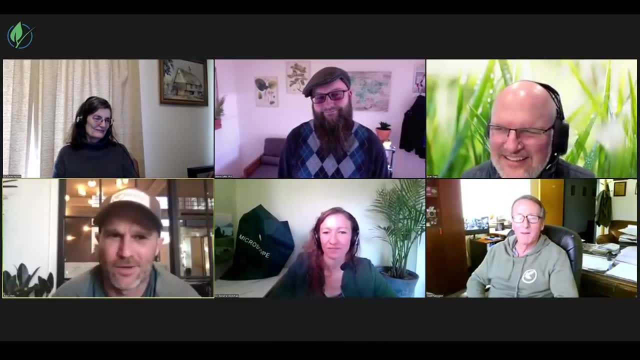 it right, Adam, And you're like, look at all this rhizomorph and all that you know. you're using all these terms that I wasn't really aware of. Tell me about this. I'm like, oh well. 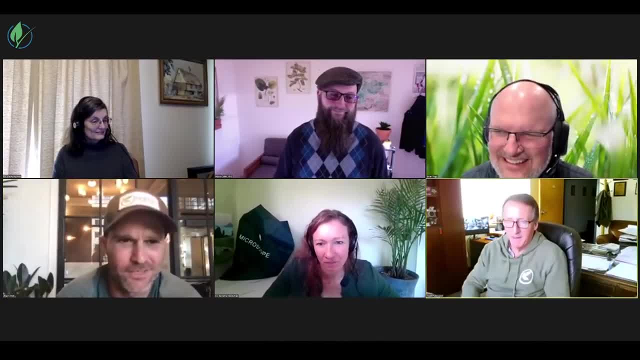 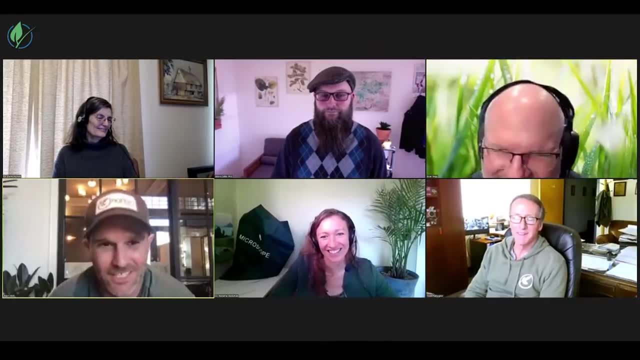 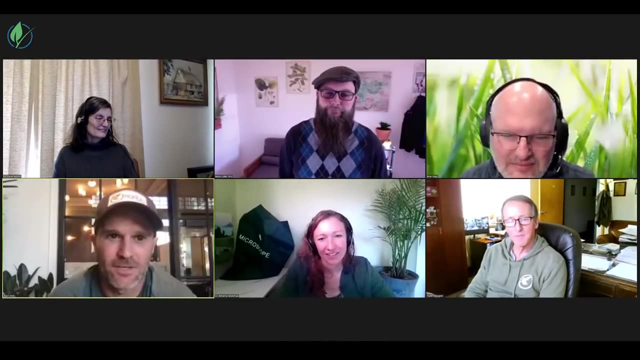 I just remember there was a guy that dumped wood chips down here about four years ago, I don't know. there they are. We've gotten pretty good about finding local sources because Todd's helped us. you know, and just you know, most everybody has them. You know, you just have to open your eyes to. 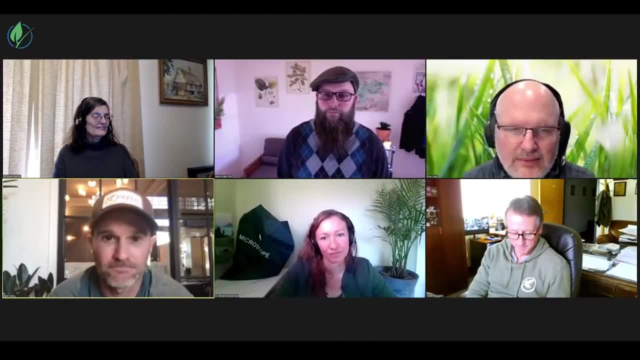 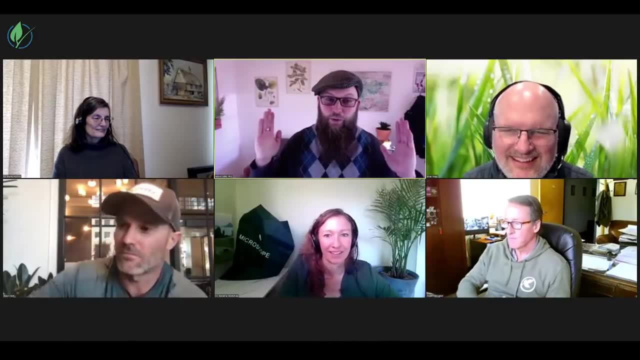 what you're looking for. at the end of the day, you know, And I do, I do feel compelled, as the mycorrhizal ecologist in the room to say I really hope people are cautious. you know, with mycorrhizal inoculum because I've been involved in research where we took 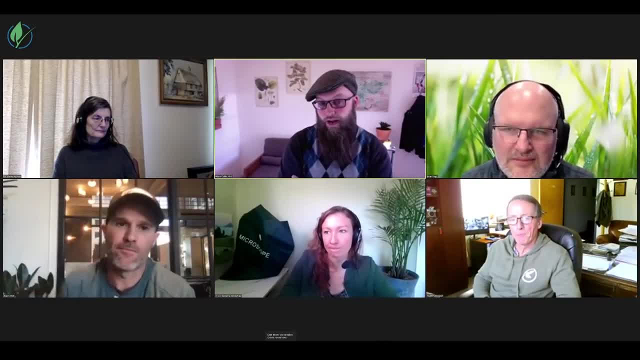 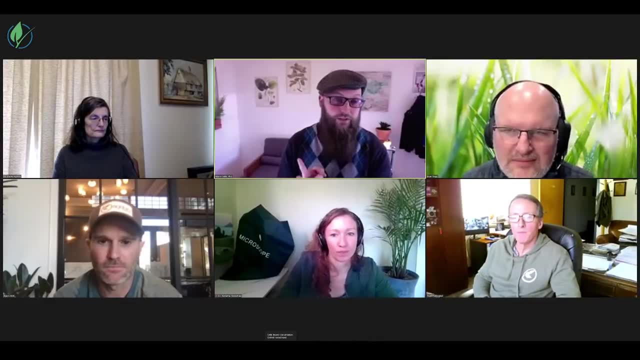 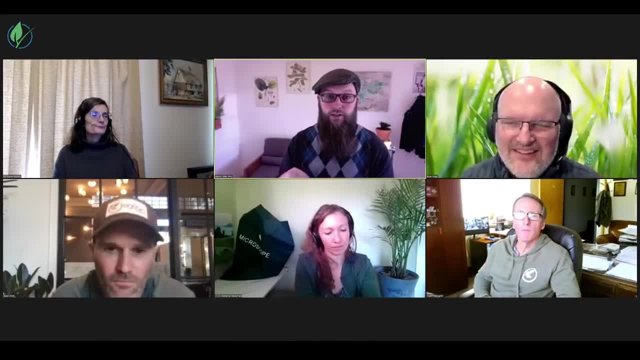 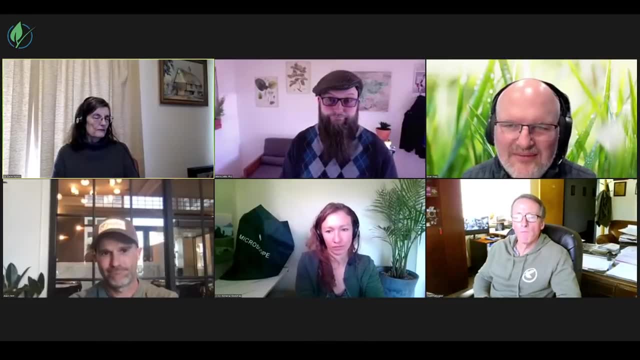 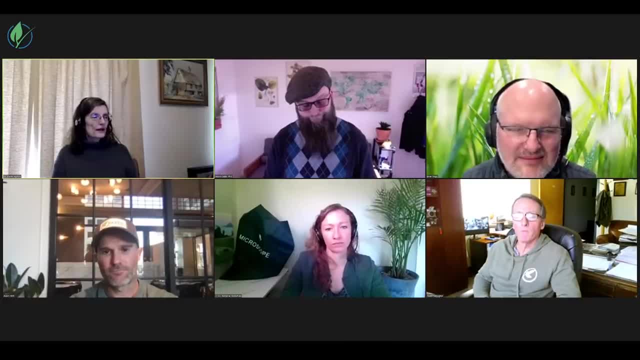 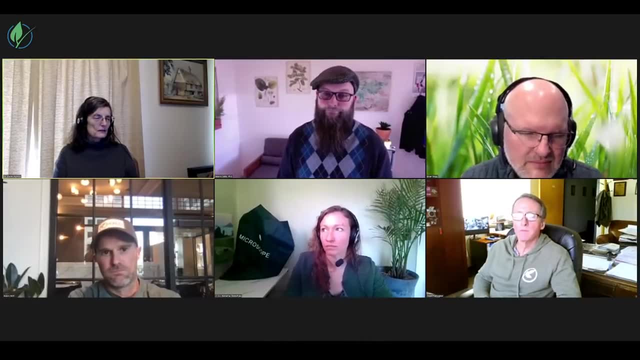 I think it won't. are we we're? we are we do. we are making some Chella inoculum. You know you're sick, champ. New Speaker. 1. And so you know there's a lot in it of nitrogen and phosphorous, and this is what it's about. anything in the water's. 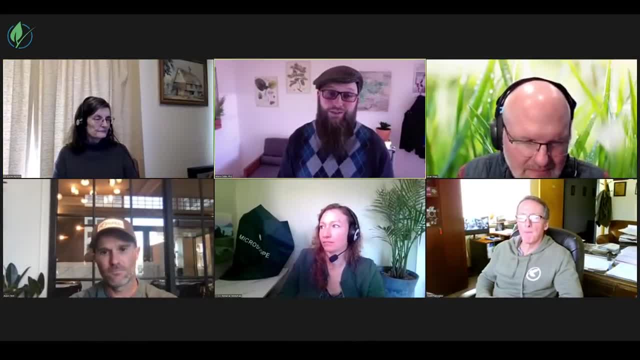 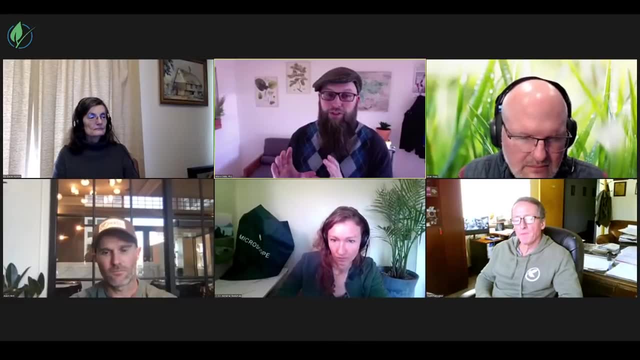 anything out there. They'reил new, too dangerous. them in here, like the barium column of parts coming out of Hurricane Laura's wild balls and all that. you know every region of the world. there's people that are um using methods to cultivate. 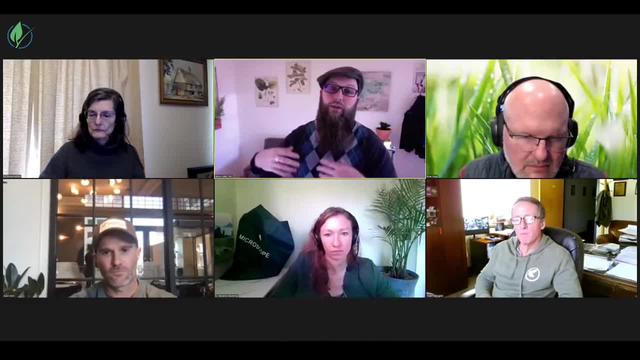 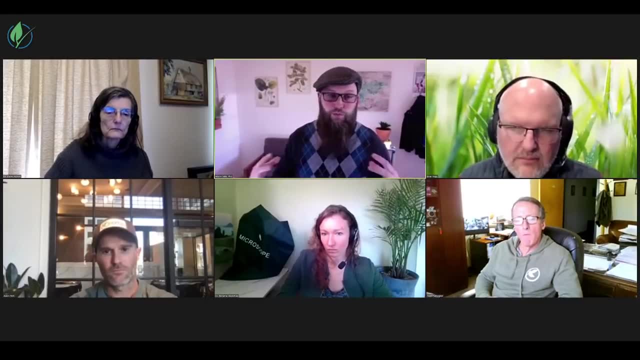 the native mycorrhizae from that area And that those become available because it's very powerful, along with everything else, When you reestablish the soul food web. those, those mutualistic partnerships, especially for grasses, are phenomenal. but don't put the wrong thing in there. 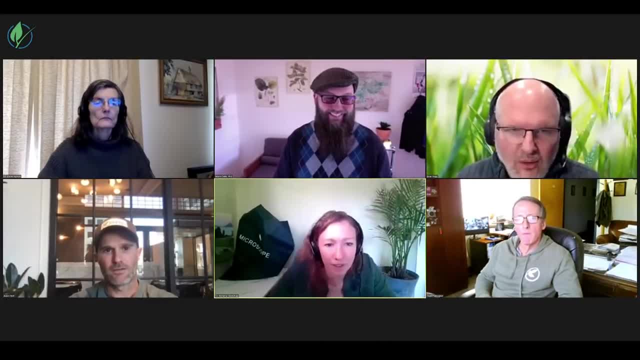 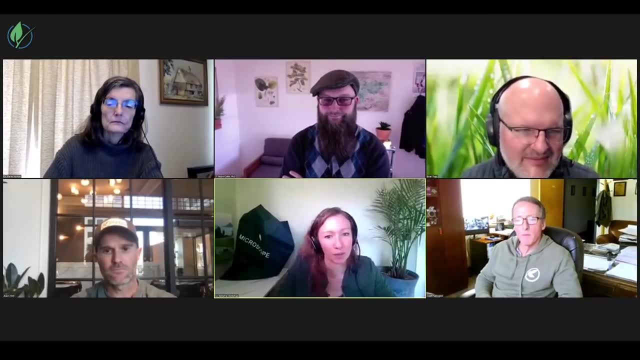 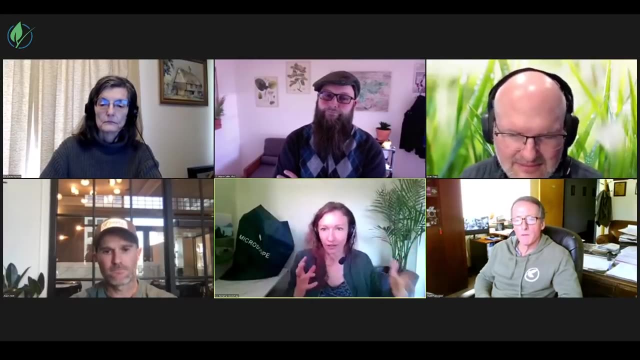 Right, Well, and I want to. I want to give a props real quick here, because I just think it's so incredible what Dr Elaine Ingham has created to be able to empower us all to take what's growing around us, create and understand how to create healthy compost. get that out onto the 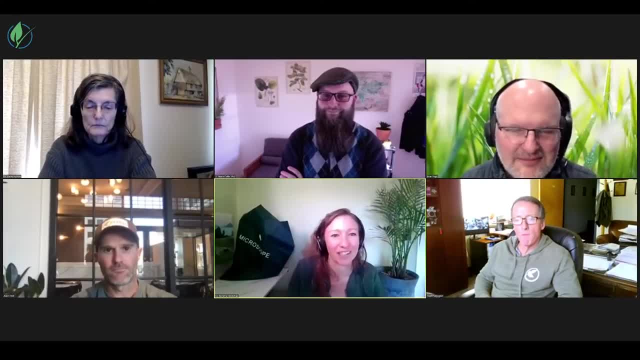 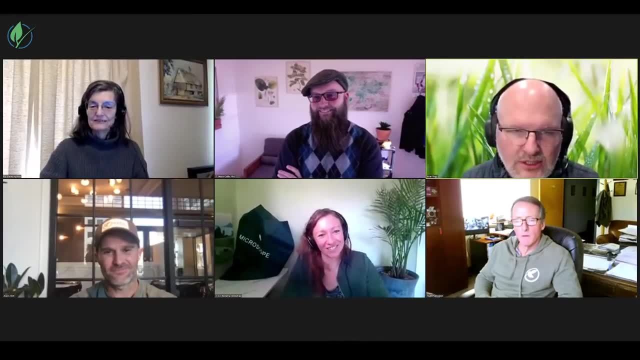 field and really start this movement. So thanks for doing what you do. Elaine Got it. Second, that, third, that Okay. Um well, we had a lot of great, great questions. I say let's move on to our next part of the webinar and we'll continue our Q and a at the end. 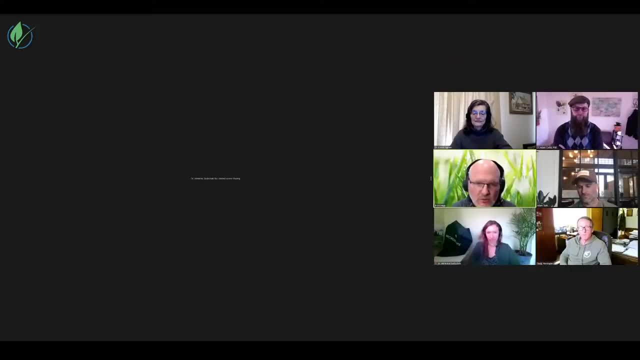 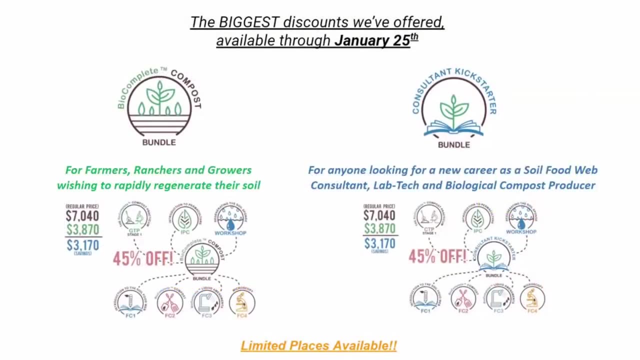 of our next section here. Um, so I think we're going to talk about our promotion that we have running, And so, uh, this is the biggest discount we've offered and it's going to be available through January 25th. So the timeframe is coming up shortly here and there are limited places. 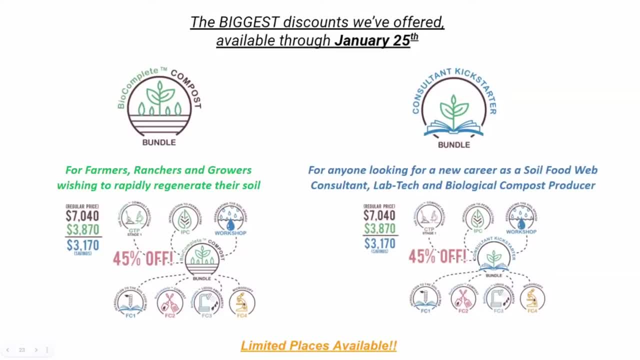 available for the promotion that we're running. And, uh, we're going to watch a video that's going to describe about our new bundle, which is going to be the uh bio complete compost bundle, And then we'll also talk about the consultant Kickstarter bundle. So, Adrian, if you want to, 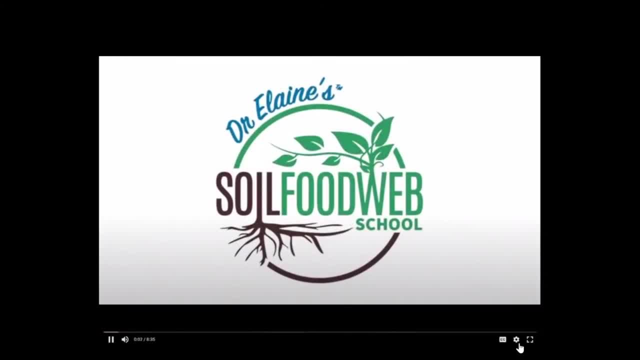 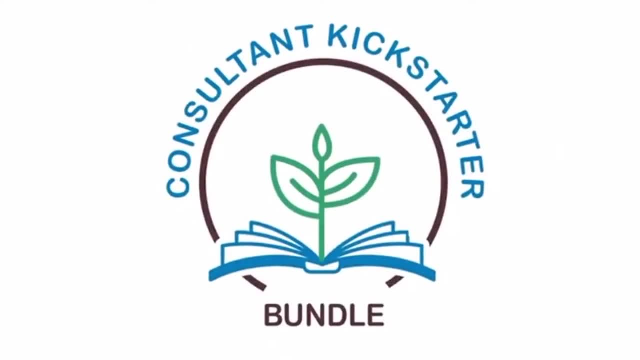 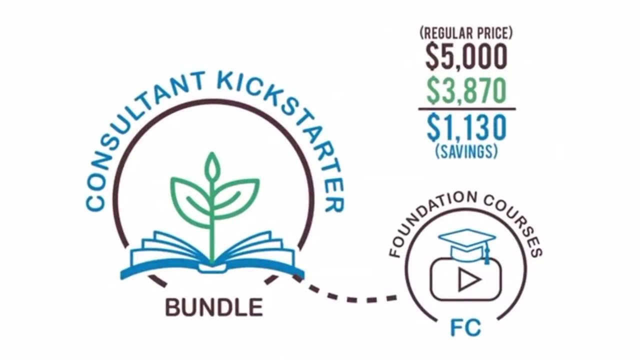 go ahead and kick that video off and panelists, if you go on mute. This month we're presenting our biggest bundle with the biggest savings. with the consultant Kickstarter bundle, You can register for the soil food web foundation courses with Dr Elaine Ingham for just 3870, saving over $1,100 through October 21st. You'll also get stage. 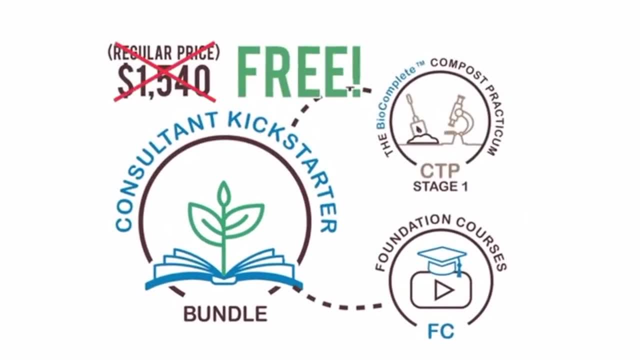 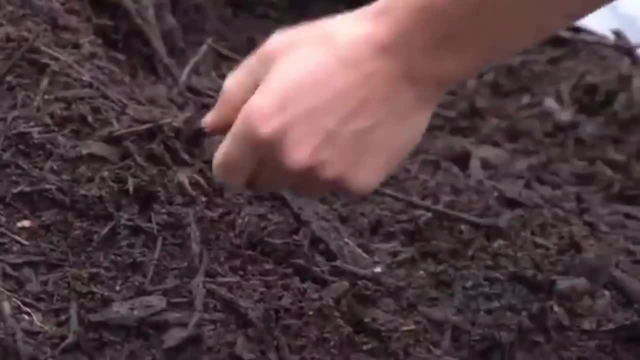 one of the consultant training program totally free, saving a further 1540.. That's 26, hours of mentor time dedicated to helping you make your own biological compost and develop your microscopy skills to the standard required to qualify as a certified soil food web lab. 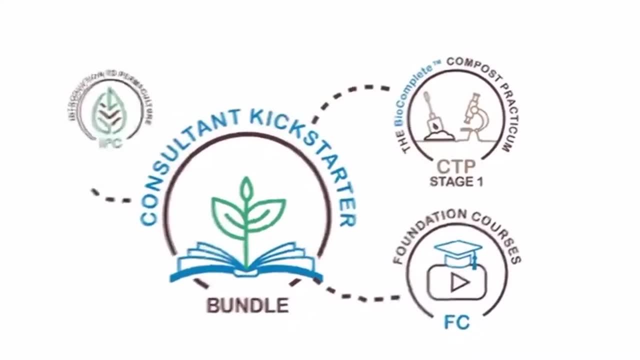 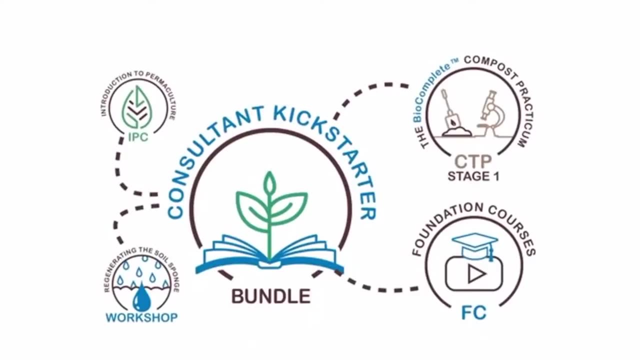 technician. You'll also get two free bonuses with this offer: the introduction to permaculture course by Graham bell and the all new soil sponge regeneration workshop with DD Pursehouse, saving a further $500.. This is the biggest discount bundle we've offered, with a total 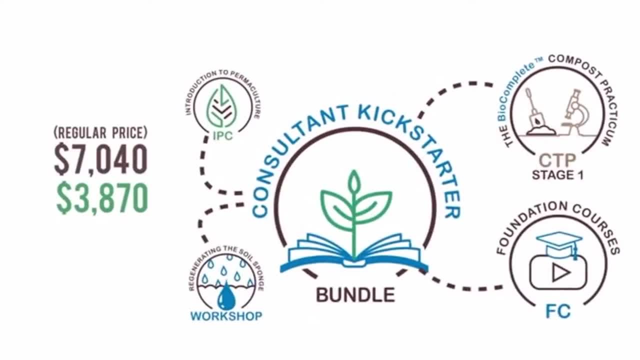 value of over $7,000.. For which you'll only pay 3870, saving you over $3,100.. That's 45% off. There are limited places available with the consultant Kickstarter bundle, So please don't delay In foundation. 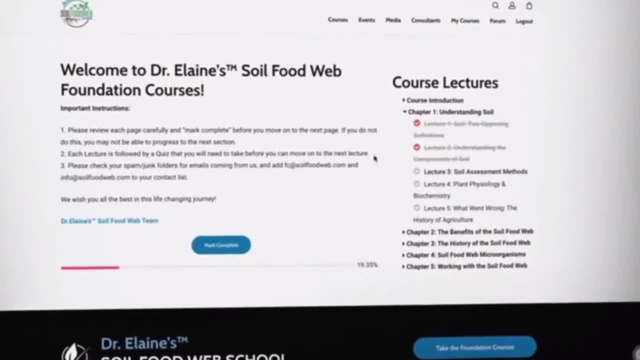 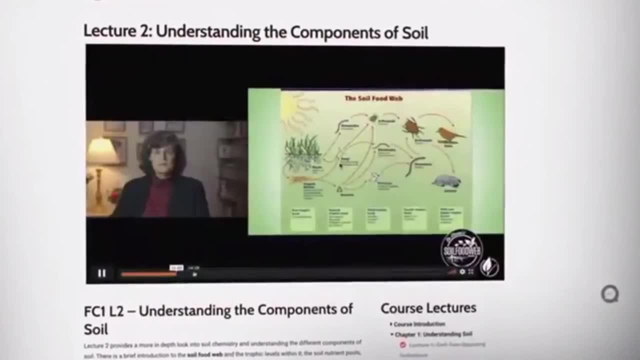 course one, you'll take a deep dive into the science and methodology that underpins the soil food web approach, which was developed by Dr Elaine Ingham. over the last four decades, You'll study the history of soil on planet Earth and how the agricultural practices. 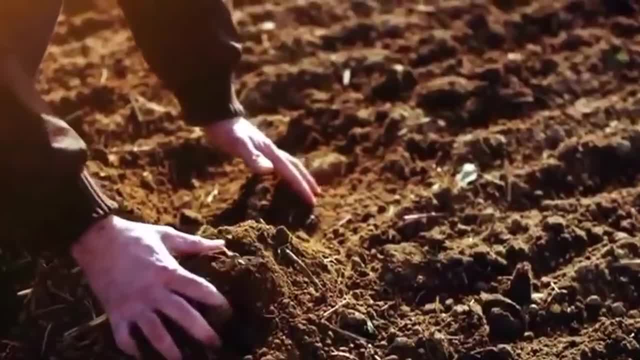 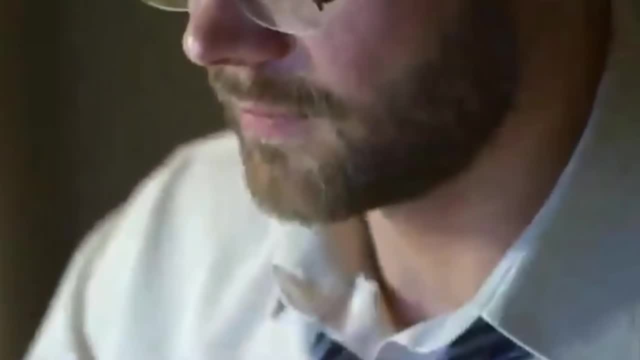 we've been using to grow and grow In the last hundred years have degraded our soils to the point where we now only have around 60 harvests left, according to the United Nations. You'll learn about the solution to many of the problems that are familiar to farmers all over the world today- Problems: 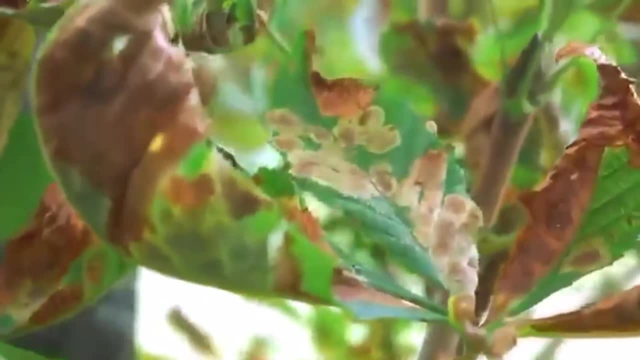 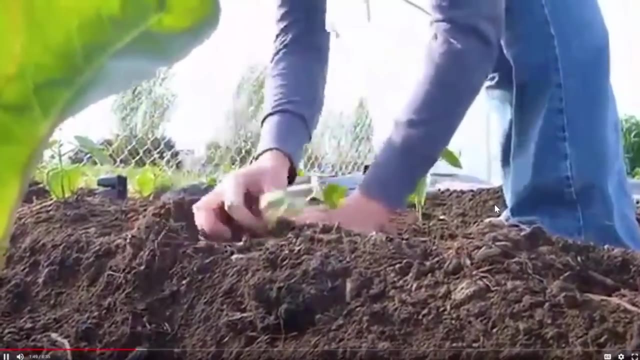 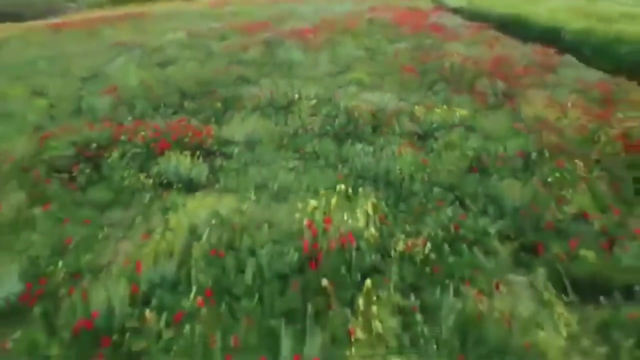 like diminishing soil fertility, pest and disease pressure, low crop yields, drought, flooding, compaction and soil erosion. Regenerative agriculture can address all of these problems. You'll be introduced to regenerative practices like no till and the use of cover plants. You'll also learn about the four major groups of 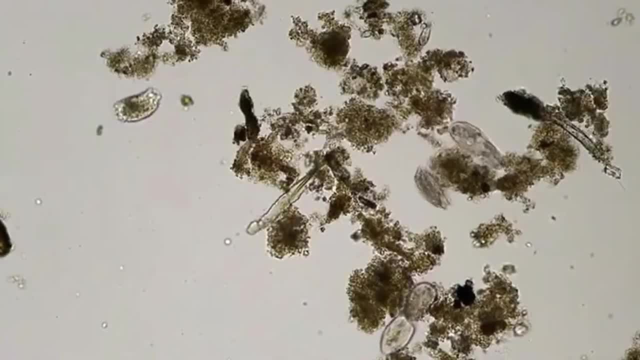 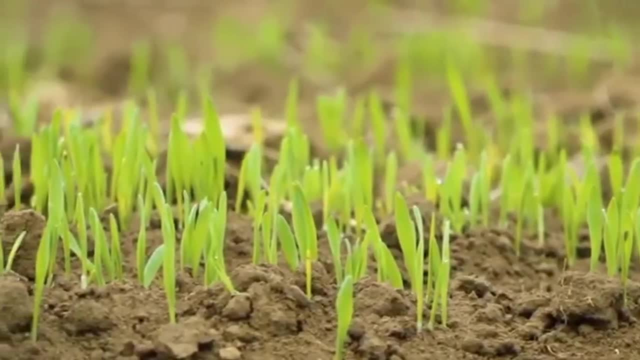 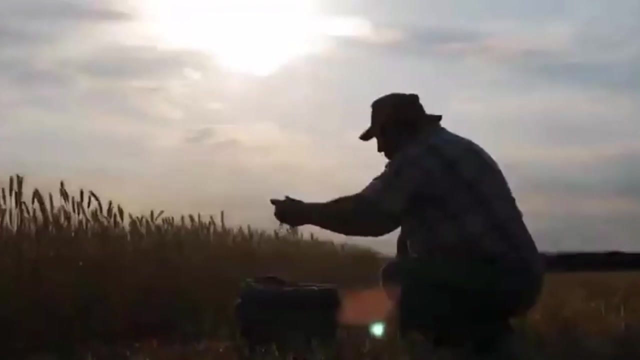 microorganisms that drive soil regeneration and how the process can be accelerated by restoring the microbial community, or soil food web, to your soil. Dr Elaine will present a number of case studies from around the world that she has worked on personally. Here you'll see some of the amazing results that have been achieved using. the soil food web approach, Dr. In foundation course two you will learn all about the characteristics ifotic County soils見 a trail down the road while trying a seed plant R тест my soils and see products in soil mellow mix. and these Vanity radicals are soon more workoutable as soil new available. 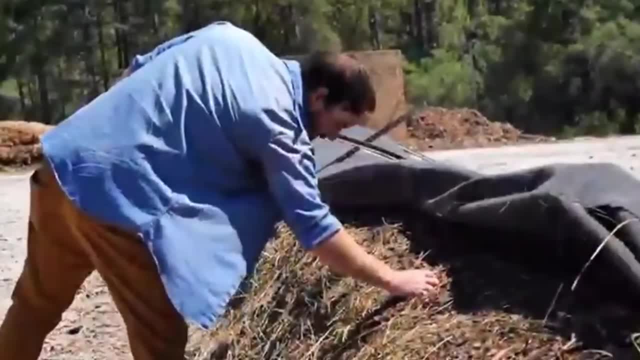 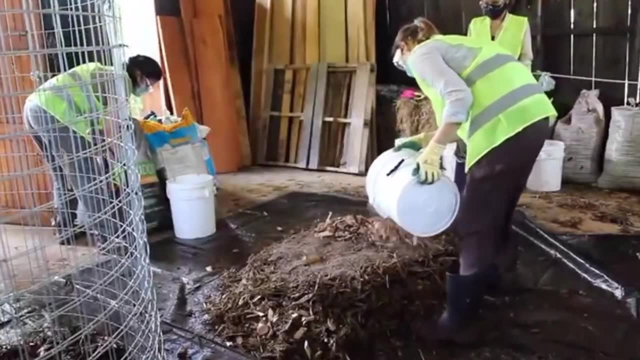 Bye, Joe, Anne, Yang, Simon, część, Jim. the importance of biological compost and how it's very different to regular compost. when most people look at compost, they only see a means of delivering nutrients to their plants, so they think about how. 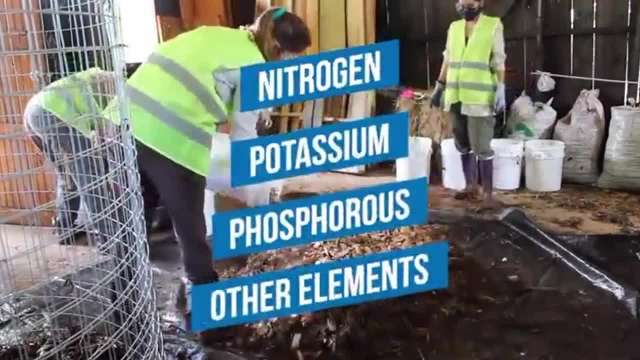 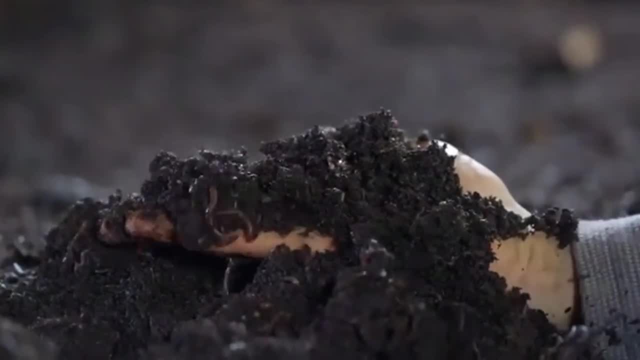 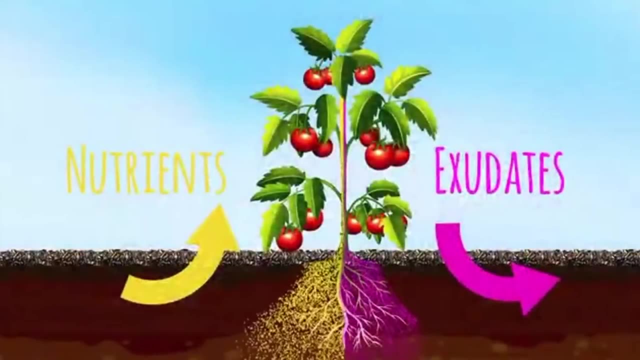 much nitrogen, potassium, phosphorus and other elements are in the compost. when we look at biological compost, we see a means of inoculating the soil with beneficial microorganisms so the soil ecosystem can start to function again, providing plants with a continual supply of nutrients. this is kind of like teaching someone to fish so they can feed themselves for life as. 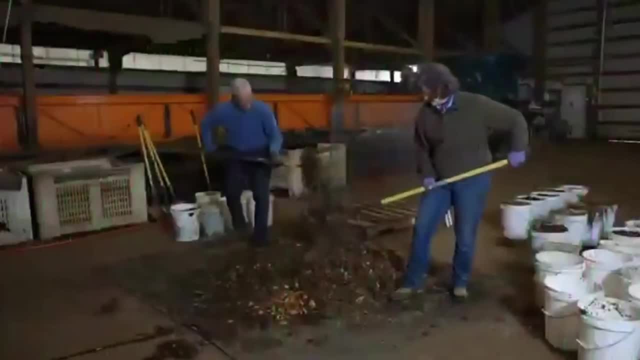 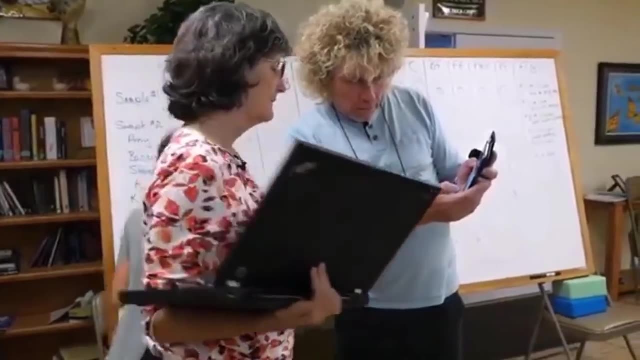 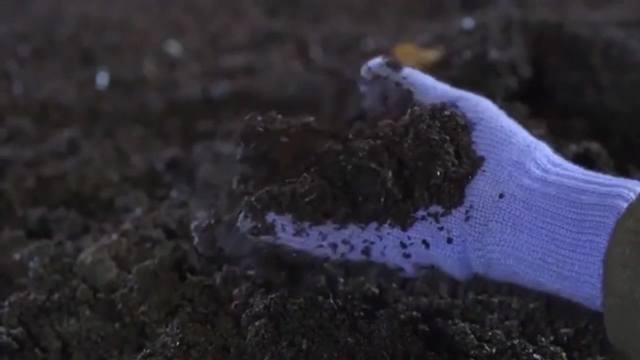 opposed to just giving them a single meal. in this part of the training, you will learn how to make biological compost using various starting materials to create a recipe that will produce results. you'll learn how to monitor and control moisture levels, aeration and temperature in order to ensure that beneficial microorganisms are multiplied while disease-causing organisms. 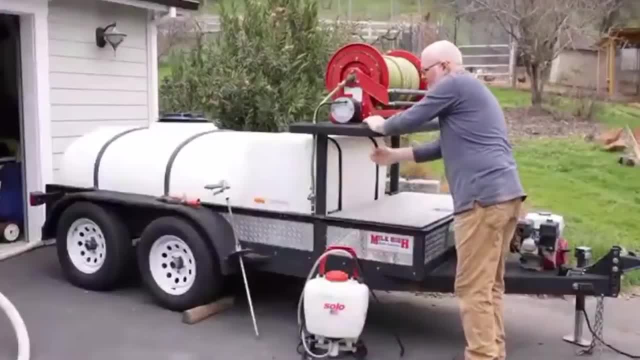 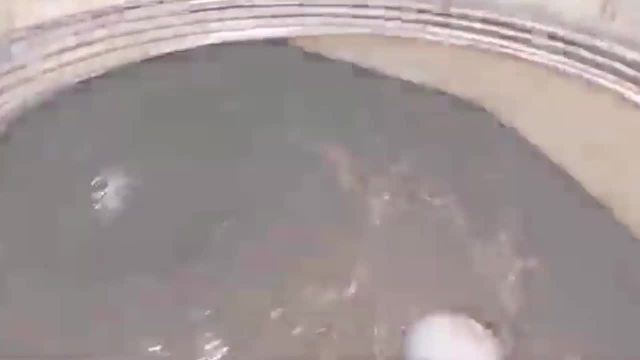 are destroyed or become dormant. you'll also learn about the various types of equipment that can be used at different scales, and you'll learn about the different ways in which biological compost can be applied to the soil. in foundation course 3, you'll study dr elaine's 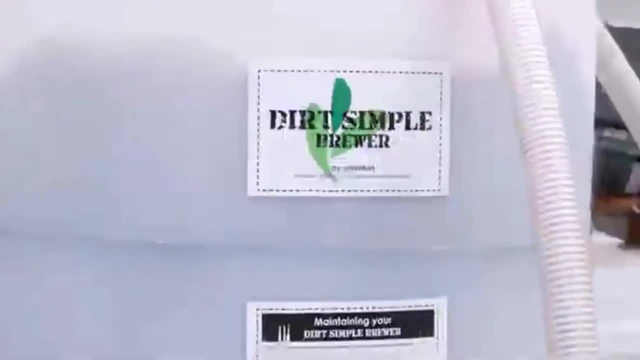 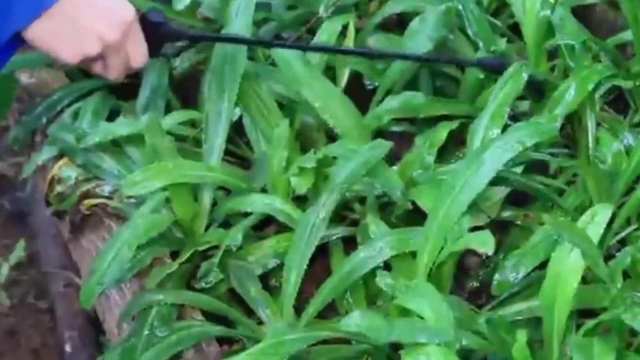 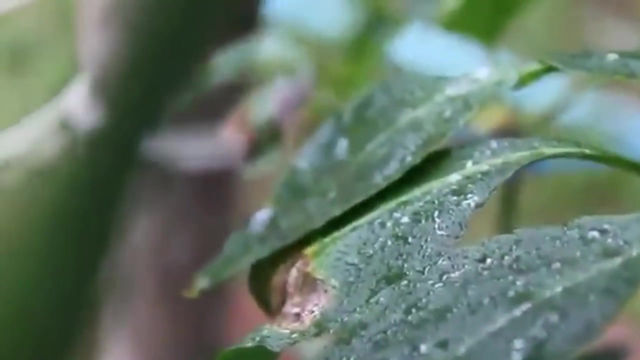 methods for making liquid biological soil amendments. compost extracts are used as a soil drench, delivering microbes deep into the soil profile where they can interact with the plant's root system. compost teas are applied to the plant's foliage, where they form a protective barrier against foliar diseases. in time, as your plant grows, you'll learn how to make compost. 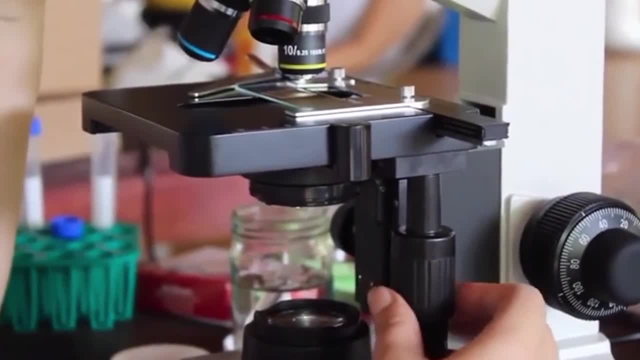 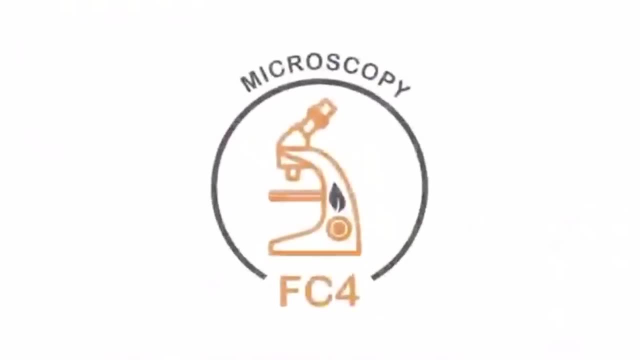 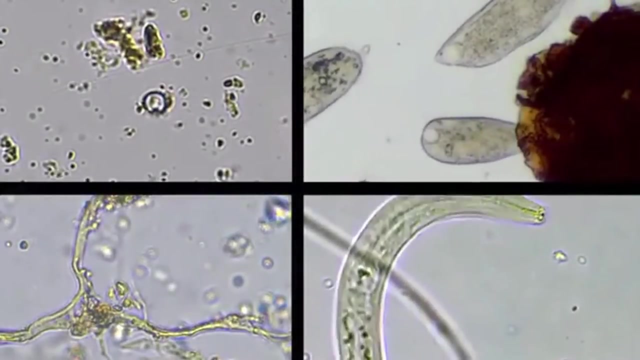 as your soil biome becomes more diverse and vigorous, your plants and trees may be entirely covered with beneficial microbes without having to continually apply them. in foundation course 4, you'll focus on four major groups of microorganisms in the soil: food web, bacteria, fungi, protozoa and 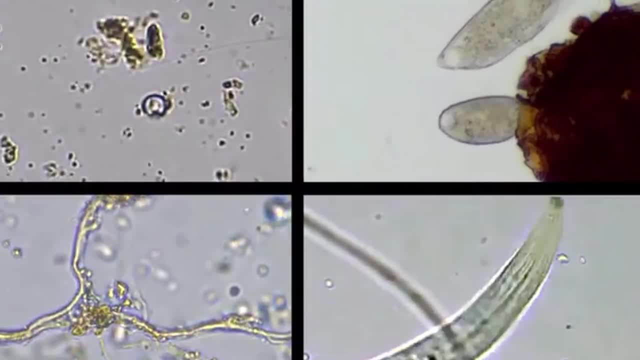 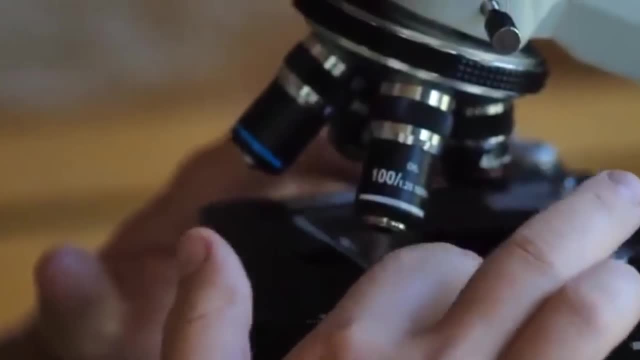 nematodes. you'll learn how to use a compound microscope to identify and quantify these microbes so that you can really see what's going on in your compost and in the soil. this will give you the ability to monitor the quality of your compost and liquid amendments before you invest all the 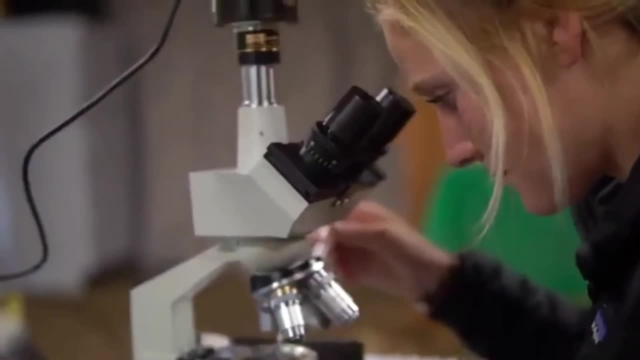 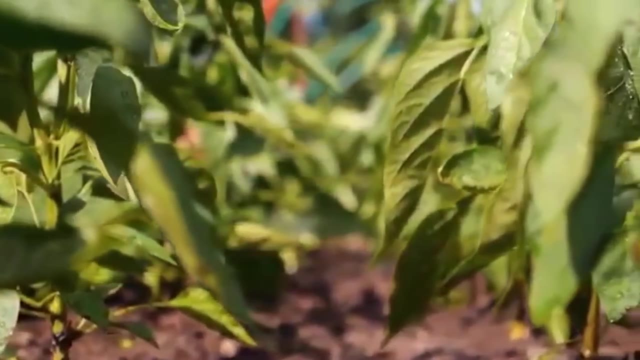 time and effort that is required to apply them to the soil. you will also be able to monitor the progress of the microbial community in your soil over time, so if something is going wrong, you will know about it before the plants start to suffer. this gives you the opportunity to take remedial. 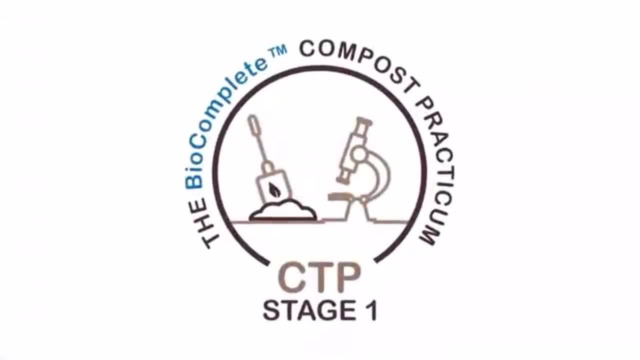 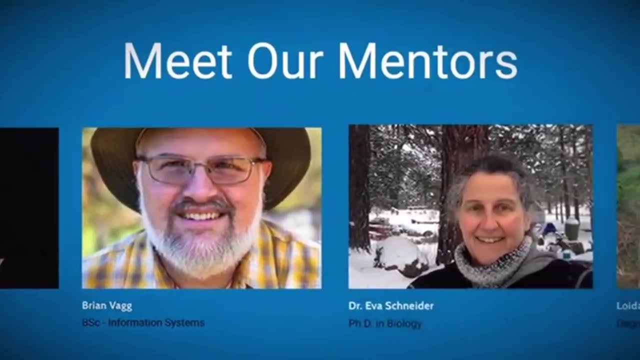 action early on in the growing season. in stage one of the consultant training program, you'll be assigned to one of our highly skilled mentors, some of whom are soil food web consultants who run their own businesses supporting farmers to make the transition to the soil food web approach. 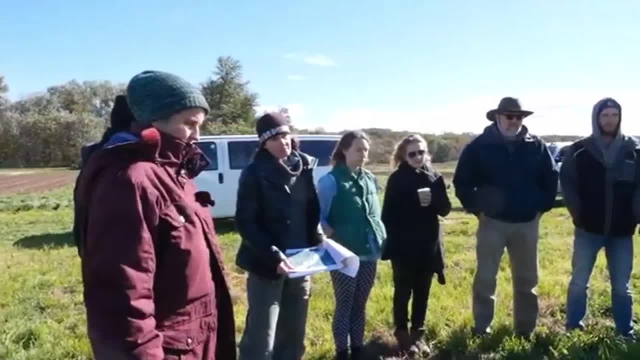 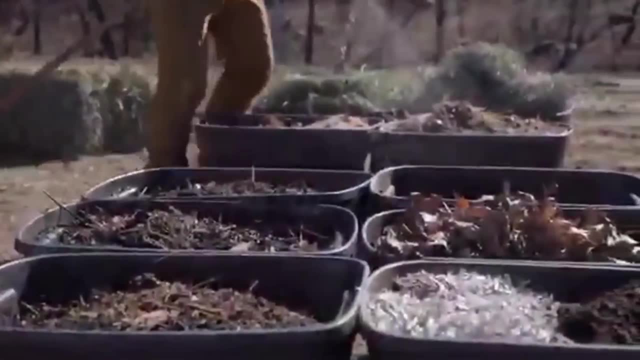 and others are phd biologists who have been working closely with dr ingham for several years. you'll work one-on-one with your mentor to develop your compost making and microscopy skills. when it comes to making great biological compost, there are many variables and every situation is 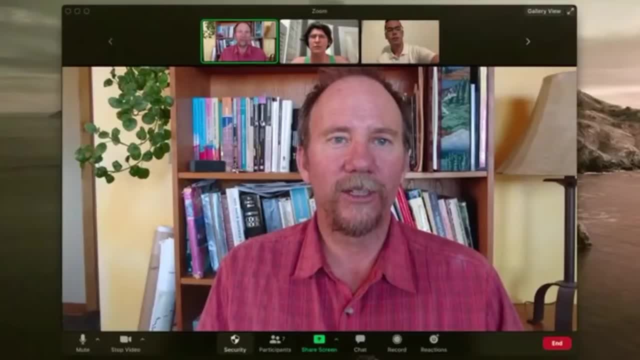 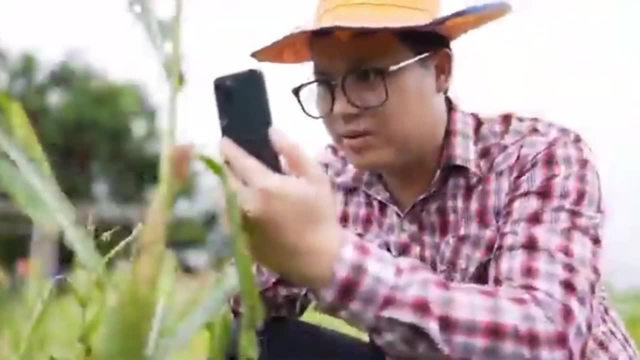 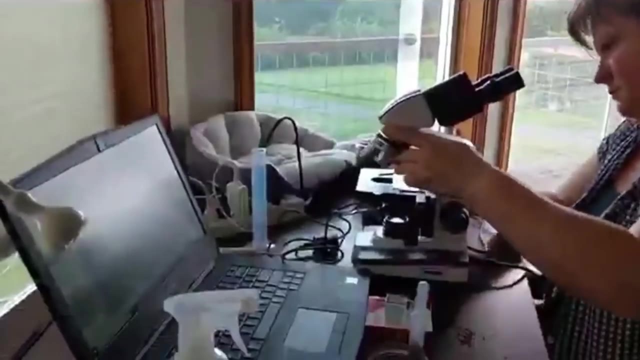 different. our mentors have worked with dozens of students making compost in many different conditions, so they'll be able to help you address some of these challenges that are unique to your location. they'll also guide you to avoid making common mistakes that can cost you lots of time, money and effort. your mentor will support you as you develop. 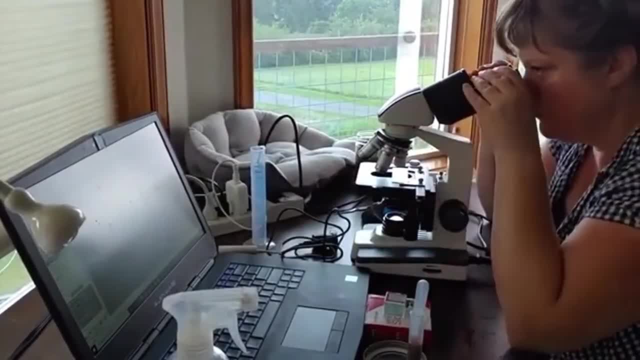 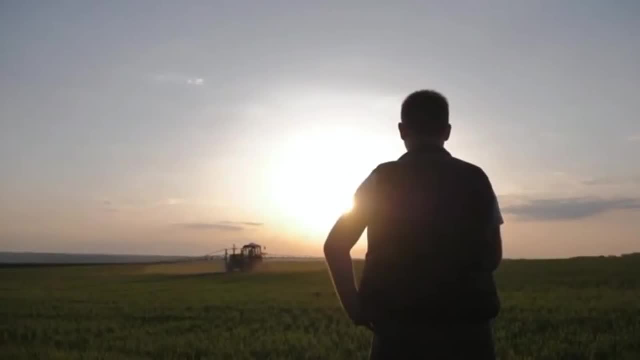 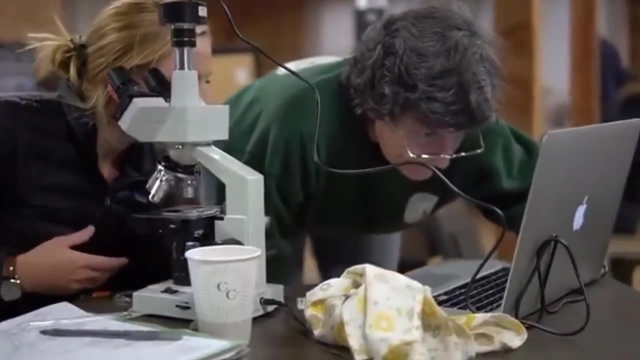 your skills to the required standard to pass the microscopy proficiency assessment. achieving this standard will give you the confidence to really know what's happening in the microbial community in your compost and soil. you'll be able to identify and quantify the four major groups of microbes in the soil in about an hour or less, once you successfully 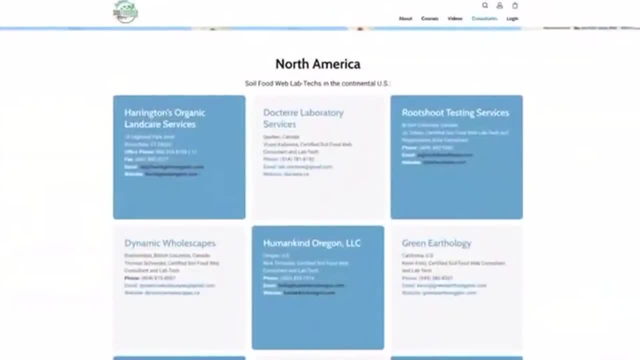 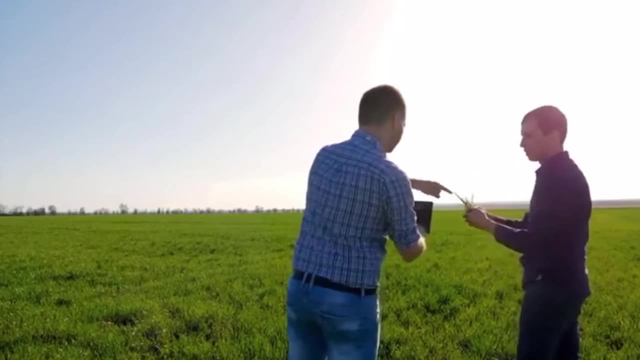 pass the microscopy proficiency assessment, you can elect to be listed on our website as a certified soil food web lab tech, which means that you can assess soil samples for other farmers and growers in your region. you'll have a total of 26 hours of mentor time so you can arrange zoom calls and 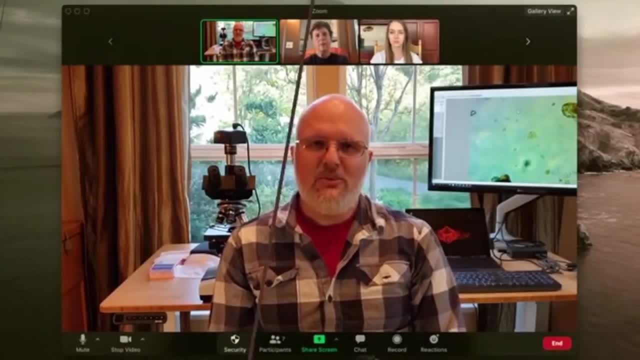 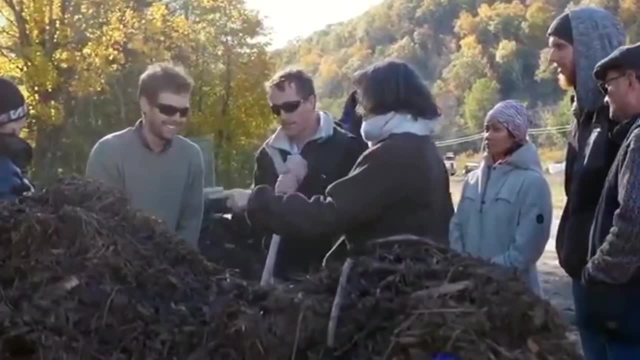 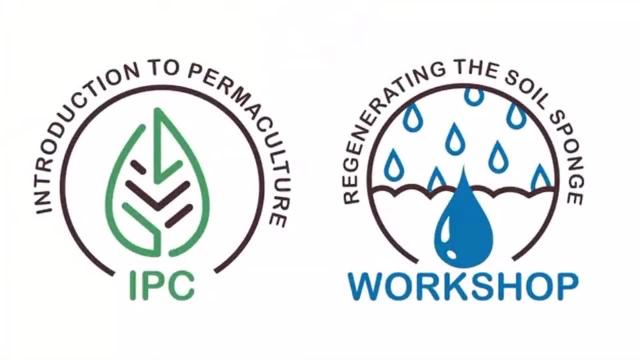 exchange emails with your mentor whenever you feel you need help. our mentors work together as a team and there's lots of diverse experience and knowledge between them, so you'll have access to a great deal of support. your also have access to the two bonus courses in the introduction to permaculture course. 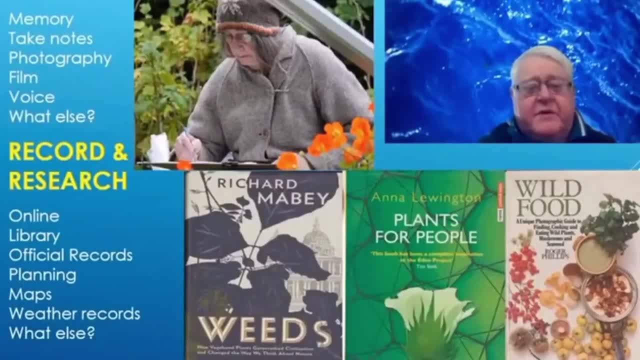 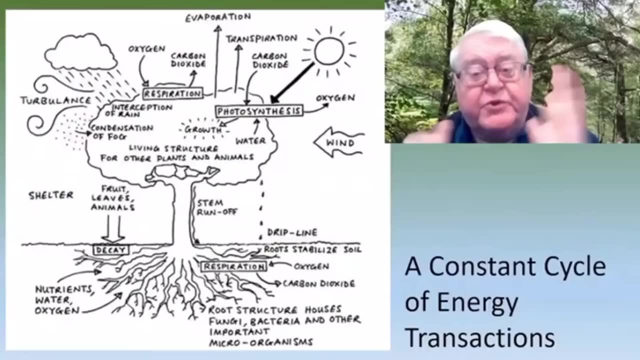 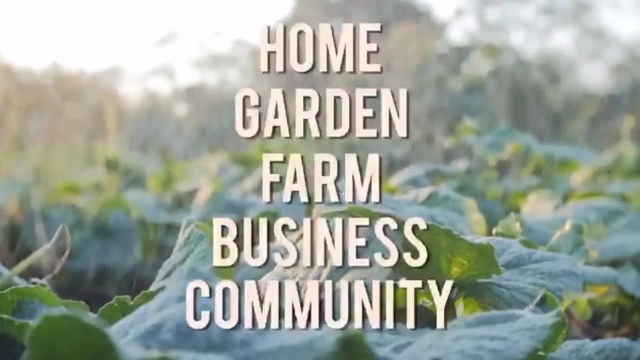 you'll learn from internationally respected teacher, author and lecturer in permaculture, graham bell. this is a series of 18 lectures and quizzes where you will take a deep dive into this amazing design system that can be applied when designing your home garden, farm, business or community permaculture. 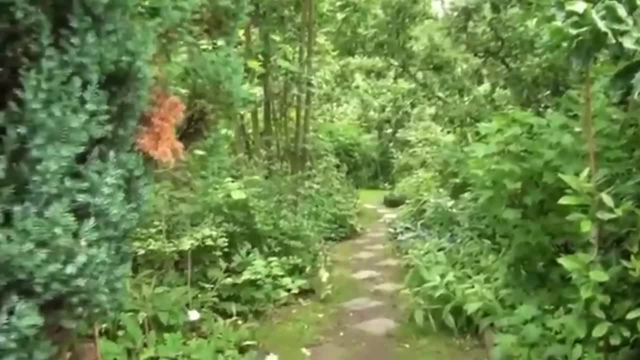 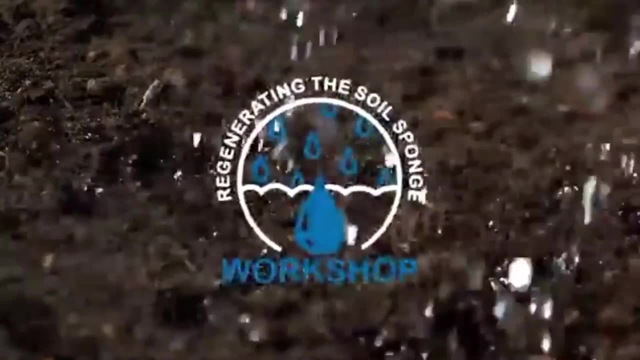 is all about being in balance with the planet and is an ideal tool to have in your bag whenever you're considering making a change. the soil sponge regeneration workshop is delivered by educator and author dd purcells. this five-session course is all about regenerating the soil sponge. 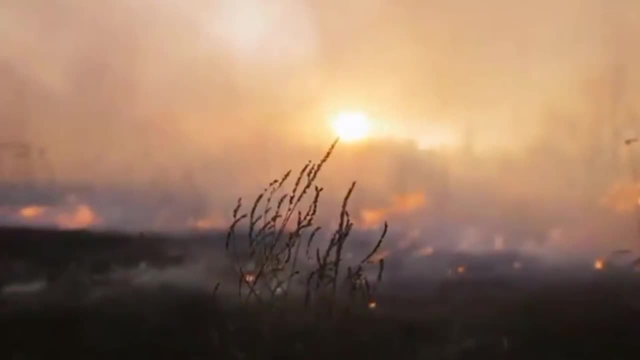 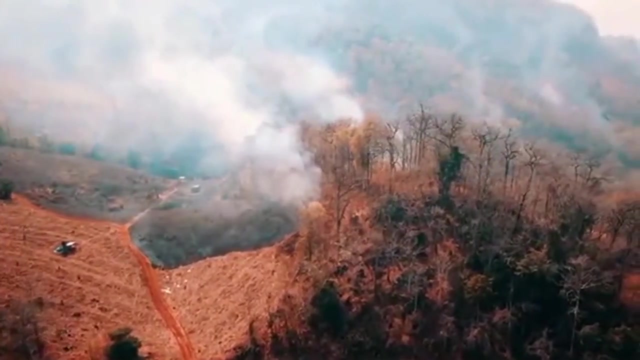 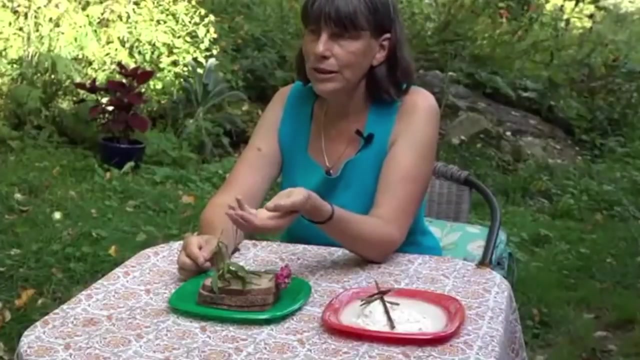 for flood, drought and wildfire resilience. it builds on the successes of innovative land managers around the world who are saving huge sums and damages from extreme weather events and crop diseases, while restoring the dignity and profitability of farming. dd teaches participatory workshops, both in the soil sponge regeneration workshop and the soil sponge regeneration workshop. 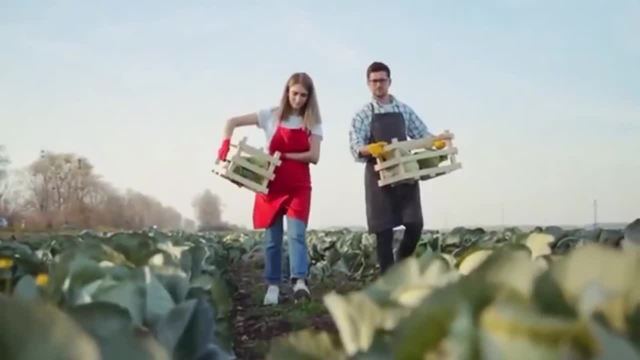 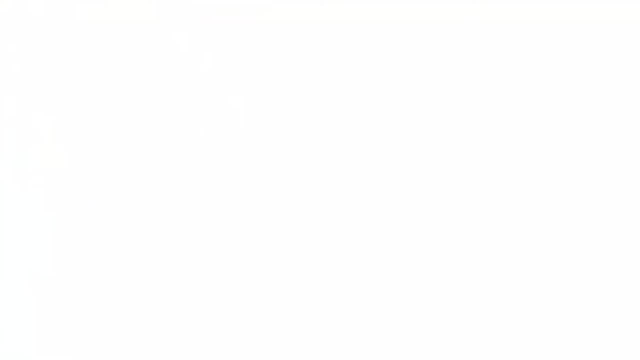 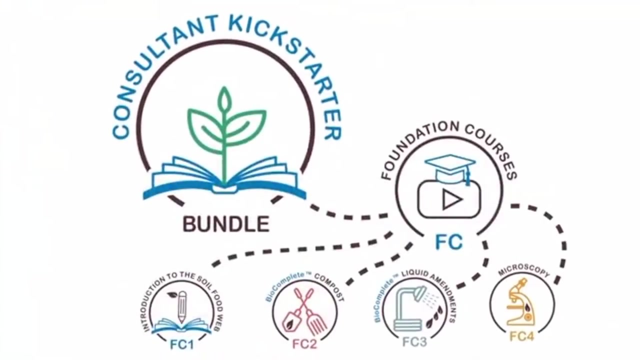 in person and online, helping to show the nested relationships between soil health, human health, water cycles and climate resiliency. so just to recap, the consultant kickstarter bundle comprises the soil food web foundation courses with dr elaine ingham where you get to study the theory. 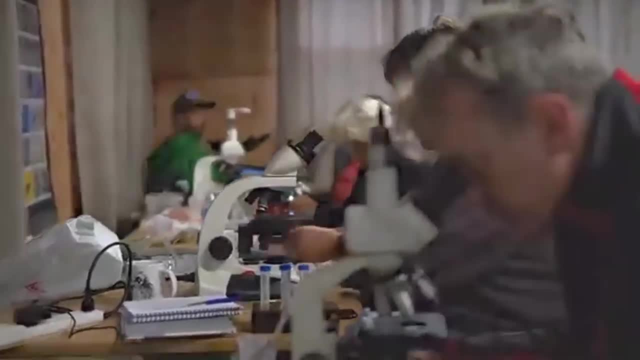 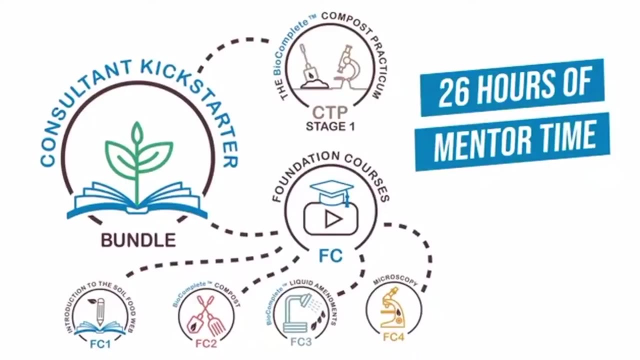 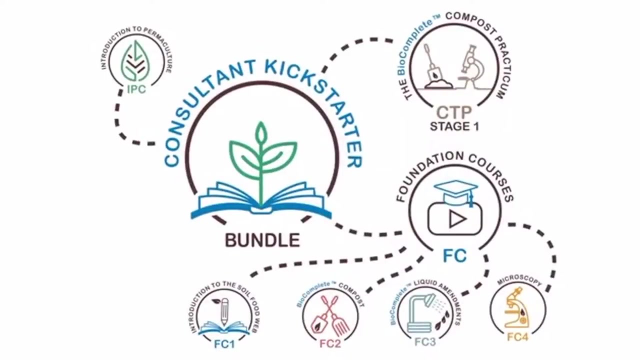 and application methods behind the soil food web approach and that all-important 26 hours of mentor time in stage one of the consultant training program, designed to help you develop your compost making and microplastic processing methods for your soil sponge regeneration program. you'll also get the two free bonuses: the introduction to permaculture course with 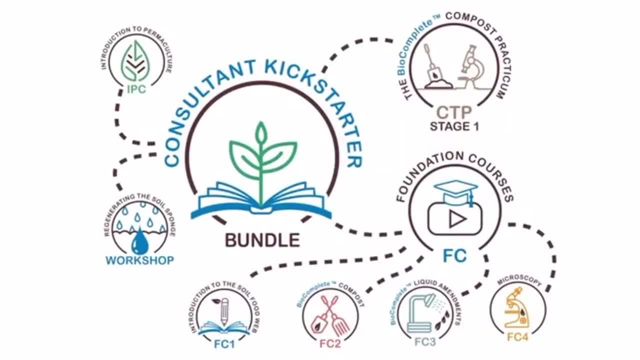 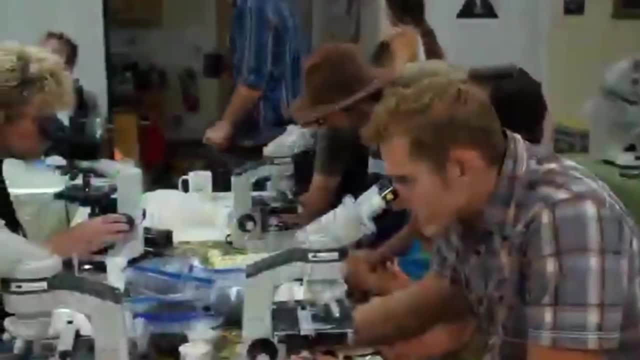 graham bell and the soil sponge regeneration workshop with dd purse house. this bundle is ideal if you want to kickstart your new career as a soil food web consultant. once you have completed the foundation courses in stage one of the consulting training program, you will be well 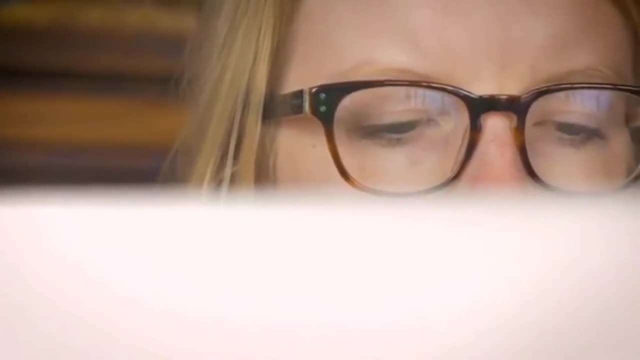 positioned to complete your certification and be listed as a soil food web consultant on the school's website. with these programs, you'll be on the path to a better future. with the soil food web consultant program, you'll be on the path to a meaningful and impactful career. 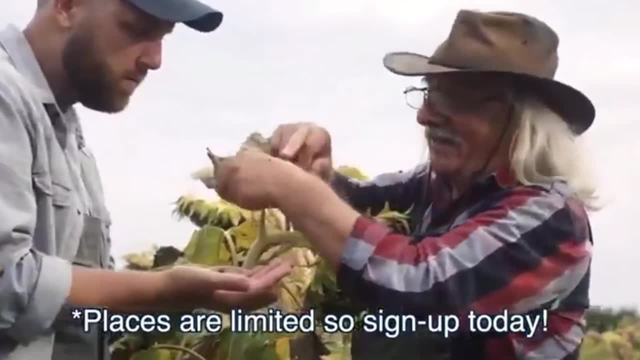 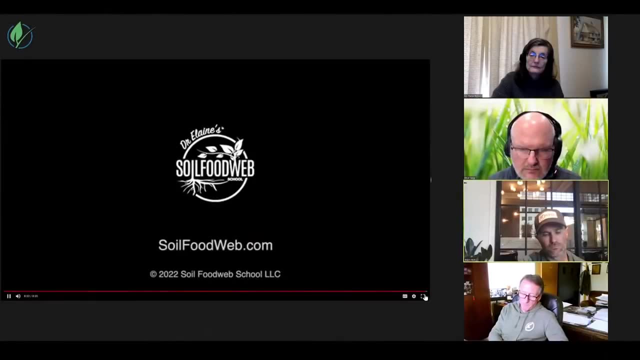 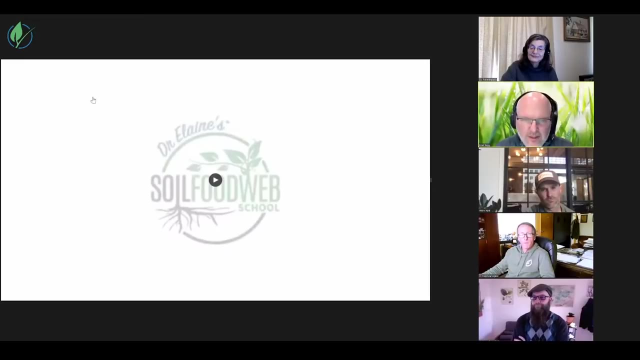 as the soil food web consultant or biological compost producer. all right, okay, so we're going to move on to our part two, where we're going to have todd and adam talk about, uh, the operation that they've kind of created here. and this is the fun part when i try to escape this month. 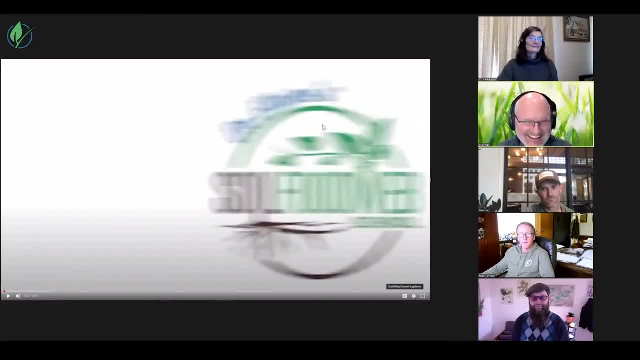 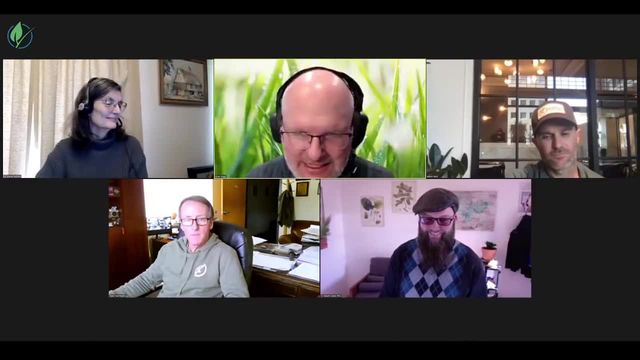 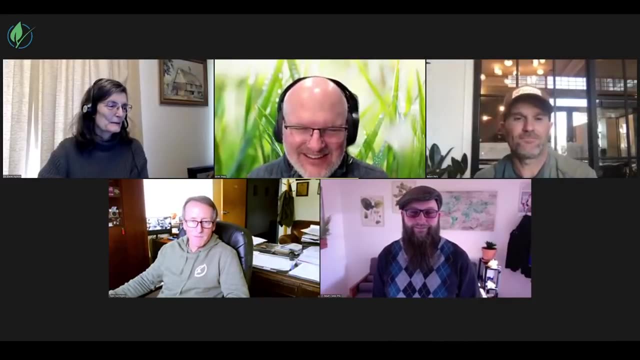 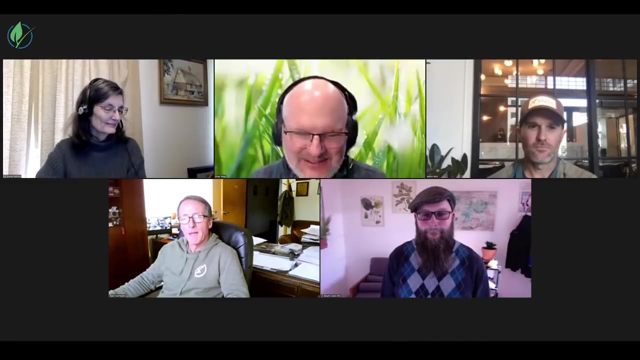 it always takes over. let's it does. we're just gonna get out of it and come right back and then, yeah, skip that slide, it is frozen and full screen. all right, there you go, escape, escape, um. yeah, programs are a blast. my students are the best. uh, sign up, it's, it's great, i agree. yeah, i second that. okay, okay, um, so we're gonna be like i said. 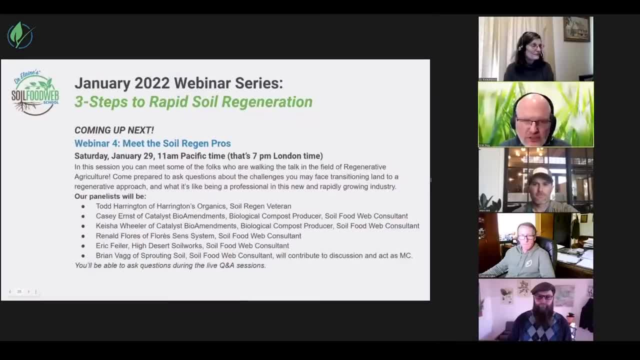 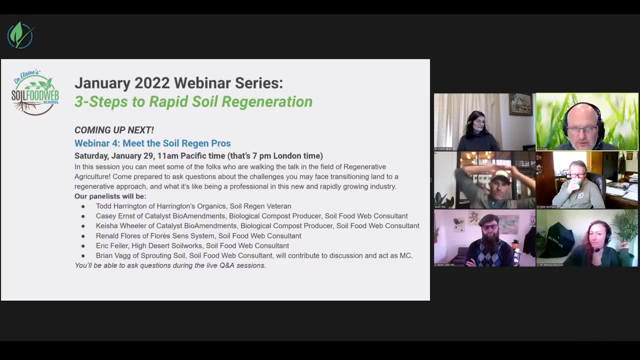 moving on to part two, um, and so we'll just almost talk about the next webinar and then, oh, thank you sorry, i forgot about that. so, yeah, webinar four, which is meeting the soil regen pros. so that's gonna be saturday, um, and we're gonna have todd uh, who's already on the panelist. today. we'll have casey. 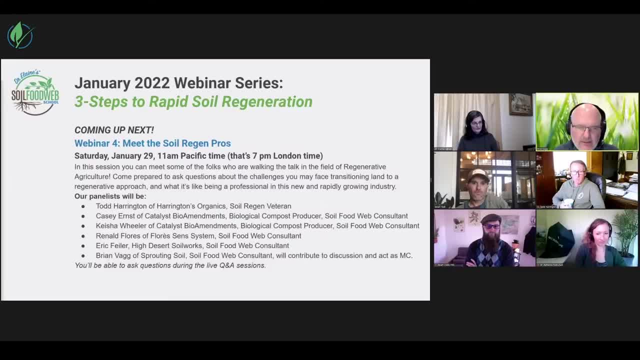 ernst and keisha wheeler from catalyst bio amendments, um, and then we have ronaldo flores from flores and systems, we have eric feiler from high desert soil works and we have myself from sprouting soil, and this would be a good opportunity for folks to be able to ask questions about, uh, the 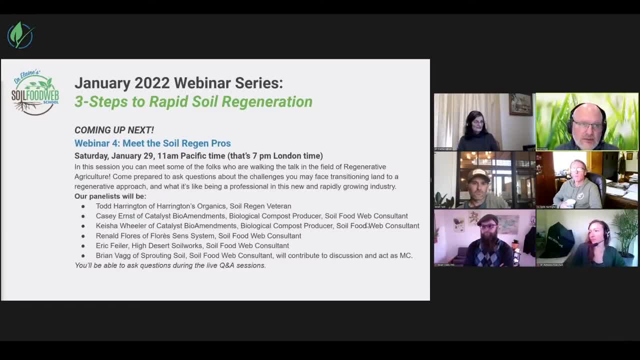 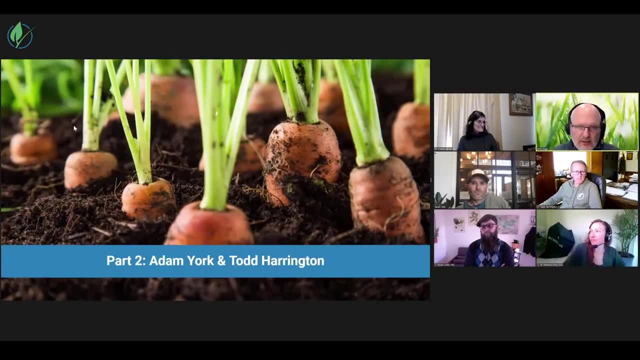 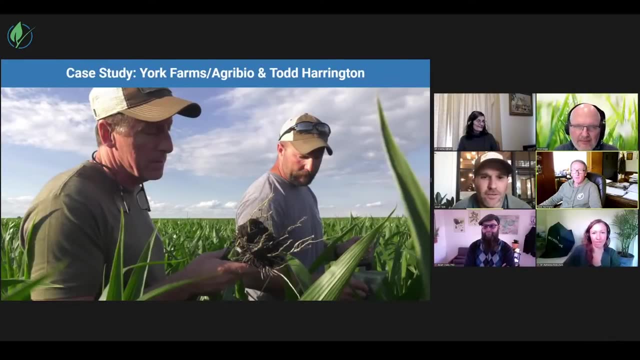 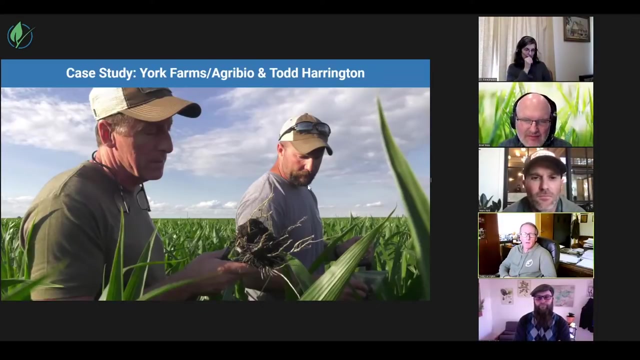 consultant works. that we do you know, and how we go about it and how do you become a consultant and all that kind of good stuff. okay, all right. so part two: adam york and todd harrington. so you guys take it away. so, adam, so, um, yeah, so we, uh, we've been working together for quite a while now and um, 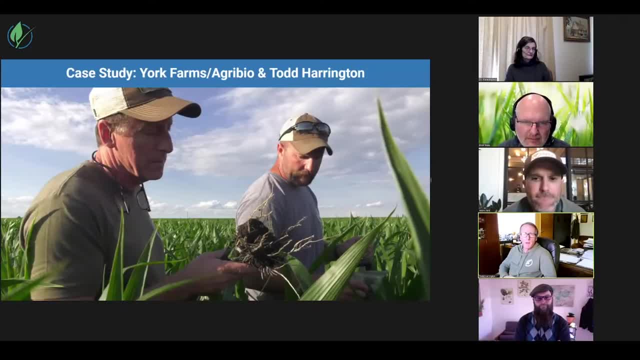 you know, every year, uh adam, like many other farmers, have challenges and uh, i think both uh 2000 and 2001, uh adam was challenged by excessive rain, a rainy season. um, certain fields got flooded again. uh, and you know once, once you get these conditions, there's. 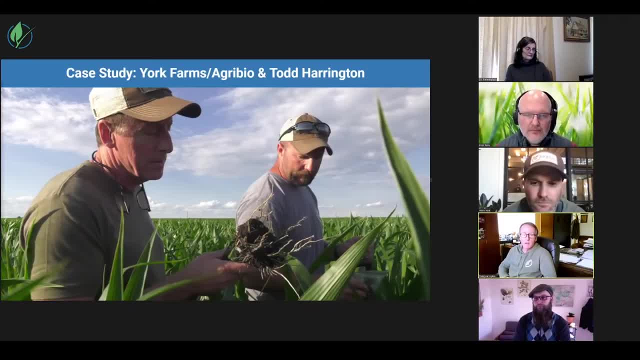 not a lot you can do. um, if anything, adam might be able to talk a little bit about how these fields might have been able to recover a little bit better. um, but really you know, there's a certain point where, when the soils are so saturated, no matter how much you do biologically or organic, 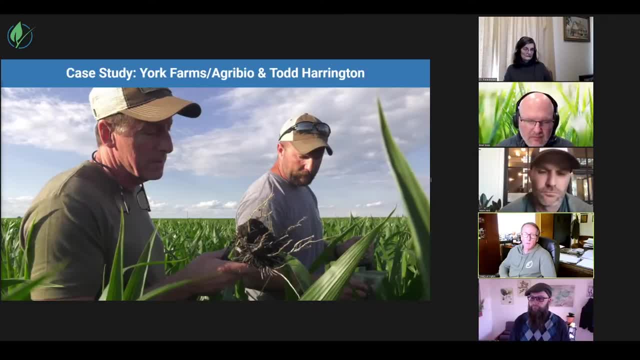 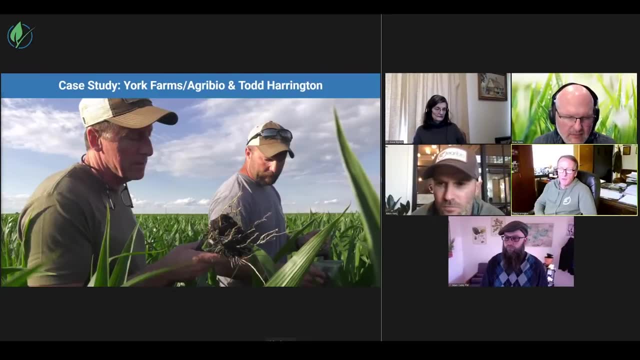 regeneratively. there's limitations, especially when it comes to weather. so, adam, maybe you could just talk a little bit more specifically about you know those challenges and maybe how it's important to have a contingency factor, maybe on how you know we're going to keep those crops from going south. 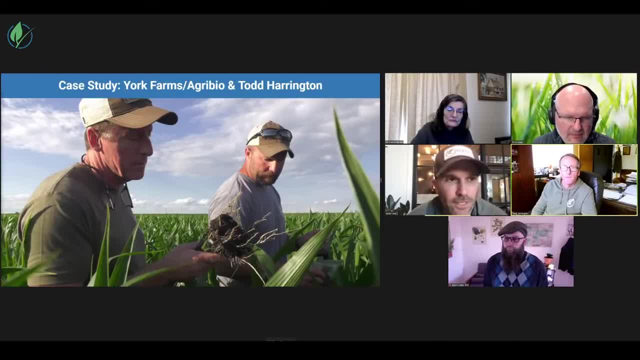 completely, especially when it comes to nitrogen. yeah, so uh for us in 2019. i think it was for a lot of people. it was uh very wet in our area and then another we were very wet again this year. um, so i think one area we had uh down our river bottoms. we had 54 inches of rain from april 1 to 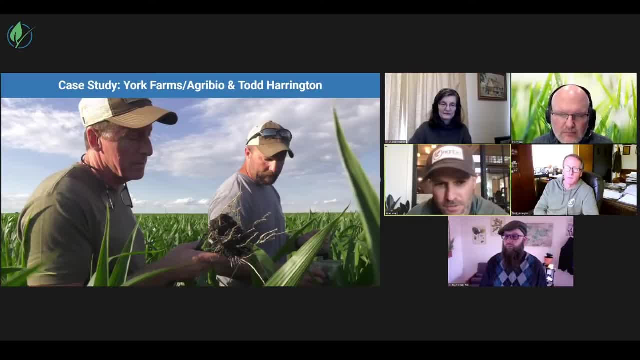 i do believe it was the end of august, um, which is, you know, twice as much as what is on norm, um, so there's kind of been some interesting things that that we have done. so in 2019, we, there was 2 400 acres that we couldn't even plant. uh, it was so wet and by the time we could even plant, 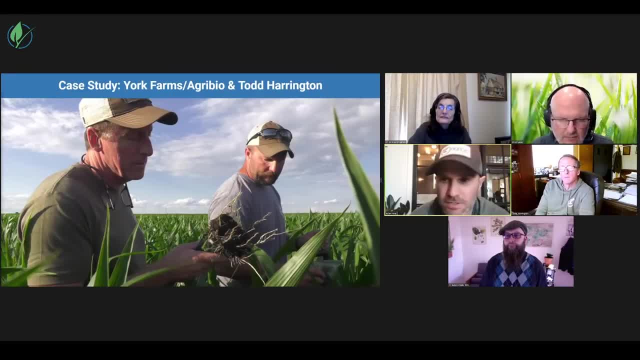 it was, um, i do believe it was the first part of august, so that's when we just chose just to go ahead and grow a bunch of cover crops just to help build the soil. um, it seems like what we found out is: the soil is pretty resilient. you just have to kind of come up with um, um, you know, try to be as synergistic. 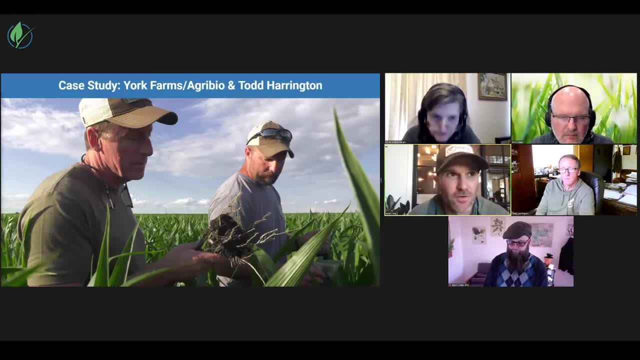 with the soil instead of antagonistic. you know there's you're going to be certain every farmer is going to um have certain challenges they face and it's going to differ from year to year. um just trying to make the best decisions um to help build your soils at that point in time. 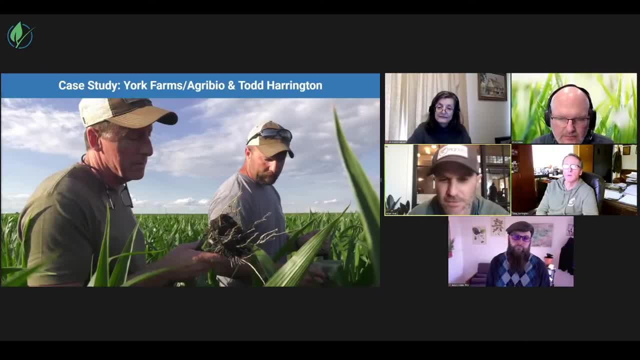 um, it is, it's pretty key. so we had that issue and, like this year, we we did have a crop down south. it was not very good after that much rain, but we did choose to. um, you know, we did some foliars. um, there's certain things you know when you get. 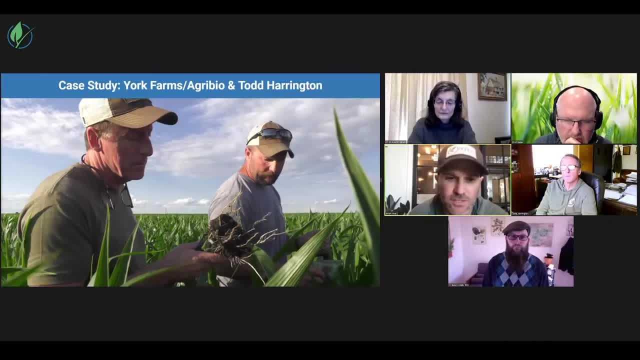 in those circumstances, it's it's really challenging to overcome them, but, um, we're the type of people that we don't give up very easily, so there are certain things you can always do to help um better yourself. um, i think what's important here too, adam, though, is that you didn't. 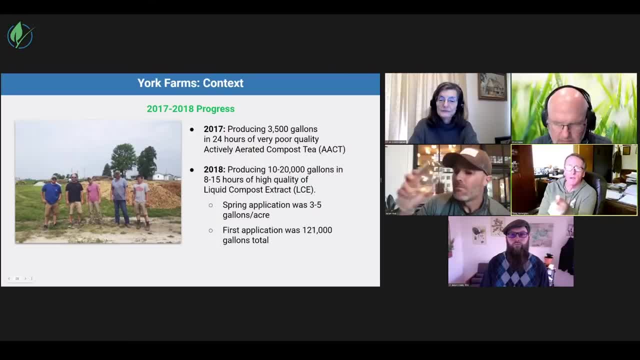 like most conventional farmers, right away started playing applying fungicides, because obviously we had quite a few diseases in those fields because of the excessive brain and things going in aerobics. so instead of applying a fungicide you just let the crop do its thing, and obviously you didn't. 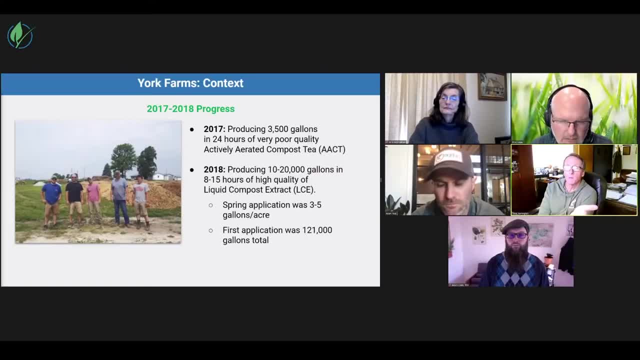 have good yields, but you didn't go. you know, switch to a fungicide and try to save the product there's. there comes a point in time where, yeah, and you know. so what's the difference in cost, though, if you were to apply a fungicide and save that crop, versus let it go and let nature takes its course? 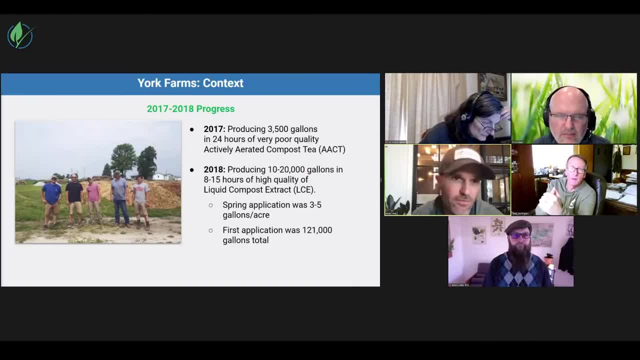 you know, i mean, everything's gotten pretty expensive anymore. so 30 bucks an acre plus application, you know, and in certain, in certain circumstances, you know um it's not worth it, but um you know when, when crops are good, we've not used fungicides. you know, it's just, it's one of. 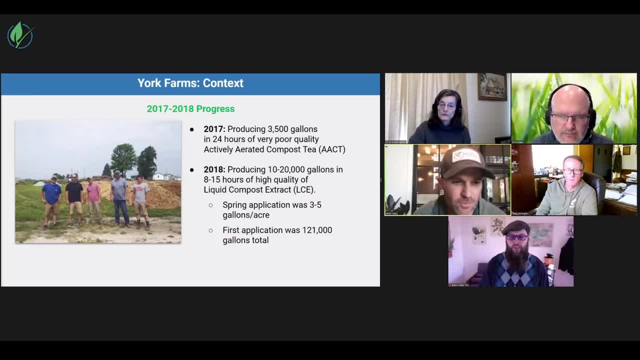 those things. it's a tool that you know, i think in agriculture, when you're making the transition, all these things are tools. it just depends on you know what, what goals you have at the end of the day, you know, i do believe in what you're trying to accomplish. so here we are, back in the 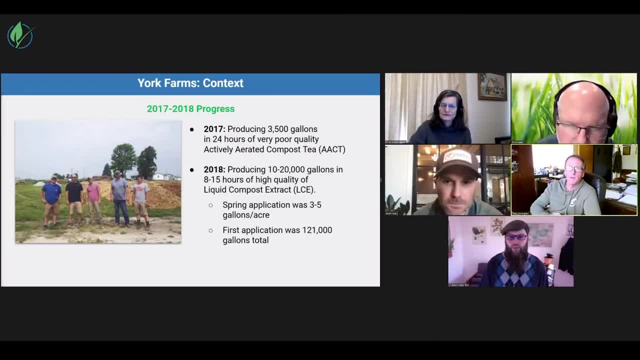 making of the farm, and we're going to be making a four hundred and six thousand pound farm, right? so it's we all here with the focus on the future of your farm. your everything that you're doing is, you know, being able to save the energy for your farms and for your crops. 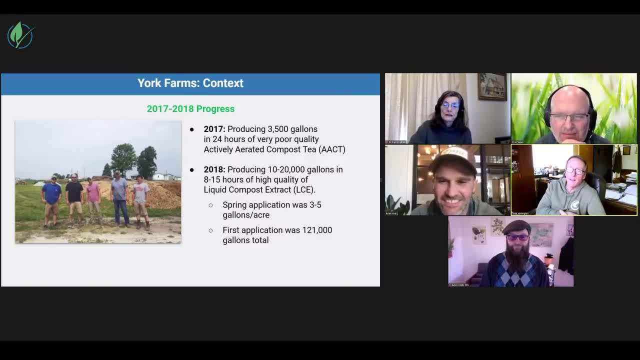 and and and what's um- one of the great qualities about the art ofな- and, of course, of the years- and i think i'm also an architect, i've been an architect for over 20- the inputs, the amendments, probably, and the sugars and the fumates and the kelps that were. 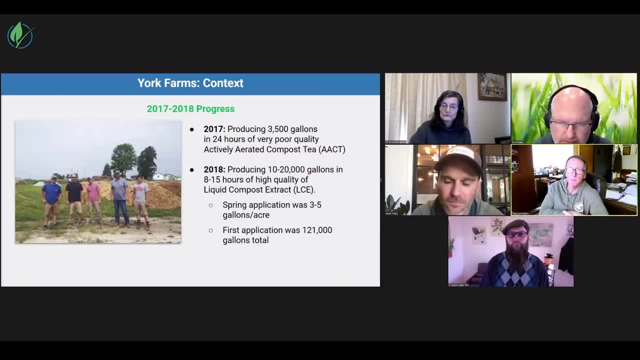 in. there is probably where we were seeing some response on the crops. but you've gone a long way since then. so you know, tell us a little bit about you know the originally starting- how challenged you were doing the activated aerated compost tea with the seven 500-gallon brewers. 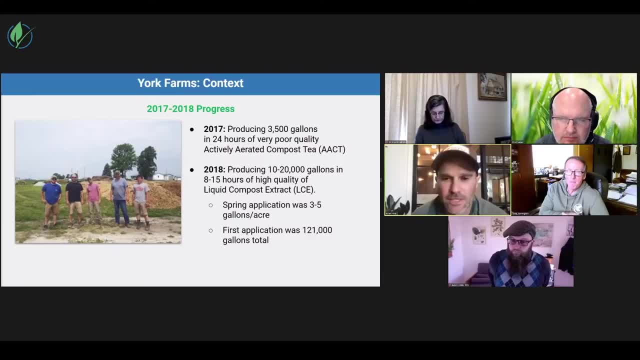 Yeah, so when we first went to the compost tea, we had seven of these brewers and we were brewing up tea. We were getting compost from not locally, We were getting it from actually California, shipping it in, getting a food source, you know, and making these teas. so 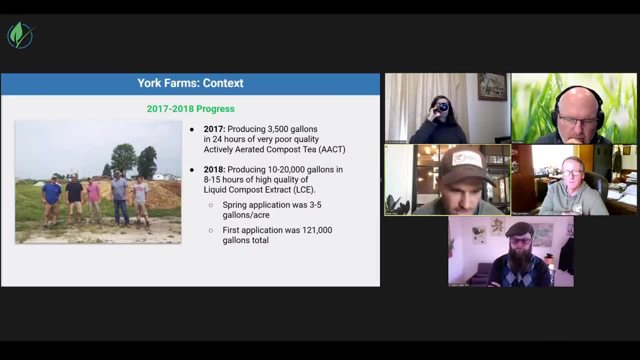 my brother and I would be, and we had a couple other guys that were helping us at the time, but we were. when we first started this, we were pretty low budget. We had an old Quonset. that it's when it's warm outside. it's hotter in the Quonset than it is outside and when it's 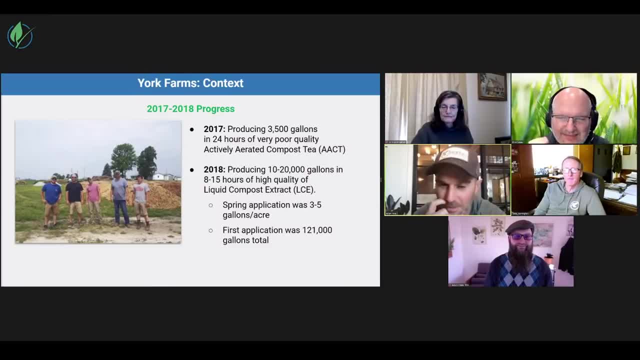 cold outside, it's colder In that building, it's just. it was not ideal, but we were just at least working with what we had at that point in time, and we were. we weren't getting much sleep during planting season when. 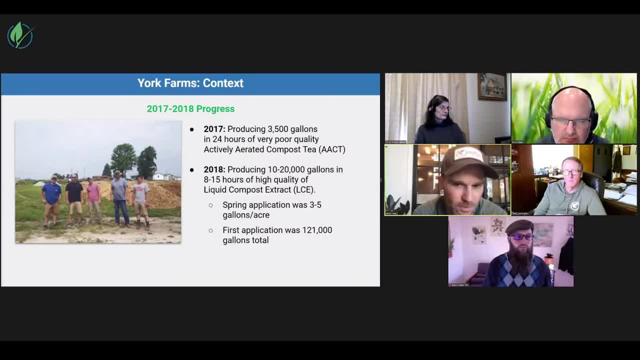 this started. but when we were doing this, I mean we were seeing some value. like Todd said, was it from you know some of the food that we were adding, what it was, you know? we were at least seeing some value, but we were also understanding that we weren't going to be. 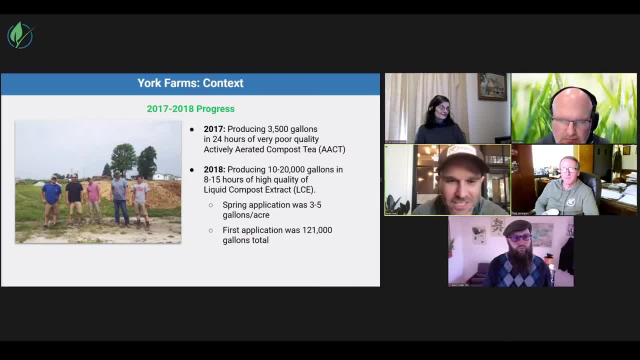 able to live our lives very, very good if we continued down this road, because I probably would have been divorced. My wife would. yeah, it comes to a point in time where you have to. you have to still have to have a life too. so we got with with Todd, and we were 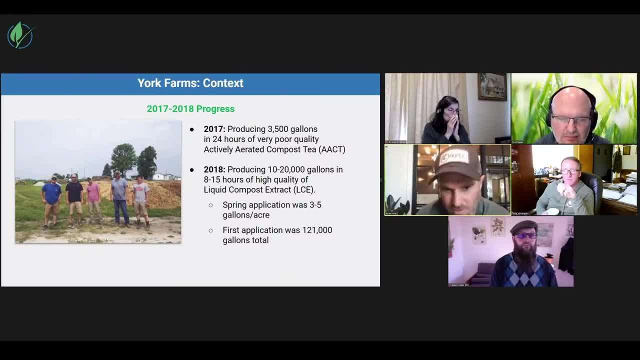 looking at this tea and he's like: oh you know, there's so many things we can do to help improve what you're doing. We ended up choosing to go to compost extract and did a lot of work on our food sources. Todd has helped us. I mean, we've we're still working on it, but we're still working. 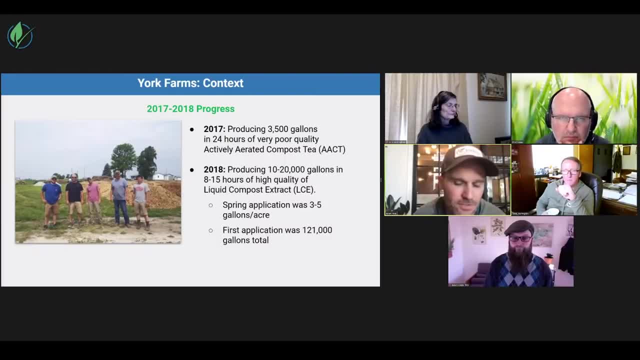 on. you know, we we do our own vermicompost, source all our stuff local sources from around home We're working on right now we're working on highly fungal compost that we have working on in the in the shed. We're fortunate enough now that we we've built a building that that is not. 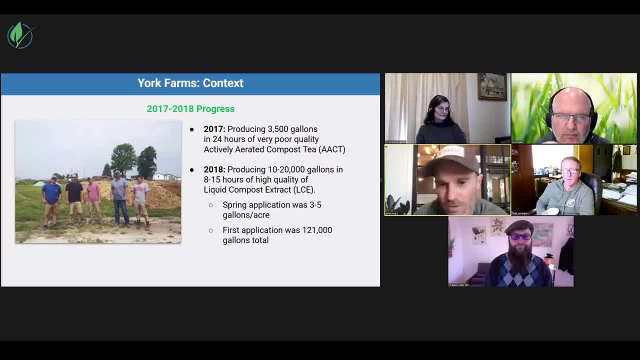 like what we had before, but we do have a worm room, what we call it, and we have a vermicompost and we do keep keep the temperature regulated in there, which which helps a lot. So, yeah, so we went from. 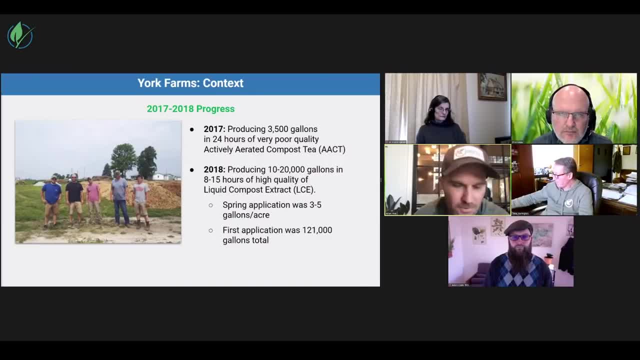 working crazy hours making tea to switching over to an extract. We have an extractor and producing, you know, a continuous flow extractor which makes- I don't know about, I would say- 1,700 to 1,800 gallon an hour, continuously. So 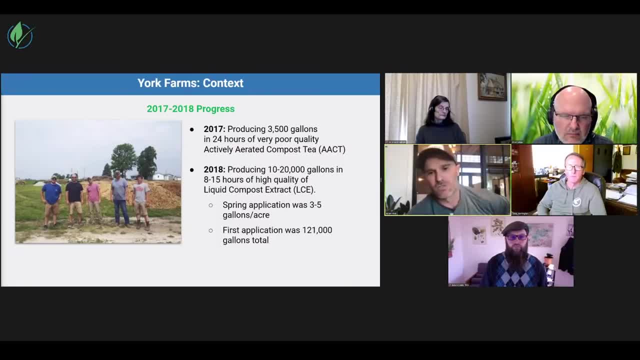 it's made our lives a lot easier. and then we add the food sources to the extract as they're hitting the planter or sprayer or however you're you choose to apply it, Yeah. so when I saw the size of Adam's operation, I'm going, wow, they're. you know, they were really limited by time and 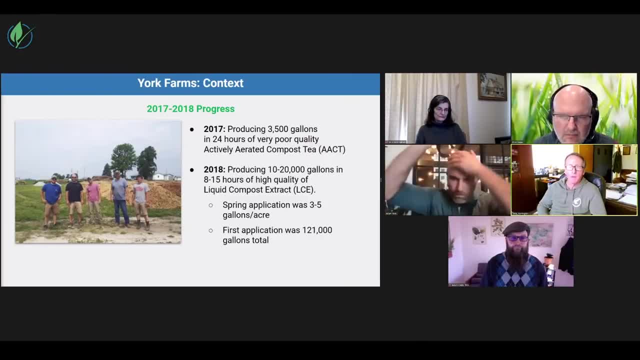 volume at that 3,500 gallons, not to mention the amount of time and labor cost to clean and disinfect and kind of get to the next batch. So we went from 3,500 gallons to you know, you know. producing in a day anywhere from 10 to 20,000 gallons. That's a big difference. And I jokingly said to Adam I said: once you go extract, you don't go back. you know jokingly And in a way, 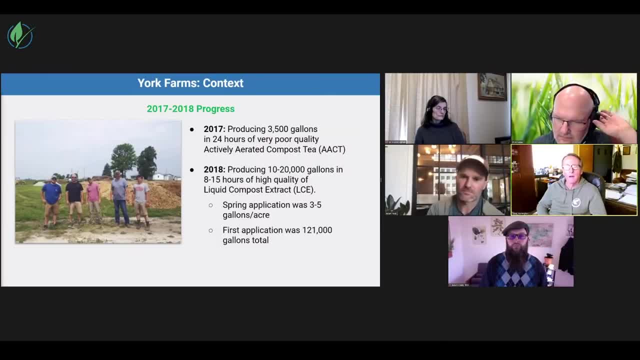 when it comes to production and doing large-scale crops like this. I mean, really the extract plays very well when it comes to the volume thing and also the stability thing and also the cleaning thing. So you know not that. 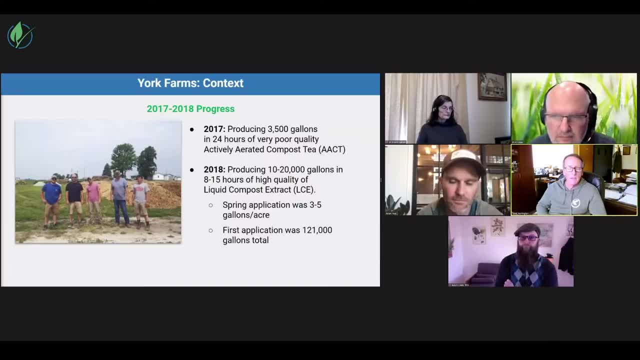 that's where Adam's you know goings and turns is, you know, the long term, I guess. Yeah, Yeah, Yeah, My thoughts are on Adam's storytelling and on, you know, some of the other folks. 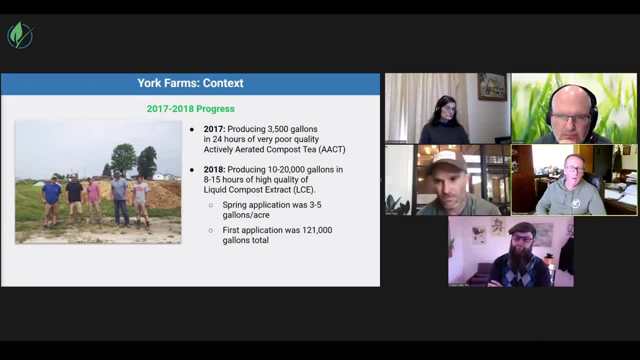 you know sort of ways that you know the small business that you're, you know, you know you get in contact with and you know, let's say, you have a really busy house, you're working, you know you have to deal with a ton of- you know- lots of stress and 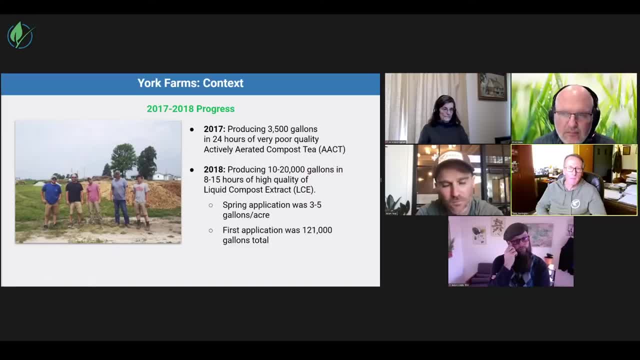 revenge going on. Yeah, Yeah, Yeah, Yeah, Yeah, Yeah. big savings and a big improvement in their capacity to produce more, more biology, even if it wasn't, yeah, and i think you hit the head on the, or hit the nail on the head too, todd, i mean. 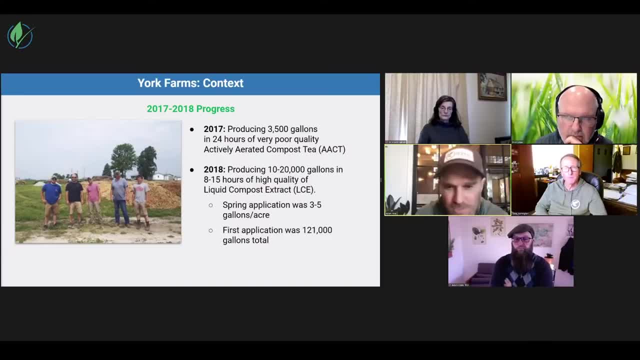 there is a place for tea. you know, in our operation it just made a lot more sense this. you know i was not going to be able to keep help um, and just logistics of it. it's just just. you know what worked for us. yeah, maybe talk a little the detail. we'll go to the next slide about how we were. 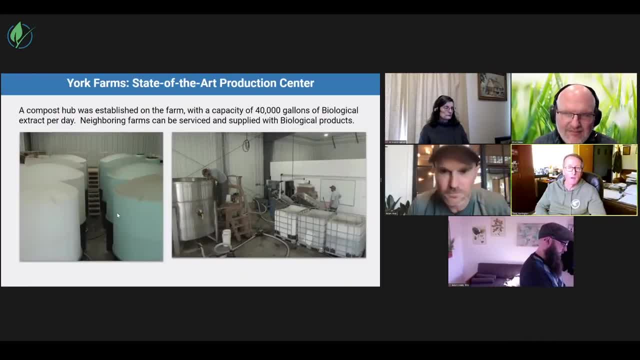 utilizing the extract in the spring in burrow during planting. yeah, so, okay, so this is how we set up our new building, um, so i'll start over here. the tank on the left is just. it's just kind of a mixing tank, how we, how we do certain things, but over you can kind of almost see it's kind of. 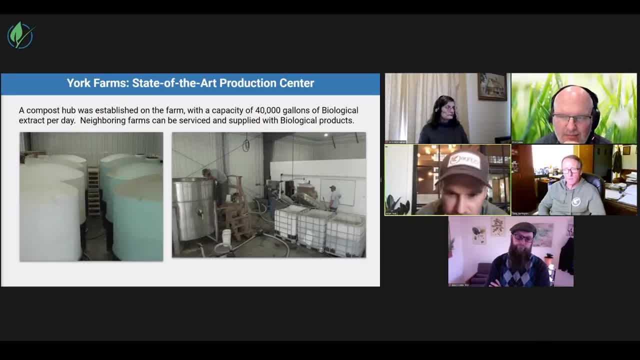 blurry, but on the right side of the picture, whatever, you can see our, our uh extractor there and todd's sitting there and you can kind of see it's got a place for um, our vermicompost. you add that vermicompost into the extractor, um, it's got water, um jetted into it and it's extracting. 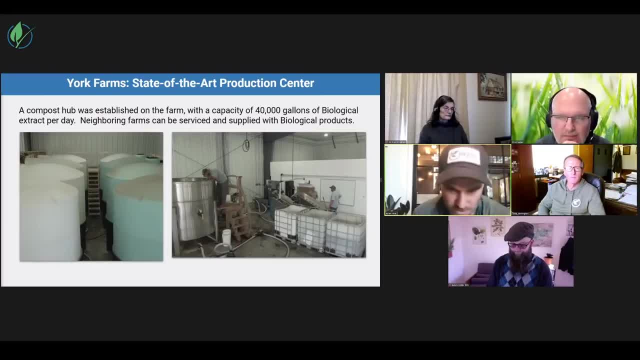 um, the microorganisms and the nutrients out of the vermicompost and making an extract. so over on the left side, the white tanks we colored we. we did this on purpose. we bought two different colors of tanks just for easy. but on the right side you have the blue tanks. those are just our water tanks. 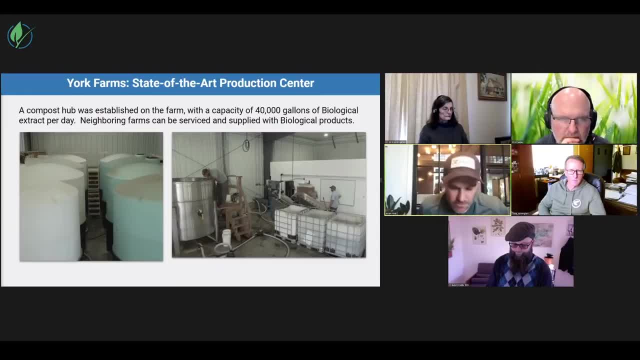 um. so we get water come in. the ph of our water is a little high um, but we use uh, fulvic acid to um to help bring the ph down. and then the white tanks on the left are where our compost extract um goes into. so you can kind of see in the back side of these tanks on the bottom you can kind of 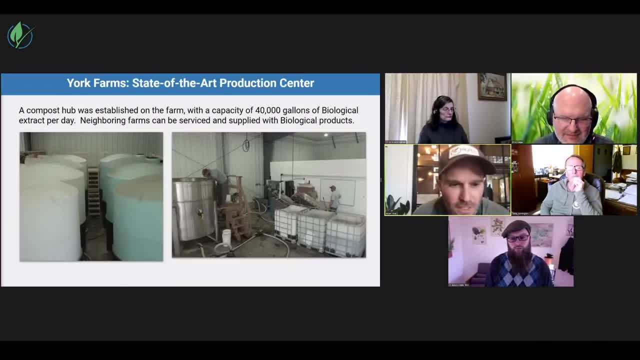 see some hoses down there. you can't really see them but you can kind of see them on the bottom, but you can kind of see them on the bottom, you can kind of see them on the bottom real well. but we have pumps and those pumps um are circulating, um on timers. they will go on and 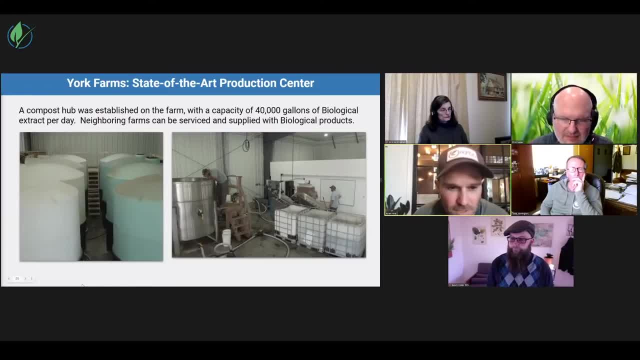 they will vortex the, the extract to keep it in good shape. but we have all this stuff uh set up on digital timers so it works out really well. but those are 2500 gallon cone bottom tanks with about they're about a 30, 30 degree, 30 degree cone on them. 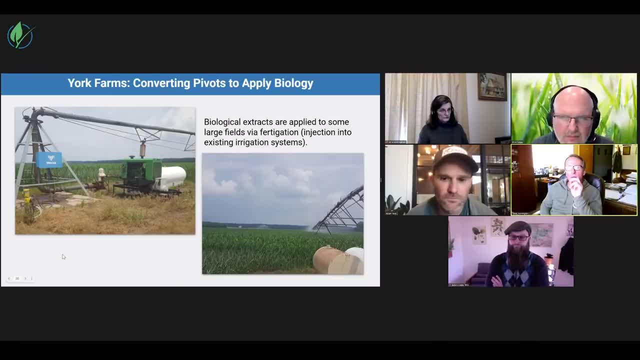 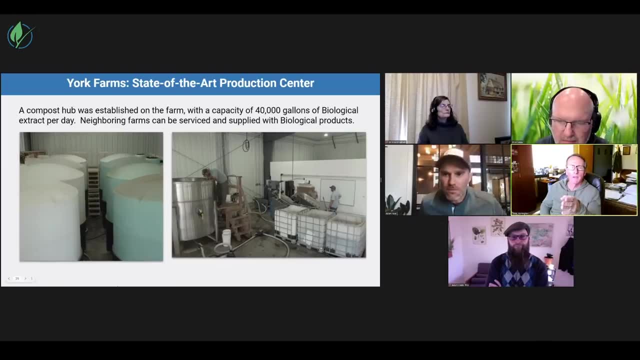 so the um on the slide on the right if you go back. thank you, um. adam had several different types of compost that he was extracting, so you'll see a couple different bins and at times we might be using different sources of vermicompost or compost. might be more fungal, it might be more. 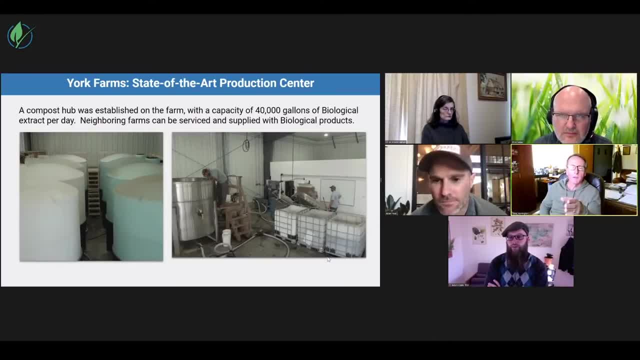 of a vermicompost. so he was definitely good about, you know, trying different combinations of different mixes to get that diversity into his product. yeah, it's a good thing you brought that up, because every every year todd todd gets together with us, you know, several different times a year. 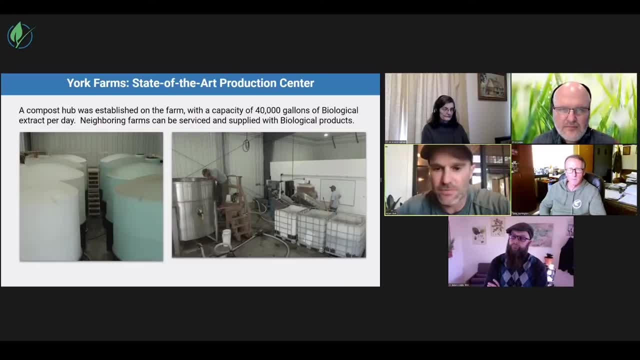 actually we got, uh, we're gonna get together here this next month as well, and we do a lot of work on um improving. you know, always, you're always trying to fine-tune and and improve the, the compost that you're, you know, creating and um, so we, we do a lot of different things and 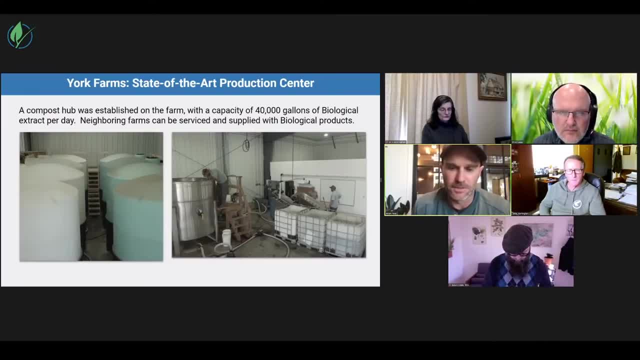 at the end of the day, we, we um, look at all these under the scope and uh, try to figure out what the best mix that they can be for that uh, the rest of the day, uh, we are, uh, we have to look at that. we've got to have a lot of examples of compost and i think we're gonna see if we can get a lot on. 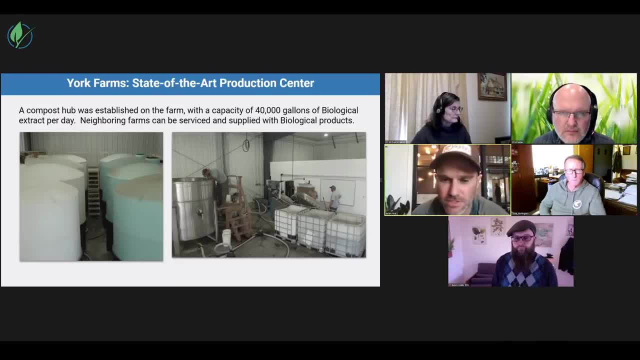 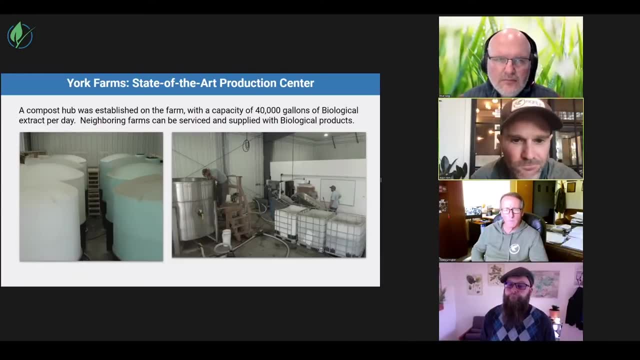 we're gonna see if we can get a lot of examples of compost- and i think we're gonna see if we can get a lot- is to kind of get to where we want to get to at the end of the day. so we might be adding three or four different types in and mixing them together and also the 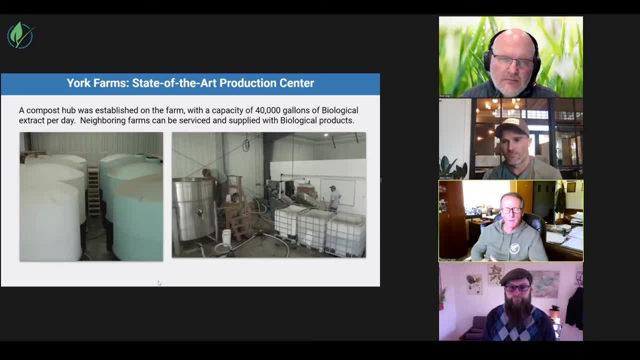 water source. Adam, you know, maybe you can just explain the two different sources of water. we had a well and then we had city water. we looked at the water, we analyzed it and then we ended up doing some things to the water. you know, doing some structural things to the water and also the pH thing which you mentioned. 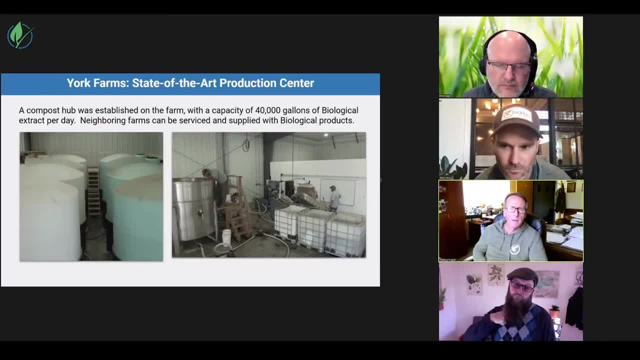 was important because your original pH's were pretty high. I'm certain I don't know which source. yeah, our pH on the on the city was was like nine. the well was a lot better. yeah, depends on where you're at, you know, and how much water you need. if we do use the city, we we are storing it in storage tanks. 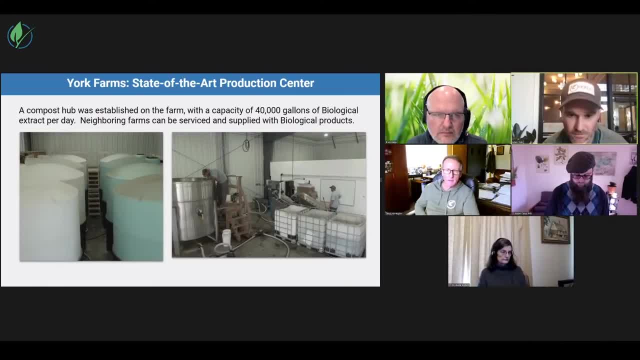 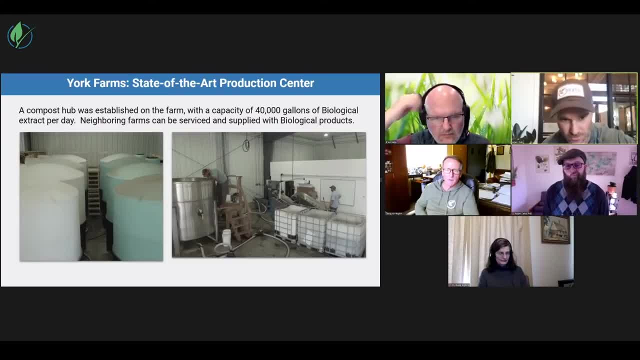 ten thousand gallon tanks, holding tanks, and uh, and then those go into these, so we have actually 30,000 gallons of water storage to ten thousands, and they end up going into these tanks here, and that's where we treat it with the filled with acid to help bring the pH down in it. now, we didn't know, obviously, as lane knows. 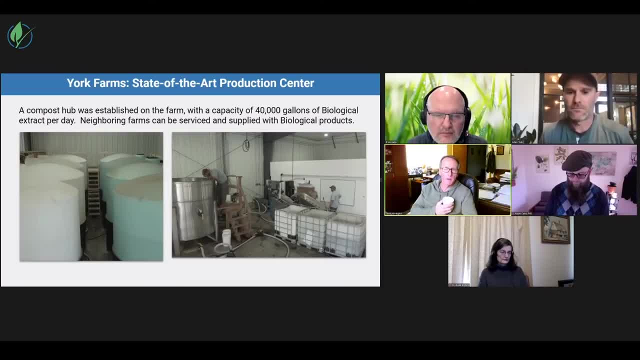 and she talks a lot about em parfaits, the fulvic in the humus or some we used especially to dechlorinate the water, but also we're in this situation. we're using it to lower the ph, but yet we know it's compatible with the biology and it's a great product to use. 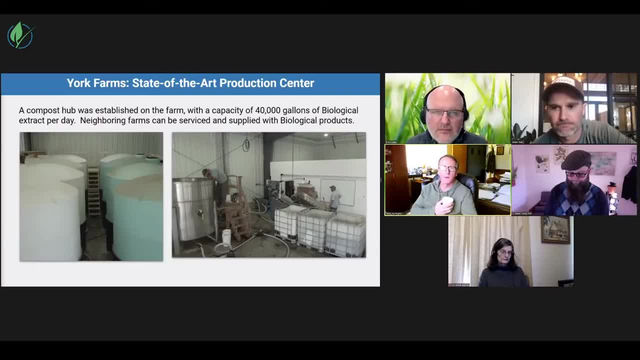 where some people might use potassium, phosphate or gas, let's say, which is pretty detrimental to the biology, to lower the ph. so we're really sensitive to those kind of things and adam found a good recipe on you know how what kind of rate to use of the fulvic on a regular basis in. 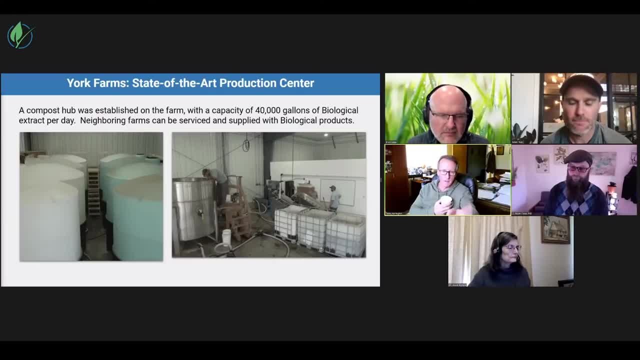 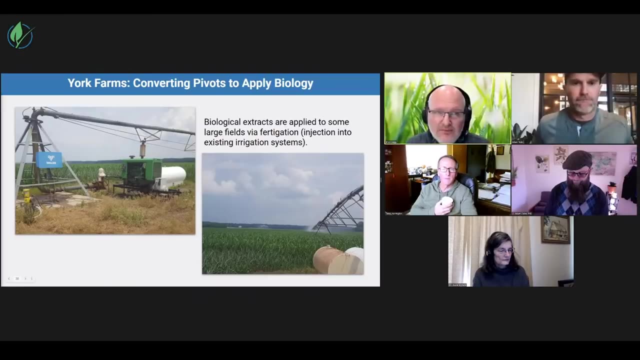 these batch tanks to the right that you see there, or on the left, the the bluer color tanks are the water tanks that have been, uh, spiked with the fulvic. so, yeah, if you want to, it's become much more of a problem too, um, recently, just because sources of water are becoming difficult. people 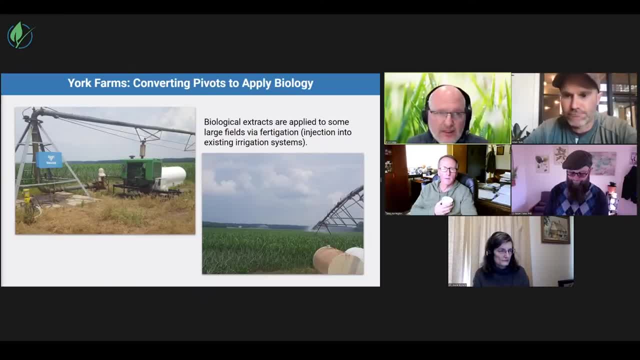 are drilling deeper. they have high levels bicarbonates and things like that. so treating your water is really important. you guys brought that out great. we did this before we. we had the slide already. but this is, adam, if you just want to kind of summarize the how many pivots you have and how many pivots. 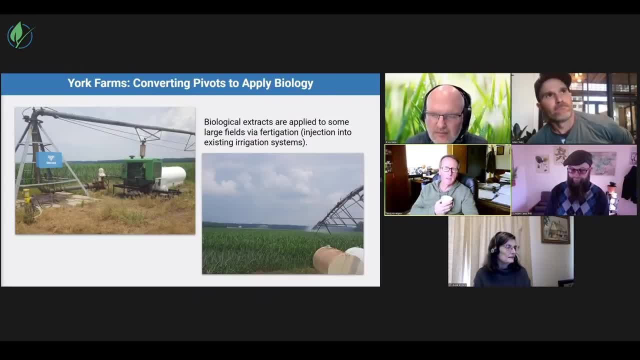 you're injecting with the uh, the extract or the actives? i think this, this one you were. actually, we had an extract that we brought in the uh in the tankers and then we downloaded it to, and adam's really great about being innovative with equipment and utilizing old equipment that otherwise would. 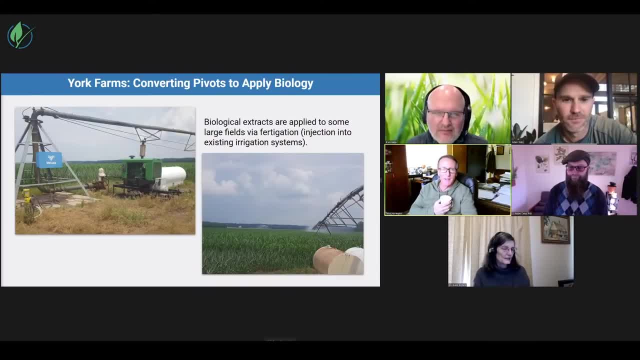 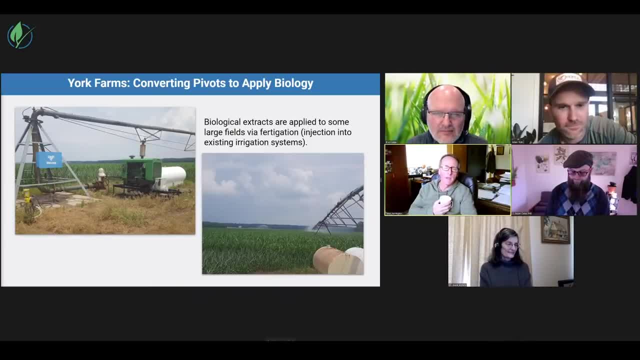 longer needed anymore. so what he did is he put them on trailers and then brought them to the pivots. we would download the extract, add the food, because these brewers already had aerators on them and they, uh, if the the location didn't have power, then he, we had a generator, uh, that would generate the 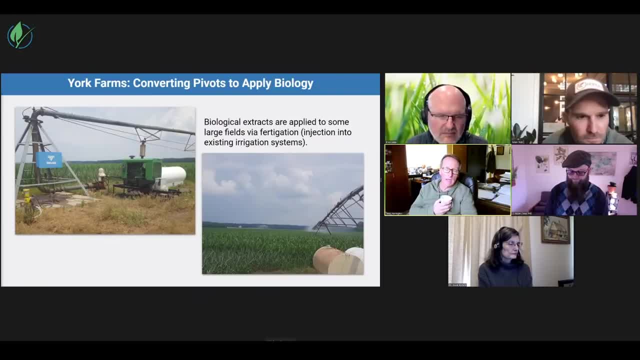 uh, regenerative blowers so that we could activate the extract for a certain period of time and then it would get injected. yeah, so, um, so these are. so we have. i guess i'll start with we operate. i guess i think it's 21 irrigator pivots and i. 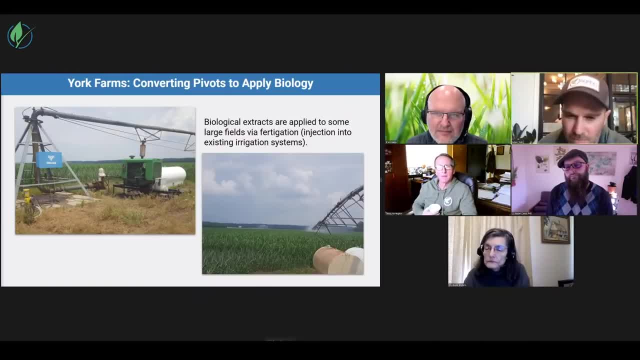 i think, i think, if i did the math right the other day, i think we're like 4 200 acres underwater or something like that, i do believe. so, um, they're a lot of work, but they're very valuable too if, obviously, if you need moisture, but you can also um inject, um inject things into them. so 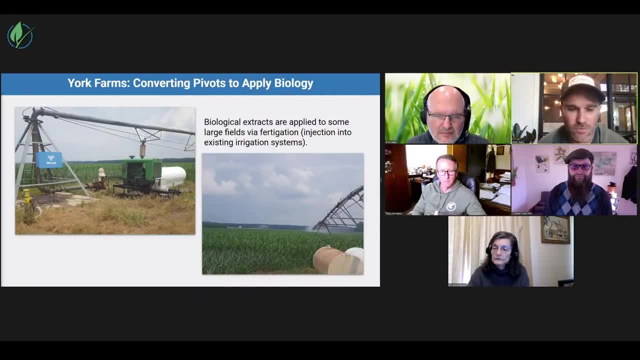 so over here, this is a diesel powered one, um, so it's running off of a. uh. i think this is a six cylinder. this pivot actually right here has a corner span on it. it actually, uh, covers about 320 acres. um, so we are uh. they have check valves in them and we'll have injection pumps over there. 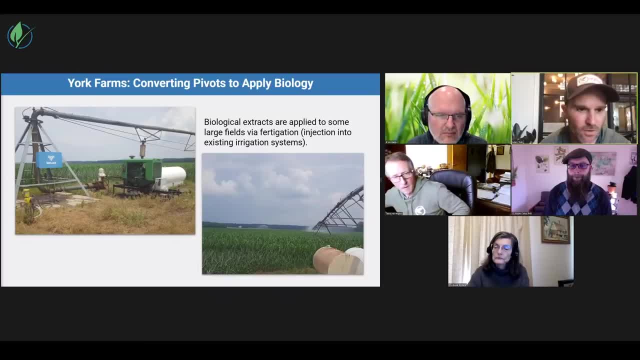 on the left hand side, underneath the valley sign, there's a yellow diaphragm pump and that is what we inject: um the compost, teas or extracts or anything like that, and then we inject the compost or you know any food sources or whatever you choose to inject. that's what. that's how we do it. 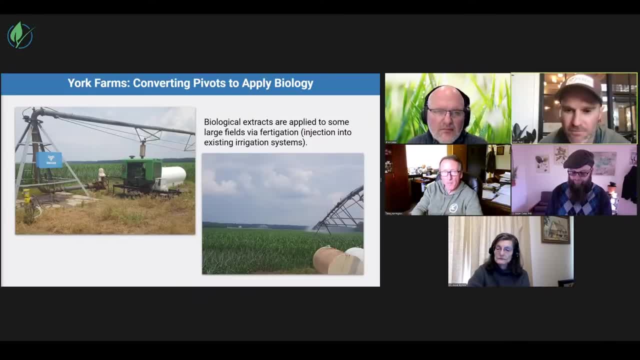 um, but it's very. it's been very, very beneficial for us to be able to do this um and very economical. um, like i said, we had to. in order to aerate the tea, we had to um use a generator, which is it's kind of a pain in the butt, but on uh, you can on these pivots if other people have pivots you. 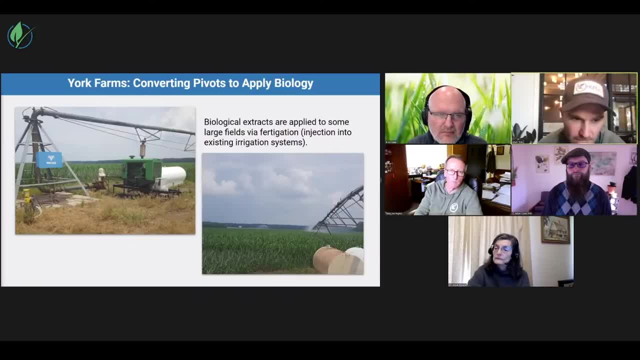 can actually get a bigger end burger inside the machine and then you can just, uh, you can get a that valley panel and you can actually while that irrigator is running. you can actually, as long as you have a big enough inverter, um, you can run a 110 plug in there and just plug them right in. 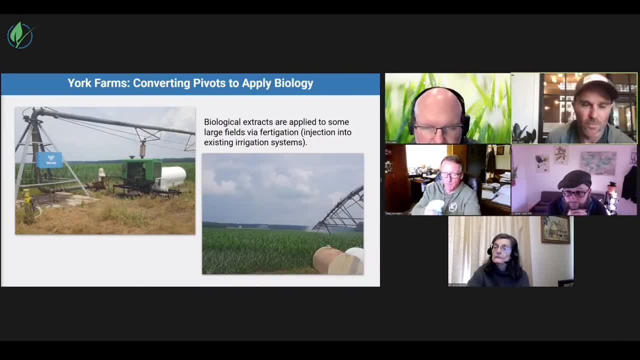 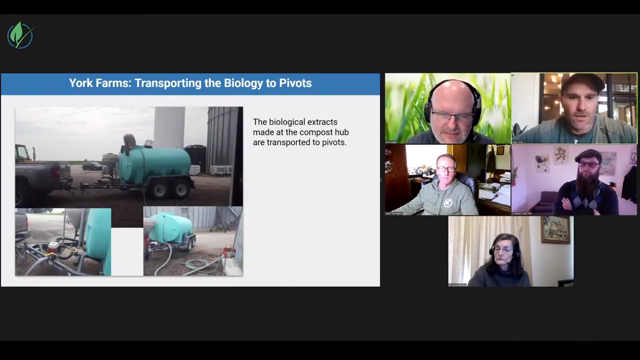 if that's something other people choose to do. um, we ended up doing that to about, oh, i think we did 10, 10 of our pivots that way, um, which has been very, very handy if you need to aerate. what next slide? okay, so this is. this is a slide here where, um, this is how we, this is how we. 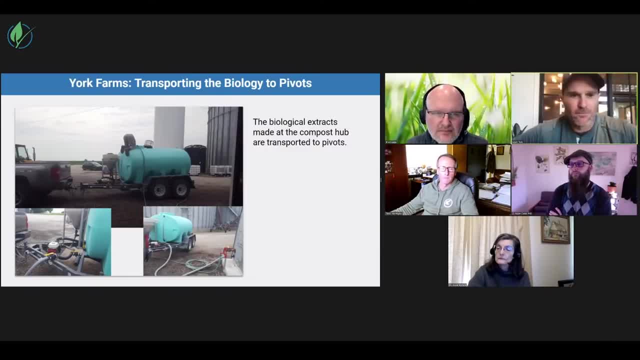 transport a lot of the extract um and food sources, so we we pull around. this. here is actually a picture of a 1200 gallon polywagon tank. uh, we have 1600 gallons um. enduro class makes some really nice tanks. they also have like decks that you can actually put totes on them with food sources or however you want to do it. 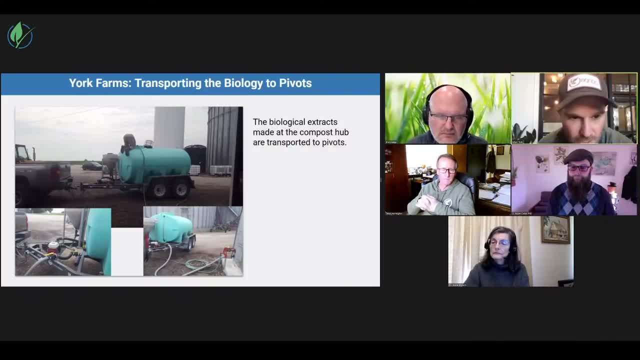 but we keep the extract in the tanks and then we have these cone bottom. you'll see the cones on the side where we'll inject the food sources in there, as that extract is going to whatever you are applying. so, um, the way we mainly apply it is through our planters. it's in springtime and we 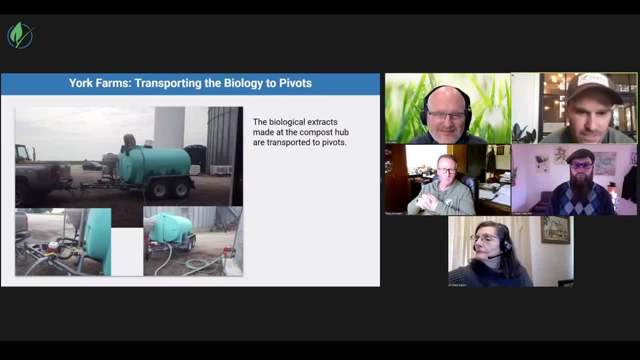 are using um we. we use an ag excel system. they're out of nebraska, um, but they they came up with a orifice list tube. so instead of having the whole the orifices with just the little, with the little uh holes in them, um, where you know if you get a piece of compost or whatever, they're easily plugged. these are like. 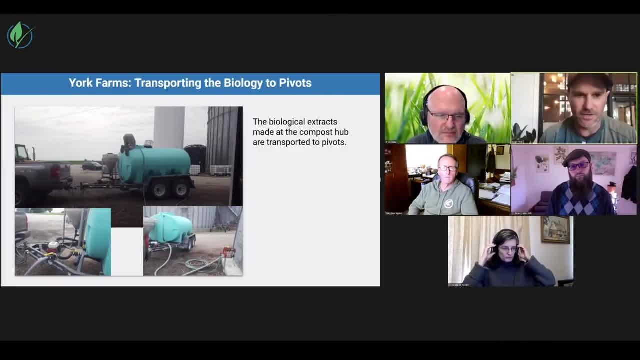 eight foot long hoses that have an orifice on it that that, uh, bigger things are able to travel through, to go down and put this around your seed, um, and from there it goes into, uh we call like a total totally tubular tube, um, which is like a. 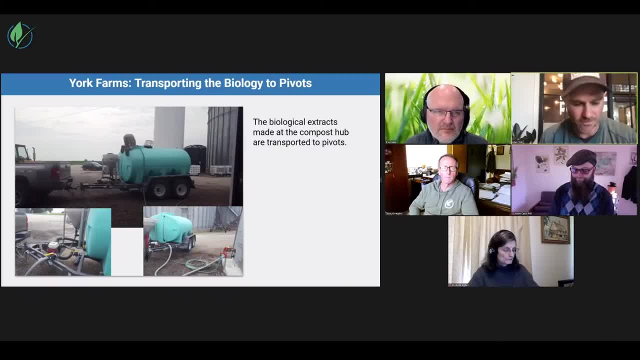 stainless steel tube, that that the extract drops right in front of where the seed is actually being planted in the furrow, but these tanks help us get it to the sprayers. you know, uh, planters? uh, we have several of these. we actually have some bigger trucks, you can put it, and we have stainless. 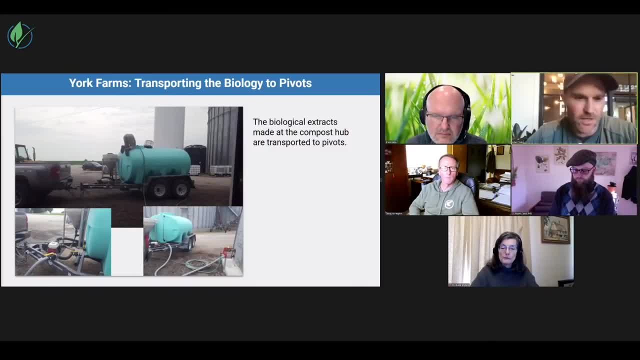 steel tankers so we can move it in. you know, however, uh, you're set up to do but, um, the main thing is to make sure that the seed is planted in the right place, so that the seed is planted in the right place, so that the seed is planted in the right place, so that the seed is planted in the right place. 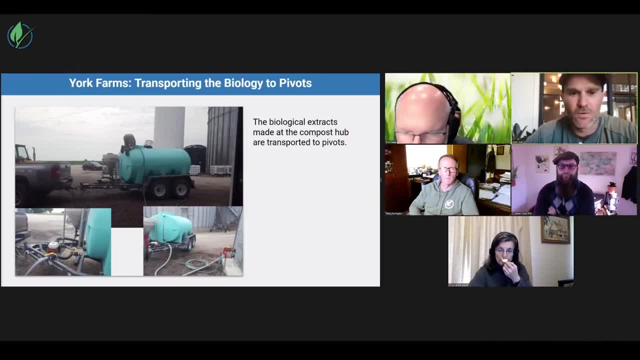 is when you're, when you're, when you're pulling around extract or any any of these biologicals. make sure that you know you're doing your due diligence to keep things clean. um, that is a big deal. you're, um, you're flushing with water. um, you're cleaning. we, we do use, uh, if we get rained. 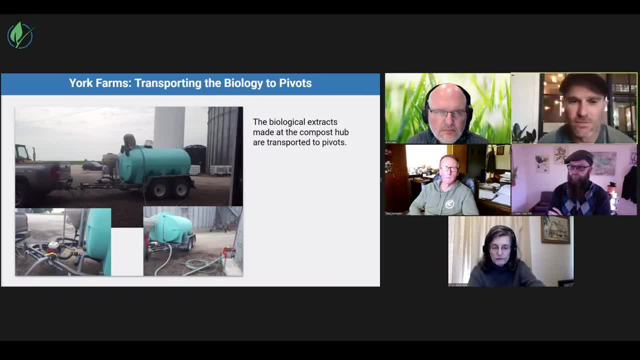 out or whatever we're. we're using a product called sanitate to help sanitize our, our planters, our sprayers, our tanks, um, certain things like that. it's more like a vinegar solution, um, but do your due diligence to make sure that you are being very, you know, thoughtful of and cleanly. 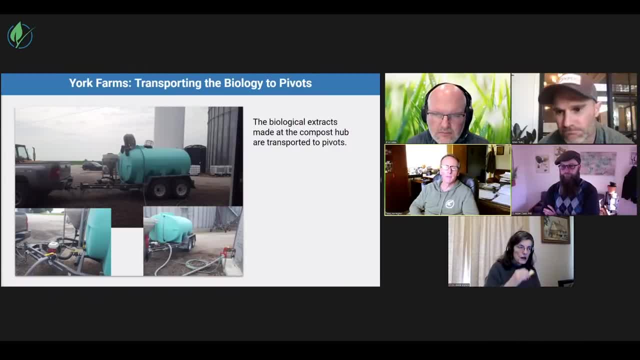 you know, clean- yeah, that's a yes. adam knows i'm a big stickler for disinfecting and cleaning these guys. a great job at, you know, putting a program together. and just just to explain this, what you're looking at here too, and as adam knows what one of the nice things about this system is, it also 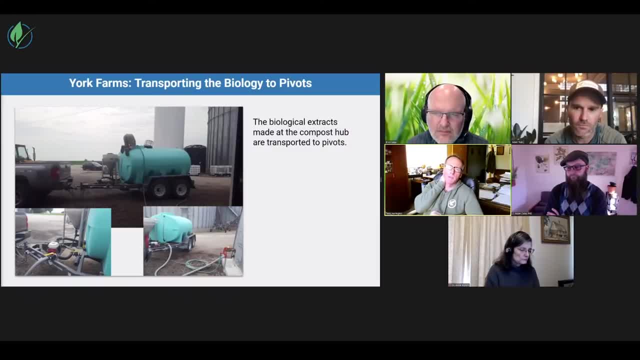 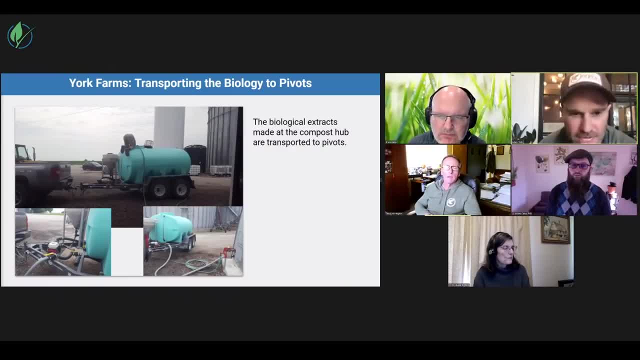 just put it in the tank, it actually circulates it so yeah, and it's actually injecting it right into the line as it going in. so it's just, i mean, it's, it's blending very, i mean, and it's all two inch pipe, which is nice, and then you have a motor so you can run it slow, so it's minimally invasive. 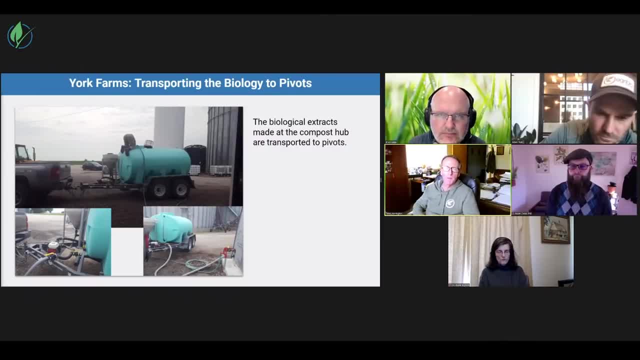 it's not like one speed, some of these pumps. you know you crank them up full bore and you're just slicing and dicing. with this system you can really passively move the biology into the tank and get everything mixed up nicely without, you know, causing too much disturbance. yeah, we've done a. 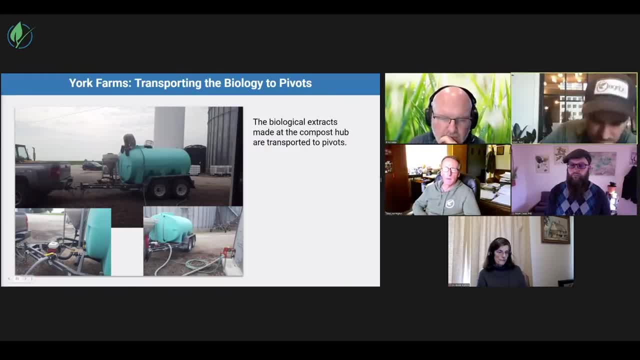 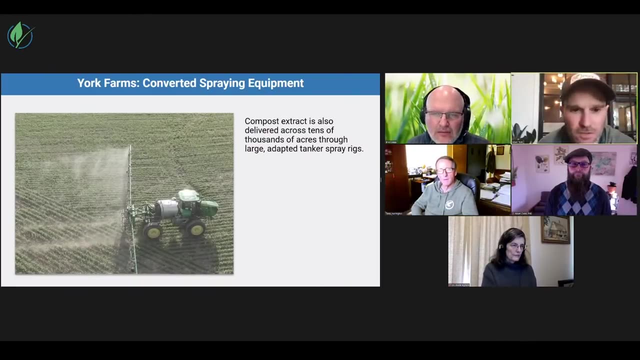 lot of checks from you know, before the pump, after the pump, you know certain things like that to make sure that we're not doing ill harm- yep, or as much ill harm- no, the great rigs, yeah, so uh, this is this one of our sprayers. um, can we start from when you first started spraying? 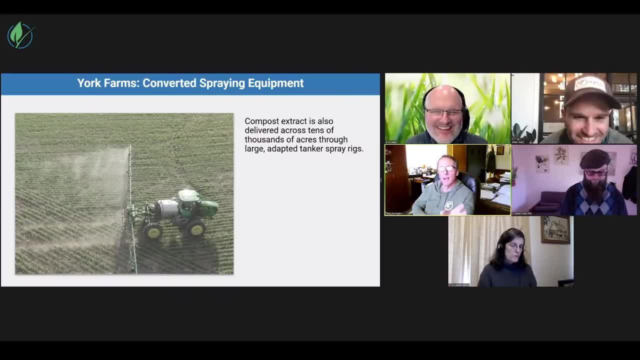 though. so so adam. when i first met with adam, we were spraying. these guys were spraying the extract out with. they only had one rig. i mean, these things aren't cheap, and adam can tell you how expensive they are, and so they were using a existing rig. that was also they were spraying herbicides out of. 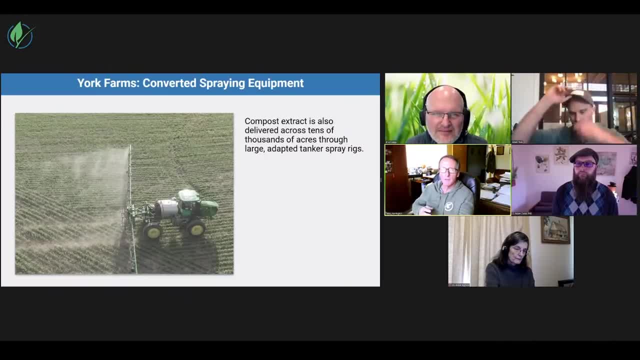 you know, like surf land and some of these other things, and it's very, very difficult to try to flush out any kind of pesticides that are in these things. but when you're first starting off, i mean there's no other way to do it. so maybe you want to just take over and kind of explain how we talked. 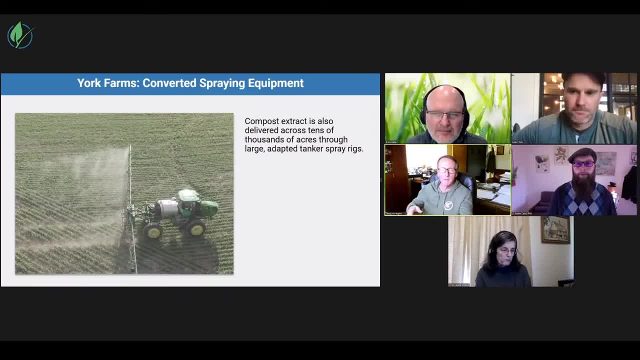 about removing screens and trying to get the materials out and flushing and disinfecting, and and you went to another. so yeah, so it's kind of a big process, but you know we'll do the same thing. you know we're very, you know, just being a disinfecting thing. it's just because anything. 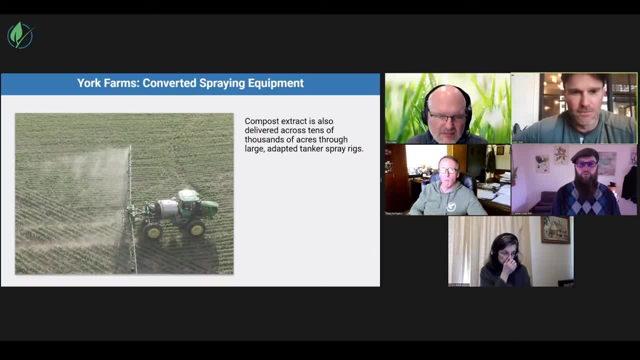 harmful, can i mean you just you don't want to be wasting your time, um, if you're trying to do something good by by smoking it, by just being lazy or or whatever, just not cleaning. so, um, so on these sprayers, you know they have pipes and they have caps and they have, i mean there's, there's a lot of lines and stuff. 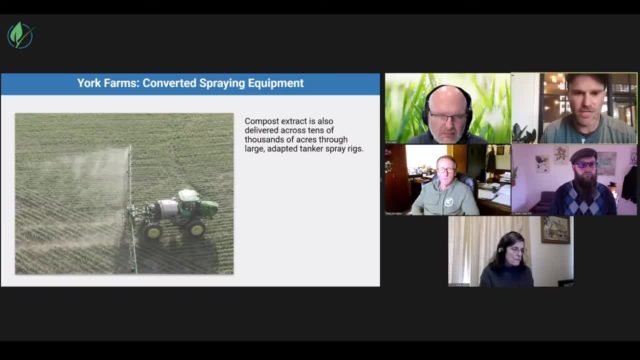 but we did our due diligence. you have to make sure that you flush everything out. um, we used hot water, you know we, we just went through and just pretty much, uh, you know everything. but you know getting inside the lines and getting in there and cleaning them ourselves, i mean we. 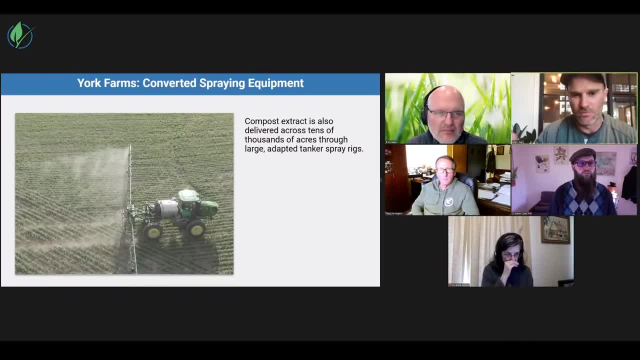 we pretty well. anything and everything you could clean you did. we put new sight gauges on them and ran sanitate through them. let them sit in the booms for a day and then at the end of the day or the next day, you flush it back out with with warm water and uh, and get these. 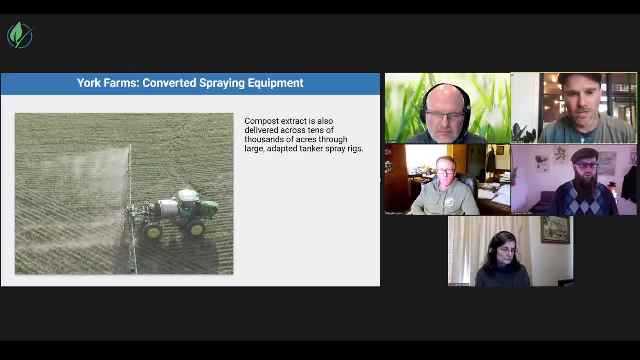 things really clean, um, we took. so when we were running compost, we were, uh, we're compost extracts. we were running a 50 mesh screen. we were taking some of the other screens out, but we would keep the 50 mesh in and um would really be pretty good because actually we're screening it with a 50 mesh. 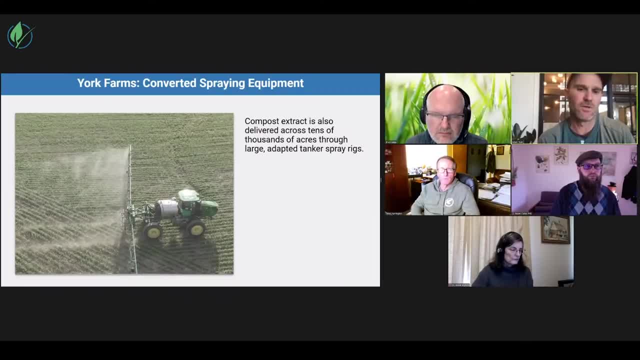 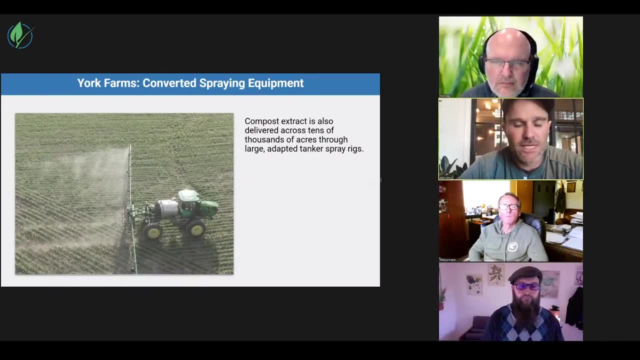 screen before it hits the tank. so it's it actually works pretty decent um at that. um, we've used some oh turbo t tips um oat sixes. we've had pretty good luck with them. um, you can use a flood tip. you can, you know, use whatever, but the bigger, bigger the hole, the better off you're gonna be, just to help. 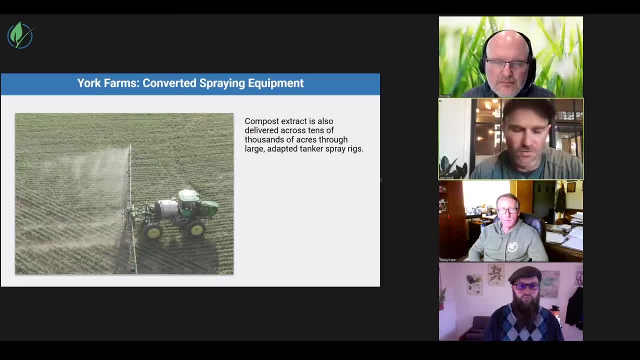 you know, from plugging tips with, you know you're always going to get a few fines in there from from any extract or any compost source, um, and that's really good stuff. but you want to, you want to keep it, you just don't want to. you don't want to also be cleaning your tips. and you know, times times, money sometimes. so 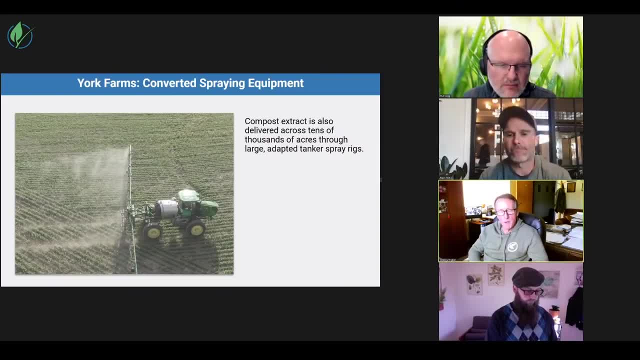 yeah, the key is really to get as much volume out with minimized pressure. and adam kind of knew this right from the get-go. and looking at all the different tips- because these rigs have multiple tips on a spiral- uh, on on that boom. and uh, adam, i don't know, did you actually have to get hips or did you have tips? 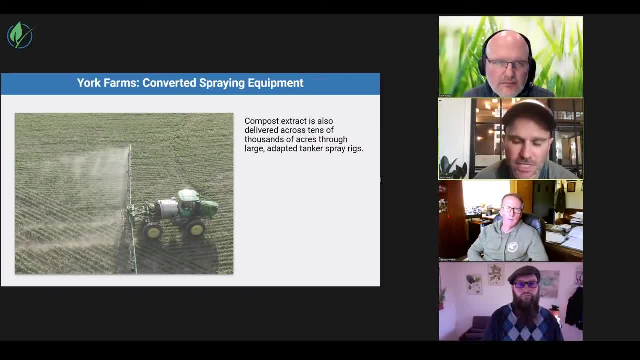 on there already that you could do. yeah, we had tips, you know, and each tip just depending on what we were trying to accomplish. you know, we were trying to keep the psi somewhere, right, you know, around 35, 40, you know. um, you just didn't want to be blowing it out there- 60, 70 or 80, you know. and 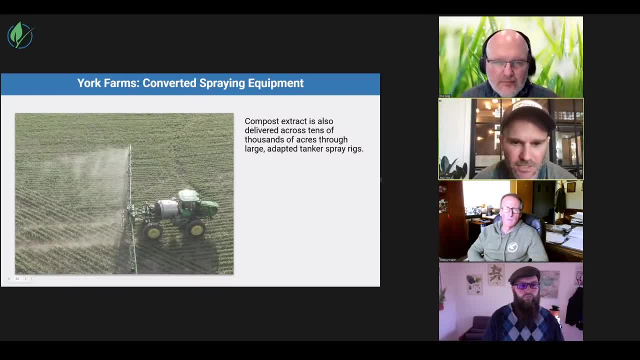 and doing a lot of damage. so, um, a lot of guys that do a lot of their own spraying, they, they kind of have an idea, you know. they're just doing a lot of their own spraying, they they kind of have an idea, you know. but we were doing 15 gallon the acre um using uh, tjo6s um and having really good luck. 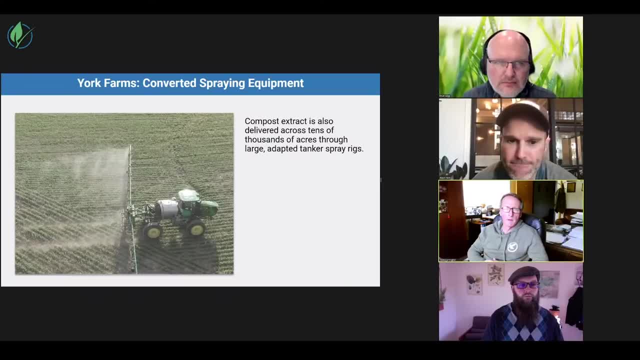 with those. yeah, so then you ended up going from uh, one rig that did it all to actually dedicating and getting a sprayer just doing biologicals and uh nutrients. yeah, like i said, we're heavily invested. now we got a new shed and a sprayer. so, uh, what does a rig like that cost? i? 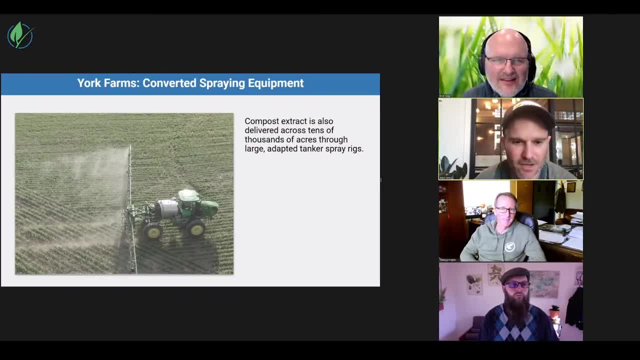 guess, just so everybody knows. yeah, they're expensive. i don't know they're more expensive now because everything's went up, but i, you know you're gonna spend 300 on one, pretty easy 250, 300. so what size boom is that one that we're looking at? that's 120 foot boom there. 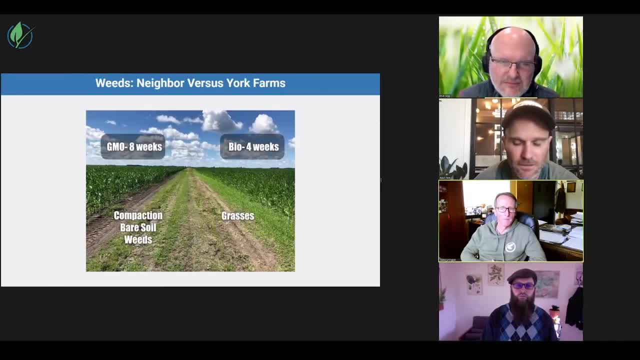 right, great, uh, there we go. yeah, so this is a cool picture. um, that's the one i was talking about earlier. yeah, yeah, so this is one of our farms. here we have a neighbor conventional farm, we have a lot of our farm on the left and then our farm is on the right. um, you do see? um. 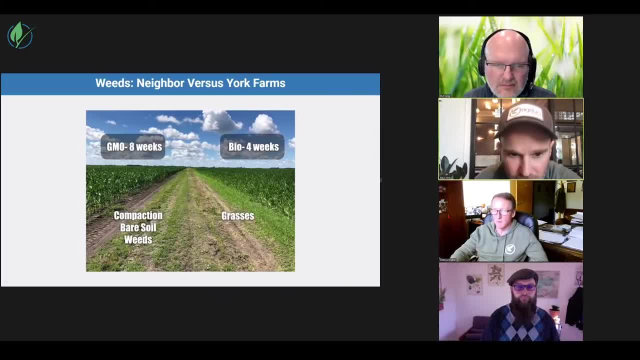 you know we have cut. you know a lot of these things that i talked about earlier. we've cut out and you can kind of see. you know, you can see that the crop on the right, even though we're doing a lot of things different, looks very beautiful to me compared to, you know, the conventional side. 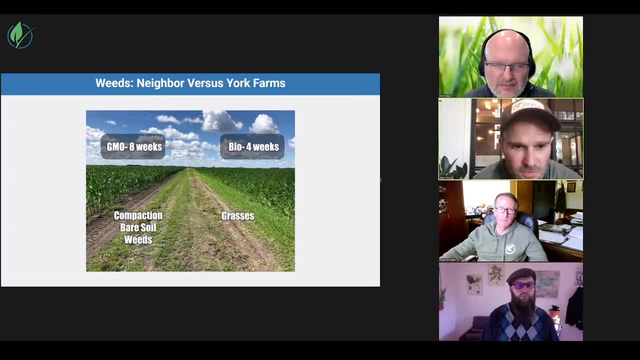 um, that's what's when you kind of go through this transition. this is something that's really interesting because you'll get a lot of neighbors- or i've had a lot of neighbors or around us that are conventional and the you know they're talking about just somehow or another or 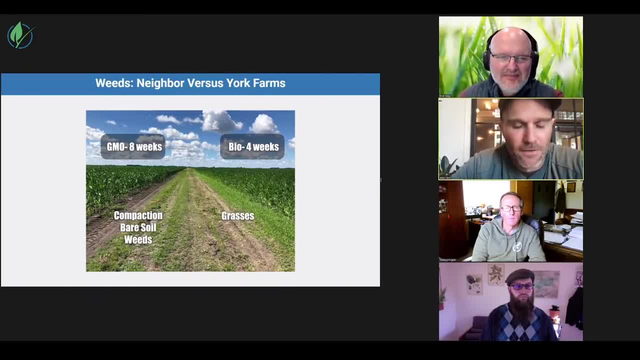 behind your back or to your face or whatever. but, um, you know, a lot of these crops are artificially that these, these, uh, conventional guys are growing, are artificially painted, you know, with high nitrates. so we've, we've tested neighbors and our, you know, ourselves too, with, with, with having so 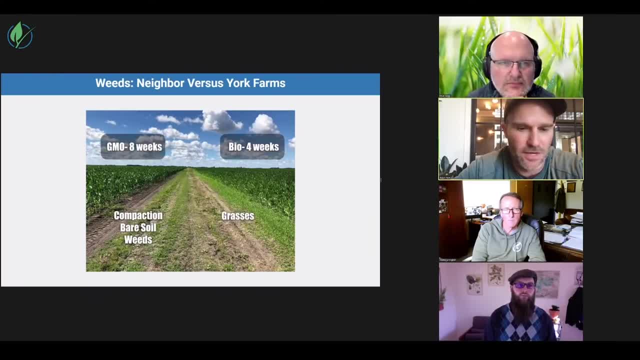 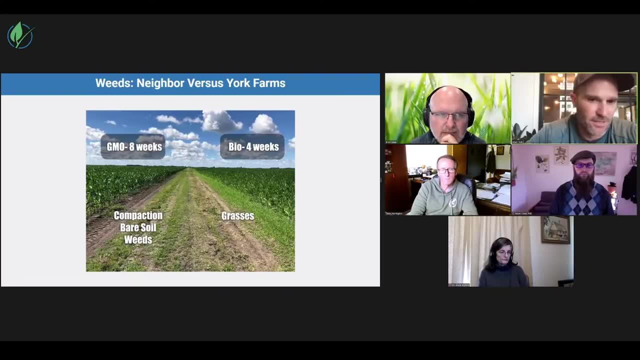 much nitrogen down on this conventional stuff. they're just. the nitrates are sky high, um, and you know it's bringing in, you know, disease, insects and everything else under the sun. but, um, you know, so when neighbors drive by and the forest is not as green, you know they'll, they'll, you know um get. 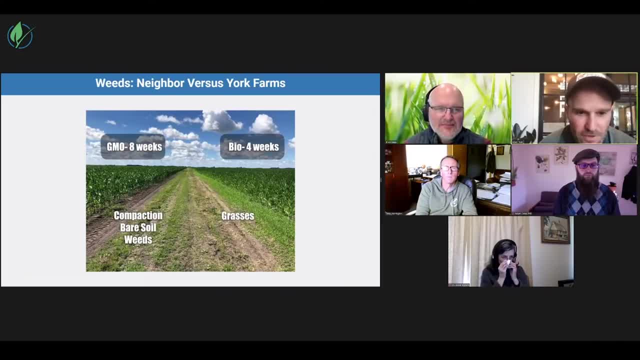 get on you a little bit, but uh, but once you start really figuring out why there's just so greens, um, it makes complete sense. yeah, but we're seeing, you know, where everything's dead on their side. um, you can see on our side where we got a lot, of, a lot of grasses. 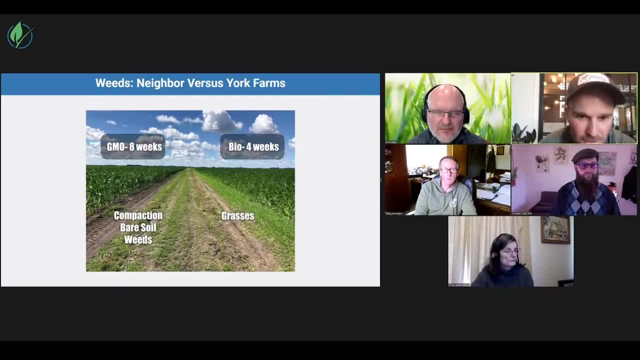 um, um, that are, that are growing and um. so yeah, we've, and we've also fought different weed species and what a lot of our neighbors have had. we've transitioned to more grasses and and not so much of the, the pigweed and the waterhemp that a lot of other guys in our area fight, which are actually on. 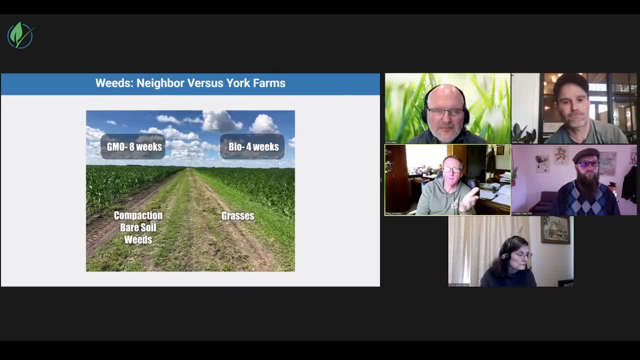 the other side. we'd see- you can't see it from this picture- there's patches of waterhemp and pigweed throughout that field, and on your field you just couldn't even find any. it's just mostly grasses without any particular species, and and so we will share some of those with you later, um, but 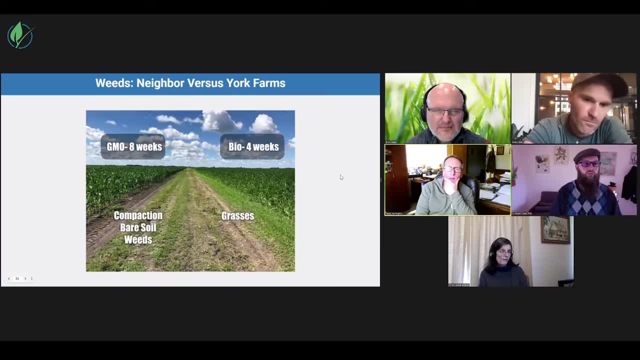 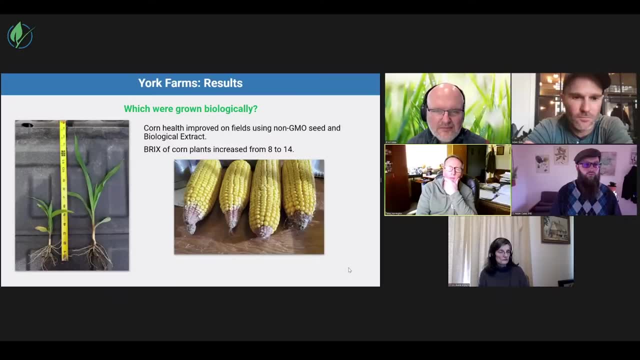 thank you so much. that's awesome. well, we do have another question. that's really cool. um, so, dollars and cents, adam, you know, like by the acre? um, what kind of what would the yield difference be between the neighbor on the left versus what you yielded? that would say that year? 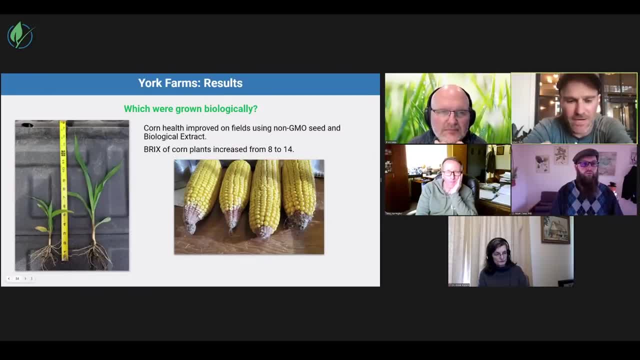 and but, and then also, what would the cost difference be roughly, and what he would spend? an acre, his cost versus your cost? and you know, um, oh, they're still your friends. i'm joking, yeah, i mean, you know, you know, we all, we all, you know, have our, have our own thought process, but you know, they're still our neighbors. 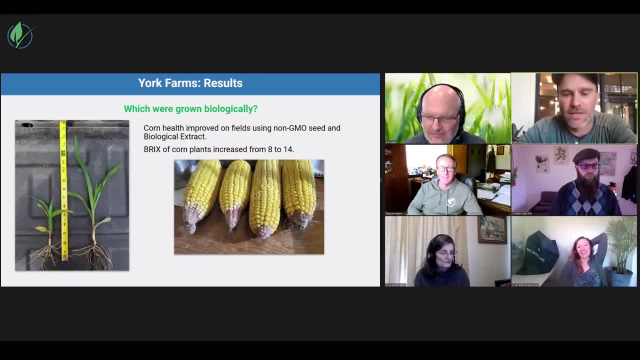 and you know everything else and uh. so the, the guys that are doing the conventional, are just mainly focusing all their money on um obviously, potash, which is potassium dap, uh, which is phosphorus, um anhydrous ammonia and um doing a lot of roundup um. so by the time that they get 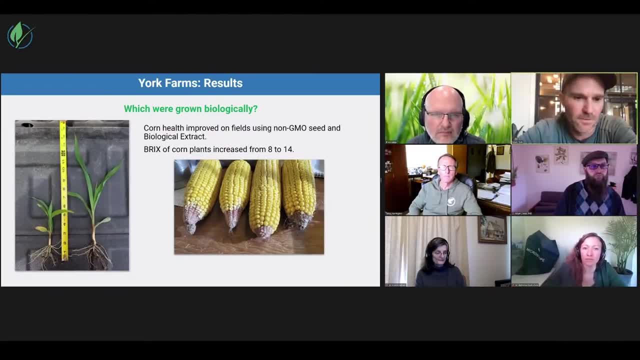 done, spending their money plus doing a lot of seed treatments. um, i would say, doing the way we're doing it and going to the non-gmo we're, you know, somewhere between, depending on the farm and your situation. whatever, you can easily be 100 to 150 dollars an acre cheaper than your neighbor. um, 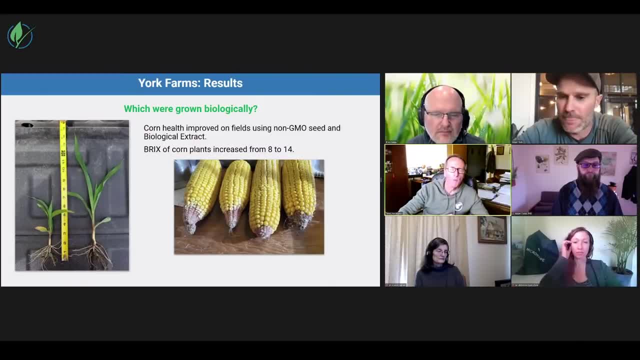 but what is that a dollar? i mean like what would it? what do they spend an acre? they spending 500 to 800 an acre. now, well, every you know that's, that's, that's always. that's a loaded question. um, because everybody has different. i mean inputs or inputs, but people have a lot of 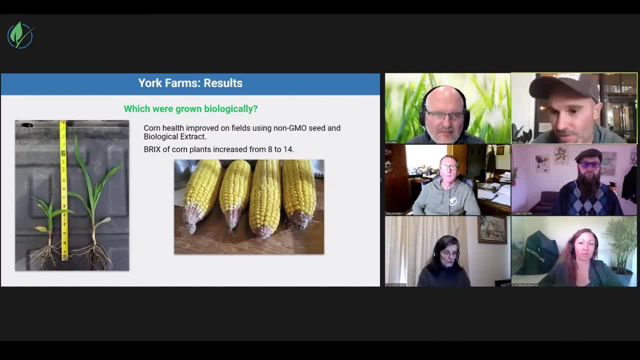 different overheads. some people are paying 500 cash rent, you know, um. so everybody is that's a loaded question, it's that's a hard one to really answer, to be honest. but general generally, that type of crop that's uh, you know, uh feed corn. it's grown conventionally. i mean, there's got to be some. 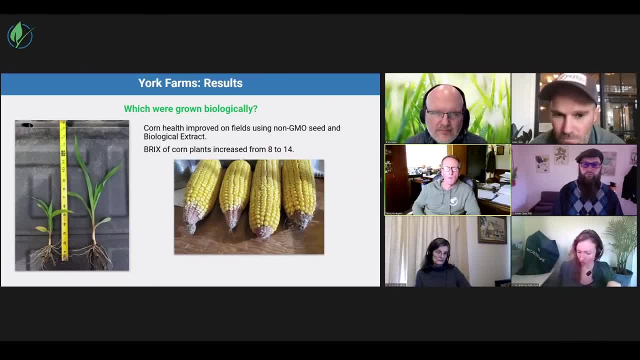 generalization to what these guys are spending with gmo corn and all the inputs. but yeah, i mean, i'm here to tell you that gmo corn is going to cost you 320- 330 a bag if you go fully traded, and non-gmo is going to be 150 to 170 um. but isn't it conceivable that these farms, these guys, could be spending 500 to 800 an acre all in. oh there's, guys got a lot more money in it than that right, right. so you could, what technically you could save? you could cut that in half right within three to five years, if not more. yeah, i mean you. i don't know if you, i mean you're never going to change your land. 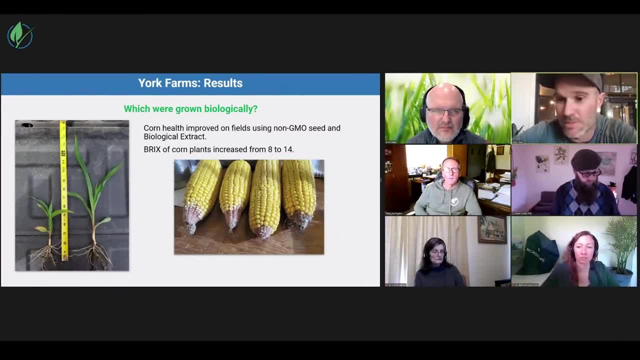 expense is going to be your land expense. you know your. you know your fuel expense goes down. um, you know your insecticide expense goes to nothing. if you choose to do that, your your seed corn and seed beans. you can. you can cut a lot of that out. um, you know. so you can cut a lot of your. 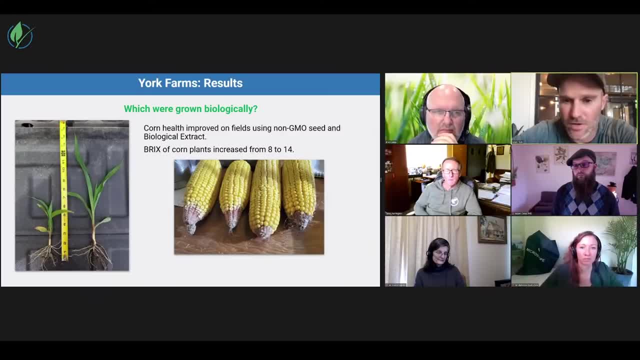 inputs off. but you know, some guys have. you know the per acre cost. it depends on what the guy's overhead is too. you have fuel, i mean, you have uh equipment, you have land costs, i mean you have a lot of that type of stuff. but on the input side, yes, you could cut a lot of that. 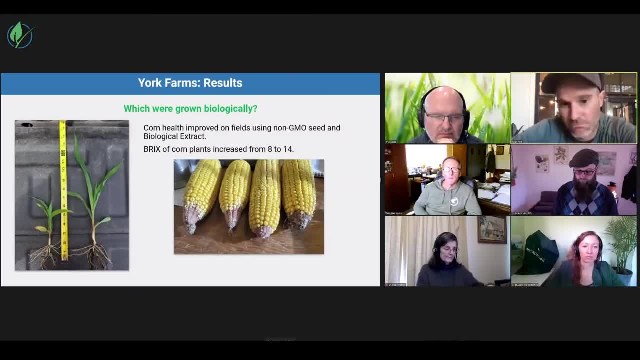 down by 150 dollars an acre- pretty easy, depending on you know how you choose to go, but um, but i think in this picture here we've tested a lot of uh bricks on a lot of gmo plants over the years and um, it's all relatively pretty similar. every year is a little bit different, but um, and you know, this is these. 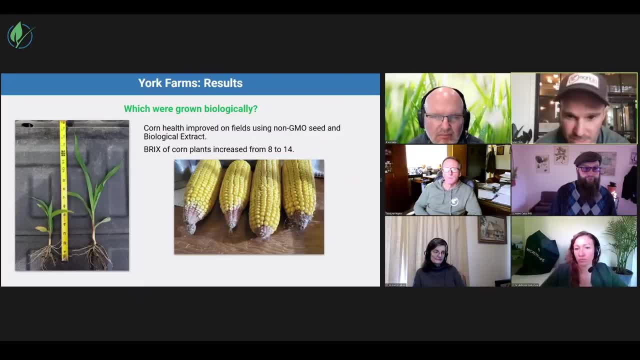 are? these are gmo plants in a, in a non that we've tested against in a non-biological system. um, if you you know, a lot of times we'll see bricks levels from four to five um, we have seen them up to eight um depends on this year, but um. but when you start getting into the biological program. 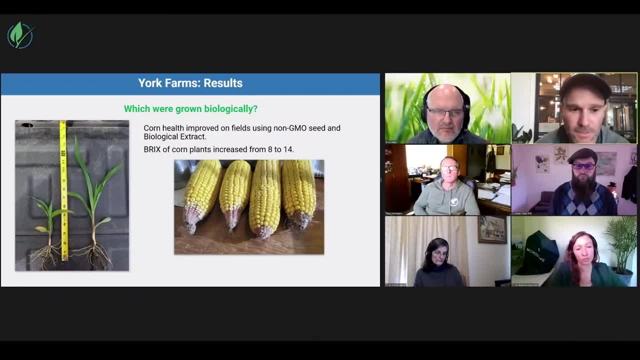 and you get more into the uh gmo crops and just just doing things better. um, you see that bricks level jump up and be twice. it's not not hard to see that be twice as good as what. um, um, some other guys around the area are doing so. the other thing that's kind of really interesting about this picture: 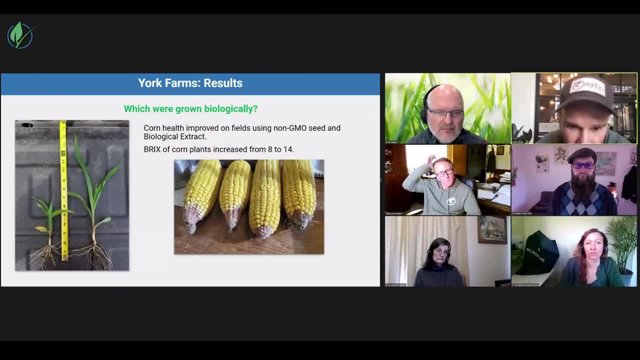 is where you have the ears of corn. we've seen this a lot, um and a lot of growers around. uh, the area is, you know, they're spreading a lot of high rates of fertilizer, high rates of nitrogen and really boosting that energy up early, but uh, you see the tip back really bad, late. 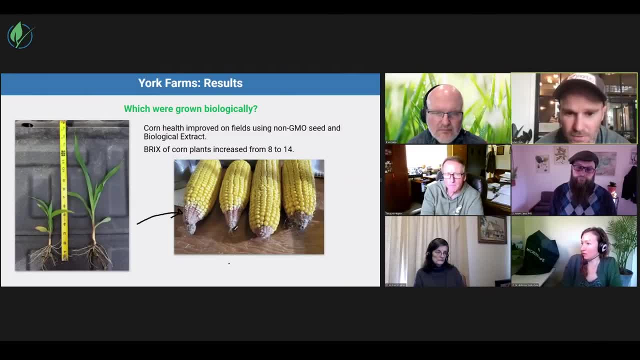 um, where what we've been doing and trying to feed the, the crop, um, you know, throughout the season, um, not do everything at one time. try to keep that energy level up and you know your biological activity fed and and going, you can do a lot better job of. 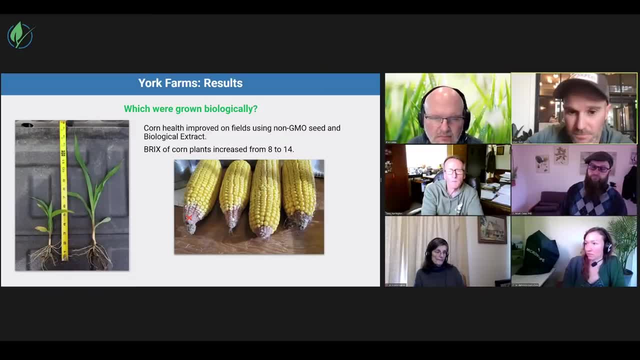 being able to fill that ear out to the tip. um, and at the end of the day, when you're trying to cut costs early, you have more money that you are able to spend if you need to late in the season, you're not budgeted out at the end of the day. so, um, those are some things. 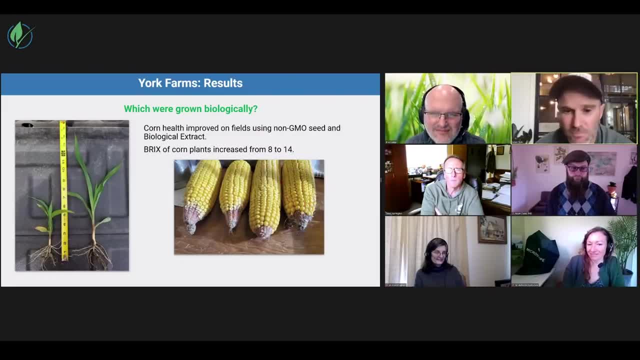 that we've seen and it's been, it's been, it's been very rewarding, um, to be able to see that and try to figure that stuff out, because years you know, and the methods that i was farming and grew up and taught farming i mean it was, it was very typical to see that tit back from year to. 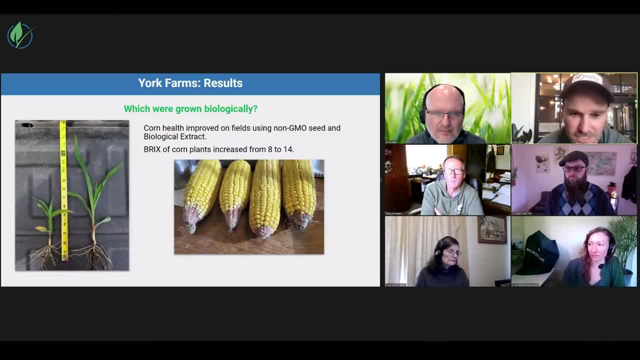 year and it was like, oh, it's normal health. everybody said, well, that's just you, just you know, got the right population. and no, that's not normal. that's money and effort that you spent, that you did not fill out your, your full potential. is what that really truly means: well and adam for folks. 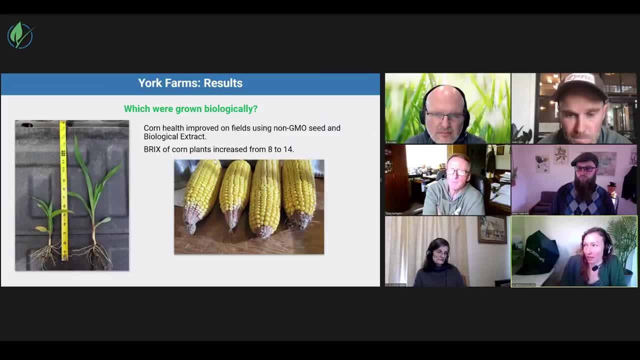 who don't haven't worked much with corn specifically, um, help us understand. do the kernels, the kernels back here are the ones that develop first, right? so this tip back really means that it like was boom, boom, boom and then ran out of steam? yep, ran out of steam is exactly right, it just ran out and 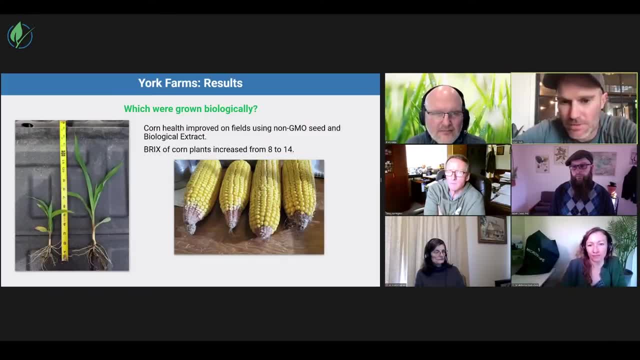 started cutting back and, um, it would go like you know, probably you know real similar for certain crops, whether it's soybeans or whatever, and you don't. you had the pods that were created, you know, and the beans that were created, but you did, you ran out of energy and you didn't fill them or they. 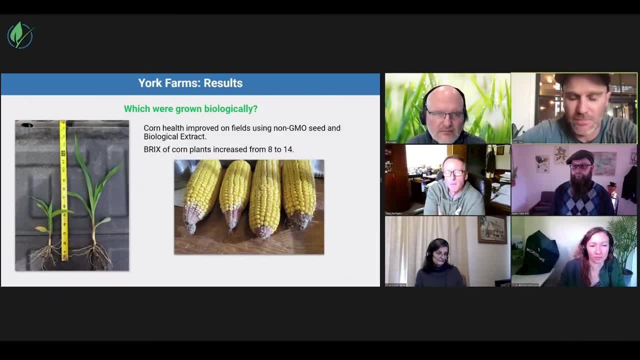 you know they have blanks or or whatever you know. the other thing about any grain crops that we've been growing is is: um, you know the the more nutritional, the more balanced you are in everything: biology, minerals, you know everything all around- the the more balanced your crop is going to be, the you know. 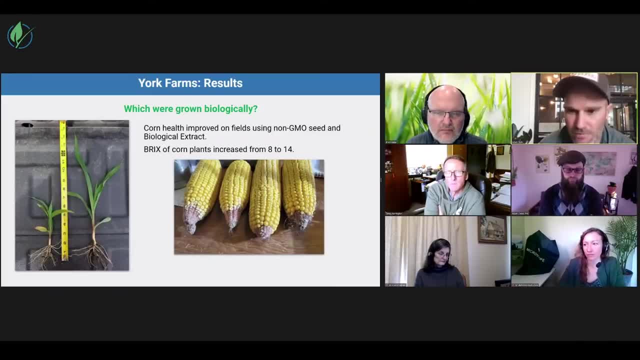 the better your the fruit is going to be, the better the the grain, or however, it's going to be more nutrient dense and it's also going to have a lot more weight to it, as well as what we've found. yeah, so it's more nutrient dense. when you talk about energy, adam, um, i'm assuming you're talking. 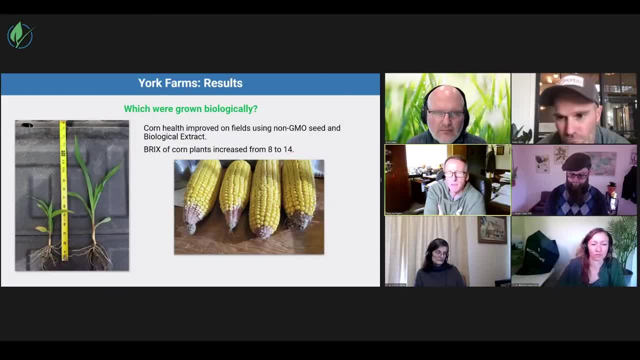 about all things like maximizing photosynthesis, converting complete proteins to- uh, completing, you know, having the, the nitrates convert to complete proteins and then you get lipid production. so your plants are going from an active to passive resistance and so you have a really you know, all in all this energy. 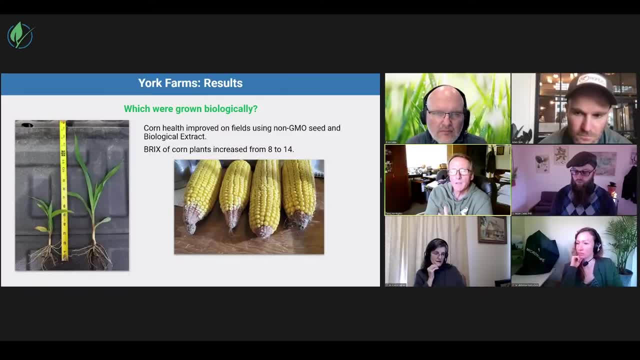 are you talking about all the different things that occur both biologically and chemically? or are you talking about certain minerals like nitrogen? yeah, i mean nitrogen's part of it. you know getting that converted over to an amino acid protein, you know, as soon as possible, um. 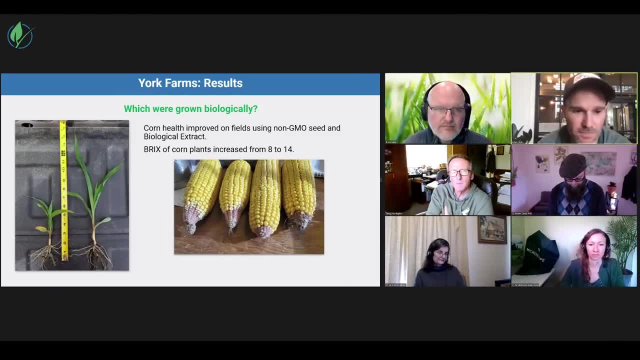 yeah, it's, it's everything. uh, you know, i mean um, it's biological, you know, and keeping. i think a lot of the energy has to do with keeping your biological fed, um, and keeping them active throughout the growing season. i mean, it's just just trying to keep that energy. 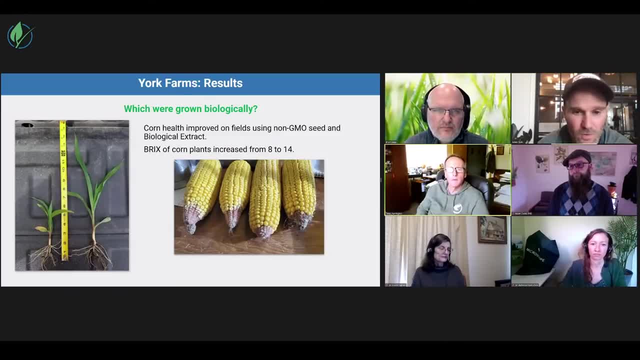 up throughout the season, um, you know, if you're running low on a, on a specific mineral or whatever that is, you know, um, so we can see. if we can theorize, then, that, because of all the biology work that you've been doing in your soils, now it's actually maintaining your minerals or your 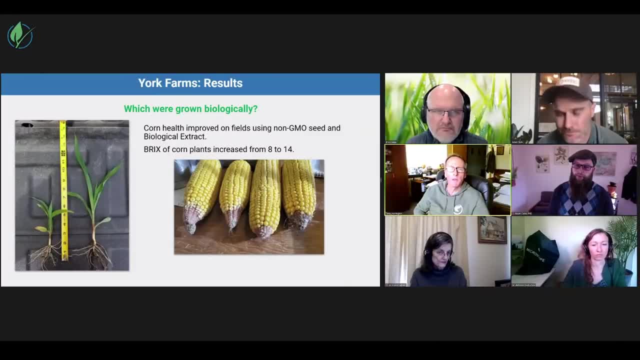 energy and you're able to keep that energy up throughout the growing season. i mean, it's just keeping that energy in the soil once it didn't have that charge, or that you know the battery in the soil, so that what you're seeing is contributing to the kernels probably growing out there. 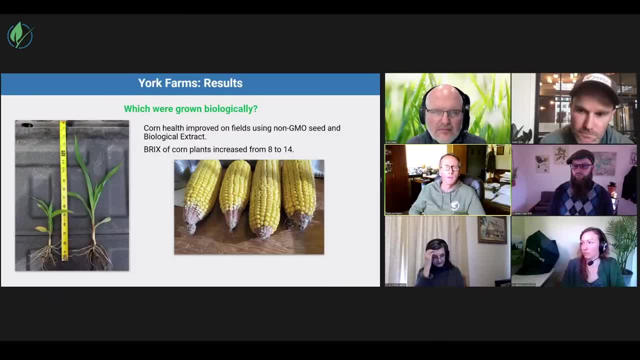 further, right, and then you have this longer term energy. yeah, and i think it has to do with that and also, like i said, is is keep keeping them fed and just keeping making sure that you know you're doing the best of your ability to keep you know things synergistic and not so. 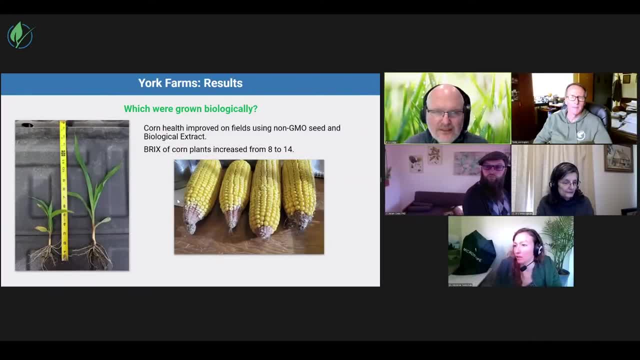 oh, we lost that, we lost him. i think we just lost out. well, i was. i was gonna also say: you can even see it right here, right like so they both, all corn plants, have these support roots right, these wide ones that are out there to help keep them upright, and that's what the western corn rootworm will. 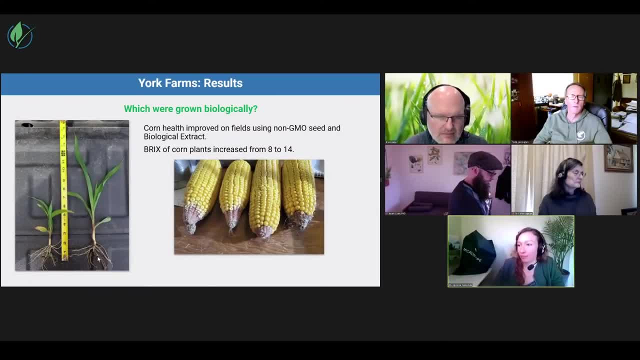 attack and knock, knock the plant over, um, but the fine root hairs- you can see the amount of just detail in there. those are the surface areas that are enabling microbes to access and exchange with the soil, and so that's what we're doing right now, and i think it's a really good idea to do that. 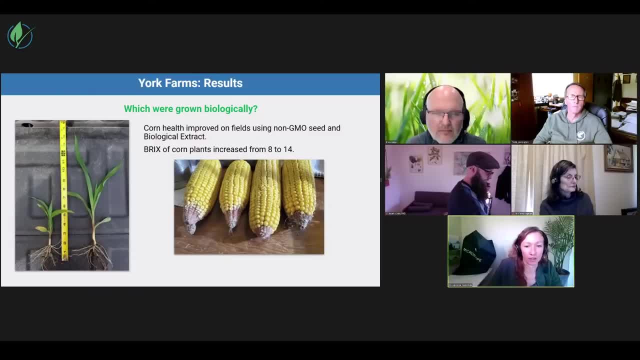 plant. that enables that plant to have that long-term seed production throughout the season, one of the things that brad's been really- i mean, adam and brad have been really great about. we're not only very intelligent farmers, but they- they do a lot of work also. looking at the bricks: 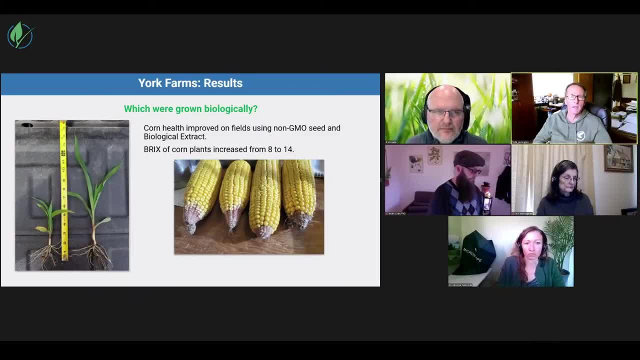 and the sap testing. they do quite a bit of sap testing and they do supplemental foliar sprays when and if needed, while these crops are going through this transition of, you know, being chemical dependent to more biological plants, and so that's what we're doing right now and i think it's a really 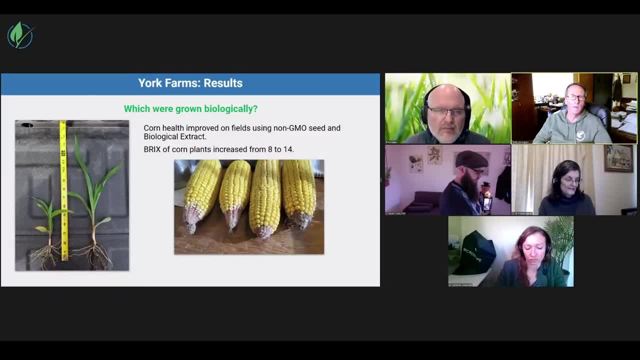 good idea to do a lot of work. also, looking at the bricks and the sap testing, they do quite a bit of sap testing and they do quite a bit of sap testing and they do quite a bit of sap testing and they do, and they've been really innovative with their foliar sprays and i think that's another reason. 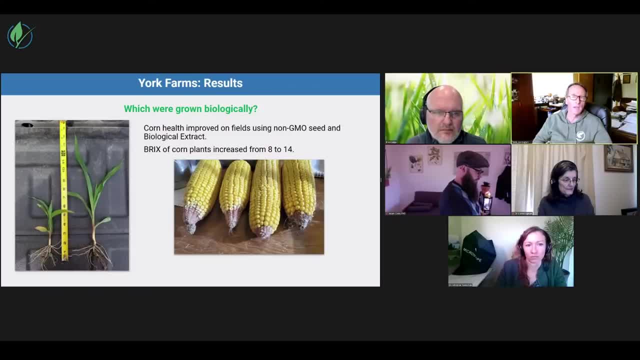 he talks about this extended uh energy they're getting. i think some of it also has to do with the sap testing and foliar sprays. unfortunately he's not here to ask the question, but, um, that was one of the things i did want to ask him. so do you know if he has? you know he extensively assesses. 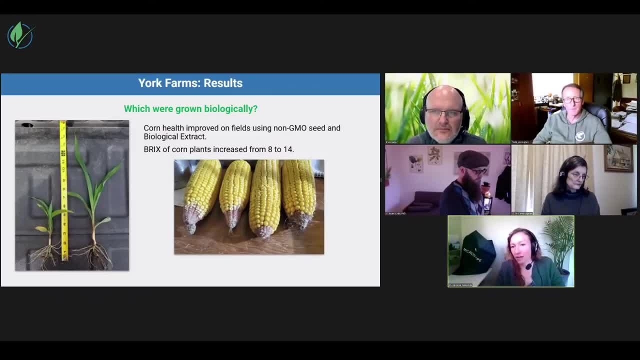 the biology in his soil. so he, theoretically, would have data that could be used to assess the biology that could be correlated one to the next also. right, absolutely, oh yeah, that would be a beautiful thing to start playing well, and that's a lot of the work. i think that the future of all the work, 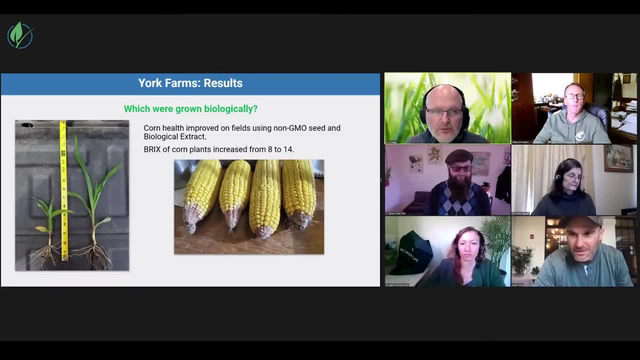 that i'm doing is- and i'm sure todd's same way- is: how do you become much more specific in that transition period so you can reduce the amount of those inputs that the farmers are requiring to maintain the production while you're doing that transition and if you get very prescribed and 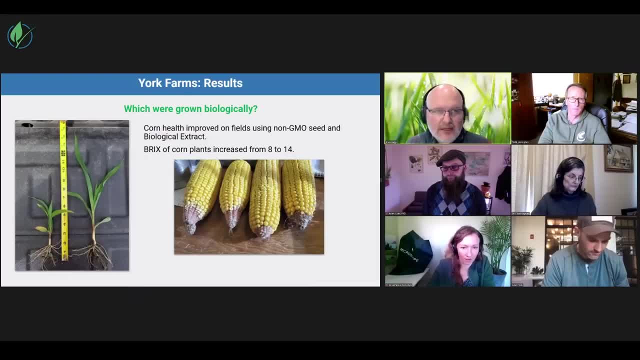 you can minimize the amount, then you're having less impact to the microbiology. i mean, that's you start putting on those agrochemical products, you're you're taking some step backwards. how can we minimize those taking a step backwards while we're going through a successful transition? yeah, 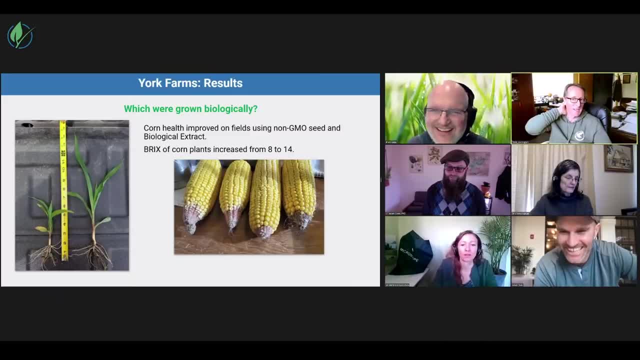 right, oh, we got back. yeah. so, adam, one of the questions i was going to ask, yeah, is that i? i just assumed that this was the case too, but i had mentioned that you guys are really, you know, very intelligent farmers and have done a lot of work with sap testing and doing. 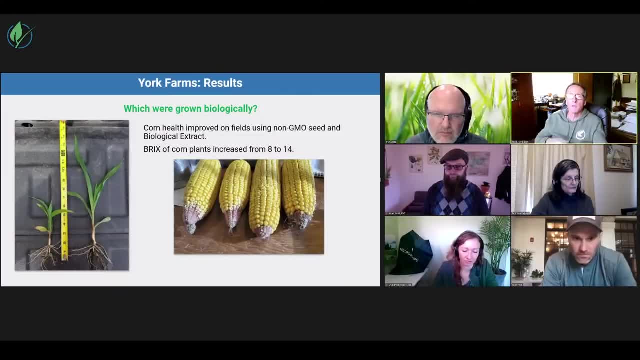 foliar sprays as supplemental sprays, going through this conventional to more sustainable biological program. so maybe you could touch a little bit on the benefits of doing the sap testing, doing the foliar sprays and and being able to. you know how that's part of this energy, you know regenerative. 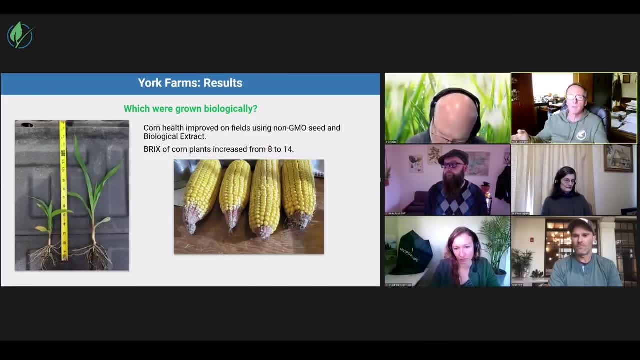 energy, uh, or reduce energy that you're not getting as much of, because you're doing the sap testing in the foliar sprays. yeah, so i think it's. i think it's a good thing to be able to test your. your sap test is, you know, throughout the growing season. i think it's great to test, uh, take samples of. 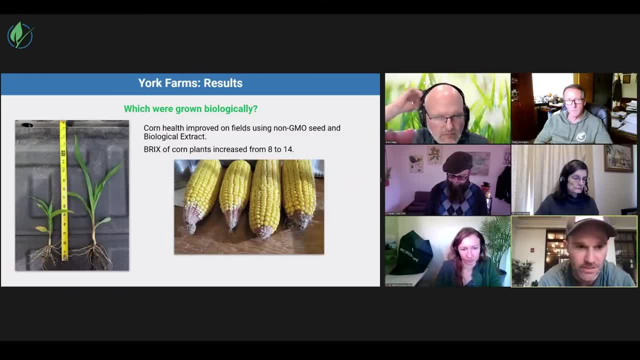 uh soil, kind of see where you're at biologically as well um throughout the season and just try to adjust accordingly. i think if um the the foliar sprays are very beneficial, um, the one thing that we've been working on- uh we've been doing a lot of testing- is uh mixing some minerals with the. 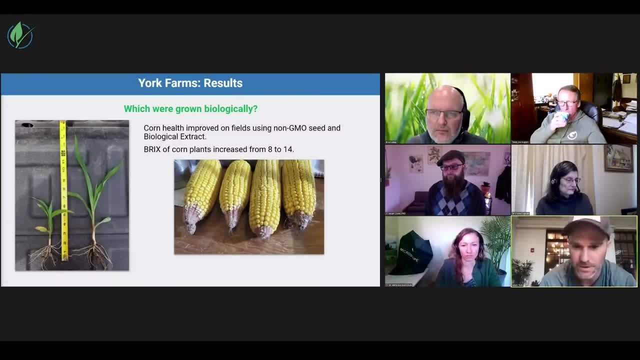 compost extracts as well. we've been doing a little bit of work with that, um, having pretty good luck with that. haven't done a lot of it, you know, in the past i've kind of played around with it, but that's something that we're going to be really looking at. um, you know, bringing some of the minerals with. 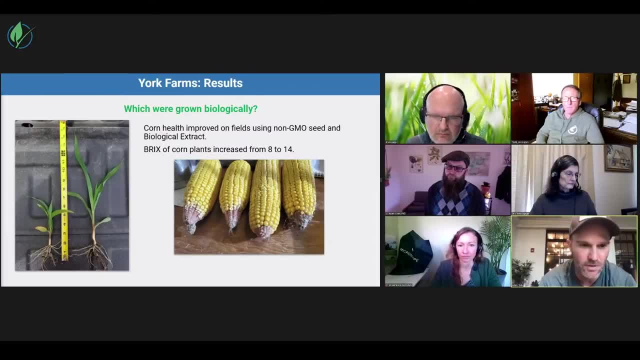 the with the biology, um, you know, through certain testing, if you need those, those minerals as well. so, um, and that helps with the energy and just helps, you know, increase your, your bricks. um, you know, and just, and doing the due diligence, you know, having a refractometer and and uh, doing you. 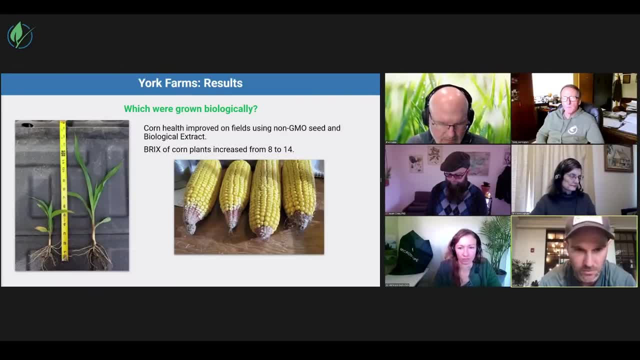 know whatever foliar sprays you're going to be able to do that. so i think it's a good thing to have a foliar spray that you choose to do. but you know, make sure that when you're doing them you're checking your bricks and you know you're if you're getting the, the jump um that you're looking for. 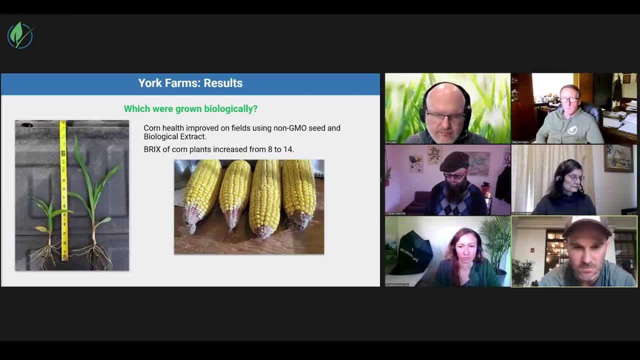 then you know that's a good way of testing and then you go to maybe doing some more acres with it. um, if you're not seeing that jump, try to figure out why you're not seeing that jump. um, if there's something in the mix that's maybe not um rolling like you wanted to um, so that's. that's a lot of. 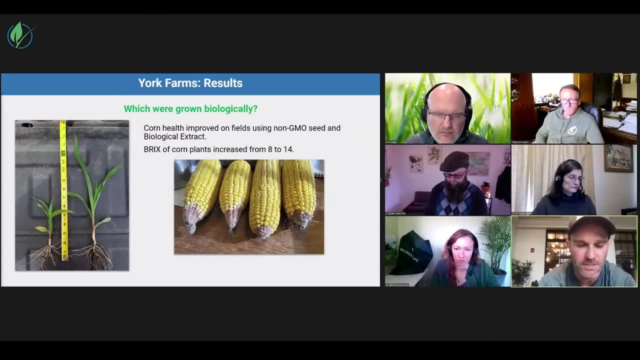 things that we've been we've been doing and haven't been been very successful. if you're not doing that, um, yeah, yeah, so when you, when you're adding a foliar amendment to a leaf, forgive me for not understanding the theory, but is the theory that that is then feeding and stimulating microbial? 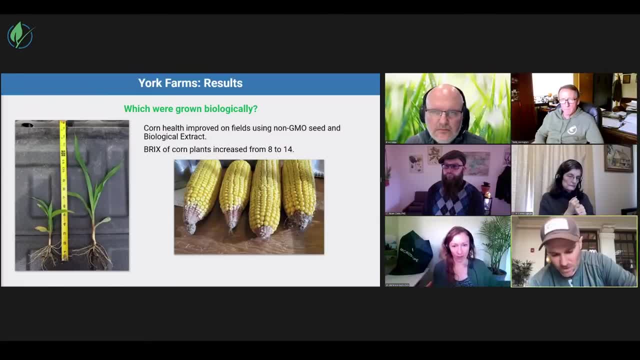 growth that then protects and and supports the plant. yeah, so, if you are, you know, kind of. what we found out too is if, if so, over the years of weed, degraded soil or some farms have been degraded, you're not having the organic matter and you're not having the organic matter and you're not having. 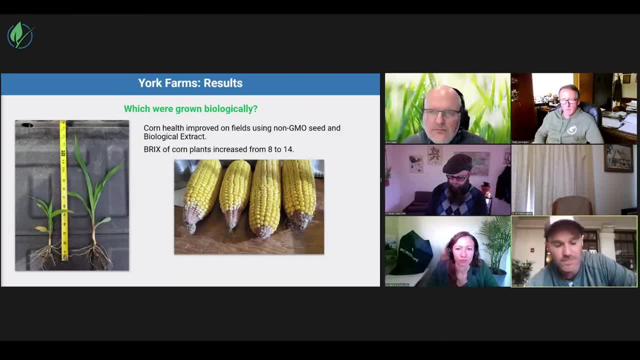 the organic matter. you know there that you would, um, you had 60 years ago. so some of these negatively charged minerals are not just and depend on your situation too. if you have, you know if you're sad, you know if you've had too much rain or you know, uh, we've, we've kind of fought, uh, like boron. 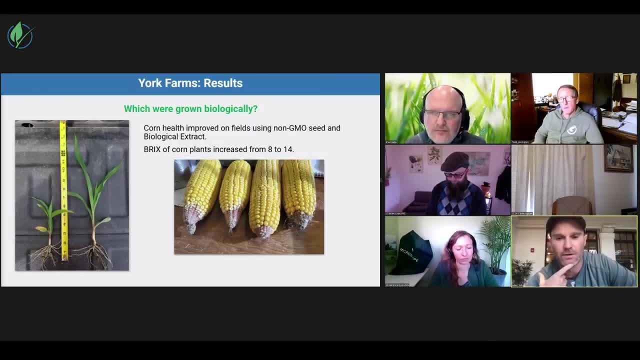 for example, you know we've had to feel like we've had to add boron, um, to get the levels up with it, um. so, yeah, just just doing all the due diligence, i think, with testing and trying to, um, you know, only add what you need to, but also be very balanced about how you're adding things. and 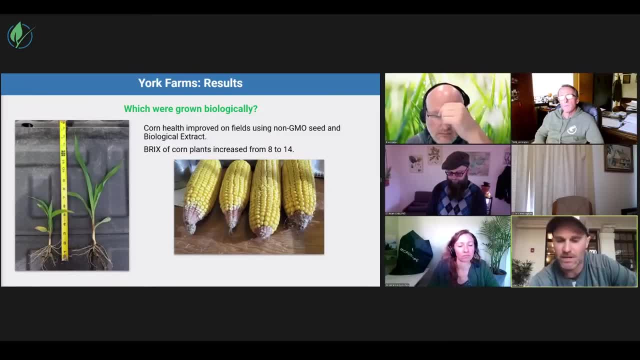 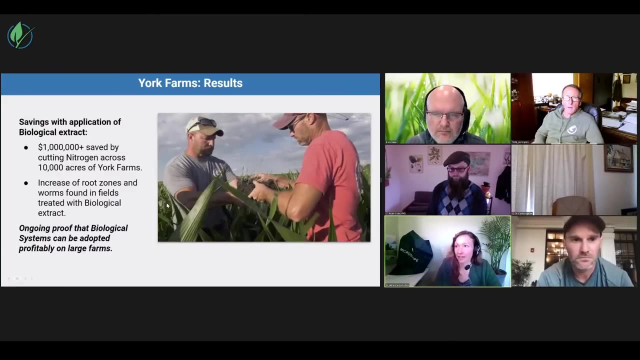 and when you're, when you're, uh, applying a good foliar, you're, you're raising, uh, the bricks in the plant and you're, you know, you're photosynthesizing at a higher rate, which, in tune, is feeding, feeding everything in the soil. so rock on, yeah, and then you get these benefits. oh sorry. 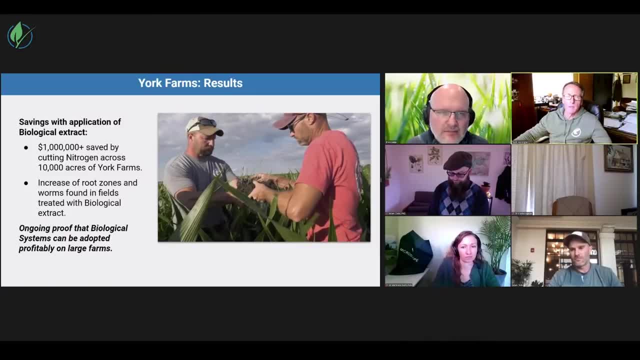 i think one of the things that we're seeing happening, especially with adam, is that because we do a lot of work with companies, we do a lot of work with companies we do a lot of work with, we do a lot of work with companies, we do a lot of work with companies we do a lot of work with. 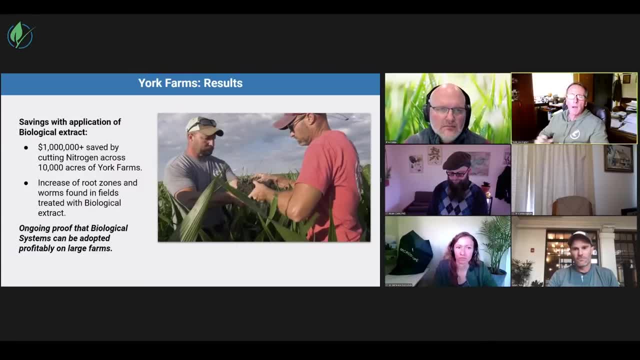 compost and we're looking at putting minerals in compost and letting the microbes solubilize and convert these minerals to more plant available in the microbial biomass. and with adam you know he's, he's applying these, these trace minerals. he's kind of looking at it like you know, clients and farmers. 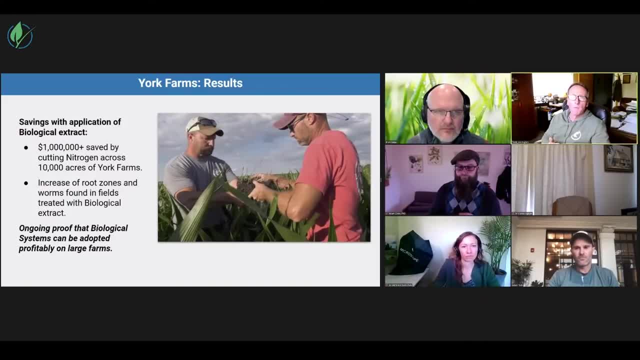 will use foliar sprays either in a chelated form or in a cation form. right, and it depends on you know what crop is spraying, why they're spraying this. but i think when we're applying these minerals, these these trace minerals, and we're looking at putting minerals in compost and letting the microbes 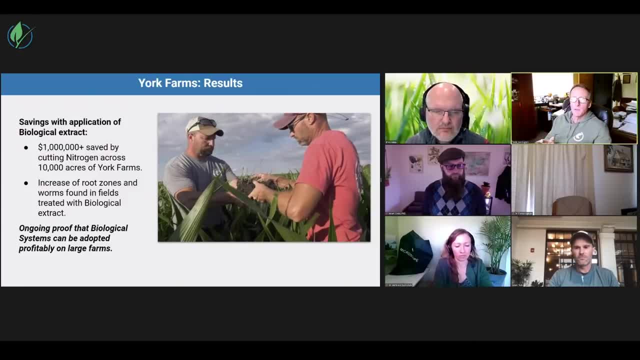 and we're looking at putting minerals in compost and letting the microbes with biology. the biology has the ability to break these things down further, like a chelate, but it's in the biomass of the microbes, in the, you know, the bacteria and the fungi, and in nature we all know. 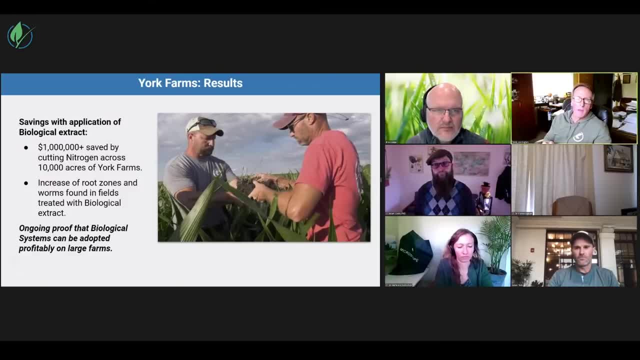 that plants should have the biology and the leaf surface right that that that film should have that biofilm on the plant. so when he's applying these extracts with the trace minerals, he's getting a better response for that because of that fact and you're using less of those trace minerals. 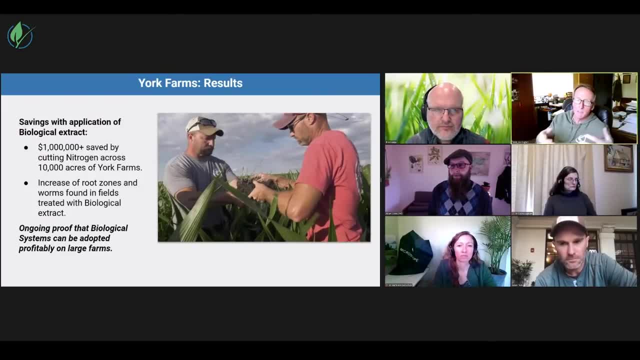 and getting the response. so it's almost like a chelated response, but it's actually a biological response because of the enzymes and the organic acids. correct, correct, right. and that's what. a lot of the minerals that we're using already you knownel chelated with amino acids, organic acids. they have humich in them, you know some fulvic, they're not. 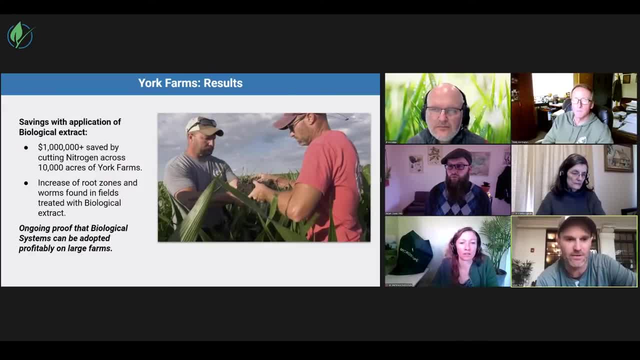 ebta, like a lot of other products sold. you know everything's jiving and we we do the due diligence and testing it with biology and so on, so forth. so the minerals are the most common ones. areses just an because inに until actually just rahi andmmingということで. so this isaxatifluidine you actually supplement. mistress, if i can, i really, really want to use this. spray it for�를. withicy b depends on the. the minerals are like a t-shirt cannon out into the crowd like, yeah, and when you're foliar and you know you're using it, you know if a foliar- sometimes you know a lot of it's- there's 10 to. 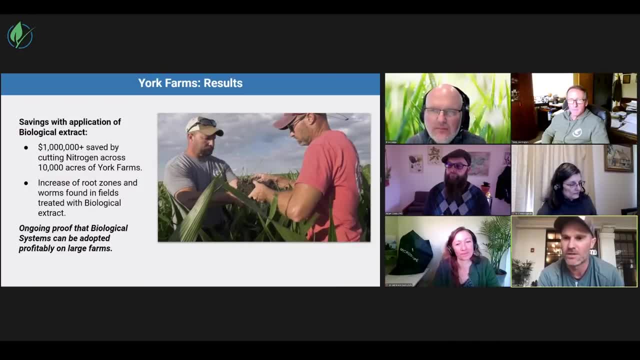 15 times more efficient. so you're just using such minute amounts and um it's making some, some really, really big results. so that's especially important. you know these trace minerals. when we're talking about the action of um leguminous plants. you know it's worth mentioning because i work with 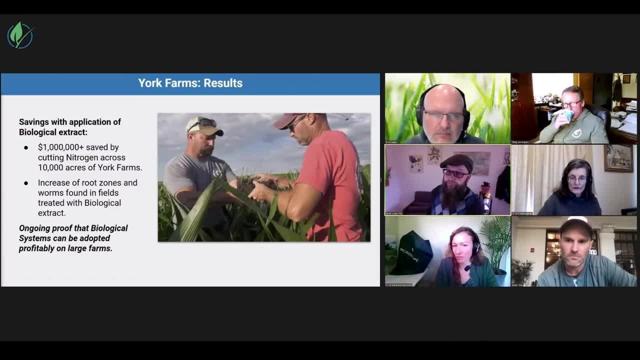 a bunch of pasture producers here in oregon um visit their pastures and all, and sometimes they are not getting good nitrogen fixation out of their um rhizobium that's associated with alfalfa or another thing that they're growing and you look at a soil chemical analysis and they have 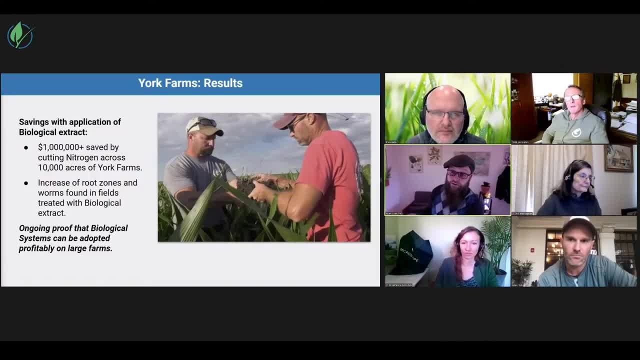 almost no boron or something else that can interrupt that process and so really prescribing, you know exactly, the trace mineral. it's something you can invest in when you're not investing so much in excessive npk, right? yeah, and adam's- adam's uh been really great. 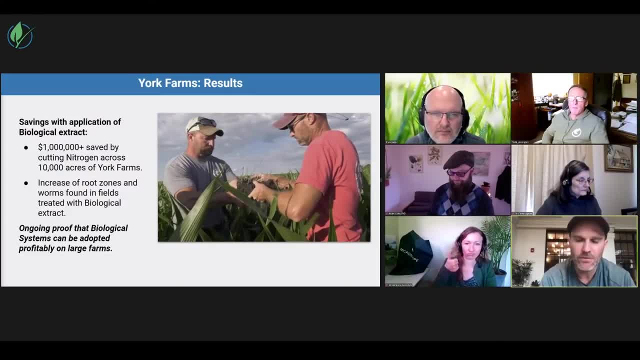 about that. you guys have been on that for a number of years now and yeah, and i mean really a lot of it has to do with understanding, really trying to know what your most limiting factor is. you know, um, biology is a big part of it. you know there's a lot of different ones and it's going to 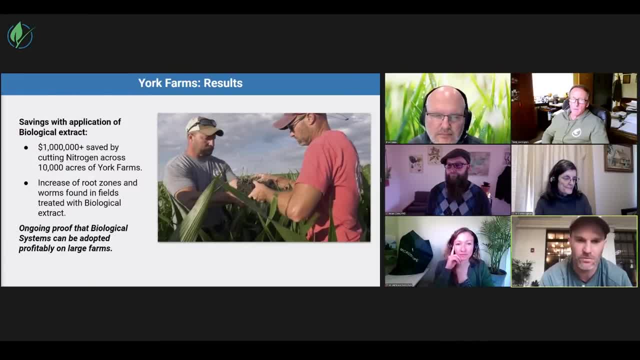 differ for everybody. you know it's just having to do your own due diligence and just try to do the proper testing and, and you know, figure these things out and really just concentrate on, on keeping a good balance of everything. can you explain which i think is fascinating, like the 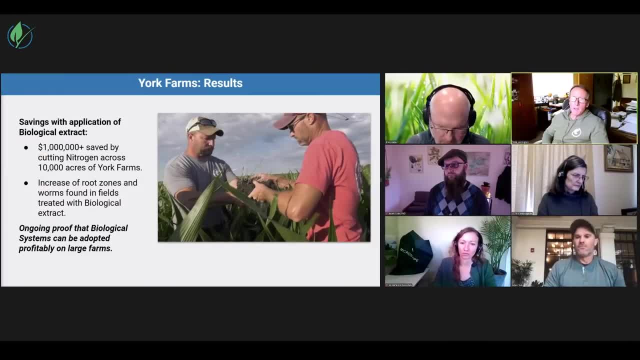 product. you know you're using quite a bit less of it and getting like what, how many times greater nitrogen on this product. so so we've, we've, uh, we, uh have a product called in hume and it's uh, more or less it's um- amine nitrogen and uh- humic acid and um, so it's a foliar nitrogen product that we use on like our. corn and it we're doing four to five gallons of the acre with 20 gallon uh mix and we will mix some kelp and in certain and like a sea crop or um other things with it and um, we're following it over the corn and you know, at the end of the day it's actually if we use 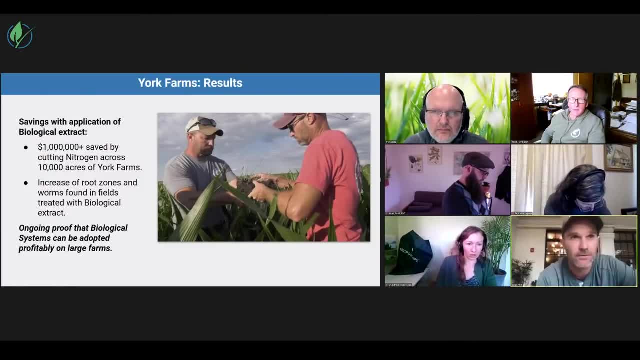 four gallon. it's like actual, like 7.6, actual units of nitrogen. but the efficiency if you're using, you know, following the, the foliar recommendations, so you're spraying, you know, under 82 degrees, you know uh, the humidity is where it needs to be. you know, some people have uh, where the moon phase is even. 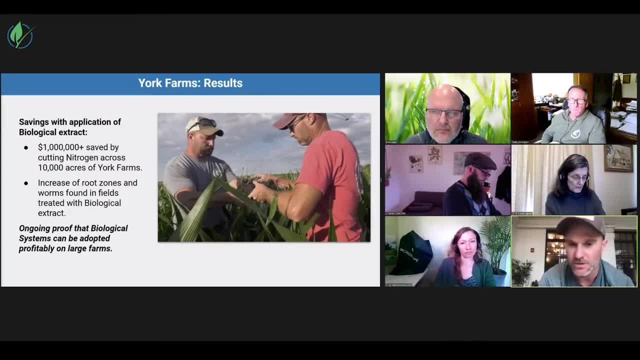 you know, if you're uh, the most efficient is uh. where the energy is the highest is six days before a full moon. so if you're doing and following all these rules, you know you're going to be able to do all these rules. that uh, this uh, this product could act like 10 to 15 times of the actual N in it. you. 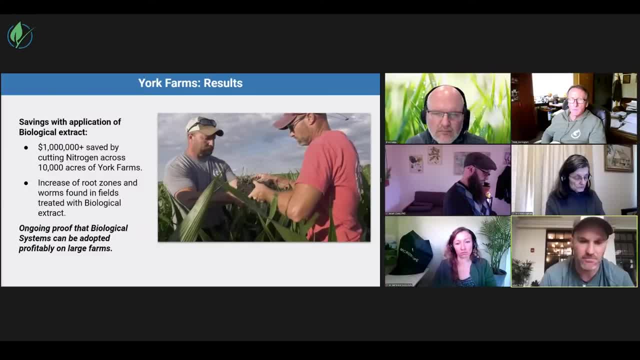 know, so you might be actually the plants actually acting like it's getting more like 80 units of nitrogen instead of just the 7.6, because it's just so efficient and it's in the and it's in a form that the plant recognizes and wants it, instead of being in like a nitrate or you know another form. 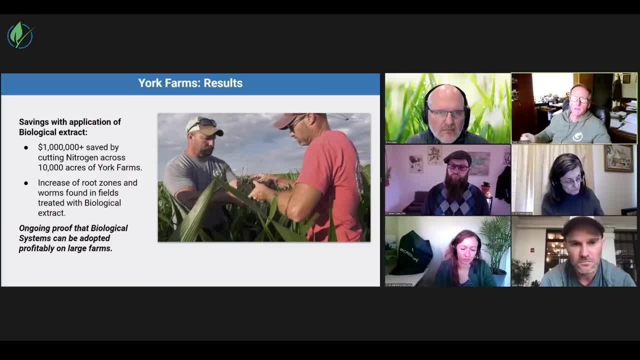 it's a really important topic because a lot of people don't understand that when they're transitioning, they want- we want to find sources of nutrients like this nitrogen form that is less invasive to biology. it's not 100 organic, but yet it's a lot less invasive to the biology and it's 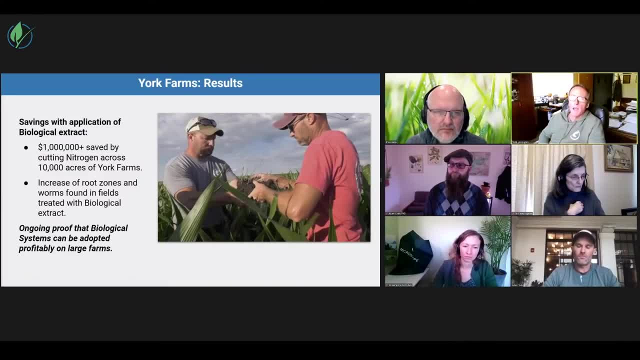 a great transitional product to use and you're using it at a much lower rate and getting much bigger Bank as your nitrogen source, right, Adam? I think it's a great. you know way to to to transition to. you know the actual organic forms of, you know like soy or something, a liquid soy or? 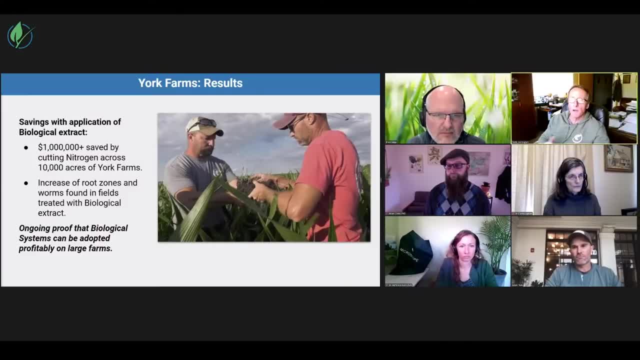 something like that, which gets really expensive, but so the cost wise, there's a real value there for folks that are transitioning from. you know. we'll just say, uh, something extreme like, um, anhydrous ammonium or something like that, or urea, you know what I mean. uh, this is a great product to. 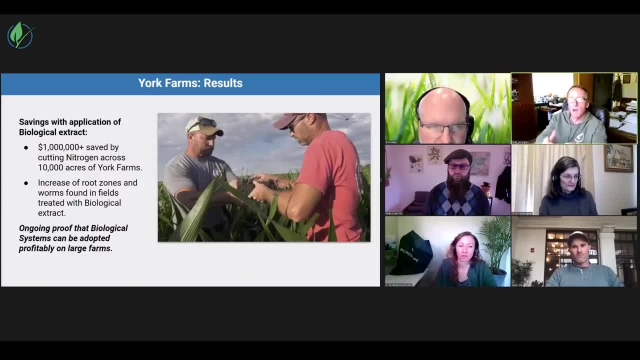 be using to during this transition. so I'm glad you mentioned, I'm glad you mentioned- talked a little bit about it, Todd. I'm really glad you brought that up, the concept of transition, because so often, um, what I run into, especially with some of my friends who are more on the traditional chemical agriculture- 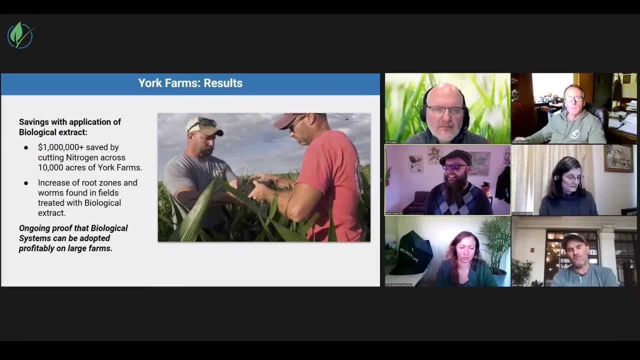 Paradigm still is that they go. nobody has the um economic capacity to do like a five-year transition and not make any money in the middle, in the middle of all of that right and it's like: well, we know there's a friend that has research that shows you can get like 150 pounds per acre potentially. 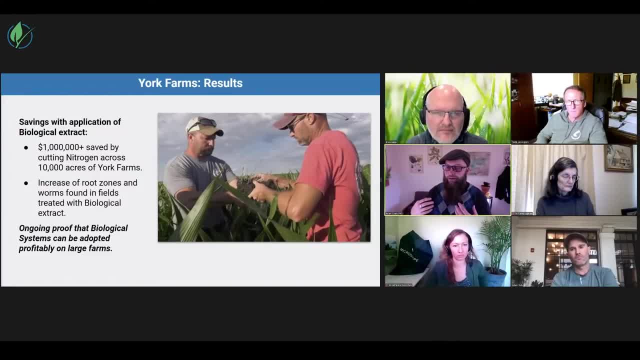 mineralizable nitrogen just from um some Vetch as a cover crop in winter, you know. and? but then how do we ease that transitionary period before your soul? biology is really taking off and running the show and keeping everything going? how do we, how do we create that um shift in the ecosystem, right? so we? 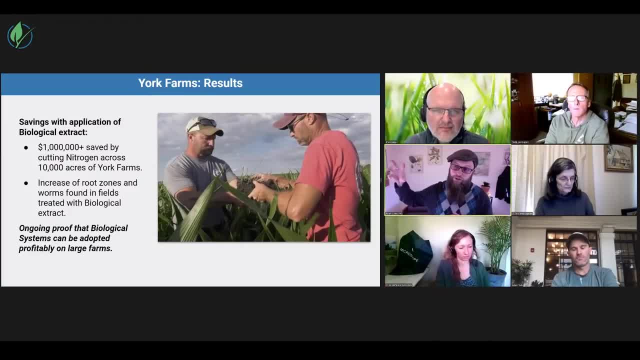 ramp it up to the right level where we really get the transformation that we're looking for, and it's such an important topic. in fact, I hope we can eventually make a whole course here at soul food web school about nutrient management through the process of transitioning. well, I think we as long 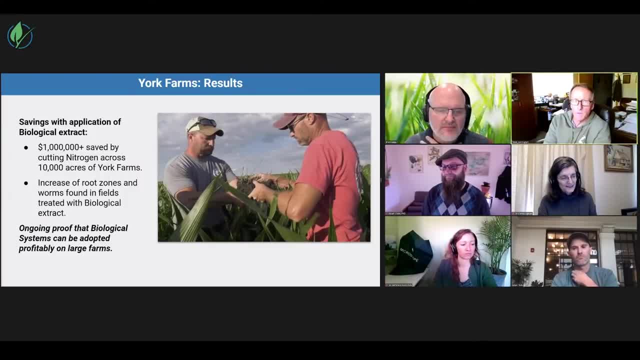 as we understand that we have all these different tools to our- you know uh, tools to the you being able to have different tools to use to and also the knowledge base to have. um, you know, it's just like you know, someone might use a a high rate of an herbicide. well, their water is really. 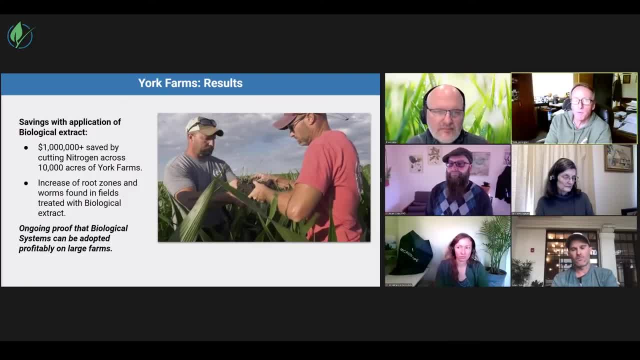 hard, and so they're only getting 50 efficacy at this full rate. well, why don't we just soften the water? I mean, there's these simple little things that people need to understand as a one of many tools to cut back on the use of these chemicals, or maybe using a surfactant, um, you know. so there's. 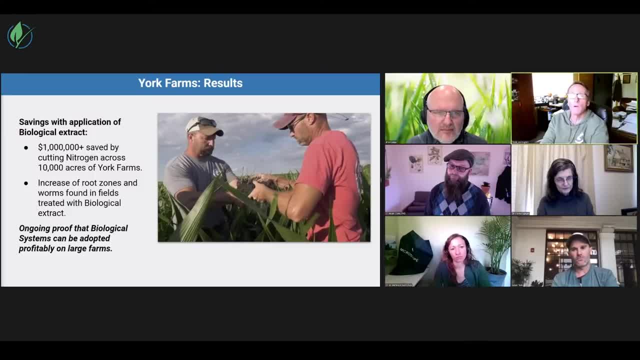 multiple tools that we have in our toolbox now that we just know, need to know or they need to have, and so Adam really done a great job at utilizing all the tools. I think the misconception that that people have, too, is that in the transition phase, they're going to be losing money. um, if you're 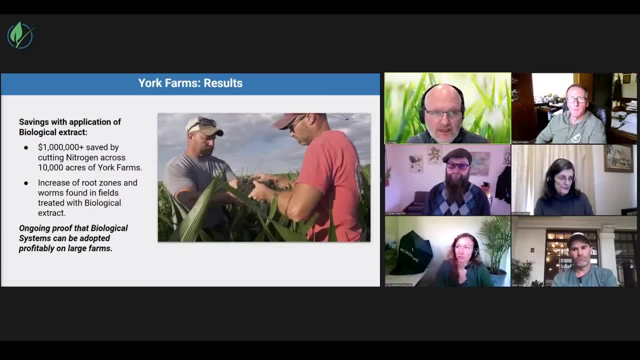 smart about. I mean, Adam's proven right here that you're still in the transition phase and you're already seeing massive cost savings. and those cost savings will tend to, you know, accelerate as you're going farther through that transition. but it's not like: oh, for five years I gotta take. 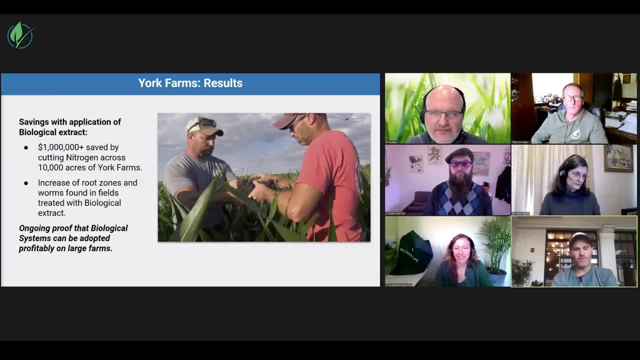 a hit financially. uh, I don't think, yeah, no, I don't, I don't, I don't think you have to, you know I don't, and I who wants to do that? anyways, you know I don't, you know so. but I think that goes back to the education: and surround yourself with with people that that, um, that. 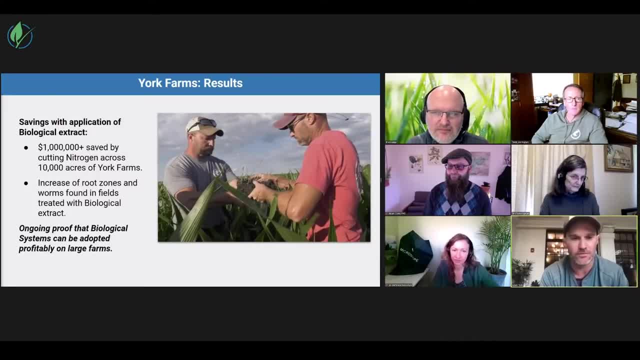 you know no more than you do at that point in time, and just learning and and trying to figure out, all right, what's the what's the best, what's the best economical way that I can do this and not go under. you know. so that's everybody's fear. you know you never go backwards and lose money. we're. 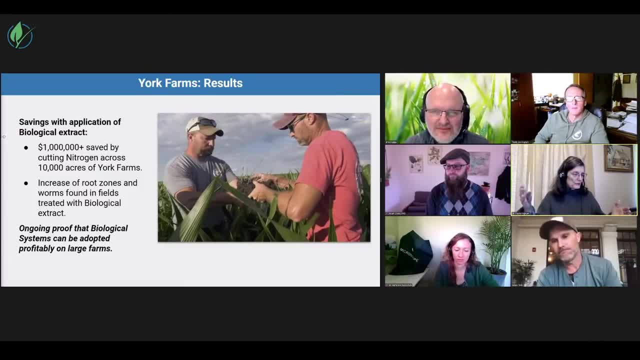 not every year. we're going to get closer and closer to the 100 goal of this is, uh, you know, up there in the stratosphere, um, in the first year we're getting, you know, 100 miles above the surface of the planet, and the next year we're going to get a little higher, a little higher, and finally, 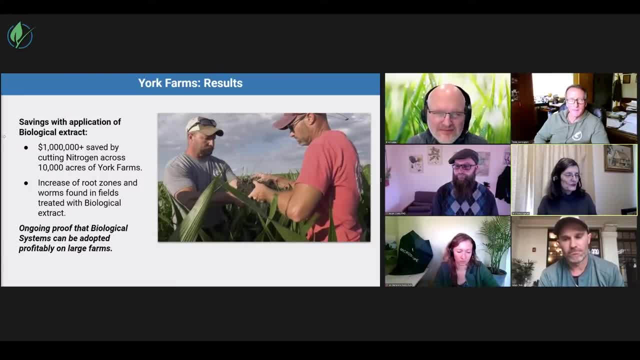 all right, we're up there now. what else can I use to minimize the costs? so it takes a little while. or maybe we can figure out exactly how we go from what we're missing to having the full food web and if we really work on it and and focus, we can get to. 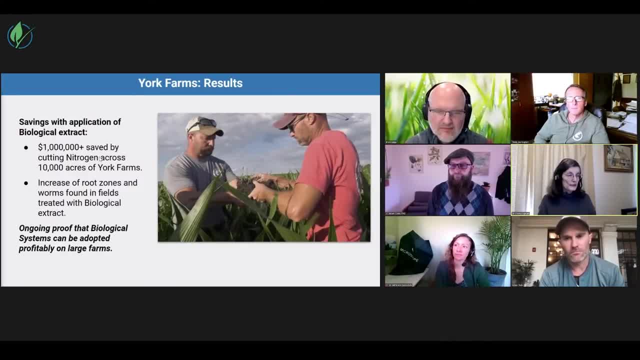 that 100 percent. the soil biology is right on what it should be, and so you can realize things in the first growing season. yeah, observation is important too. I know the last time I was at Adams one of the things I noticed pretty clearly the difference between his fields and the fall season is that he's 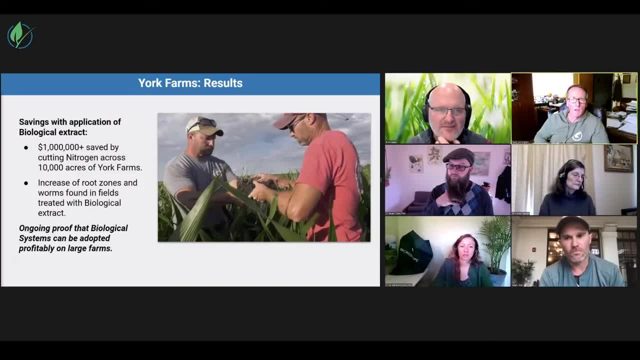 all, Adam, the residual. you know how much more coloration. you know the, the, uh, the uh, decomposing going on was quite a difference from your, the conventional fields. you know the, uh, the, the gray color that. you know that, really a noticeable difference. and you know this last, uh, I don't. 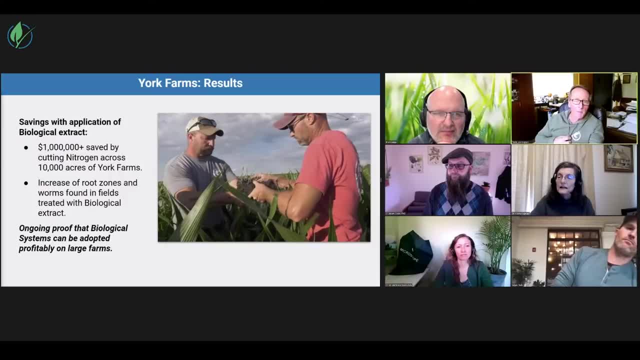 know if this is the last slide, but it talks about, you know, ongoing proof that biology systems can work well. visually, those are the. you know you mentioned earthworms and and then also the rhizomorph and the mushrooms now that we're seeing in your fields. they weren't. 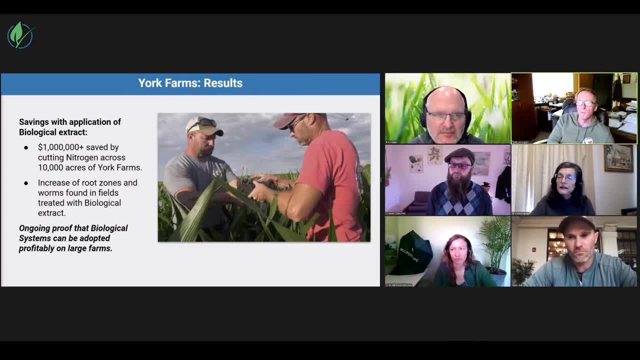 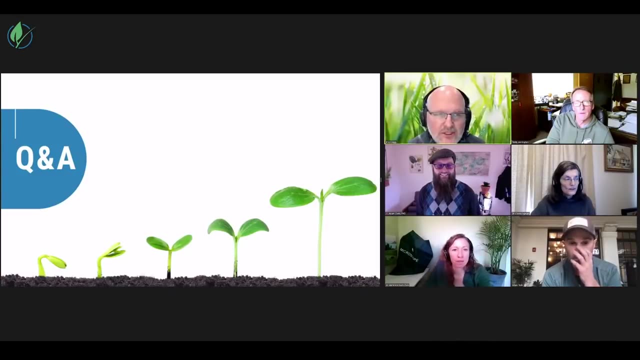 there before, but this fall residual program that you guys have has looks- I mean, visually you can really see it right- so fantastic. I love it. just as a timekeeper, I know we're getting the very end of this. what I'll actually Adrian. can we throw the one last question? I think this is a perfect 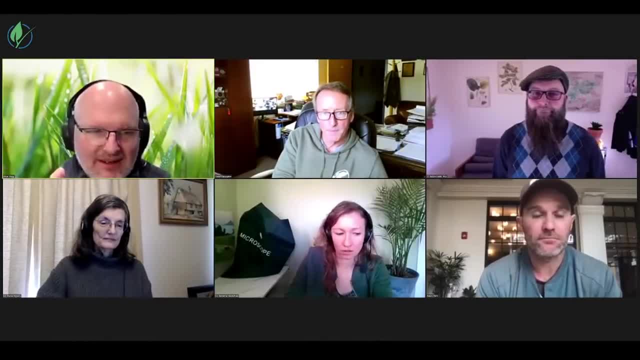 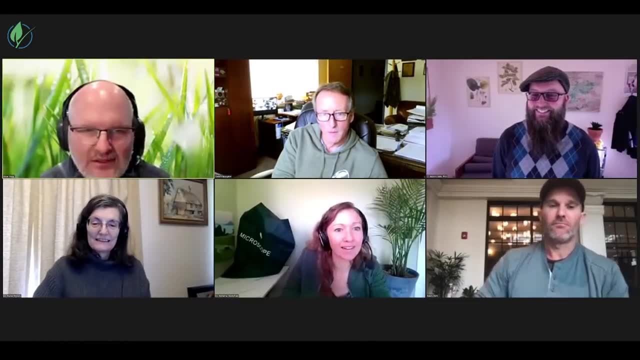 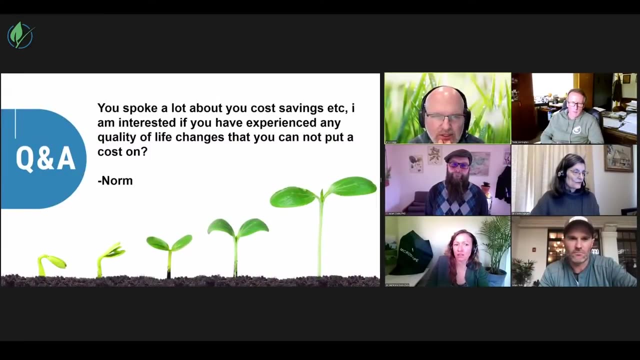 question for Adam to kind of end the Q a on um. sorry to put you on spot like that. you're good, reset, here we go, no problem. but, Adam, this question is is really for you and I think this is a great webinar, and the question is from Norm, which is: you spoke a lot about your costumes, Etc. I'm interested. 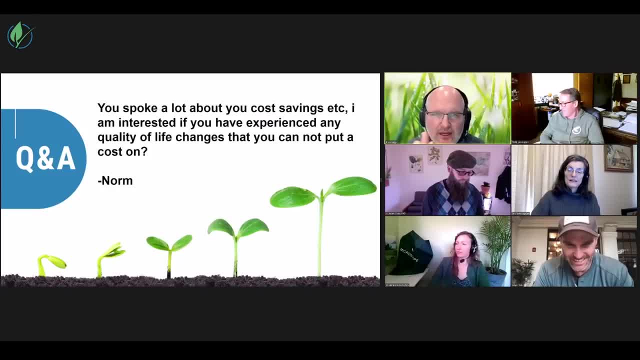 if you have experienced any quality of life changes that you cannot put a cost on. I think this is a fantastic way to end this. yes, that is a great question. I love that question. yes, um, I'm going to bring up a story, um that back when we were we were we were planting. um, you know, everybody was like, hey, we need to get more. 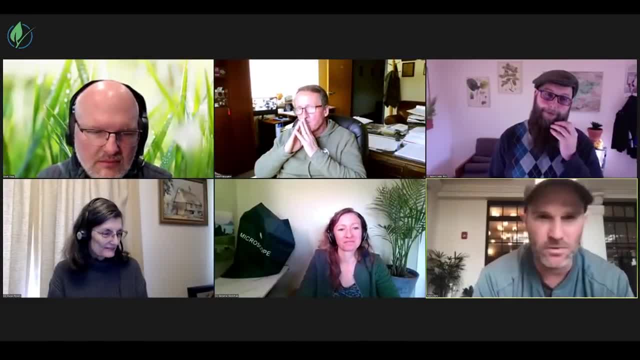 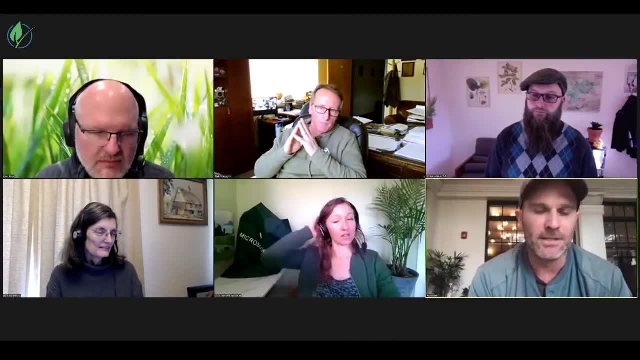 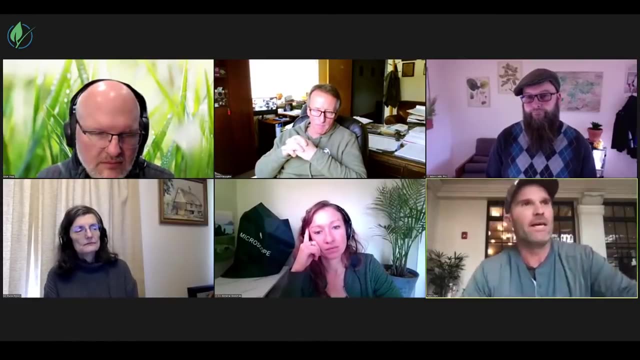 yield, more yield, more yield. that's what everybody talked about, and so that was more insecticide, more whatever. I got to a point where I was loading the planter with a product- uh, liquid or liquid insecticide, and I got some on my hands and I was planting corn and I couldn't feel my legs for about.